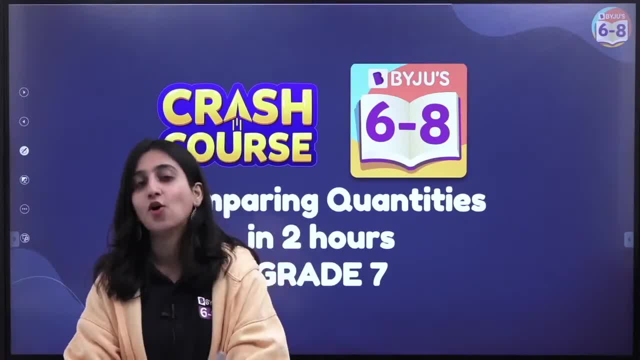 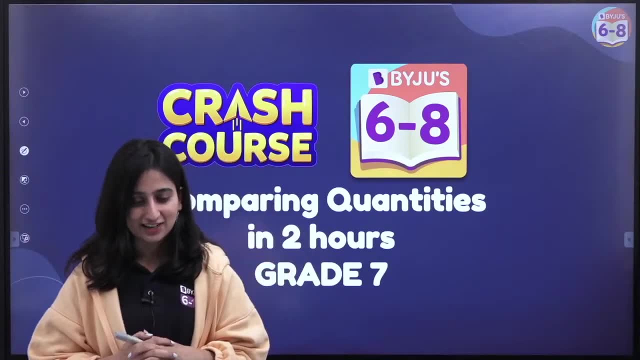 if you are new to the channel, make sure you subscribe to the channel. If you are new to the channel, also hit the like button right Welcome, welcome everyone. Welcome to your favourite channel by juice, grade 6, 7 and 8.. Hi Sneha, hello Jhanvi. hi Sanket, hi Vidhi. 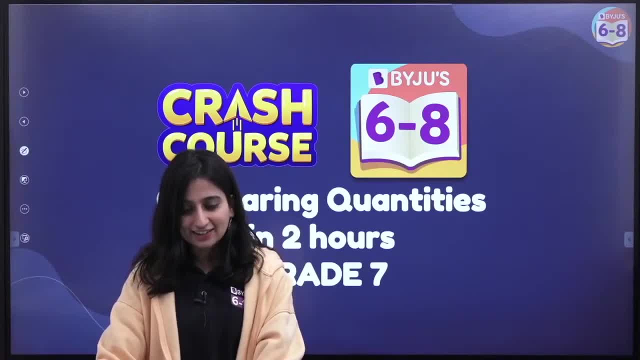 hi Aditya, welcome to the class bache. Hey Vani, hi Jhanvi, hi Nagaraj. Ok, so I am completely audible and visible. yes, Good evening, good evening everyone. Hi Miss Unique, hi Manish, hi Anjali, hi Anjali. Good evening everybody, Chalo. So let's dig into the session. So today, 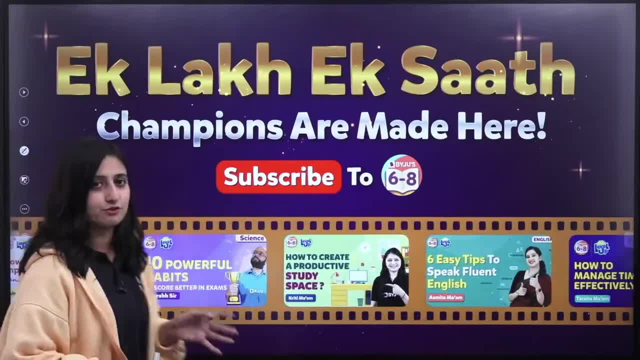 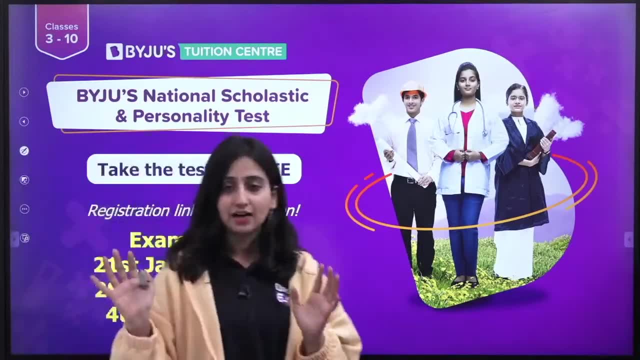 we are going to cover comparing quantities, and you know that you have to subscribe to the channel, ta ki aap koi bhi important session miss na karo. And aap logon ke liye ek bahut important personality test aa raha hai. Laaya gaya hai. So aapko iska link description box. 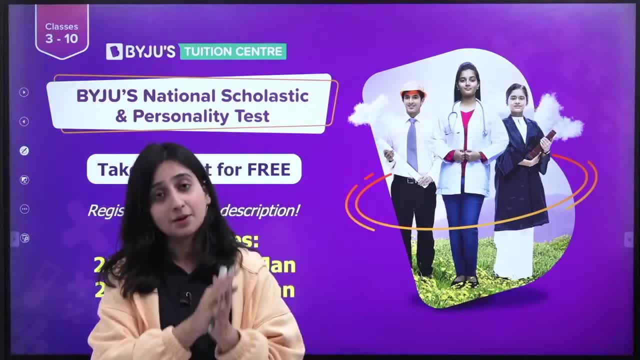 mein mil jayega. So make sure, if you haven't register for the test, aap abhi bhi register kar sakte hai. So test ki dates yahan pe dekho. de rakhi hai Toh aapke paas abhi 4th and 5th. 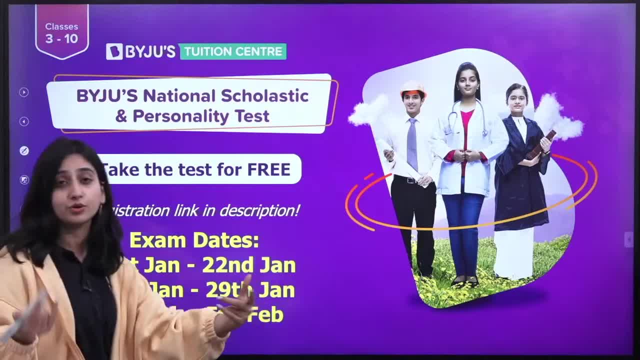 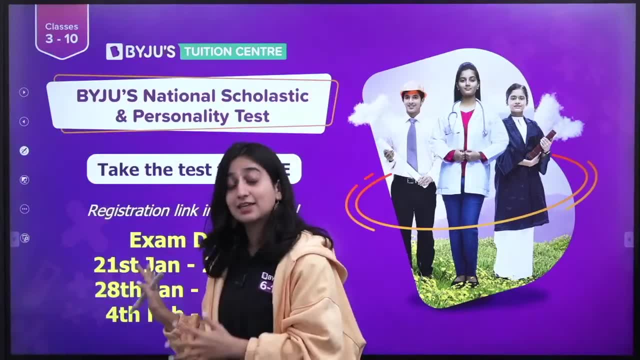 February ko, that is, tomorrow, you can give the test, and or day after tomorrow you can also give this test. Toh iss test ki liye you just have to visit the Baiju's tuition center and kyu dena hai, kyu aapko bola jana hai ki iss test mein bethiye, iss test ko attempt. 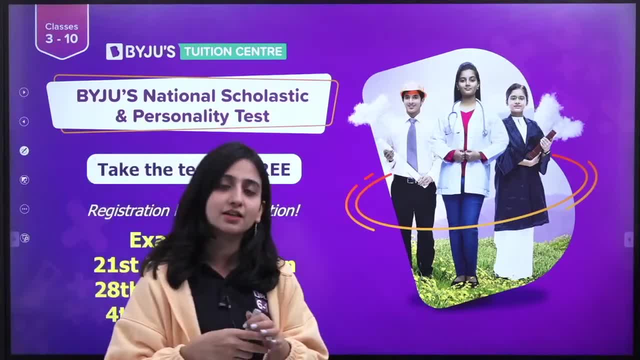 kajiye, Kijiye, kyunki aapko iss se pata chalega, ki aap kahan pe stand kar rahe ho, Aapko aage career mein. agar aapko confusion hai, ki mujhe kya bharna bade hoke, Tike toh aapka confusion. 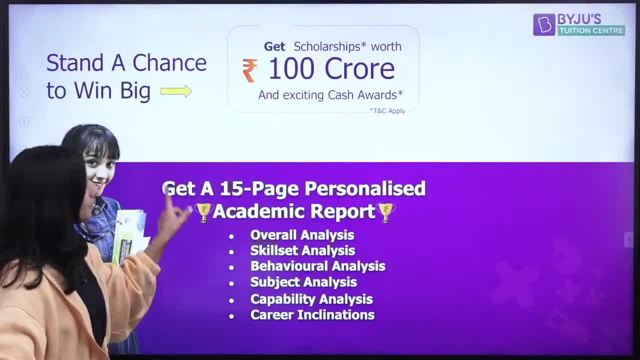 door ho jayega Aap, ma'am, kaise door hoga? confusion, Kyunki aapko, aapke test ke baad aapko ek 15 page ka personalized report generate karke diya jayega Jisme aapke saare. 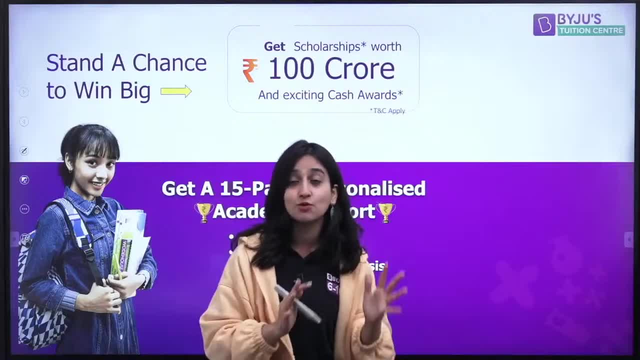 skills is. in sections mein aap strong ho, in sections mein aap weak ho. kahan pe aapko zyada work karne ki zurwat hai? kaunsa career aapke liye best hone wala hai? ya, agar aapko 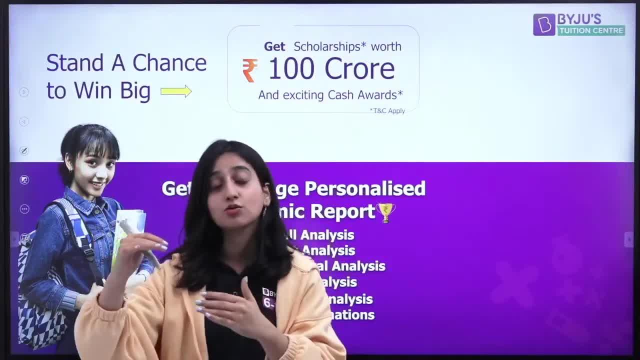 koi different career choose karna hai, toh uss career tak jane ke liye aapko kaunsa road map follow karna hai, Woh aapko ek pura, ka pura idea lag jayega, if you appear for this. 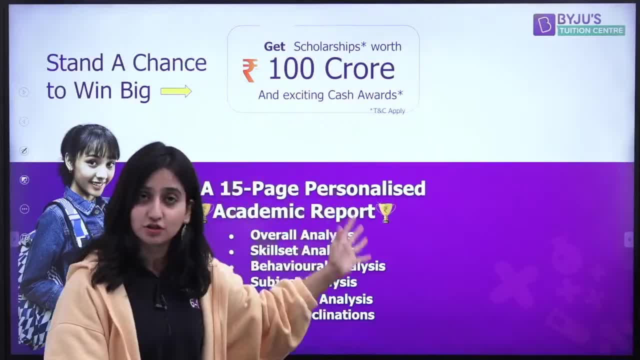 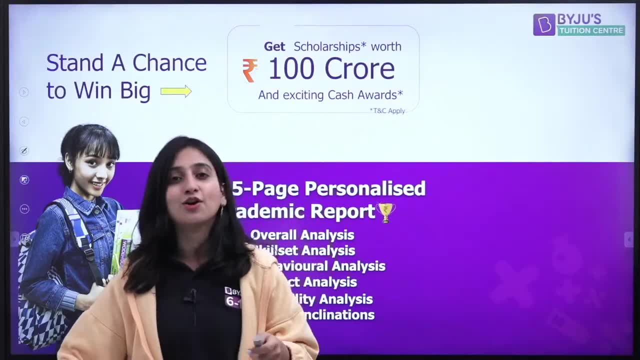 test Tike. So make sure you appear. just register for the test. It is a free test, Tike. Bas jana hai Baiju's tuition center mein, aur appear hona hai Tike. So it is very important for all of you. Make sure you register yourself. Okay, Now let's go to the next. 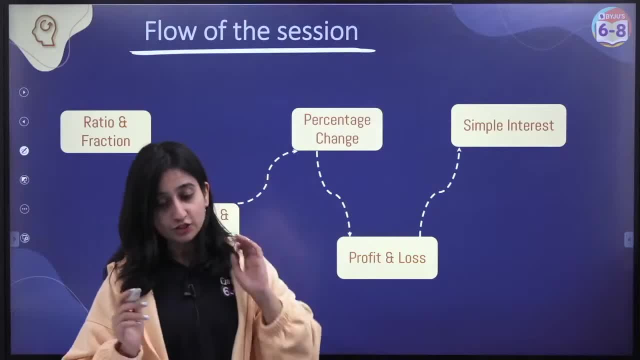 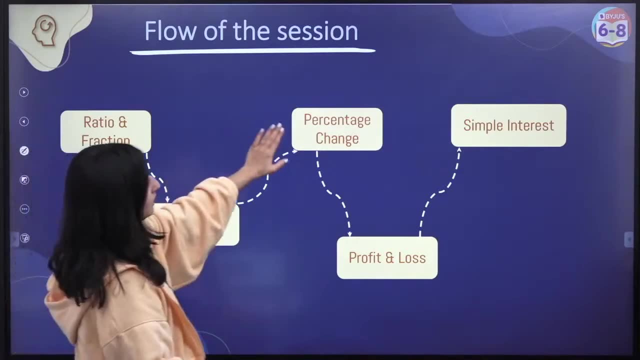 part. Let's discuss how the flow of the session is going to be Okay. So, sabse pehle, we are going to cover what is the ratio, what is the fraction, then what are percentages and what are the conversions. we are going to study then percentage change, then we will move. 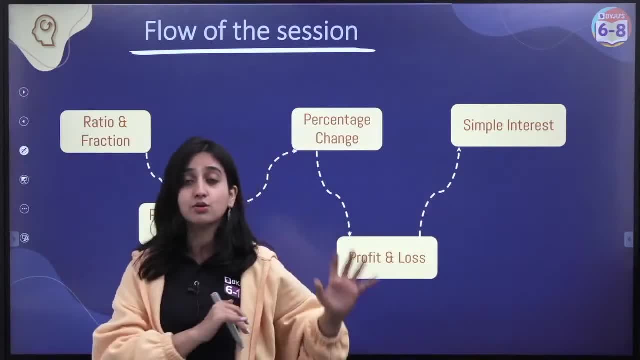 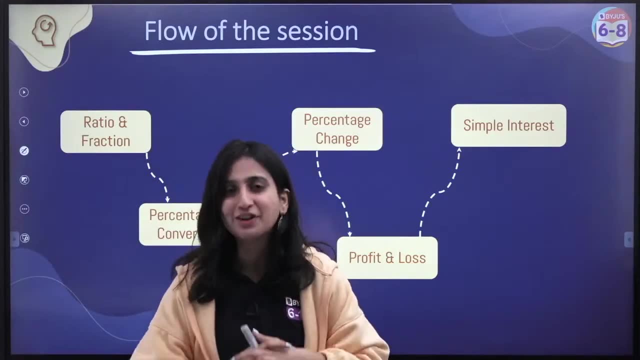 to profit and loss and then simple interest. This is how we are going to cover all the concepts in this particular session, and after that we will be solving few questions, and then we are going to have a mentee quiz. Okay, So I hope you are excited, Everyone. Yes, bacha. 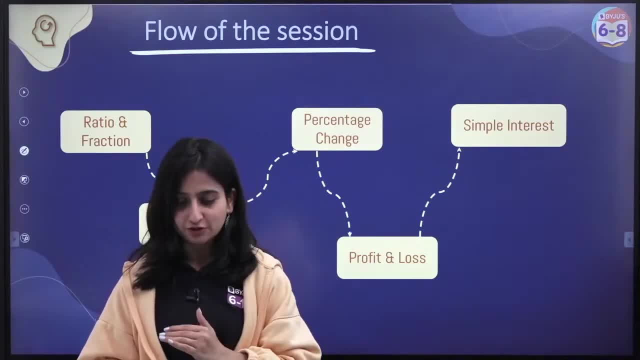 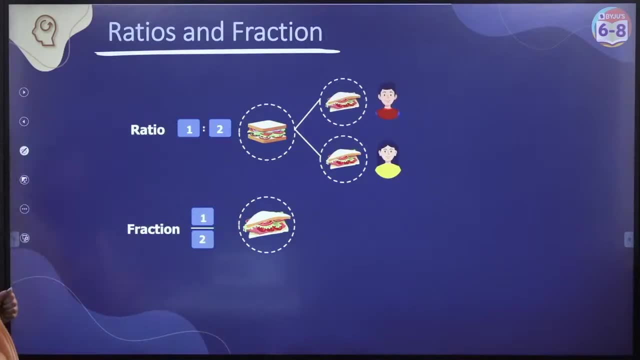 aaj hum sab kuch karne wale hai. Isi session ke andar aapko sab kuch mil jayega, Tike. Okay, Yes Hi Gulzar. Hello Vikash Hi Jamna. Welcome to the class, bache. So let's first. 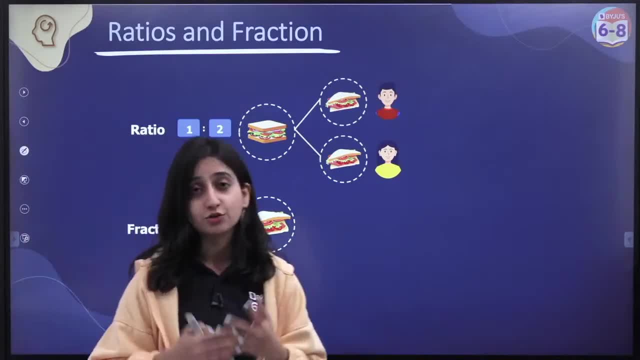 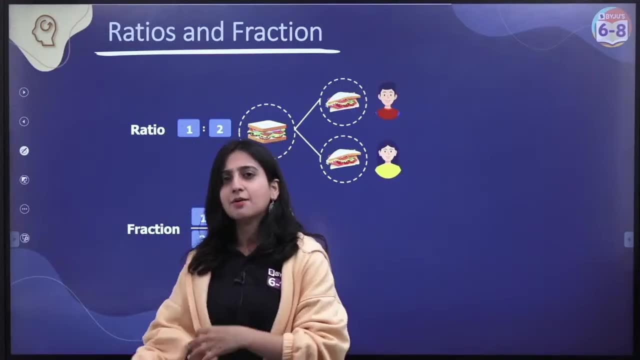 talk about ratios and fractions. Can anyone tell me what is the ratio? We have already covered this chapter. Mene aapko ye chapter pehle bhi padha diya hai. Tike Toh koi mujhe batana chayega, ma'am, what is ki ratio? kya hota hai? Can anyone tell me what is the ratio? 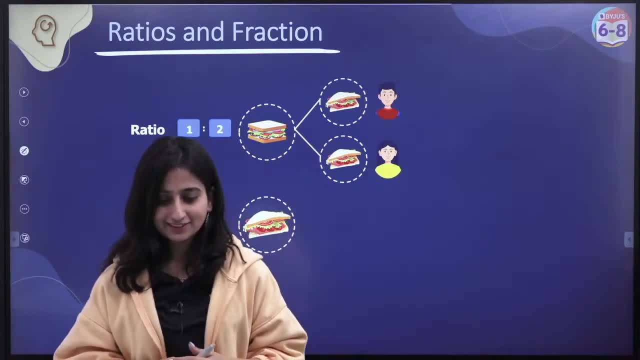 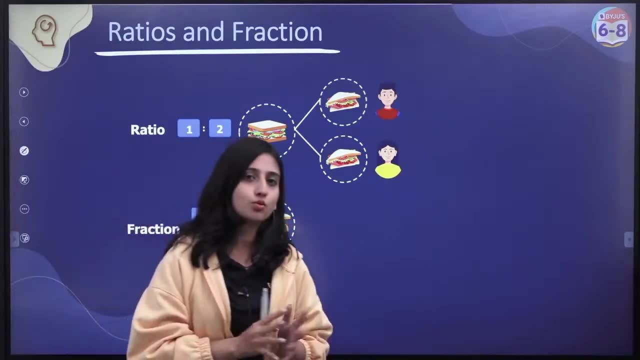 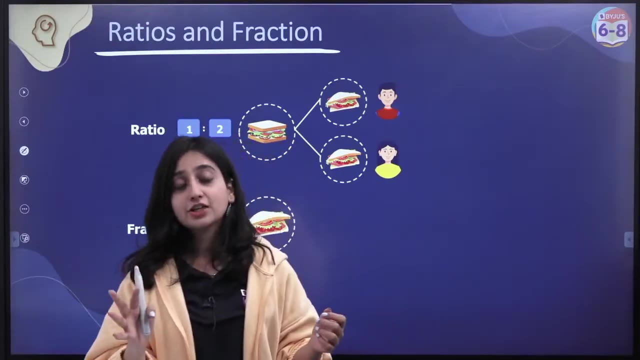 Yes, Yes, everyone. What is a ratio? Dekho, jab bhi hum, whenever we want to compare two or more quantities, Tike, We take help of the ratio. Ratio is one of the way in which we can compare few quantities. The main condition kya rehti hai? yaha pe compare jinko bhi hum kar rahe hai. 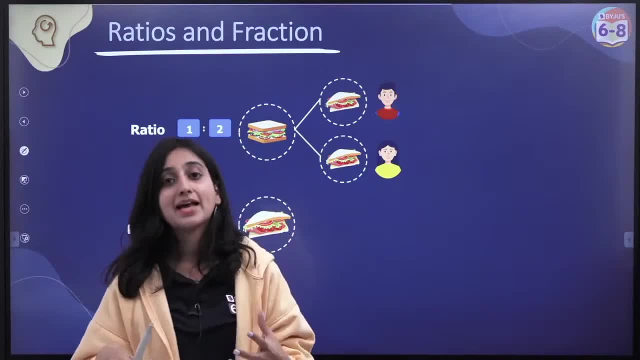 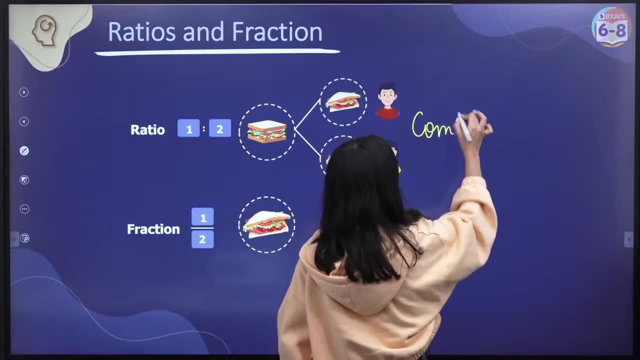 un sab bhi quantities ka unit same hona chahiye. Tike Comparison. Toh basically ratio kya hota hai? comparison by division. Agar main bilkul ye simple language mein aapko bataun ki what is the ratio, It is basically comparison by division. So basically ratio means the 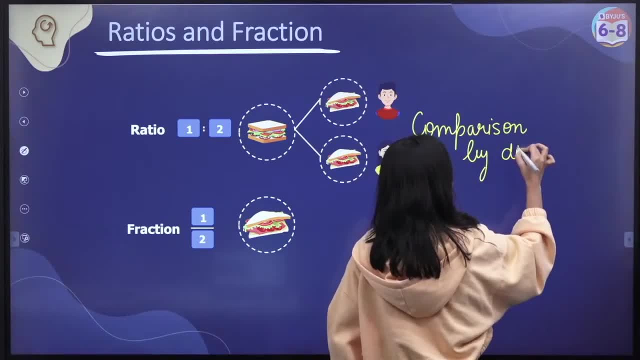 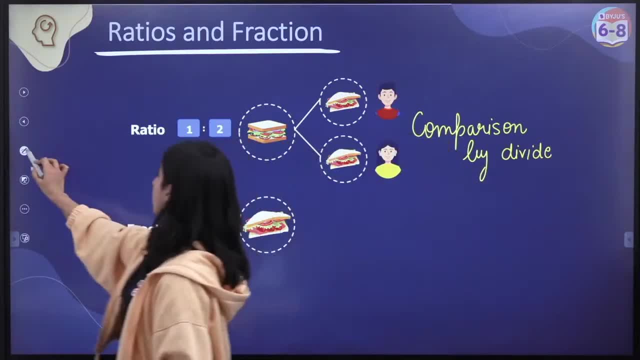 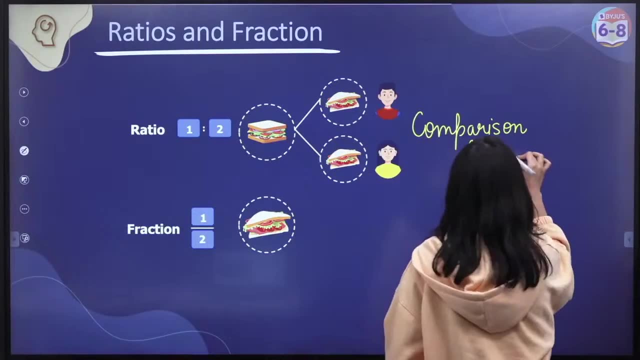 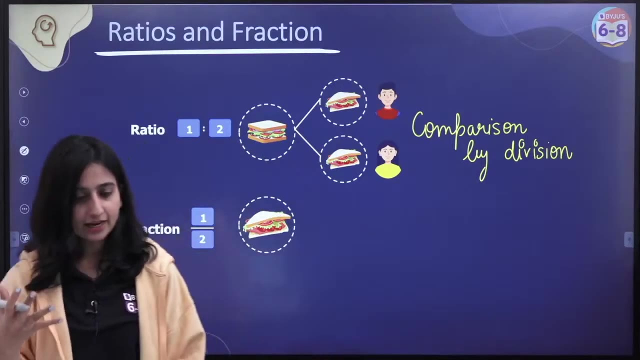 by division. Matlab hum 2 terms ko divide karte hai aur unko compare karte hai: Tike. So ratio or fraction mathematically beta equal bhi ho sakte hain. Comparison by division. We can call it a ratio Tike, For example Example. koi mujhe batayega Example kaise? 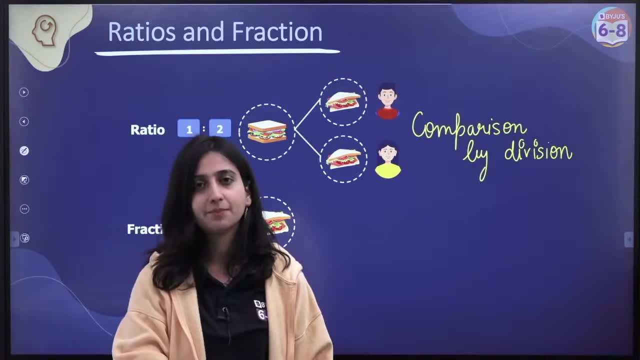 le sakte hain Kisi bhi 2 cheezo ka, agar mujhe ratio le nahe. For example, I want to take the ratio. One car is going at the speed of 5 kilometres per hour, So what will I do? 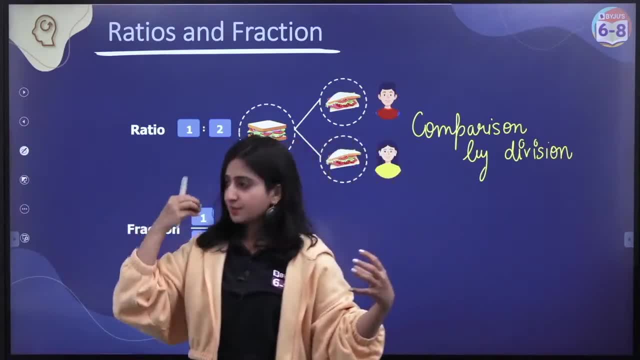 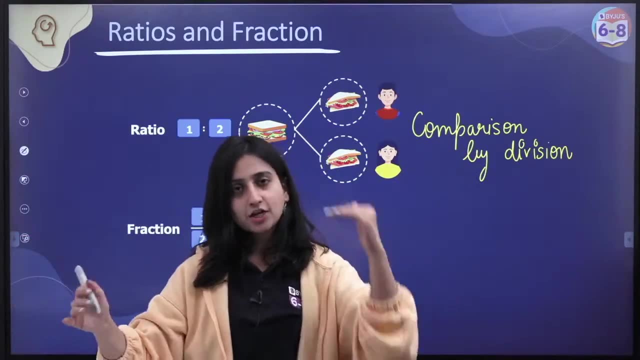 I want to take the ratio. One car is going at the speed of 5 kilometres per hour, Or 1 car is km per hour, the other car is going at the speed of 20 km per hour. how am i going to compare these two speeds by taking the ratio. i will take the ratio of both the speeds, so 5 upon 20 i will get. 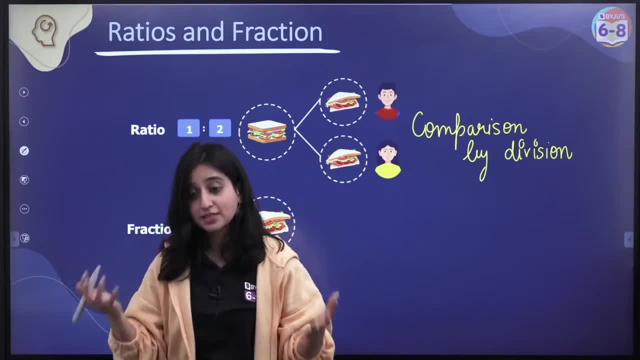 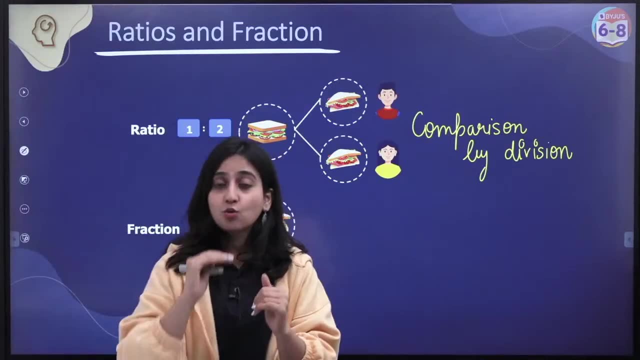 1 by 4. right, so this is how we take ratios. okay, so basically, ratio kya hai? comparison: jab kiya jaata hai 2 ya 2 se zyada quantities ka divide karke, okay, ab ye jo quantities hai. bahut important baat hai. jab bhi aap ratio loge kisi bhi 2 quantities ki, make sure ki unke unit same hai. 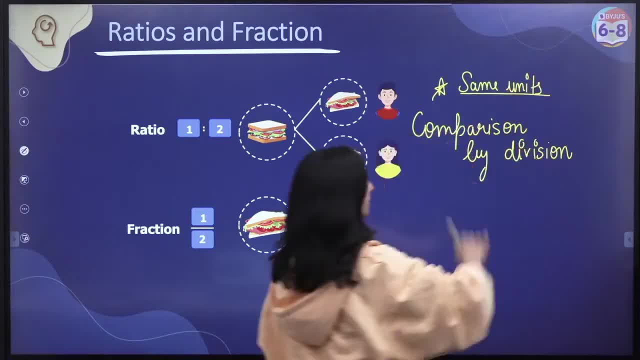 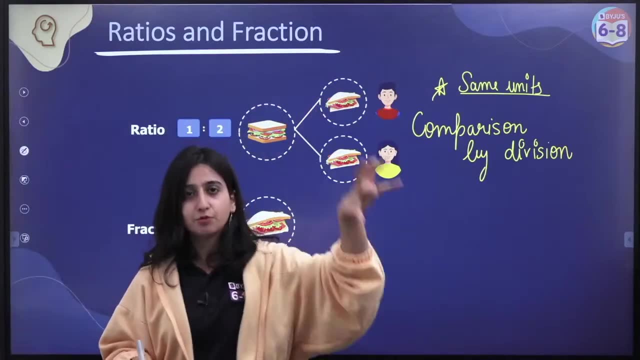 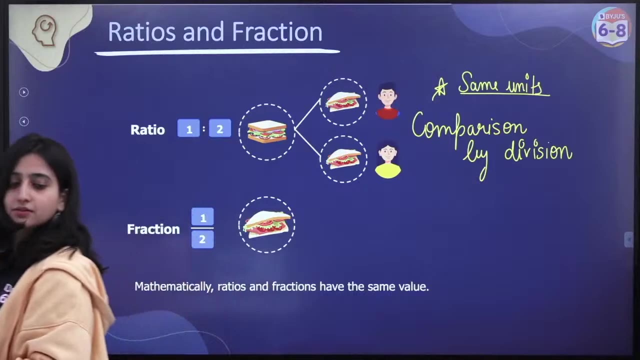 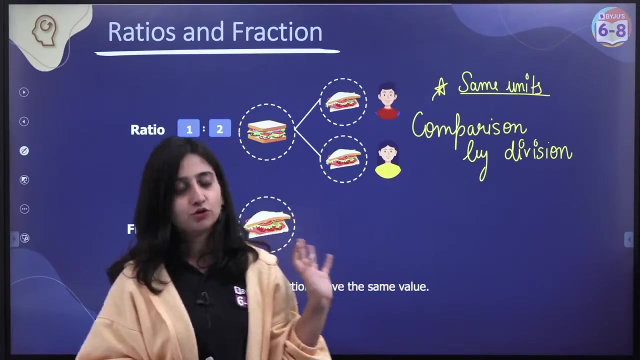 unit same hona. bohot important hai nahi to answer galat aega aapka thike and fractions. aapko pata hai fraction kya hota hai? part of a whole kisi poori ki poori cheez ka, agar ek part ki baat, okay, yeah, its fine. now alright. so i hope this is clear. toh very basic cheez. 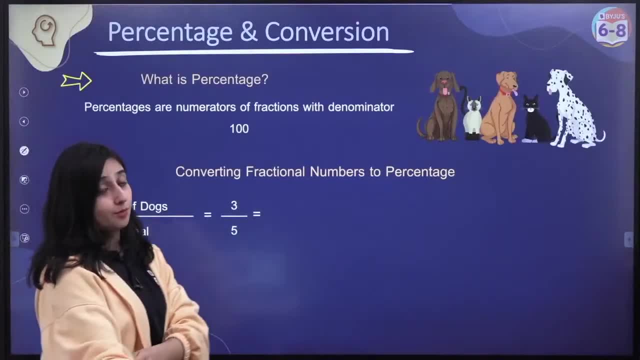 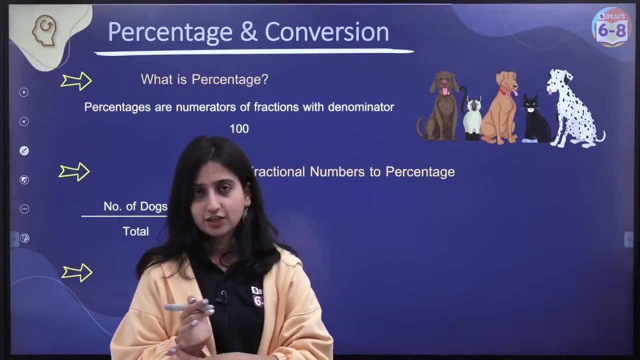 humne abhi pada hai ki ratio aur fraction kya hota hai? then, very important thing, jis me se aapko question pucha ja sakta hai, that is percentage and conversion. now, what is a percentage? kya pada tha, percentage ka matlab kya hota hai? bacha percent naam me hi answer. 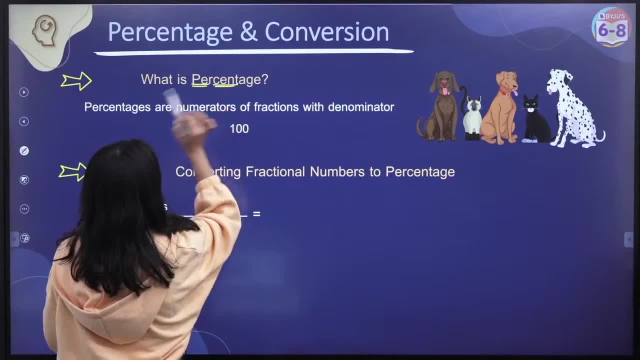 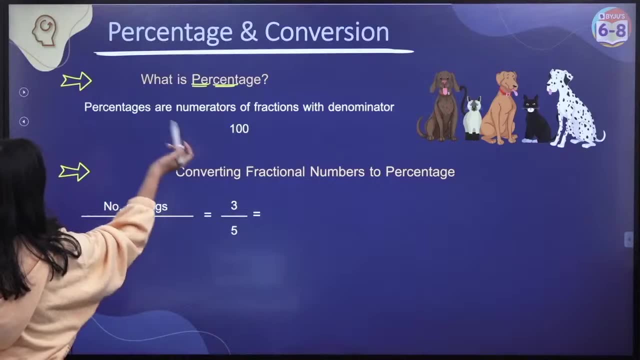 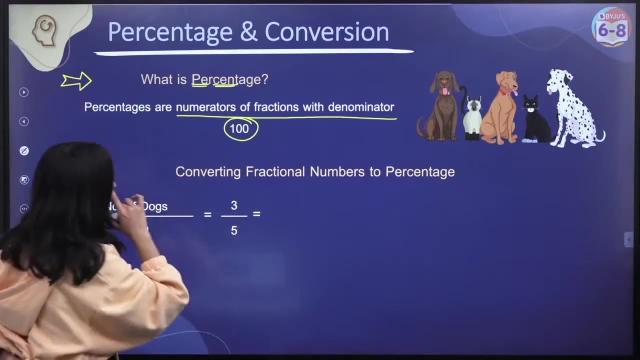 chuppa hua hai. per ka matlab, divide me aur. cent ka matlab hota hai hundred, thike. per ka matlab by hundred, toh matlab hum. agar we are taking percentages, kya hota hai? basically, numerators of the fractions with the denominator hundred. that means itka matlab ye hai percent. 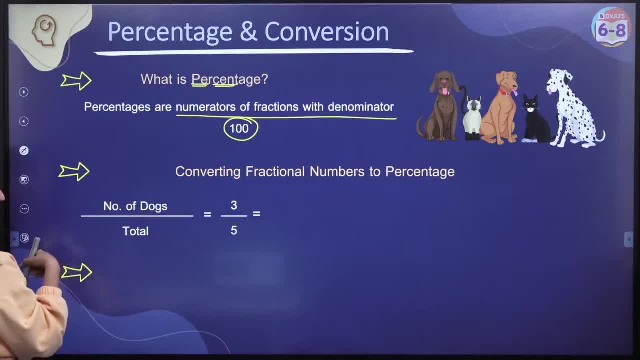 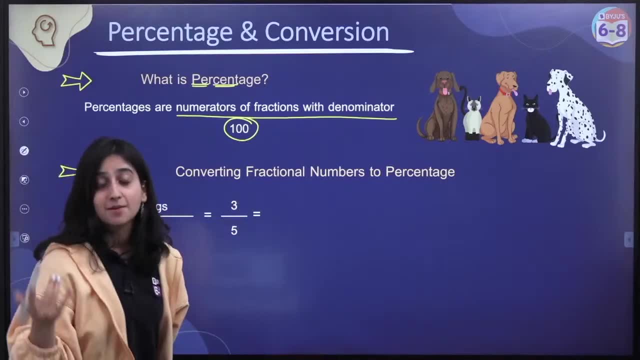 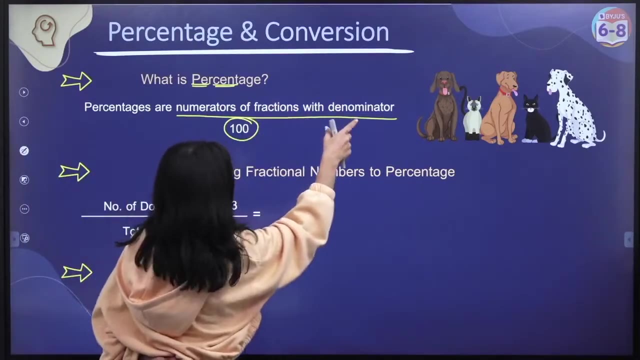 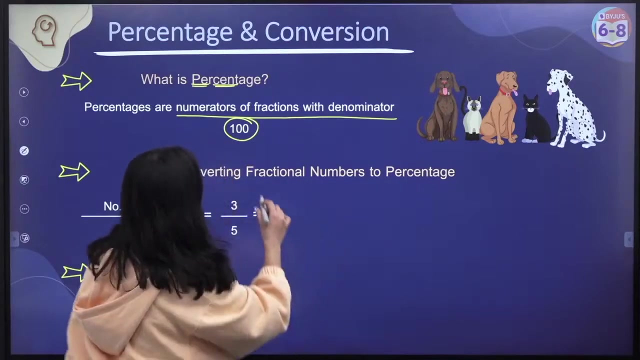 cuts are only собственно, in case you can only understand, of the fraction. so, for example, i am taking number of dogs to total ratio. im taking this ratio. now i want to convert this fraction or this ratio in to percentage. meire usko percentage. me convert kana chaati, toh mai kaysi karungi. my provoy percent are numerator fraction with denominator hundred. tike aapko denominator ko sabse pehle hundred banaan paadeyga right, so yahap post kya banayenge denominator hundred kaysi banaayega multiply this 5 x, What five? 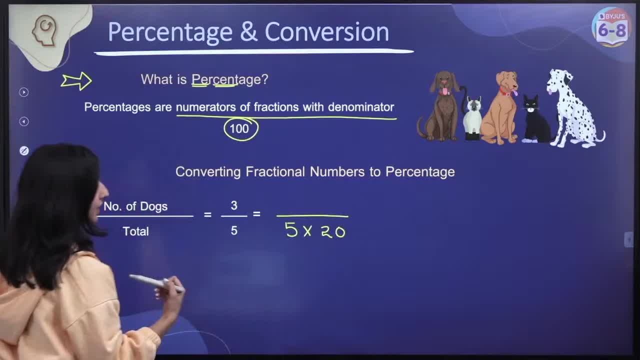 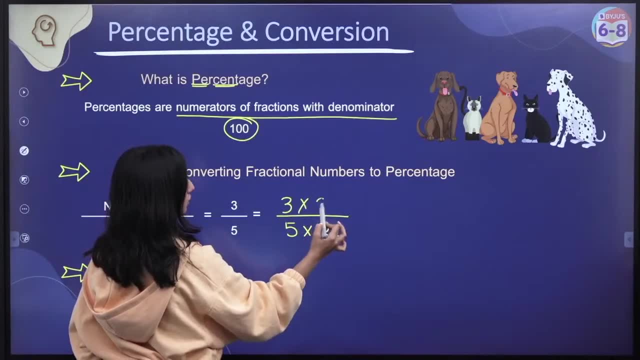 ko kisse. multiply kiya jaye 5 ko 20 ke saath agar mai multiply karu to, ye denominator will become 100 right. so if i am multiplying 5 by 20, i have to multiply numerator also by 20 right. so i will. 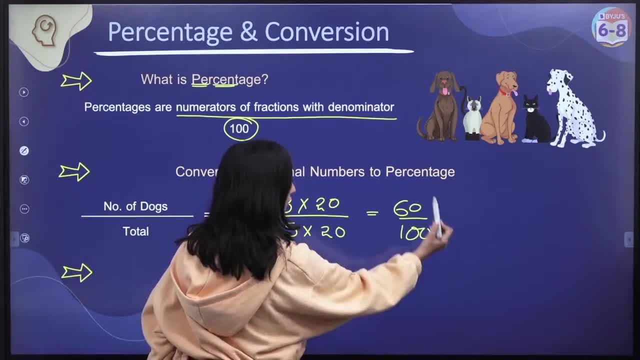 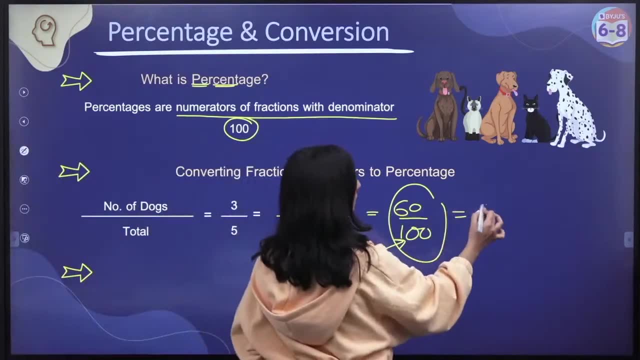 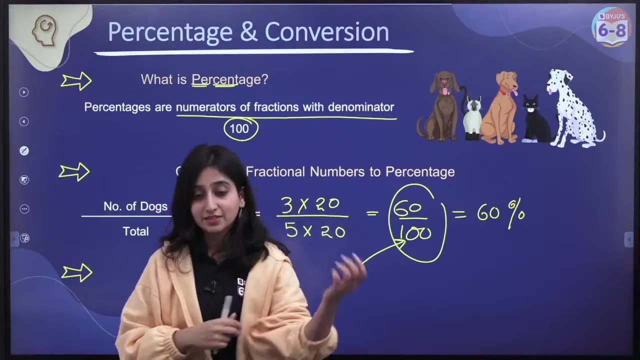 get 60, divide by 100. now we got a fraction in which the denominator is 100 to percentage kisko bula jayega. so this 60, it will be equal to 60 percent. that means per 100, that means divide by 100. the percentage is tarike se li jaati hai and percentage sabse zyada effective way hai to compare. 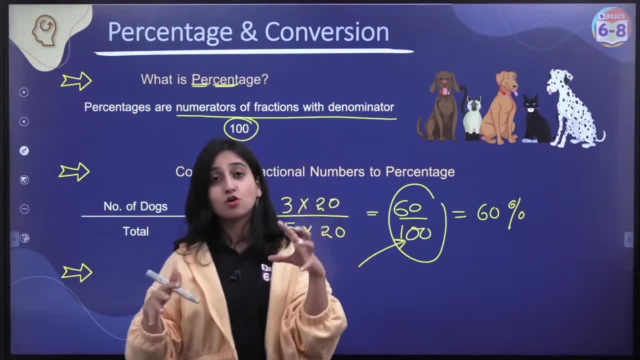 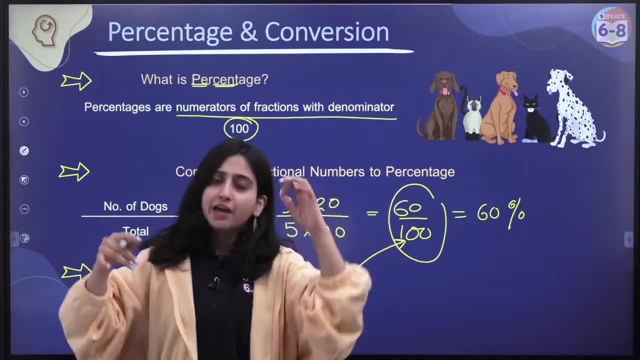 the quantities tike, kisi ke, kisi ko, kisi bhi 2 ya 2 se zyada quantities ko compare karne ke liye, percentage ek bahut hi effective tarika hai. if you remember, if you have watched the one shot to one shot, me ne apko. 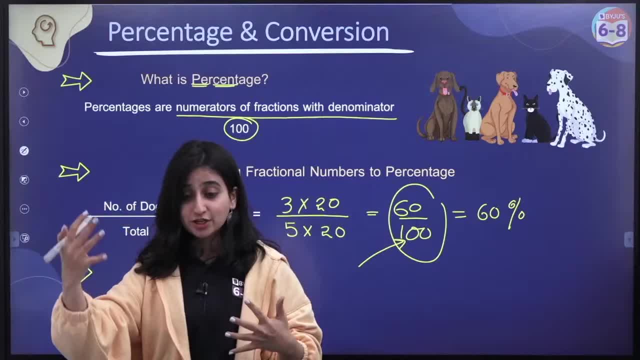 ek example diya tha. suppose, ma'am bhot bacho ke dimaag me question aata hai ki: ma'am, why are we studying percentage? kyun padha rahe ho, jab amare paas compare karne ke liye? ratio hai amne ratio. 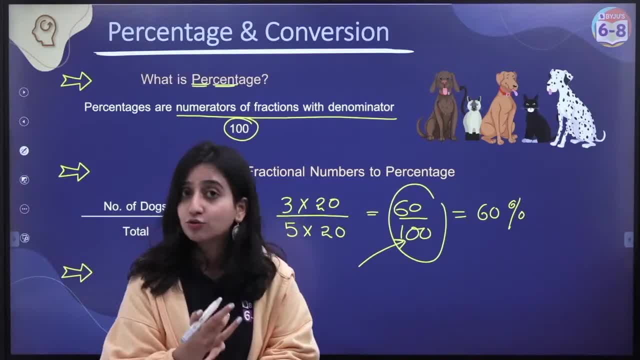 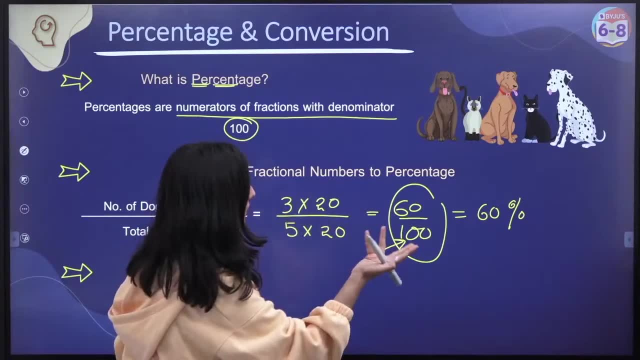 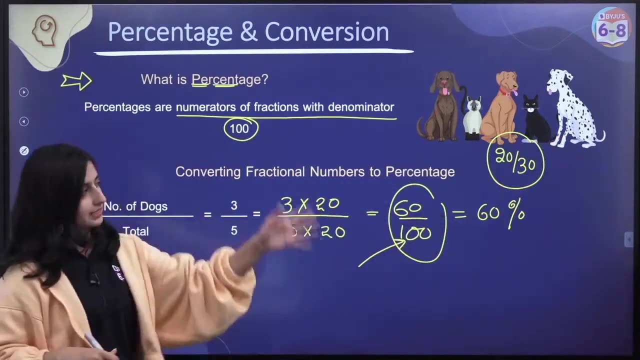 sikhi hai, why we are studying about percentage. to ap meri baat suno. suppose ap kisi apki class me test hua hai. tike 2 bache, student a and student b, maal lo ki student a ke marks aaye hai 20 out of 30 maal. lo ki student a got 20 out of 30 marks. ye kisi hindi test ki baat. 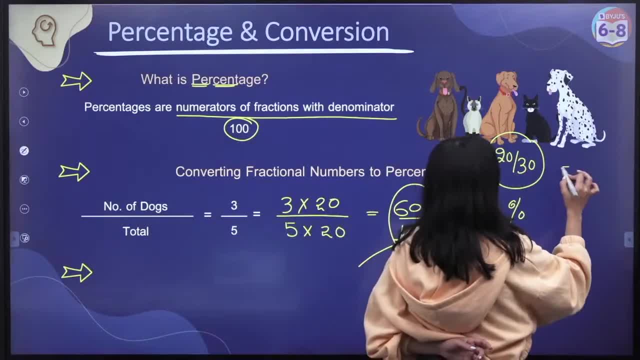 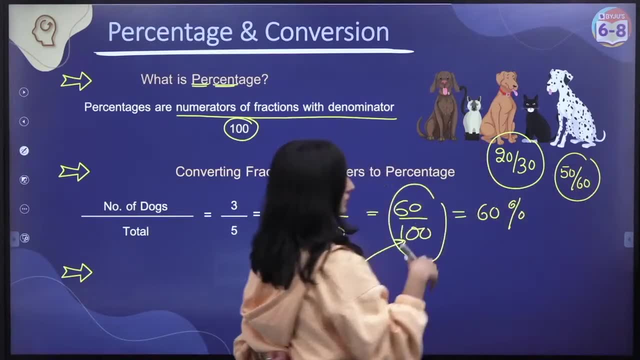 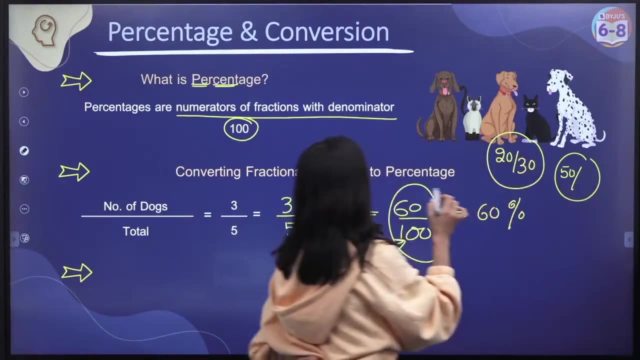 kar rahe hai and ek aur bache ka test hua hai. pass ahi hai. us k marks aaye hai 50 out of 50 out of, let's say, 70, 50 out of 60 marks. aaye tio hum in dono bacho ke kaise compare karene inke marks hum. 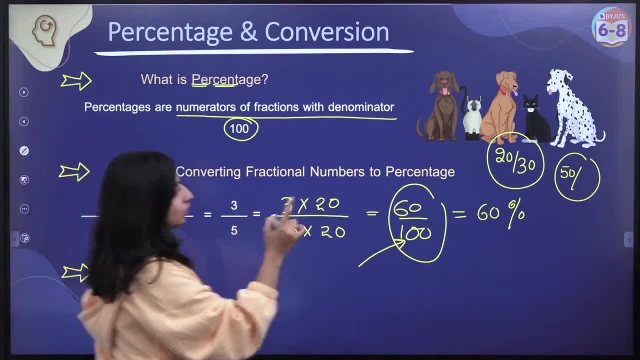 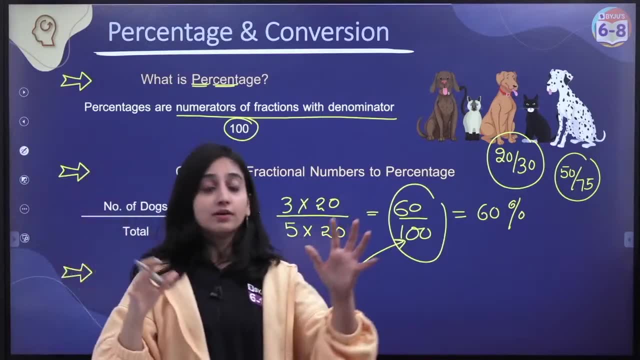 compare karene aap. kya ye bolo: ki dono bacho ne equally good perform. kya hai ki aap aisa bol sakte ho? ki dono bacho ne equally good perform. kya hai? nahi, jab hume in dono students. 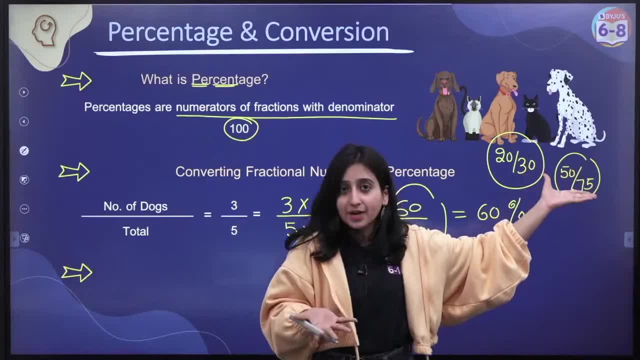 ki students ke performance. ko compare karneon ki marks? kya compare karneon ki ask? starts na testamentine sayin interessan mi writer, so apne bachi to destude kumm me 가el se пошlainna giye sa b посetka haiaro. okay, uta co llegh n yourself heir, that Bapisi have come from. Rand. view of 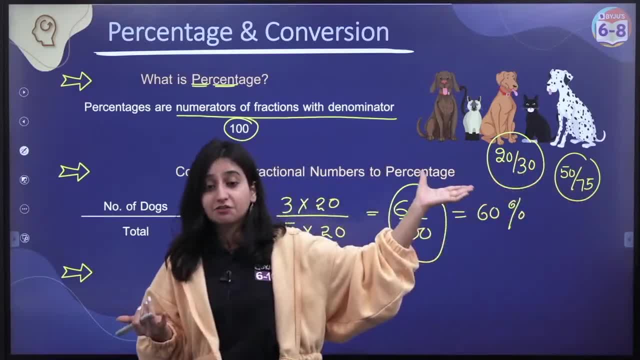 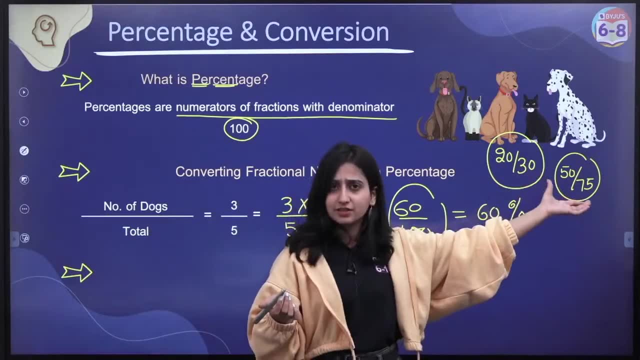 We need a comparison in them. So what will be the most effective method? We have to find the percentage. We will see the percentage that, how much it performed, and how much it performed on the basis of 100.. Yes, So here, quickly convert. 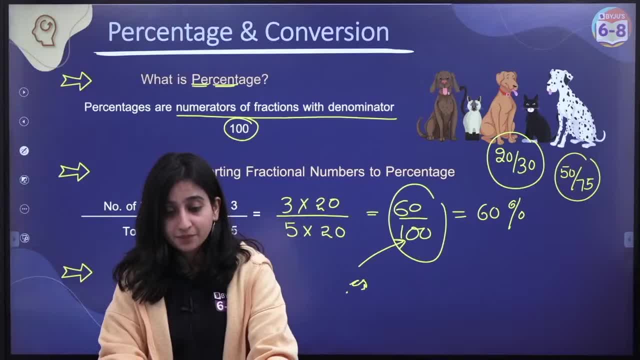 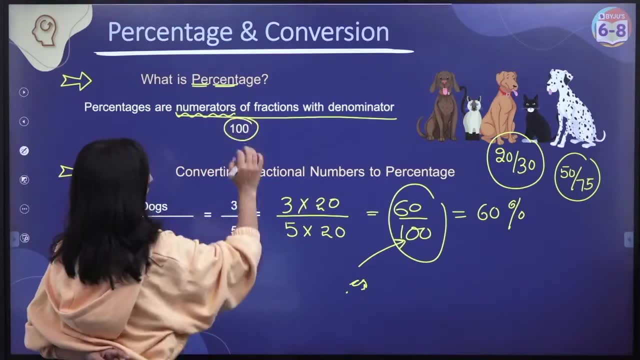 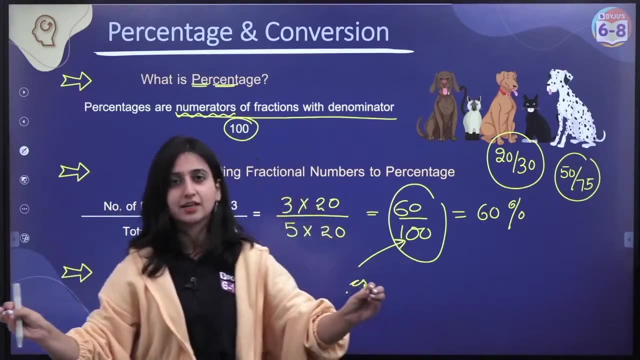 these two fractions into percentage quickly. So I will tell you a simple way. You have come to know that what is percentage? Basically, it is called numerators. Numerators of such fractions are called percentage whose denominator is 100. It is given as a very basic definition. 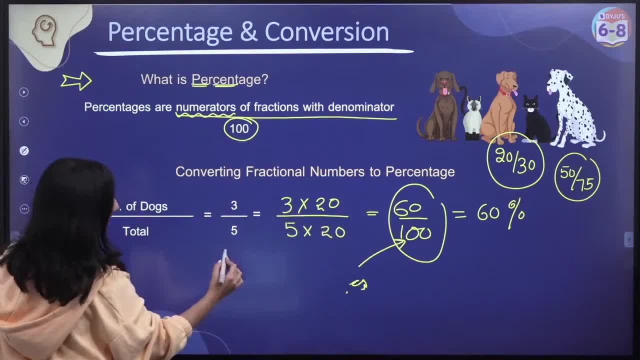 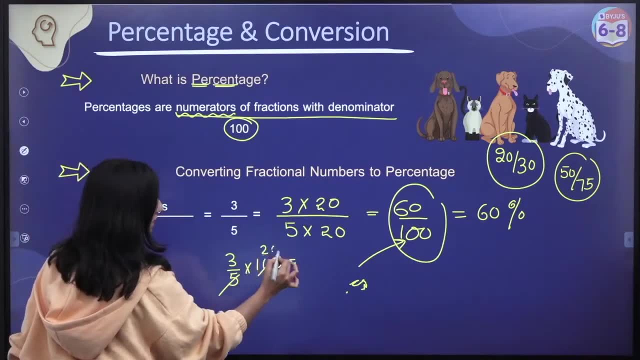 Right. So if I have to find the percentage, what could I do directly? If I multiply 3 upon 5 directly with 100, then still I will get the same answer. I will still get 60%. So whenever you want to convert a fraction, 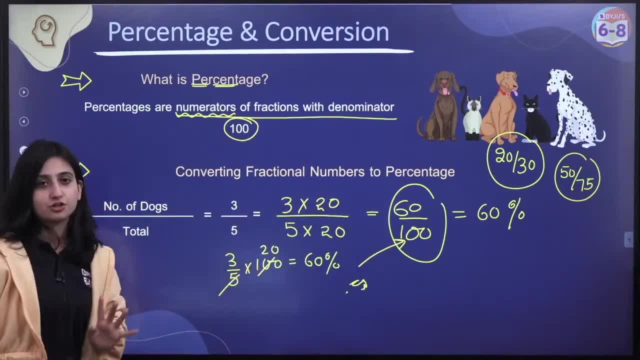 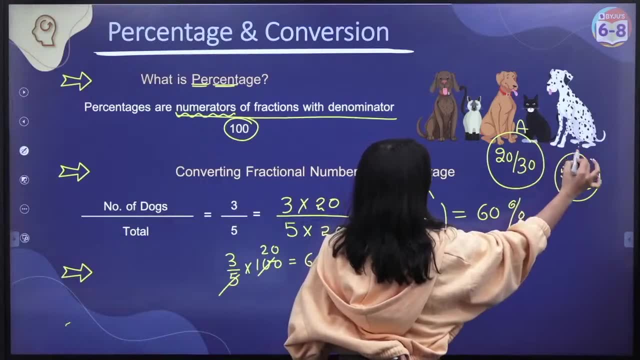 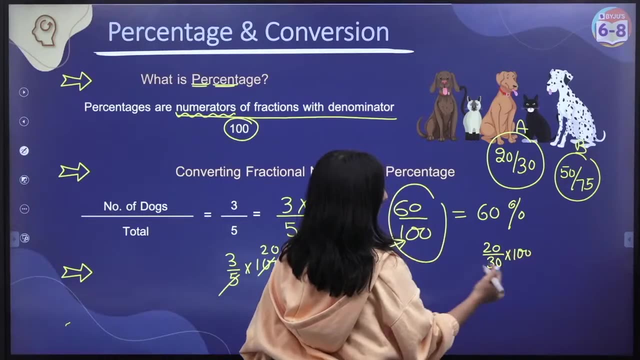 into percentage. just multiply that fraction by 100.. You just have to multiply that fraction by 100.. Now we want to compare the marks of these two students. So what we will do? We will convert these fractions. into what Percentage? Come on, Multiply it by 100.. 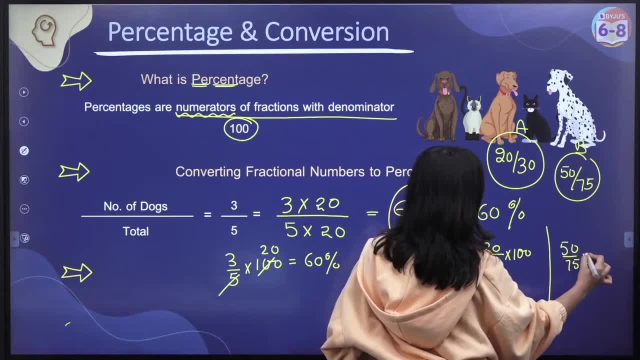 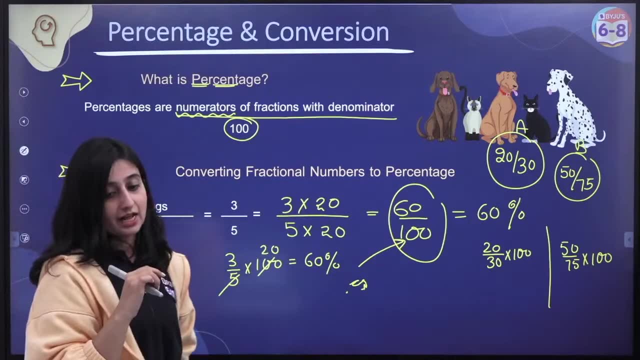 Multiply this also by 100.. 50 upon 75 into 100.. Now tell me what is the answer. Someone quickly tell me what is the answer. Yes, everyone Whose percentage is more, Who has performed better, Has student A. 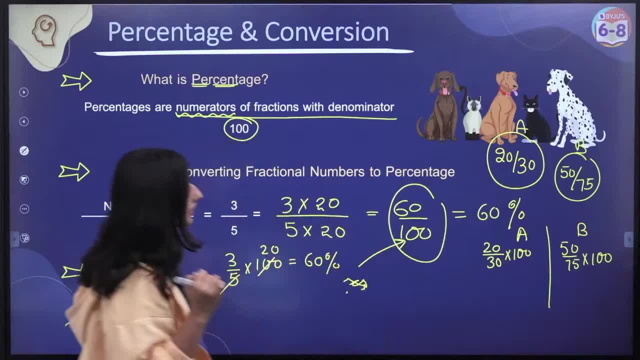 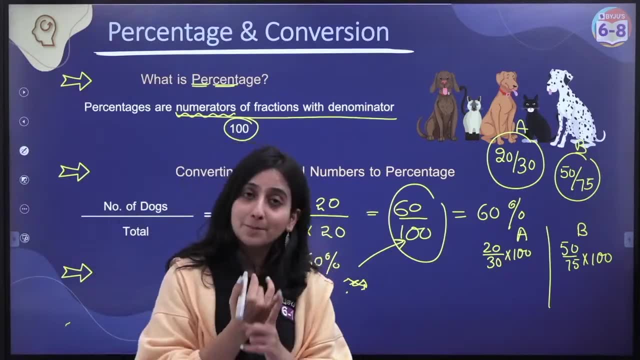 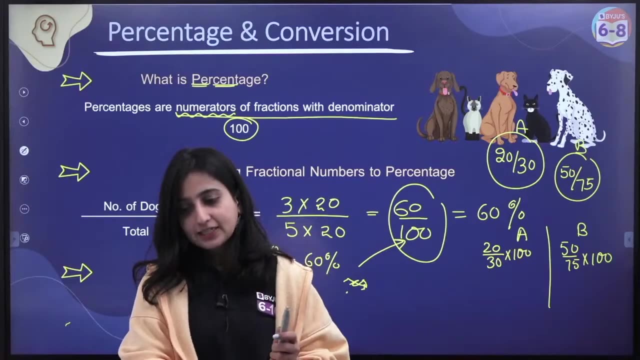 performed better or student B performed better? Quickly calculate and tell me: Okay, So that's why we are studying percentages, because this is the best way to compare. Okay, Yes, students, Is it clear to everybody What is percentage Percentage, How to. 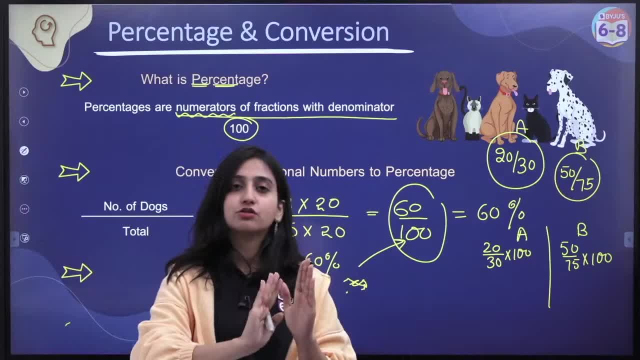 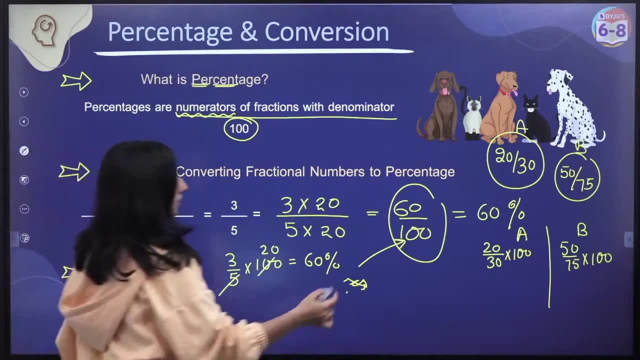 convert a fraction into percentage. Everyone understood. So just multiply the fraction by 100.. Now, why did I multiply it by 100?? You can see the reason here: Because when you multiply by 100, see here What did you get. You can. 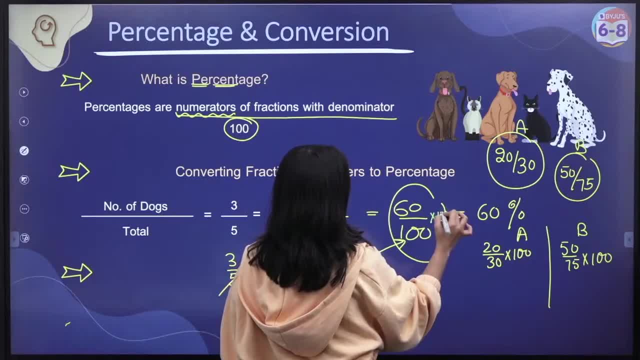 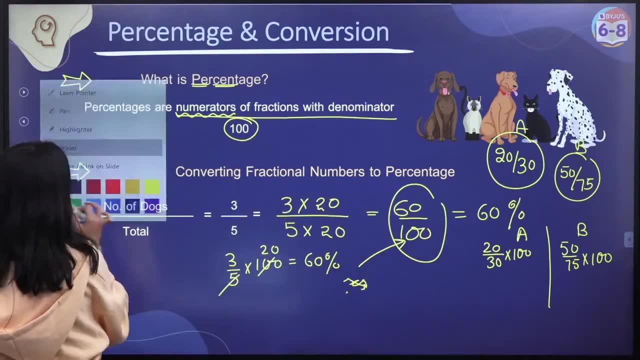 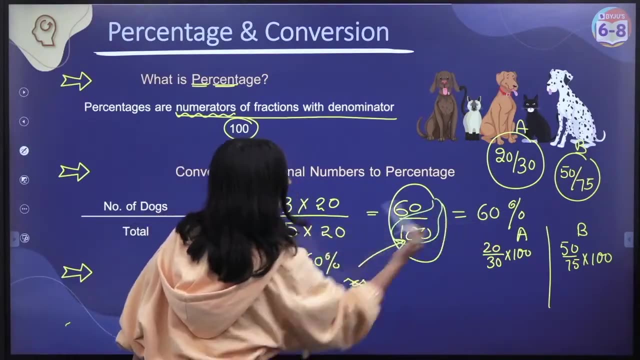 multiply it by 100.. So what will you get here? Percentage, One second. This by 100.. This by 100.. 1 by 100. This means Percentage. So 60 into 1 by 100 means Percentage, Is it clear? 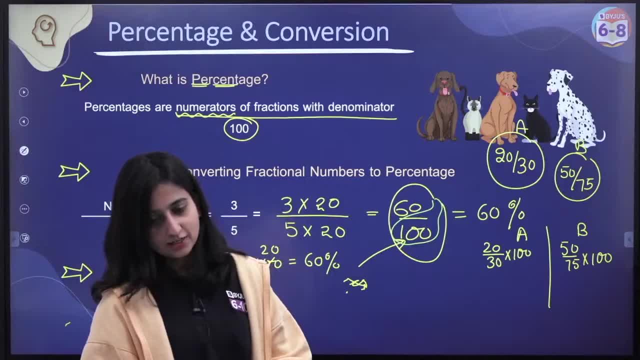 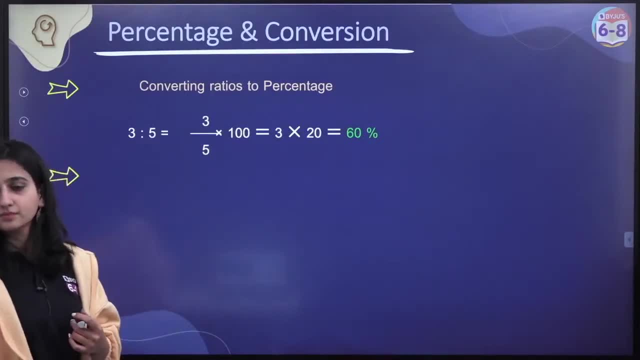 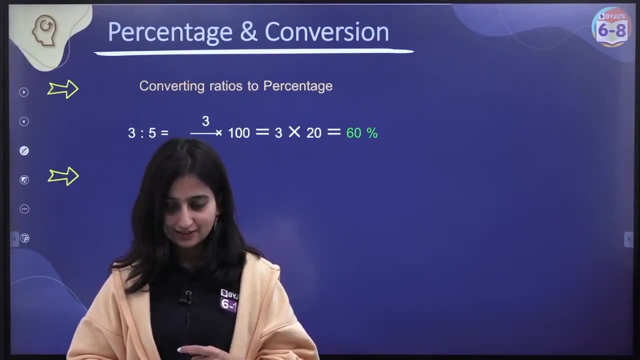 Did everyone understand? Yes, They both Okay. both are same. Okay, see now comparison. Yeah, Okay, Now am I audible Everyone, am I audible now? Yes, Okay, Very good, Mastan, Now let's move ahead. 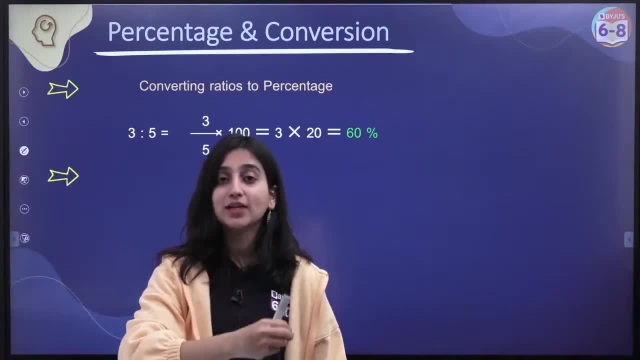 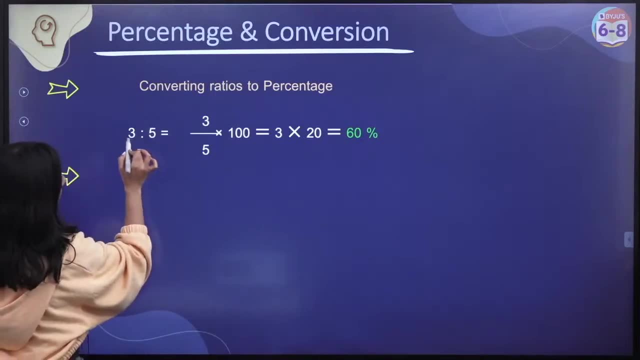 We have learnt to convert fraction into percentage. Now let's try to convert ratio into percentage. Now we can write ratio as a fraction. How to write ratio? 3 is to 5.. Now how will I convert ratio into fraction 3 upon 5.. 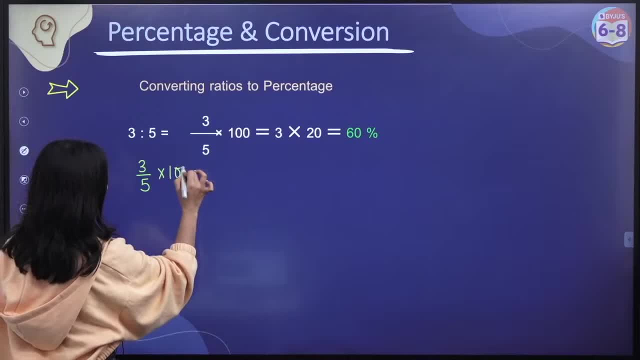 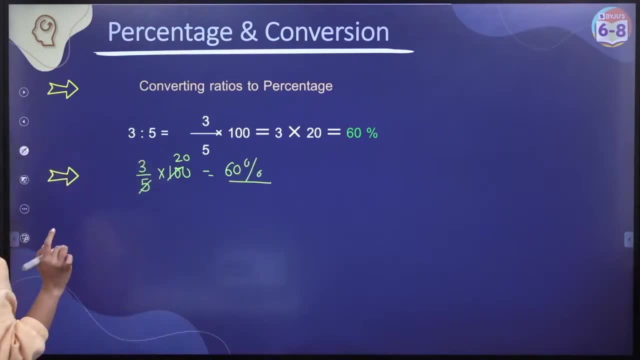 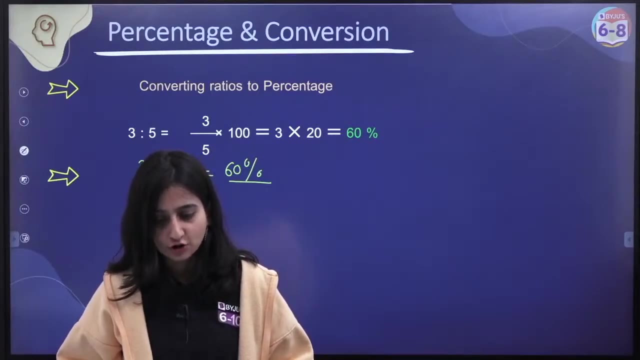 Just like you changed ratio into percentage by multiplying by 100,, similarly you had to do the same here. By multiplying by 100, your percentage will change. Same method is there? Is it clear? everybody? Did everyone understand, Yes or no? 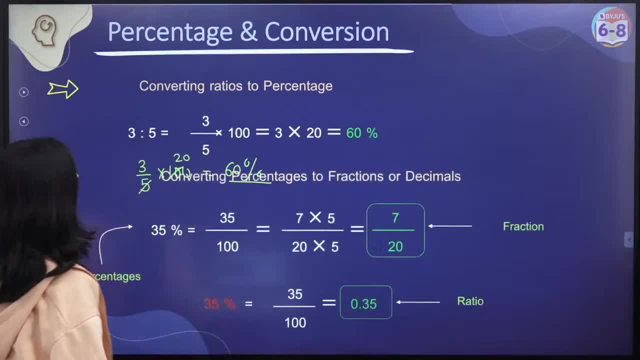 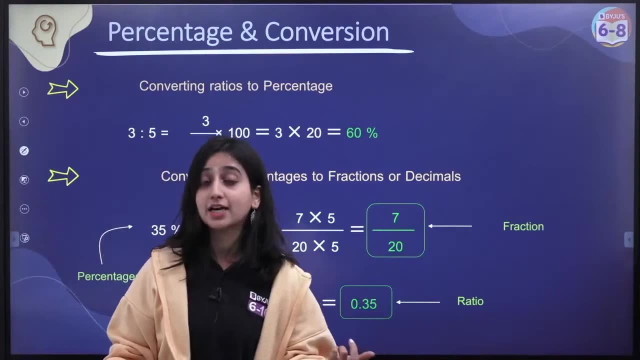 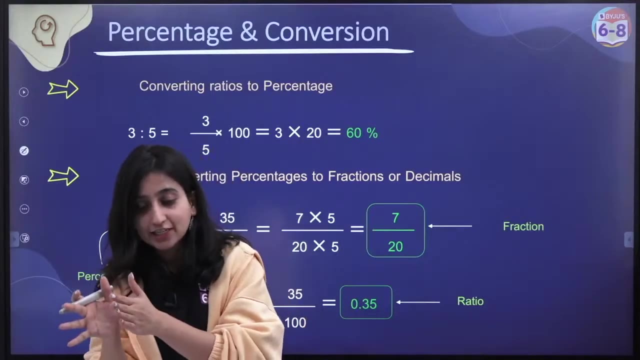 Is it clear? Okay, so now we have learnt how to convert a percentage into percentage, ratio and fraction. Now, if you are asked in reverse, if you are asked to convert percentage into fraction, then what will you do? How will you convert percentage? 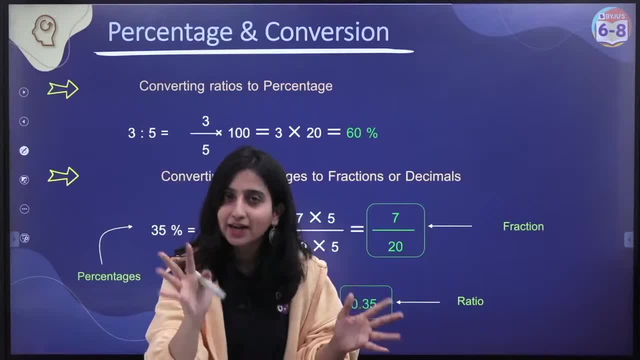 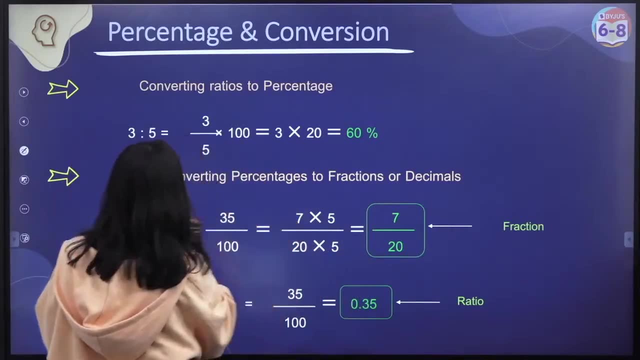 into fraction By dividing by 100.. Because what does percent sign mean? 1 by 100.. Okay, what does its sign mean? 1 by 100.. So if I want to change 35% into fraction, then what does this percent sign mean? 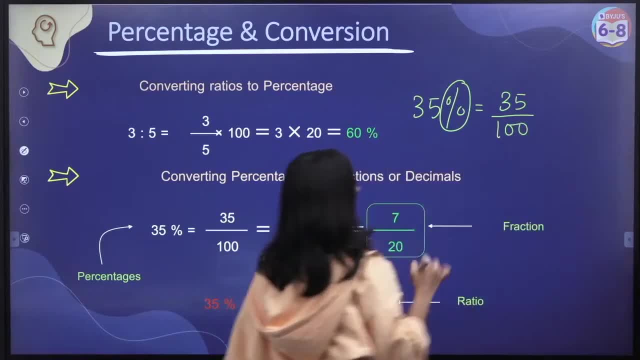 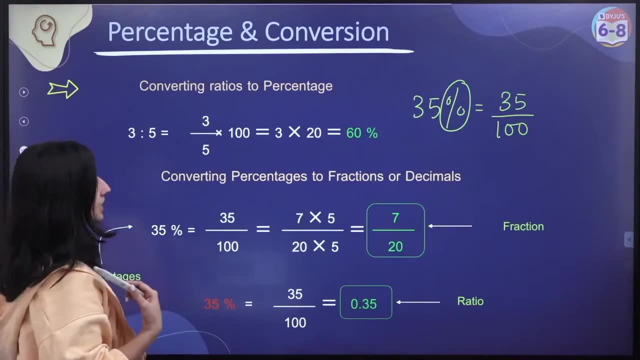 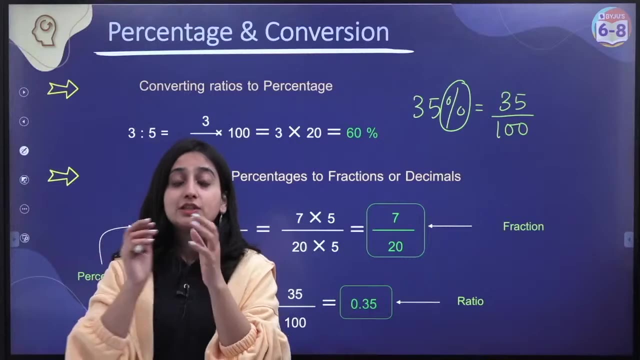 1 by 100.. So I will divide this 35 with 100.. So I will get. I will get a fraction. I will get a fraction. Is it clear? Did everyone understand? Simplify this? Okay, No problem, those who have joined late. 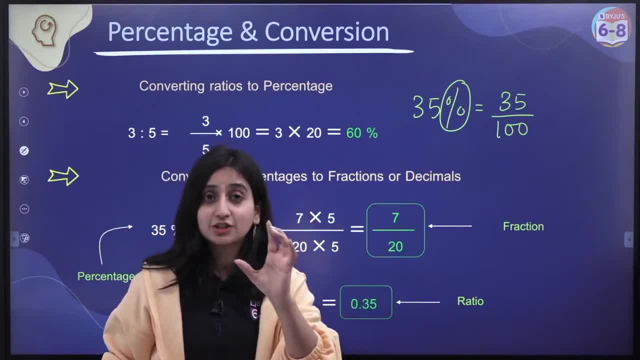 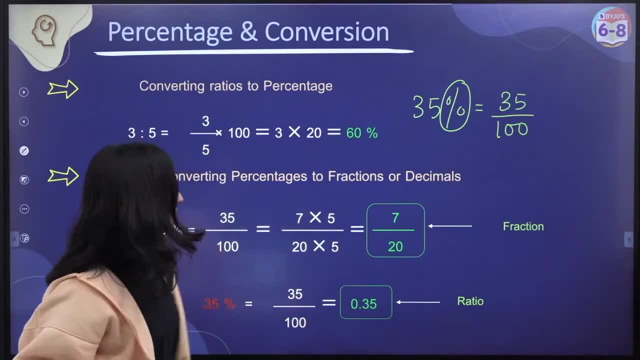 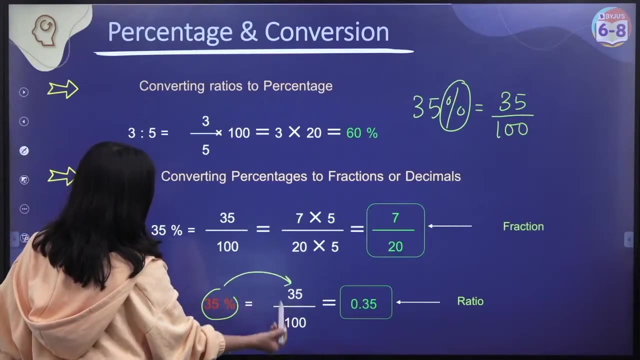 attend the class from now and the starting portion that you missed, you can see that after the session. whatever you missed, Okay. So similarly, if you have see this, 7 upon 20 is coming again. it is 35%. What have we changed? 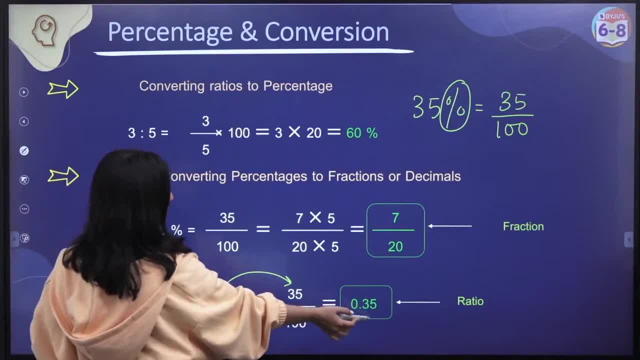 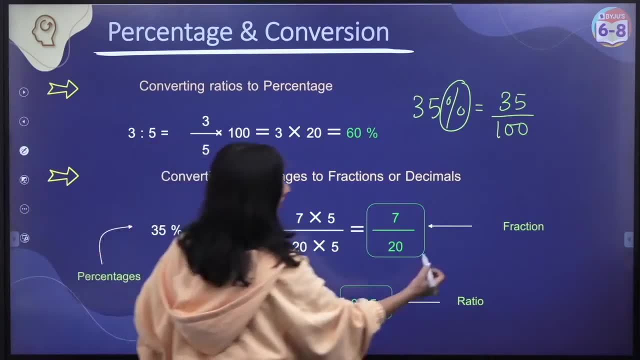 We have changed into fraction. So what have we got? It has become 0.35.. See, in fraction we will write only this much: Simplify this. When we have simplified this, 7 upon 20 has come, If we want to convert into ratio. 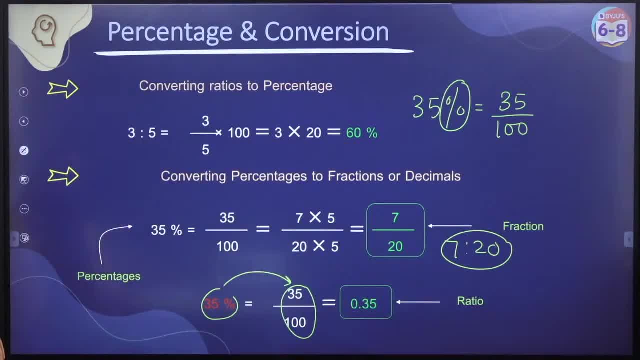 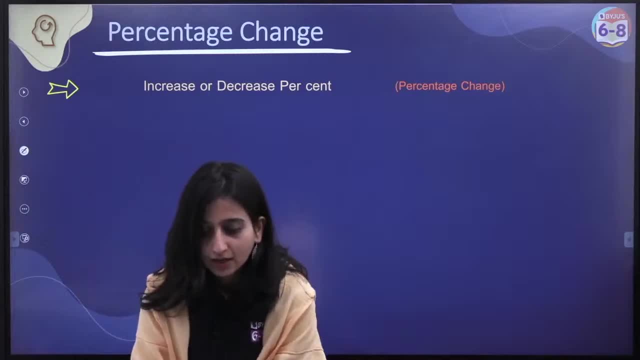 we can write it like this: Okay, Writing in symbol of ratio and writing in sign is very easy. Next thing that we have to study in this chapter, Hi Vaishnavi. So till here. is it clear to everybody what is ratio, What is fraction. 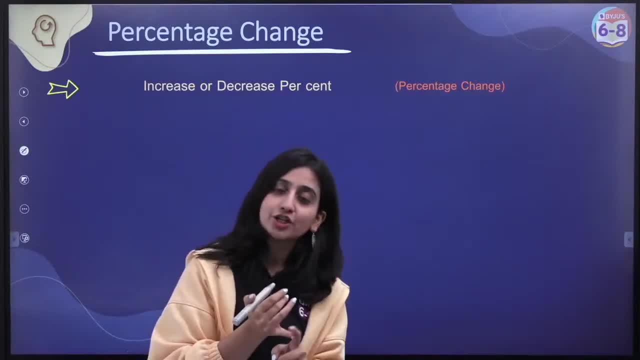 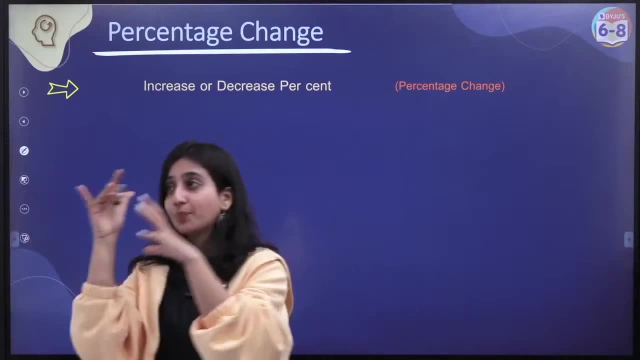 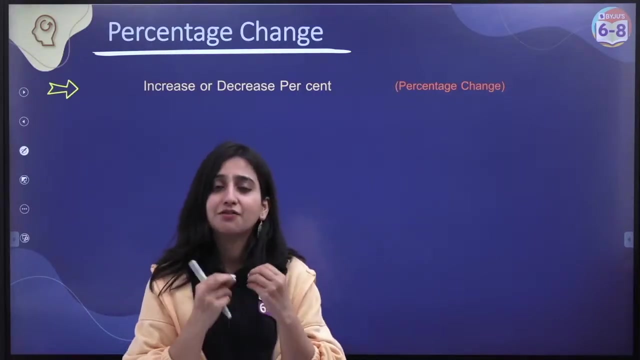 What is percentage? How do we convert ratio into percentage? How do we convert a fraction into percentage? How do we convert a percentage into ratio or percentage into fraction? All of these things are clear to you. I think these all concepts that we studied, these are very 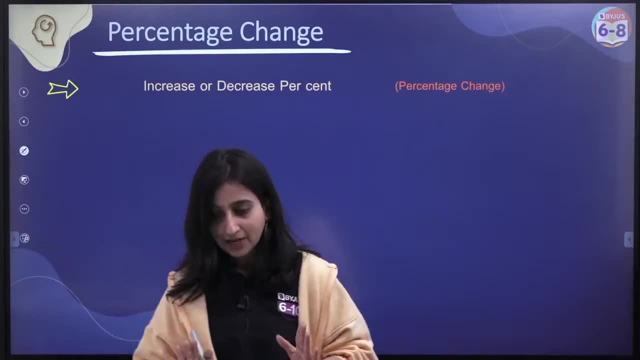 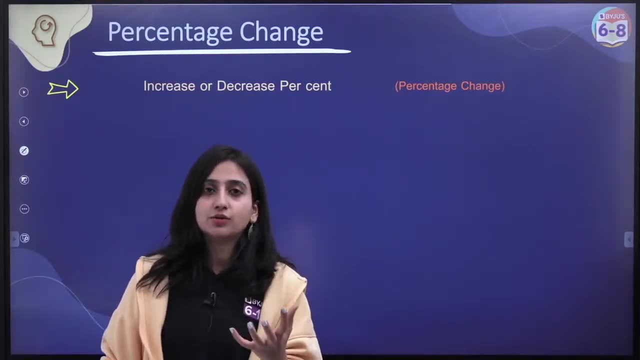 basic and very easy. You will do it easily. Okay, Now let's talk about percentage change. There are many questions on this. Okay, What is percentage change? How much change has happened in percentage Now? it is possible that, suppose? 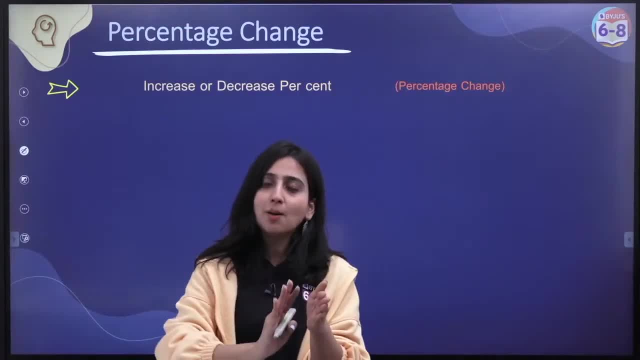 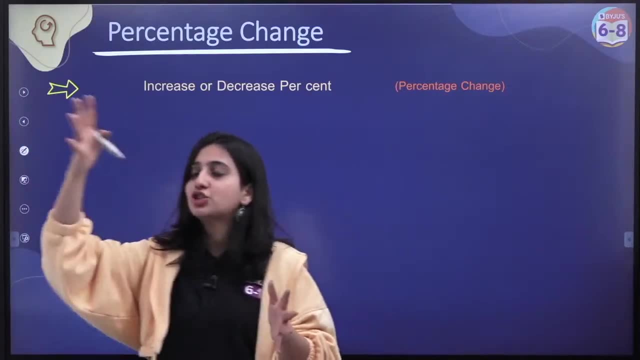 the population of our city was like this and let me say after 5 years that population increased by 20%. Okay, So we have change in population. So how do we find out increase or decrease? We are going to learn that. 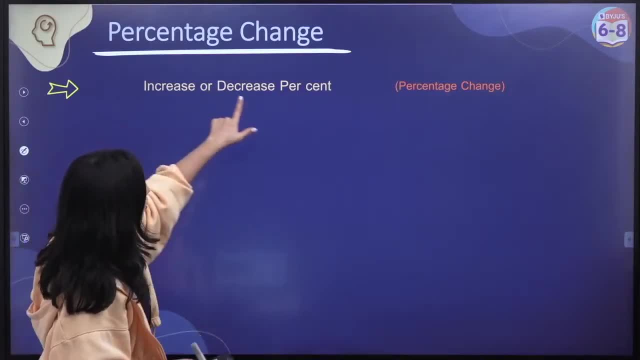 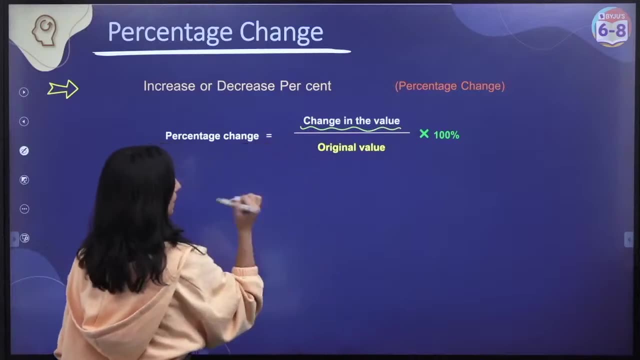 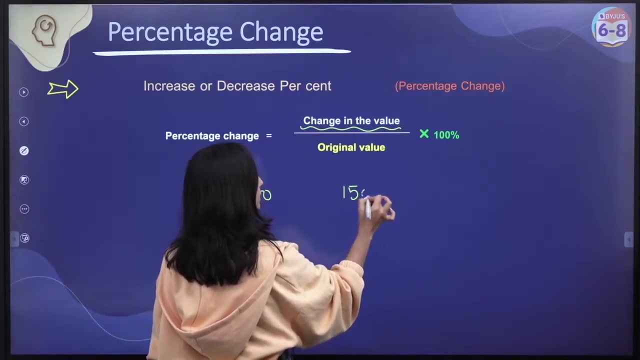 here. Okay, Yes, So how do we find out? increase or decrease percentage? How much increase has happened? How much change has happened in value? Suppose, today I have 100 students in class and yesterday I have 150 students. I asked you: what is the percentage? 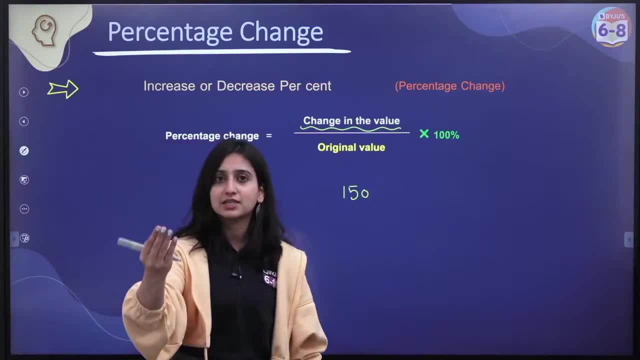 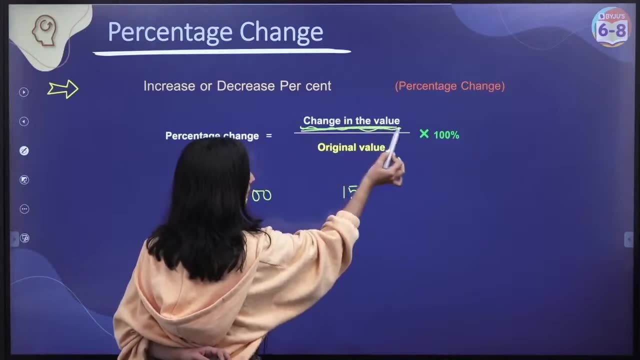 increase. How much increase has happened in students? Tell me in percentage. Okay, So what will I say Now? first of all, you write that how much change has happened in both values? So how much change has happened in both values? 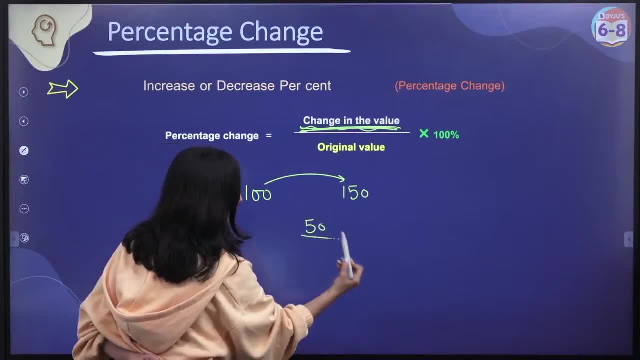 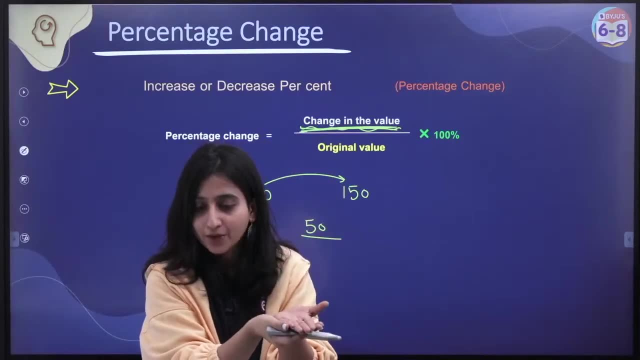 How much difference has happened in both values? Difference of 50. Divide by what was the original value. So always change is seen by comparing with original value. Always change is seen in respect of original value. Okay, So what was the original value? 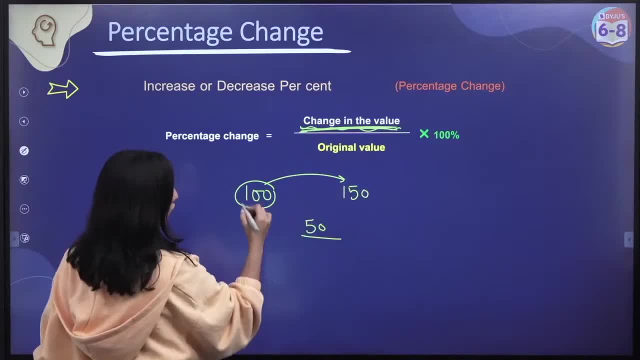 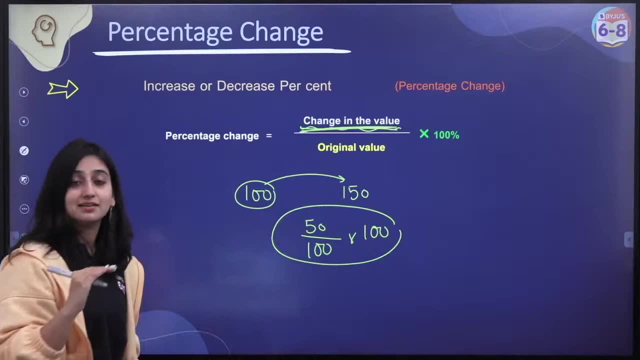 In starting there were 100 students. After some time 150 happened, So original value was 100.. Multiply by 100.. This is how you calculate the percentage change. That is, percentage is increasing because 100 to 150 happened. 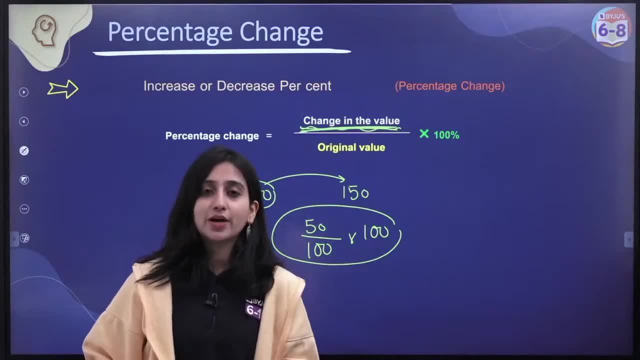 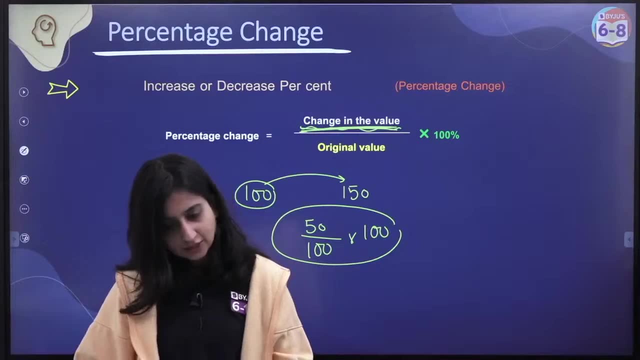 So decrease can also happen, Okay. So questions like this can be asked to you: Is it clear? Yes, kid, Is it clear? Okay, Now let's move ahead. Let's move on to the next concept. 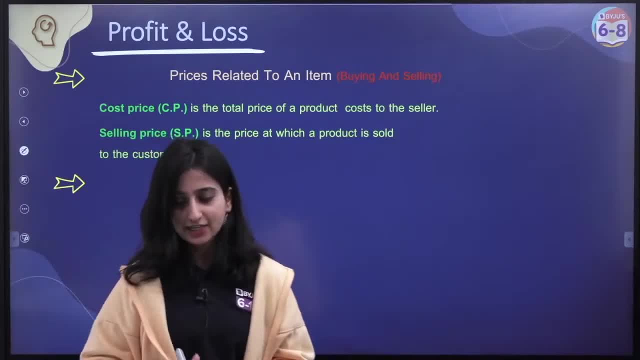 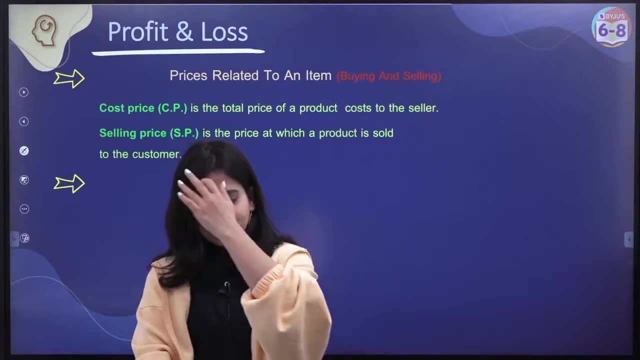 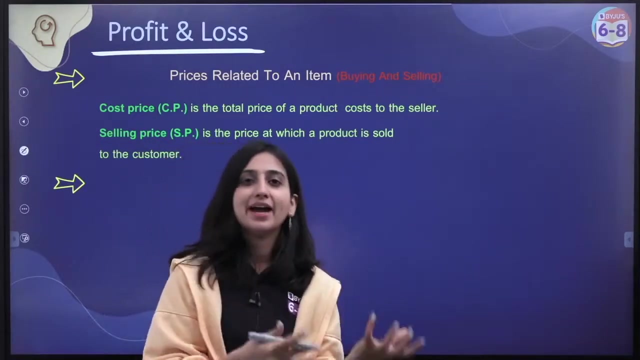 Profit and loss. Okay, how many children are scared of the question of profit and loss? How many children are scared of the question of profit and loss? Tell me quickly: Yes, To understand profit and loss, we need to understand buying and selling. How buying and 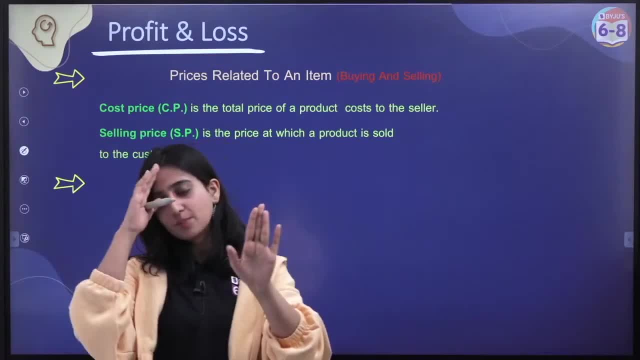 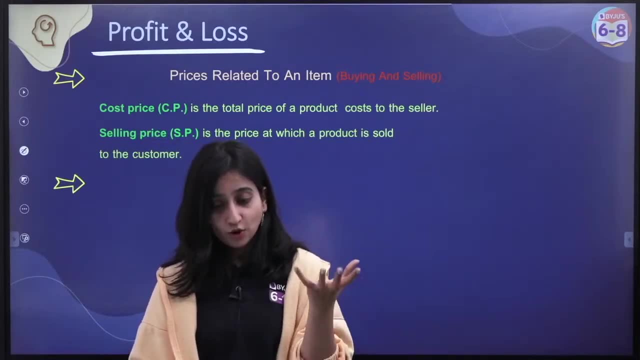 selling happens Right. So we have two terms, two important terms which you have to keep in mind: One is cost price and one is selling price Right. What is a cost price? What is a cost price, Nidhi? 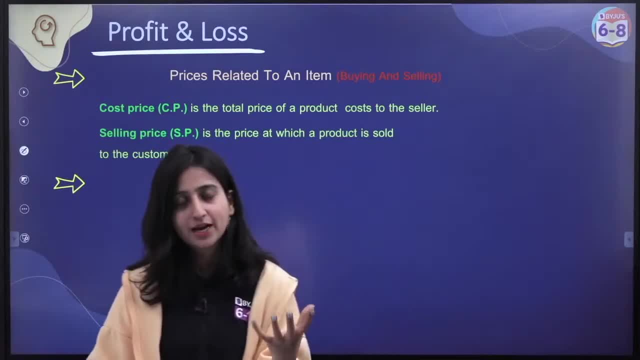 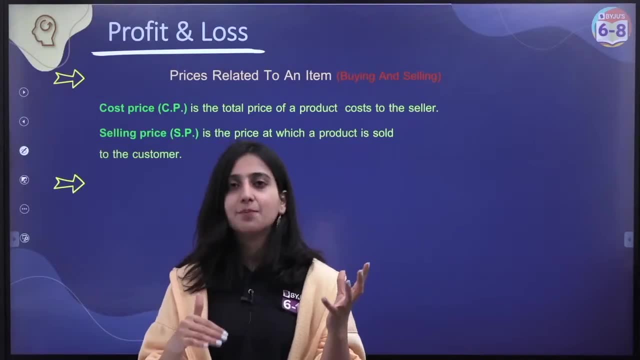 I will ask you questions. You will understand percentage increase and decrease. We will be solving the questions after revising all the concepts. Okay, We will solve it. Okay, Take the example of decrease. Suppose there are 200 students in the class. 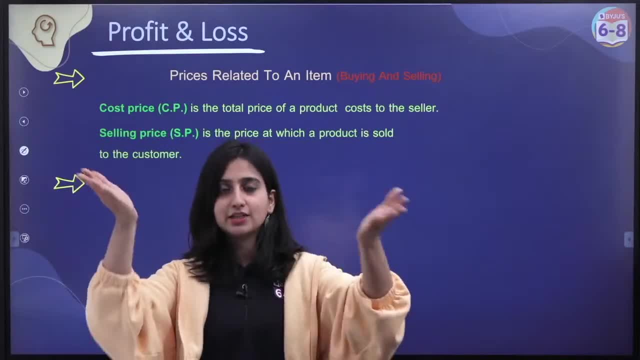 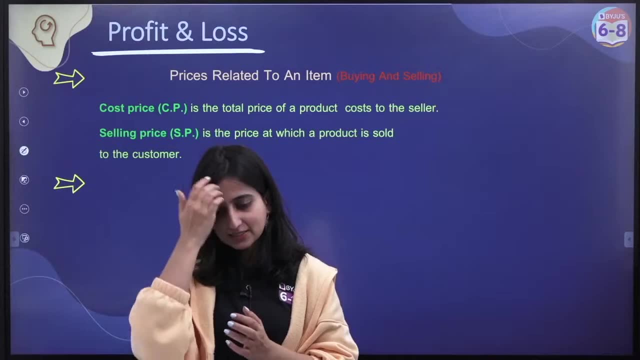 After that they have decreased to 100. So calculate the percentage decrease, That is, change upon original value into 100.. Okay, Class 6 will also come live. Don't worry about it. You will get the schedule on the channel only. 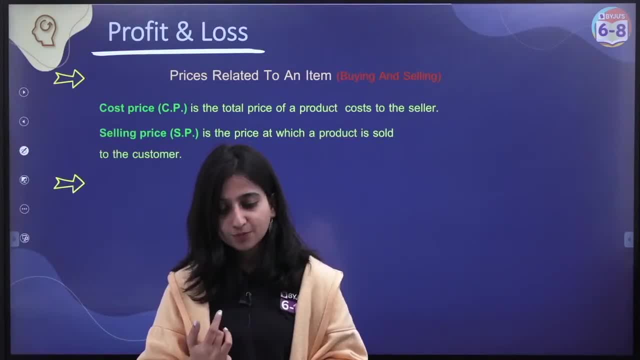 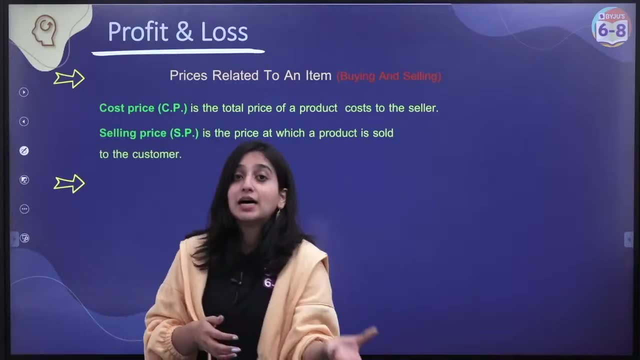 Yes. What is cost price? What is a cost price? I have asked you a question: What is cost price? In what amount means? in what amount did you buy something Right? Suppose? imagine that you are a shopkeeper. 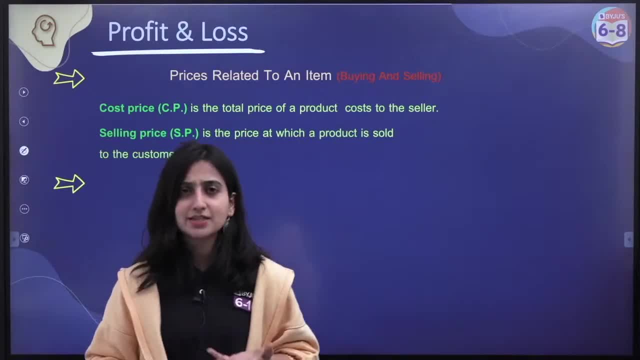 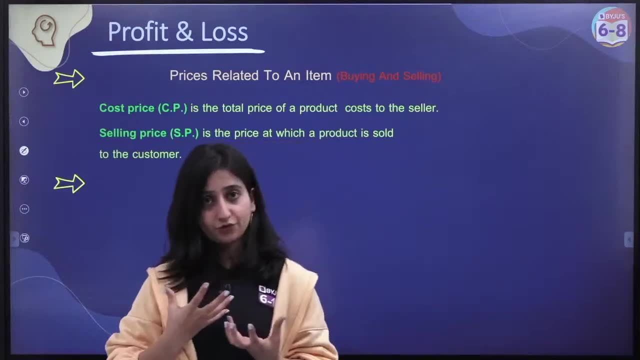 You bought things for your shop. You want to do business, You have to buy things from a vendor. So in what amount you are buying the things from that vendor? what is that? It is called cost price. In what amount did I buy? 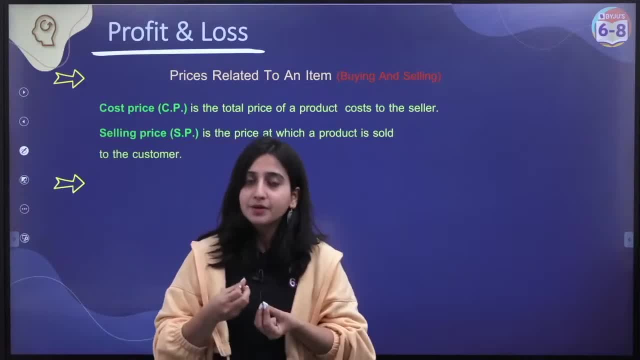 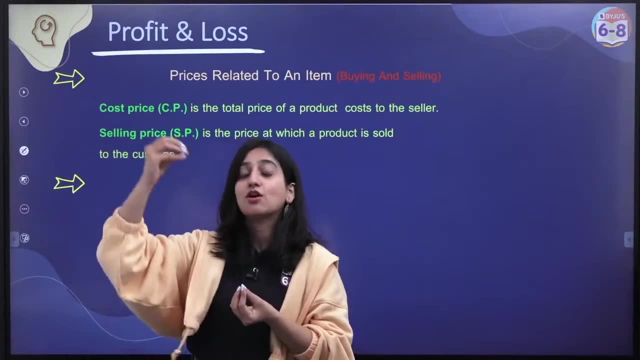 Okay, In what amount did I buy? Okay, Now, in what amount am I selling that particular thing? In what amount am I selling that thing? That is called a selling price. What is it called Selling price? Now, it is a simple thing, Logics. 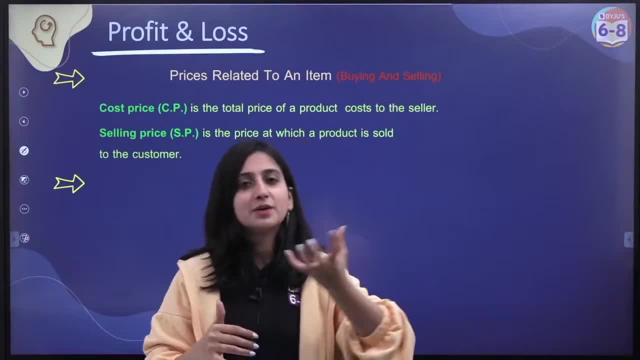 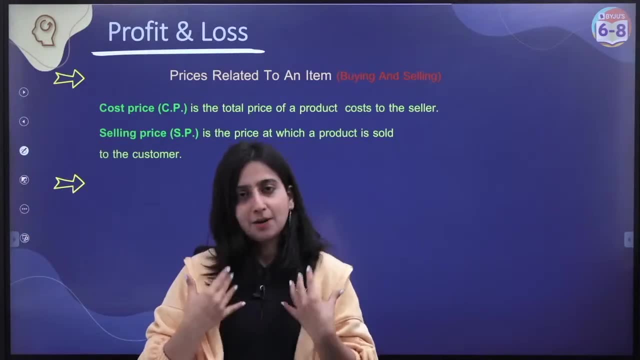 have to be applied. Look, suppose I bought a chocolate for 5 rupees and I am selling that chocolate for 10 rupees. So am I in profit? Am I in profit or am I in loss? Tell me, Am I in profit or am I in loss? 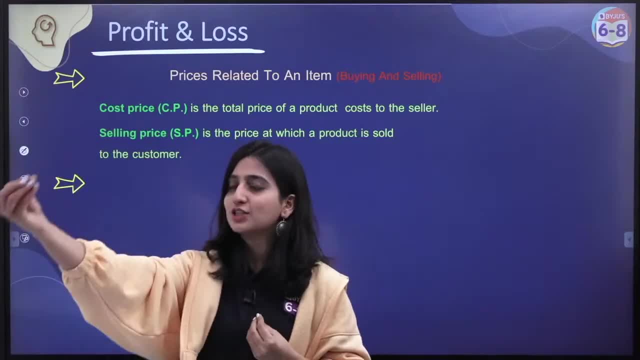 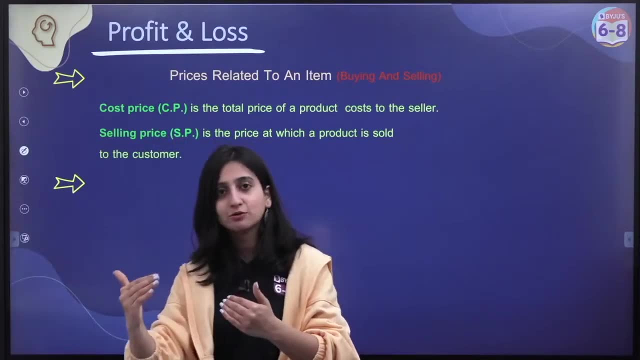 I bought a chocolate for 5 rupees from a vendor and I sold it to someone else for 10 rupees. Okay, So I am making a profit here. Why? Because the selling price is high, So I got the margin. I earned that much. 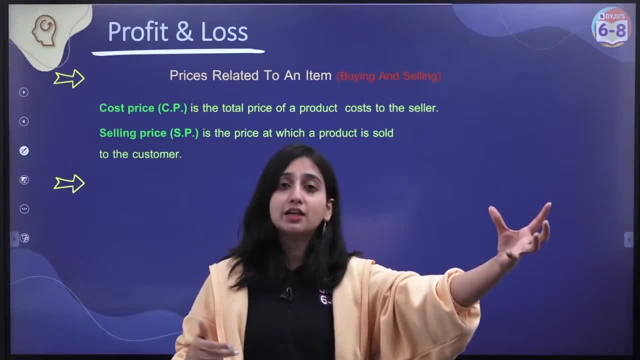 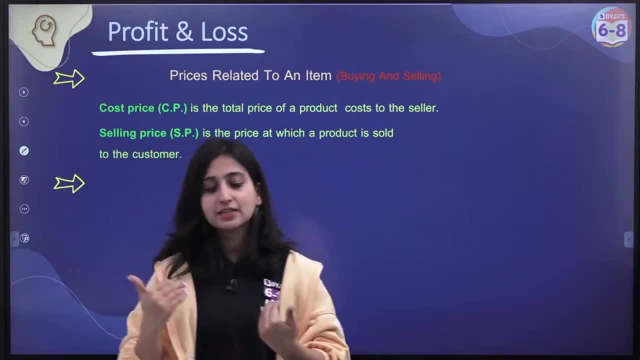 That is the profit. Suppose: if I had bought a chocolate for 5 rupees and I had sold it for 2 rupees, then I would have incurred a loss. Right, This is how profit and loss works. Right, This is how it works. 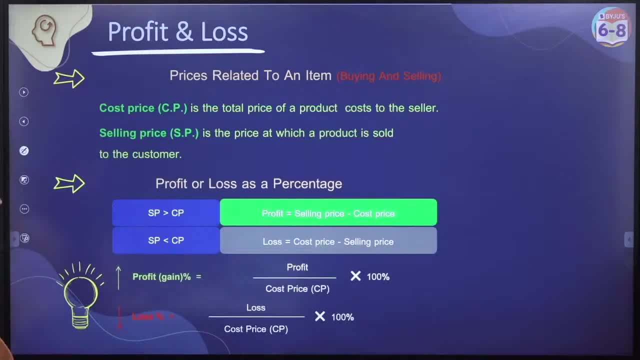 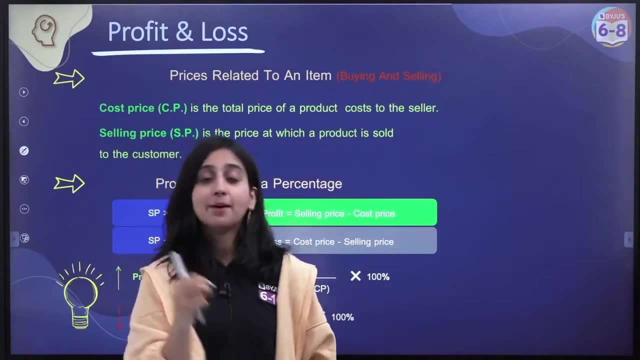 Now, what would you like to be asked? Now, what would you like to be asked? Take out the percentage, Suppose: how much percent have you gained, How much profit have you earned? How much loss have you endured? Okay, So now we will calculate those things. 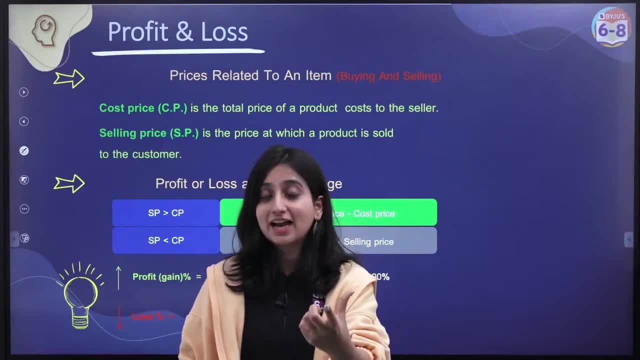 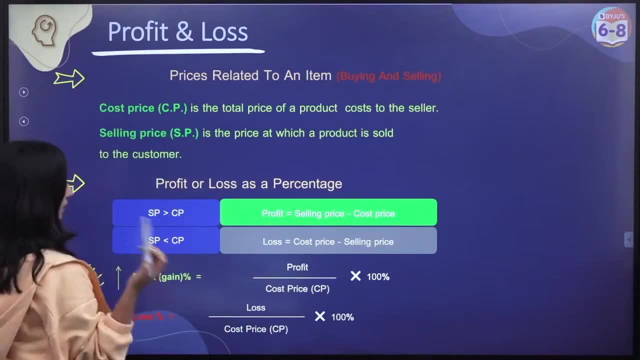 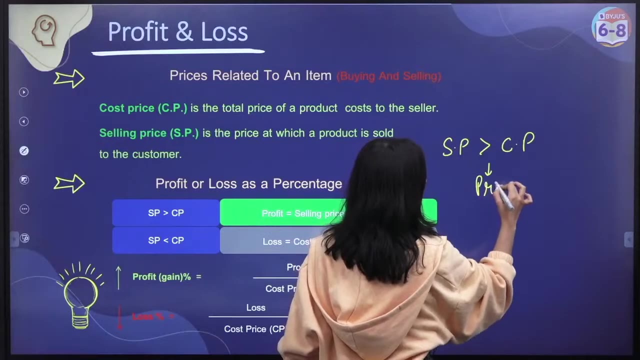 Now the same thing comes: How to calculate profit percent? How much difference is there? Obviously, look how much difference is there between selling price and cost price. Look, if our selling price is greater than cost price, then our profit is definitely. 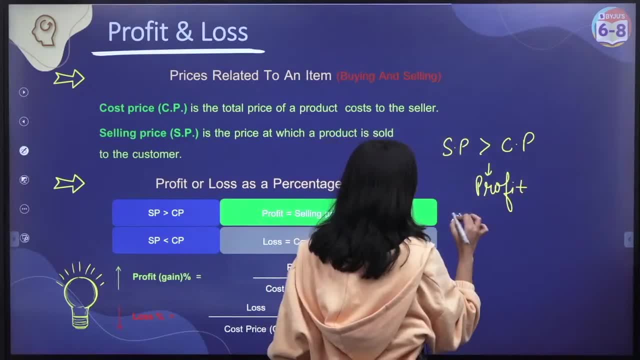 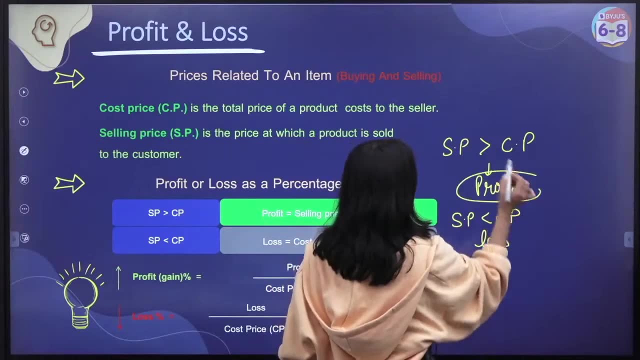 going to happen, Right, Because I have sold more. If my selling price is less than cost price, then I will incur loss. Okay, So when profit is happening, then see how much profit is happening. How will you know how much profit is happening? 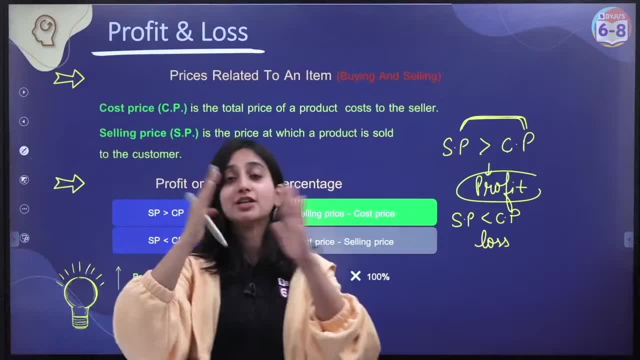 If I bought chocolate for 10 rupees, I am selling that chocolate for 10 rupees, So the difference is 5.. So if I want to calculate the profit percentage, then here also the concept of change is being applied. 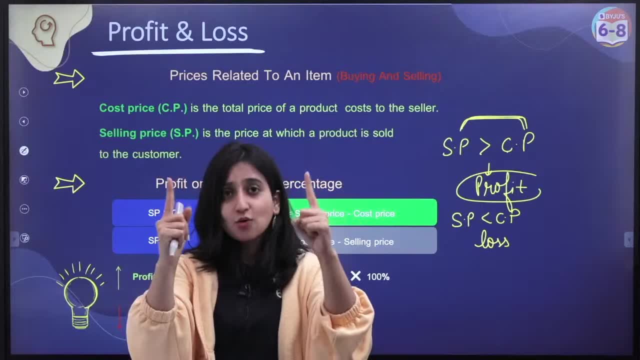 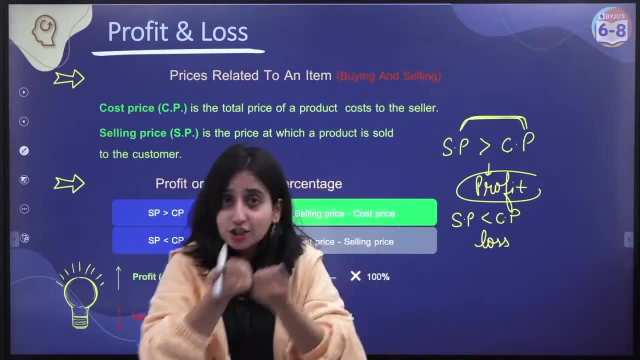 How much is the change Right? How much is the change? What is the difference Divide by the original amount? In what amount did I buy the thing? So we will keep the cost price in the denominator, Multiply by 100.. 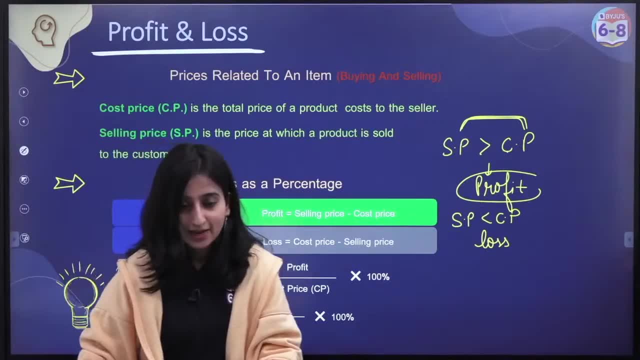 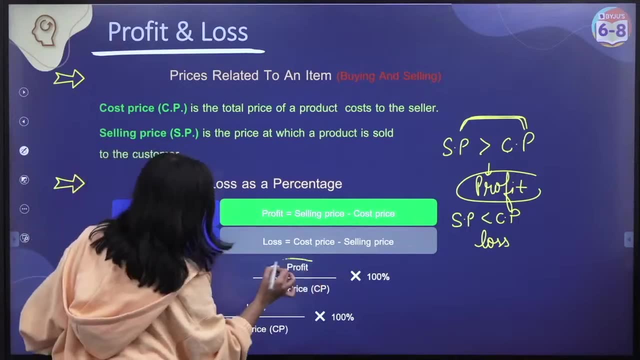 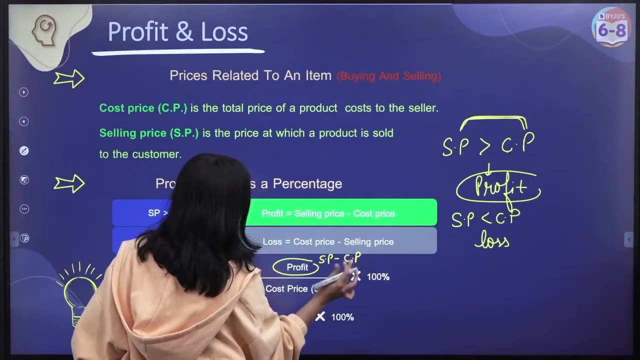 This is how you calculate the profit percentage. Is it clear? Is it clear everyone? So if you want to calculate the profit or gain percentage, then you will find the profit. How do you calculate the profit? Profit is basically selling price minus cost price. 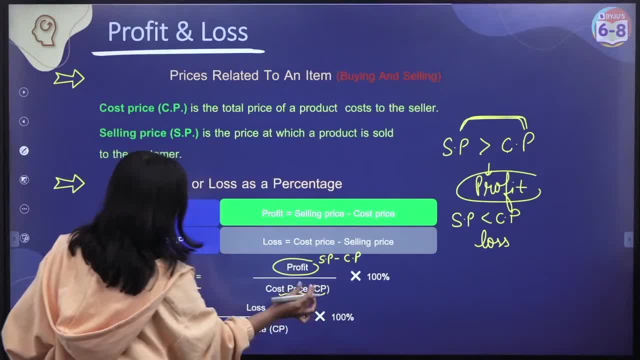 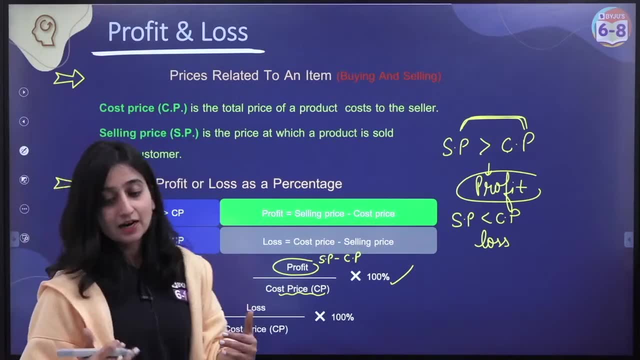 Check the margin here. Divide by cost price: In what amount did we buy the thing? Multiply by 100. That will be your profit percentage. Similarly, what will happen for loss? Now see how much loss has happened for loss. When will the loss happen? 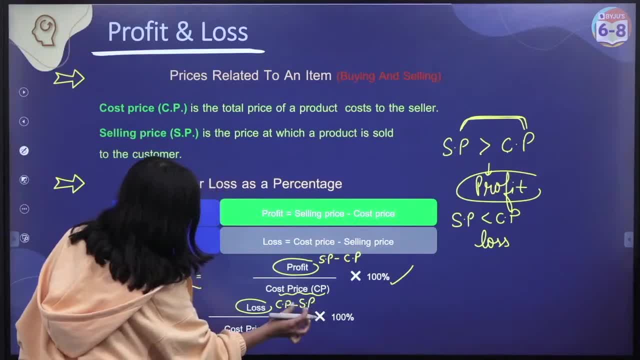 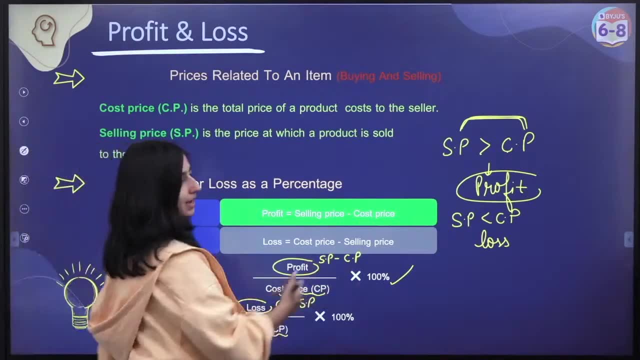 When our selling price is more than the cost price minus the selling price. See how much difference has come In. what amount did I buy the thing? It will always remain in the denominator. We will always see in the respect of cost price. 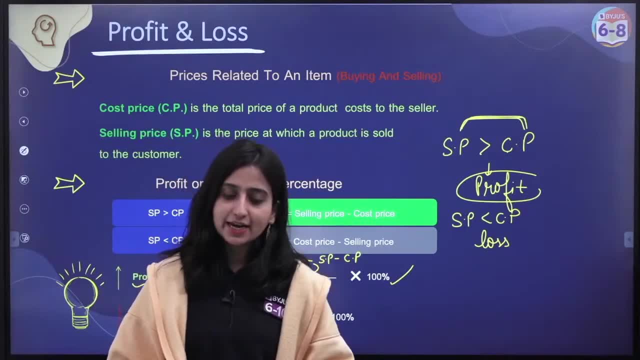 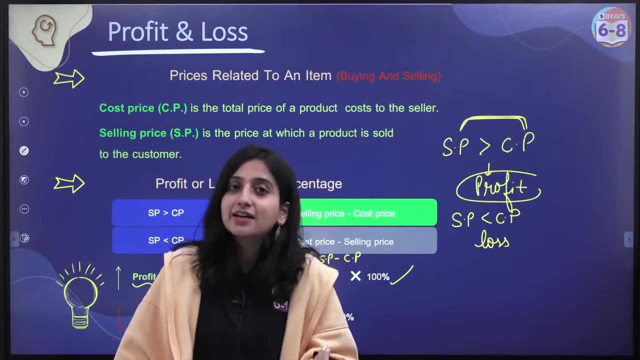 Multiply by 100.. Is it clear? Everyone understood: Yes, Srishti, Profit of 5 rupees has happened. But what is the profit percentage? If you want to calculate the percentage, then you have to divide 5 by the cost price. 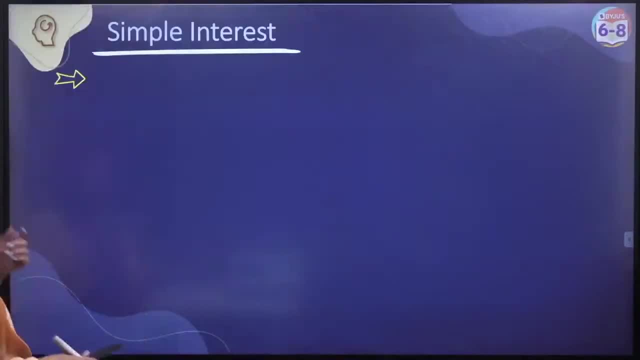 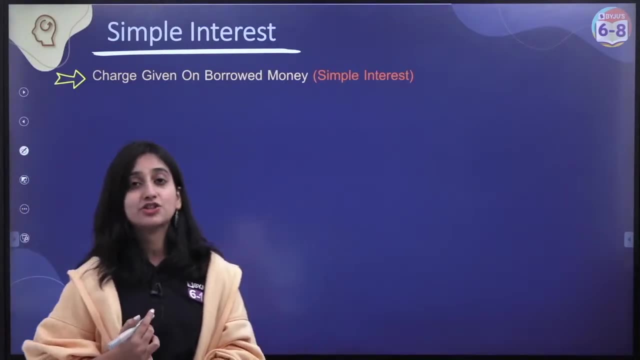 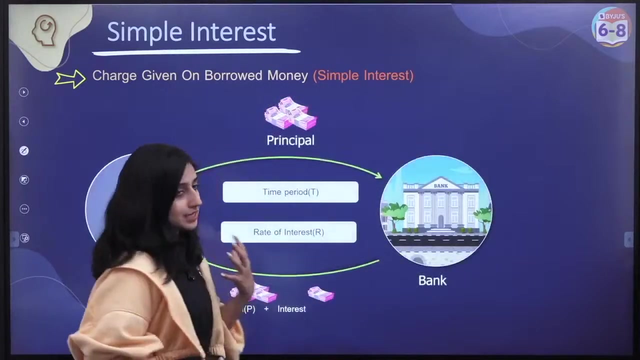 into 100.. Okay, After that we will do NTB. This was profit and loss, And the next concept that you study in this chapter is simple interest. Now, what is this simple interest? See, whenever we either deposit the amount in the bank. 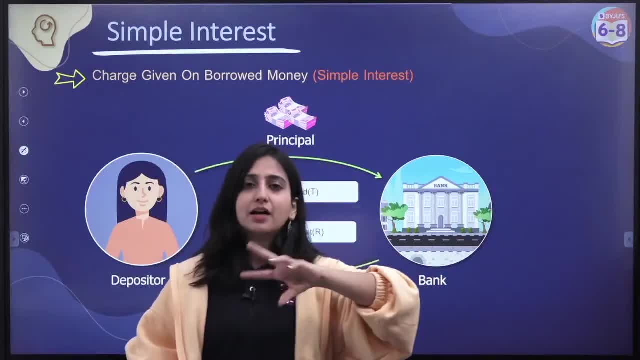 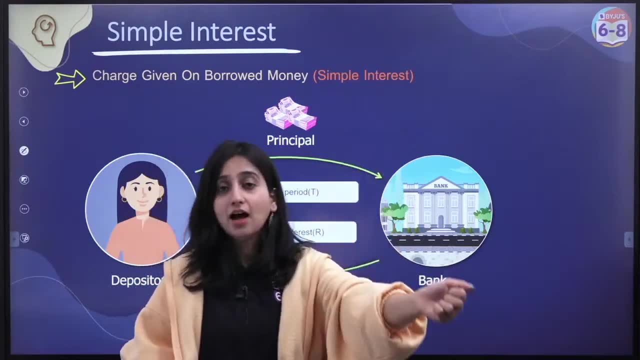 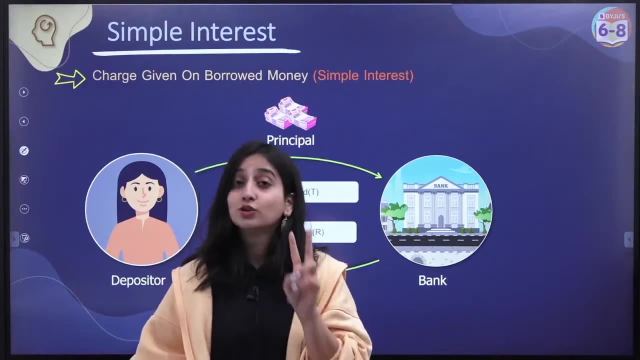 or borrow the amount. We do two things. Either we deposit our money in the bank or we take money from the bank. We borrow, We take loan Right. There are two types of cases. We have two types of cases. Either we are borrowing, 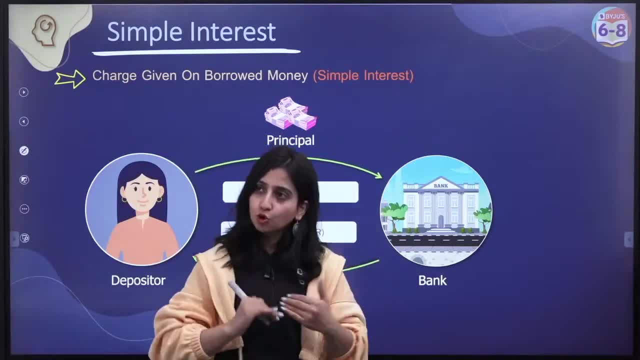 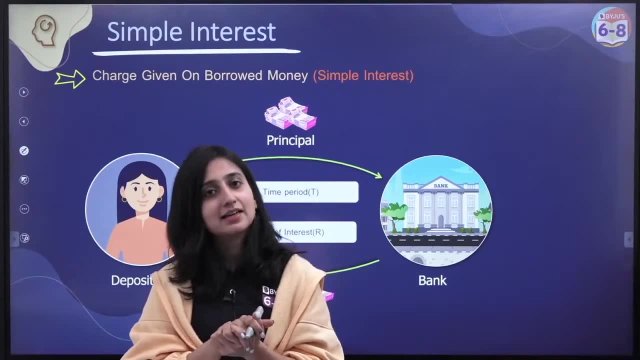 the money from the bank or we are depositing our money. So, whatever your case is, interest is applied on it. Right, What is applied on it, Interest is applied. It is not like you told the bank that I want to take 50,000 from you, Okay. 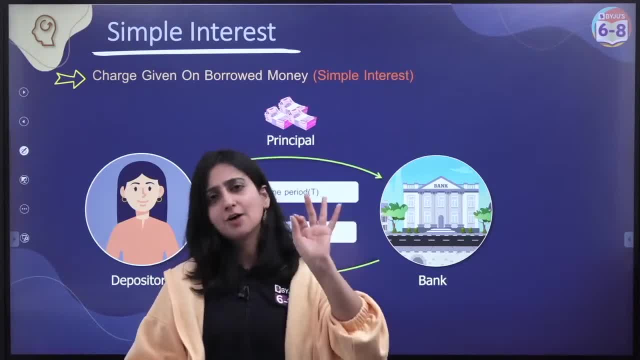 And I will return that money to you in 10 years. And the bank will say, yes, after 10 years, return me 50,000.. So what was the benefit of the bank in this? What was the benefit of giving me money? 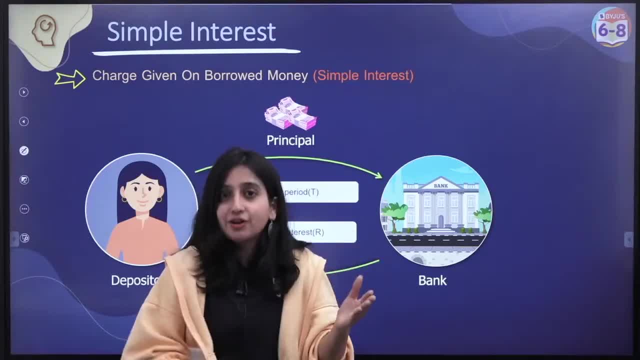 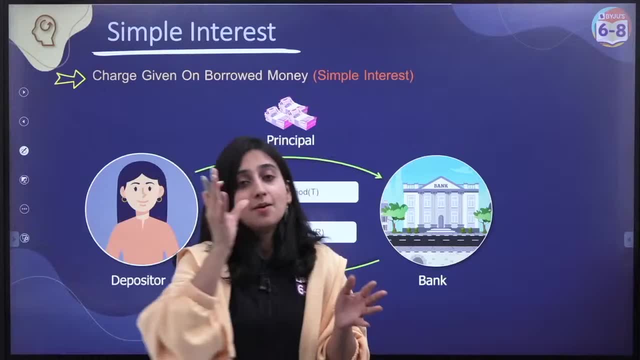 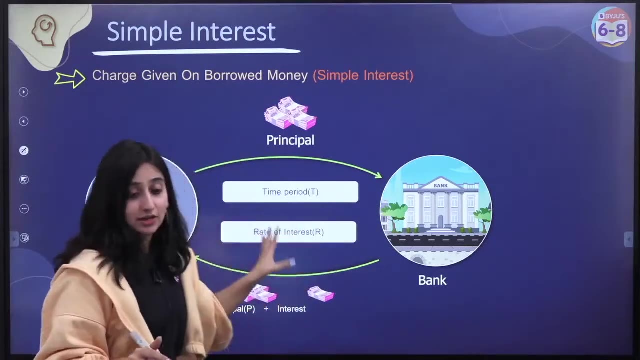 There is no gain of that. So every year, the bank applies interest on you. Okay, It takes a little extra amount from you. It keeps on accumulating, It keeps on adding on, Okay. So what is simple interest? How do we calculate simple interest? 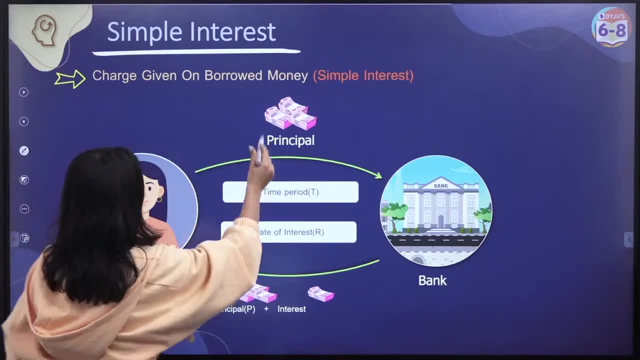 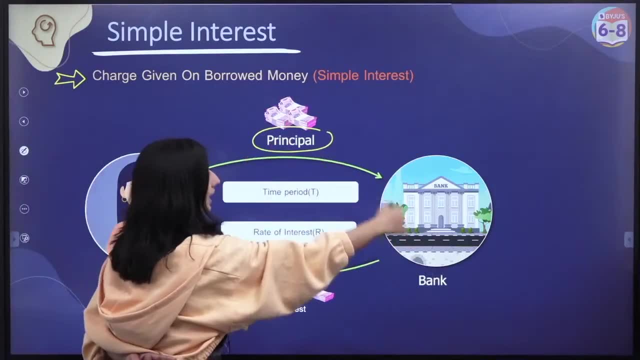 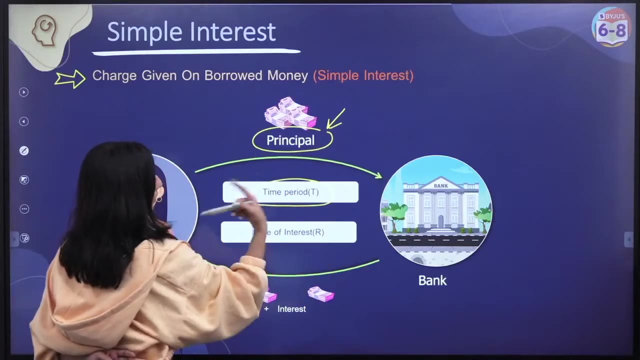 See, we have three things that you have to keep in mind. One is principle Amount- that is being borrowed, or the amount that we are depositing in a bank. that is called principle amount. Okay, Then, for how long we are depositing or we are borrowing the money. 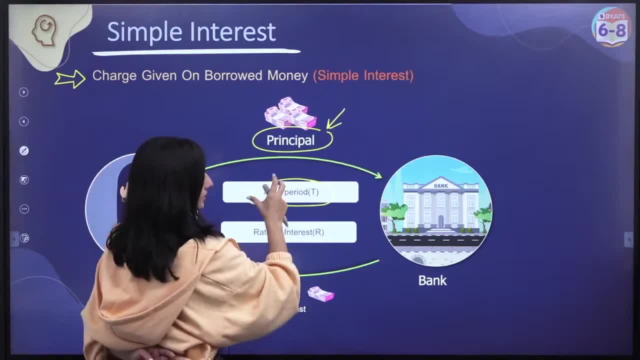 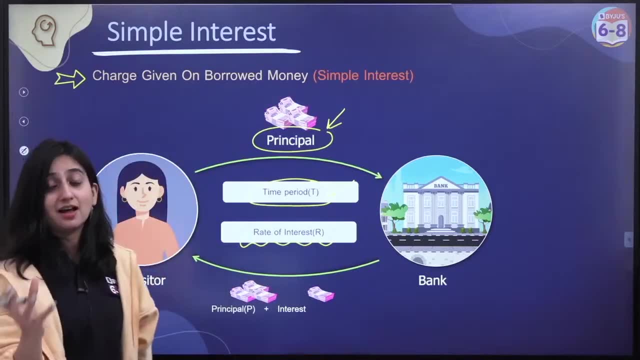 Okay, For how long we have to keep that money in the bank- That is my time period- And how much rate of interest will it take. That means how much additional will I get on it. If I am depositing the money bank will give me additional money. 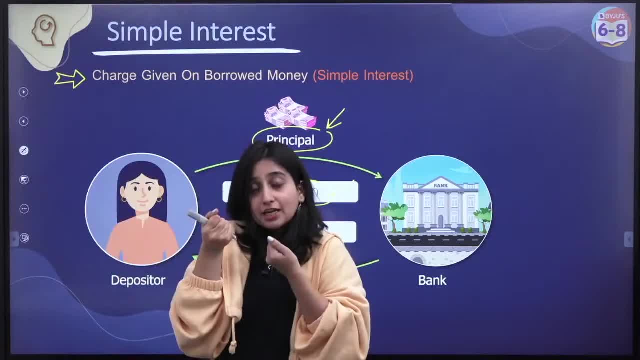 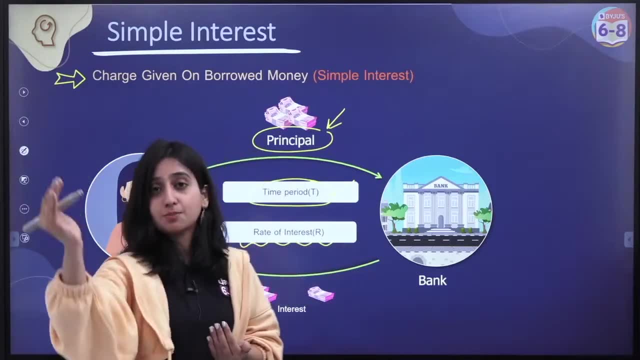 That is interest. it will pay me. If I am borrowing the money from the bank, if I am taking it from them, then I will have to pay them additional. That is called simple interest. They will have to pay interest. Okay, So from which rate? 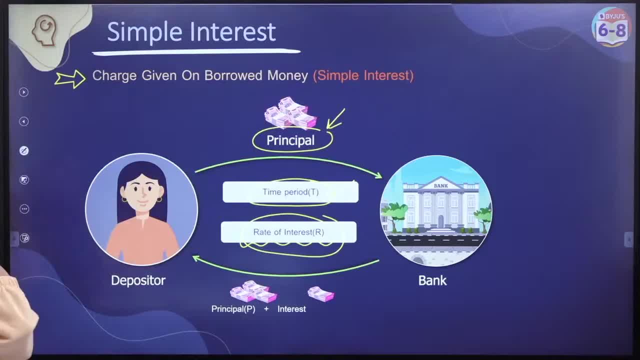 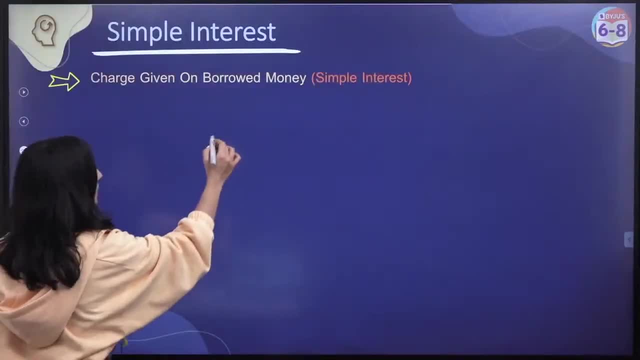 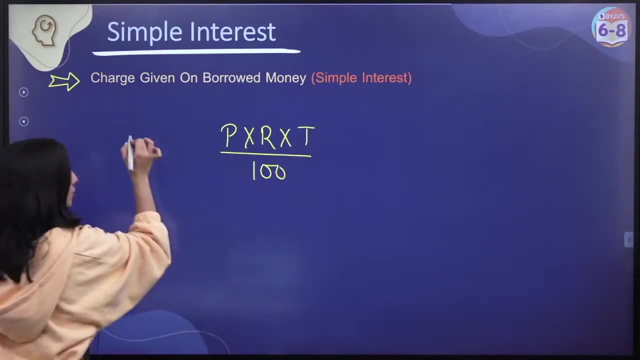 will this percentage be? How much percentage, How much rate of interest are you getting? Okay? So how do we calculate this simple interest? Simple formula is: principle into rate, into time, by 100.. This is how you calculate simple interest, This much interest. 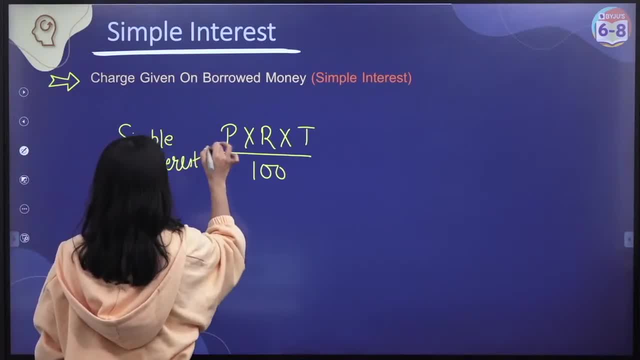 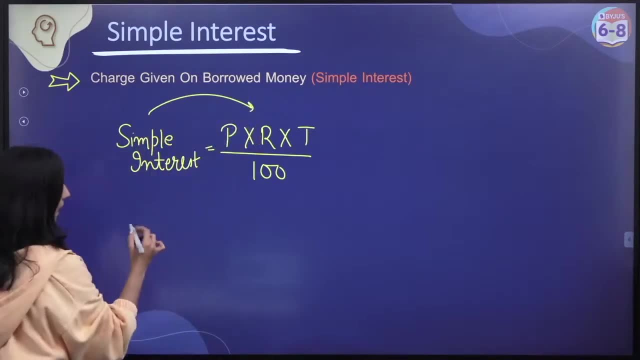 this is how you calculate interest. Okay, Now listen to me carefully. Now listen to me carefully Here. this is the interest. Now, what is the amount? Another term is very important: Amount. Amount means, after interest, what do you have? So what is the meaning of amount? 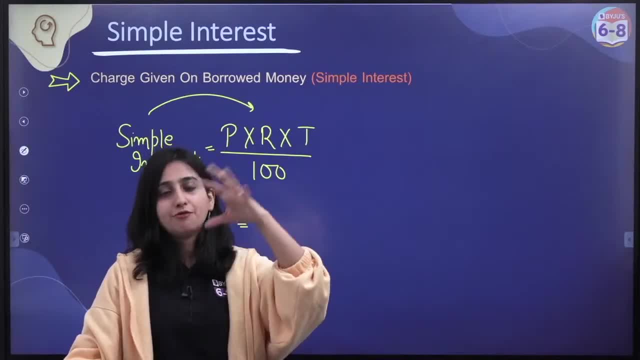 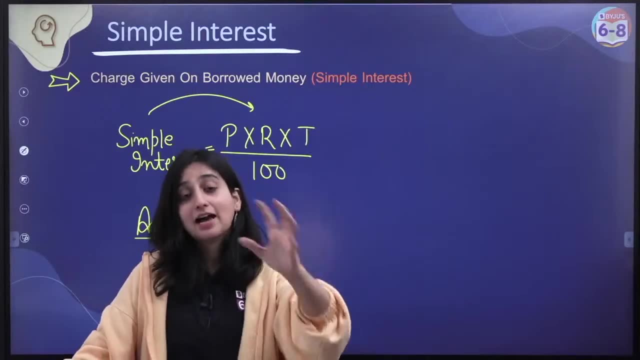 Suppose I have deposited the money in the bank. Okay, I told the bank that in 5 years I will deposit my money. Bank will give me interest, So when I will I will get back my money. then I will have extra money. So why extra? Because by investing interest. 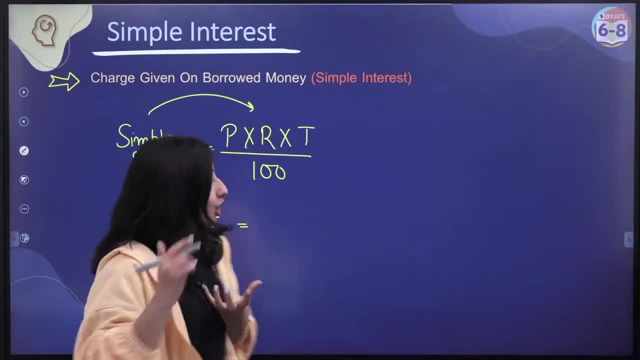 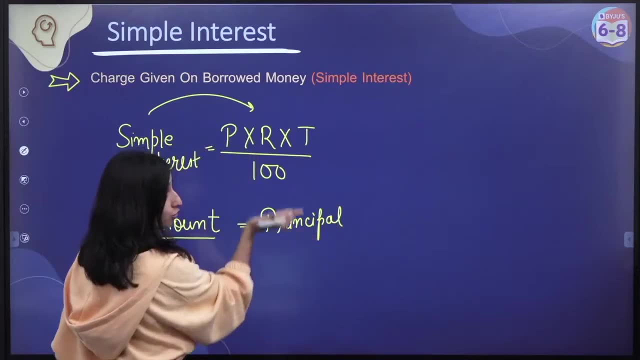 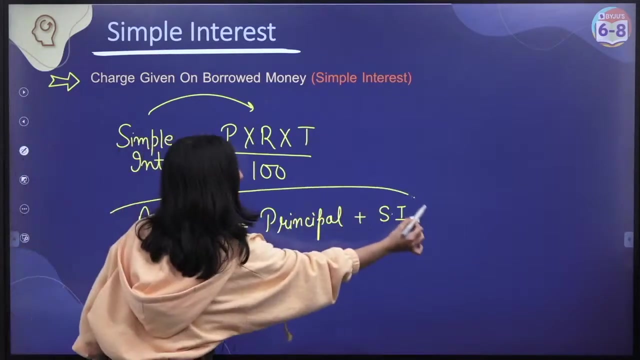 the bank has returned my money. So this means how will the amount be calculated? Amount is equal to principle, which we had given, to the actual amount to the bank plus the simple interest which is invested on it, The interest that will become the amount. 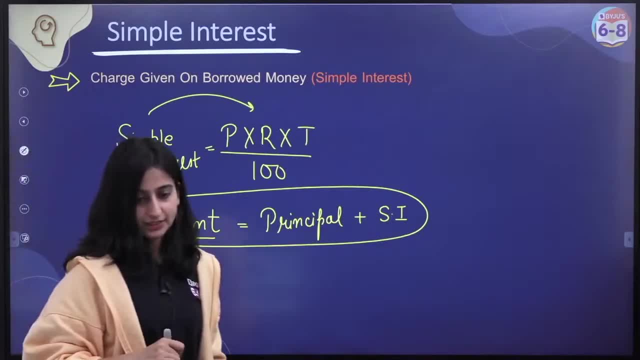 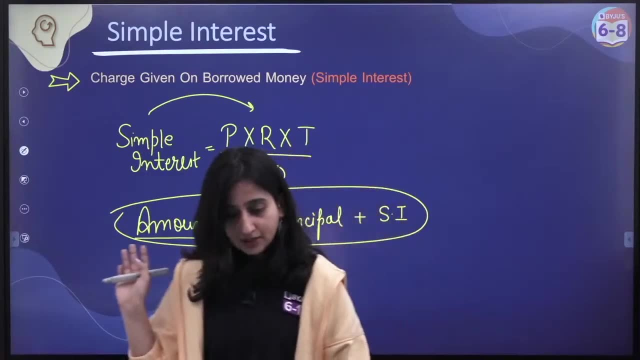 You will get this amount final. Okay, That is principle plus interest. Here we are talking about simple interest. That's why I have written simple interest here. Okay, Is it clear to everyone? Did you understand till here? So many questions are asked on this too. 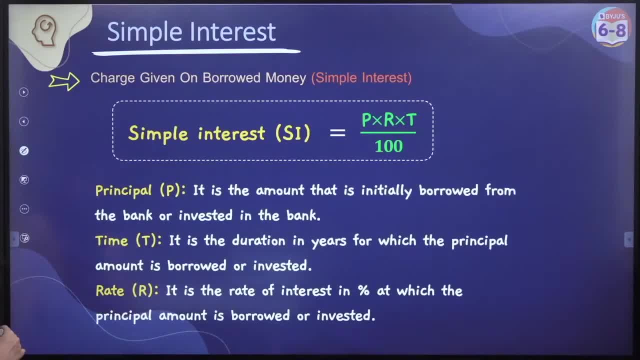 from this chapter. So simple: interest is PRT by 100.. And now you know what is principle Amount that is initially borrowed from the bank or invested in the bank. What is time? It is the duration in the years. It is very important We always take it in the years. 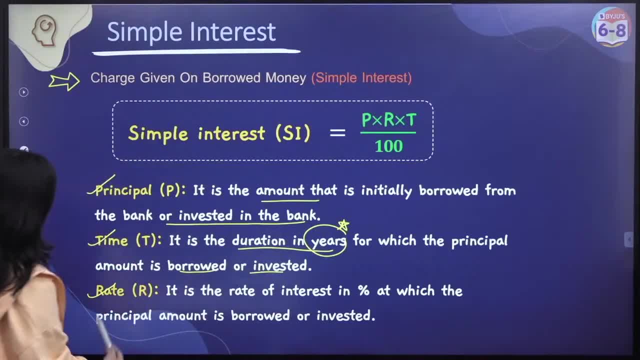 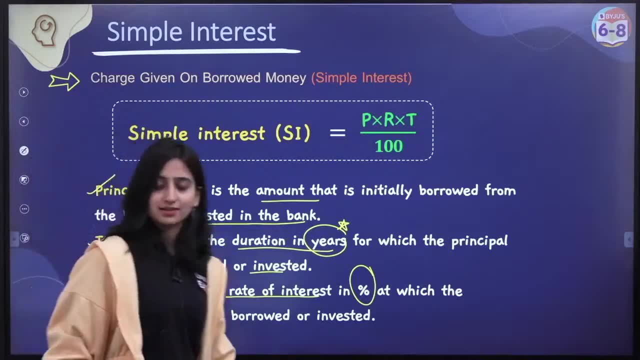 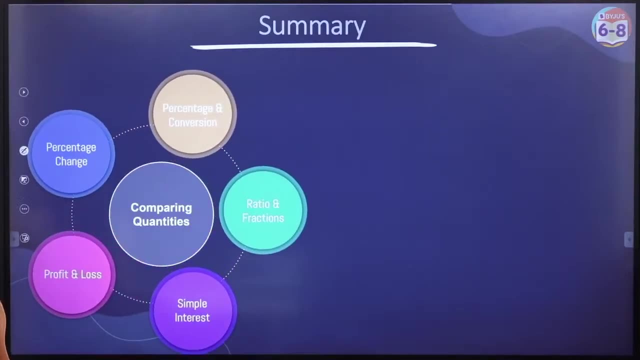 For which the principle amount is borrowed or invested, And rate is basically the rate of interest in percentage at which the principle amount is borrowed or invested. Okay, Now let's solve the questions. Let's quickly go through the summary that we did. So we did. 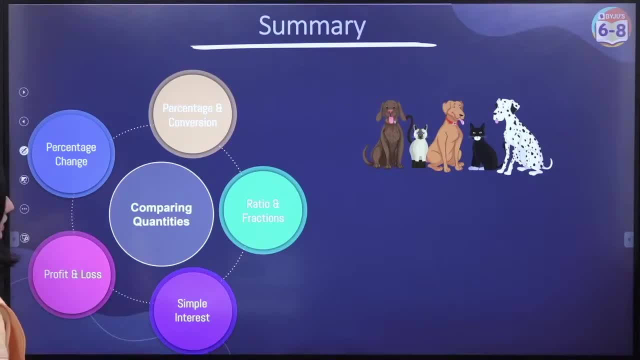 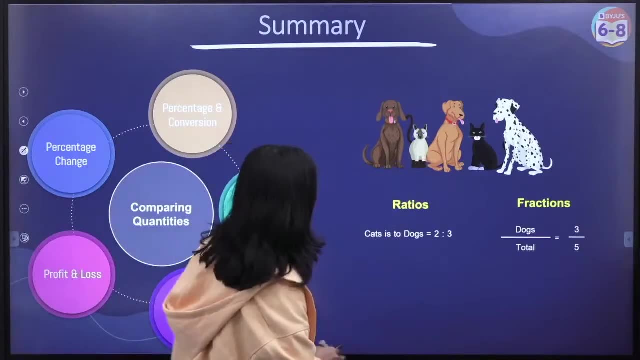 what is ratio? We had talked about ratio. Okay, What is ratio? Basically, comparison by fraction. So here we are finding: cats to dog ratio. So number of cats, how many cats we have? 1, 2. Okay, So. 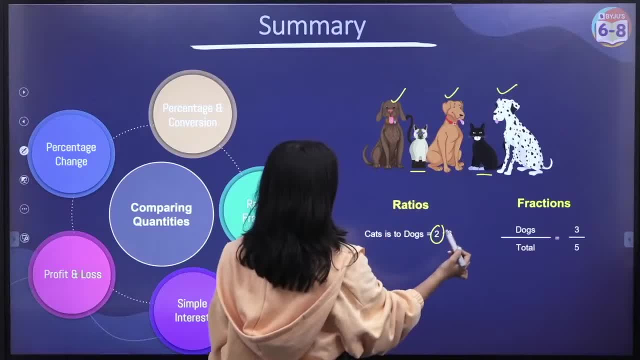 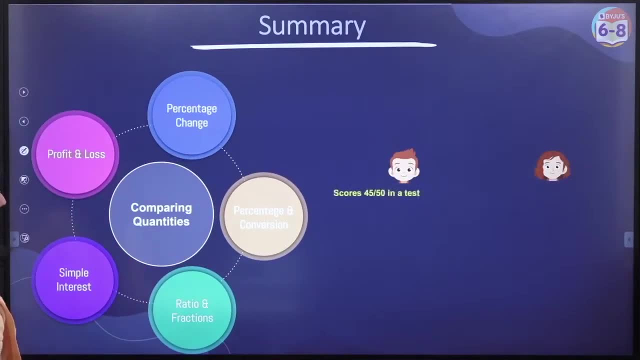 cats are 2, and how many dogs are there? 1,, 2,, 3.. So the ratio will be 2 is to 3.. Okay, Now let's move ahead. Then we talked about percentage. How did we calculate the percentage? 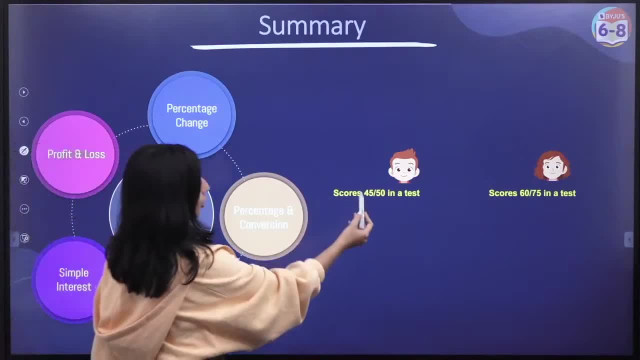 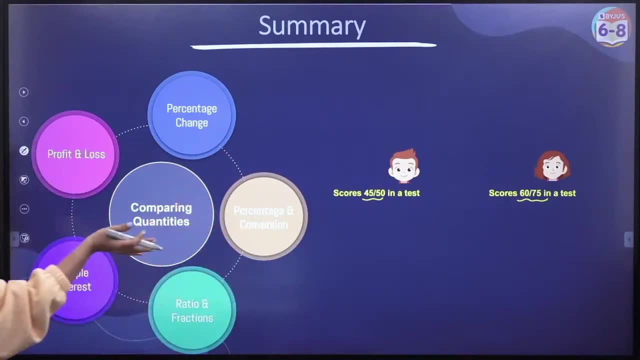 We learnt how to calculate the percentage. If this boy is scoring 45 out of 50 in the test and this girl is scoring 60 out of 75 in the test, So who is performing better? How will we calculate? We will calculate the percentage. 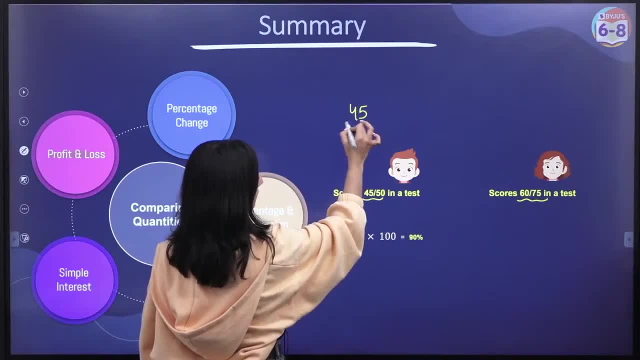 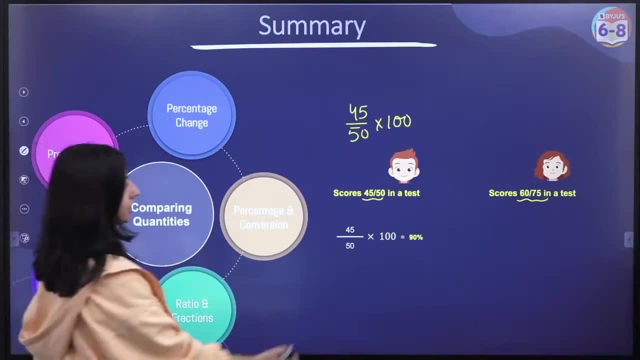 And how do we calculate percentage? By multiplying the fraction by into 100.. Right, We will multiply this fraction by 100 and we will get the percentage. So this boy is getting 90% and this girl is getting 80%. That means boy. 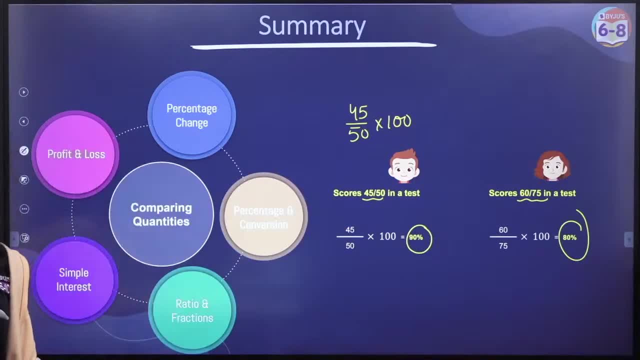 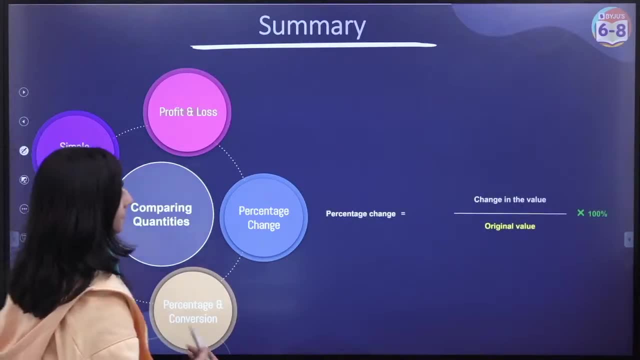 is performing better than this girl. Okay, Yes. The next thing that we studied was profit and loss, Right, So what did we see in profit and loss? What is profit percentage? How to calculate loss percentage, Then, what is percentage change we have seen there? 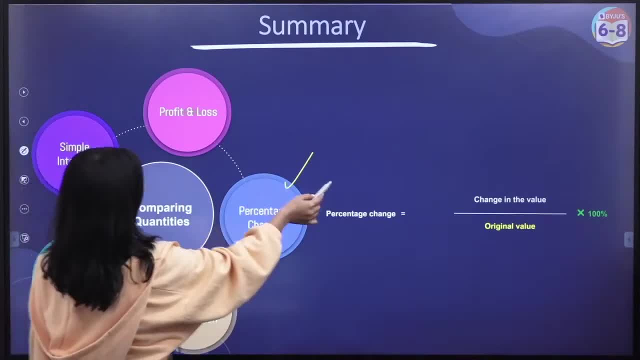 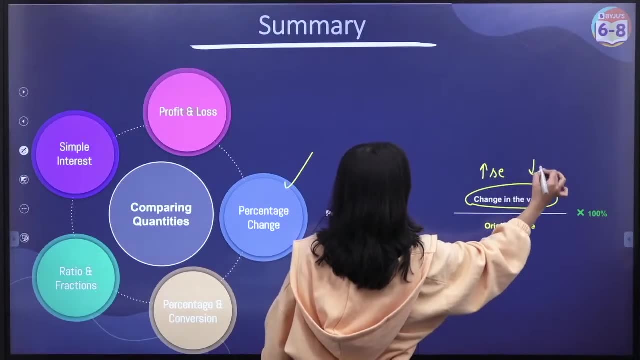 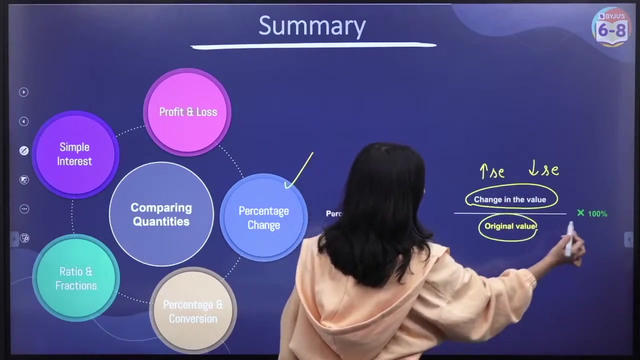 Okay, here first we will talk about percentage change. We studied percentage change, That is, change in the value. Whatever the change it can be, It can be increase or decrease. Percentage can be increase or decrease. Okay, So how much change happened upon the original value? 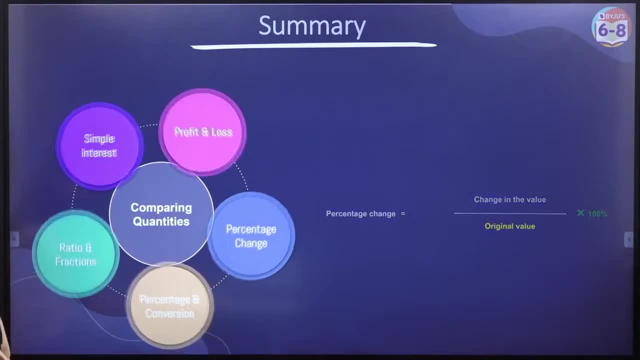 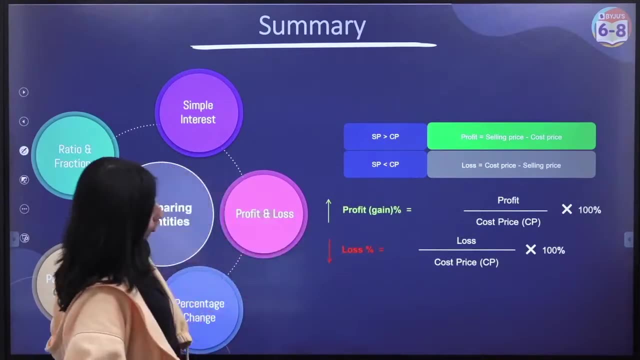 into 100.. That is how we calculate the percentage change. And then, if we talk about profit and loss, we started. how do we calculate gain percent or loss percent? So how is it done? Profit by cost. Always keep the cost price in the denominator. 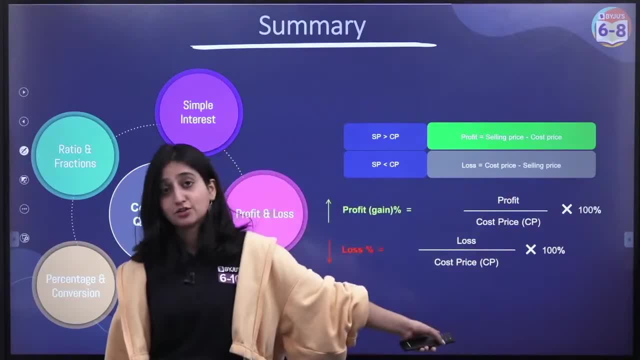 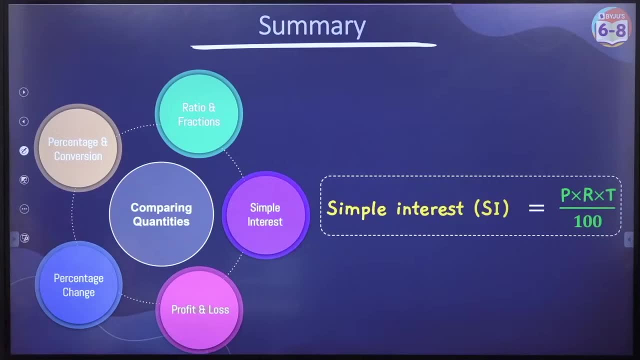 Profit by cost price into 100.. Loss by cost price into 100 will give us loss percentage Easy peasy. Did everyone understand? Yes, Let's go Now the simple interest that we just studied, that is, PRT by 100.. 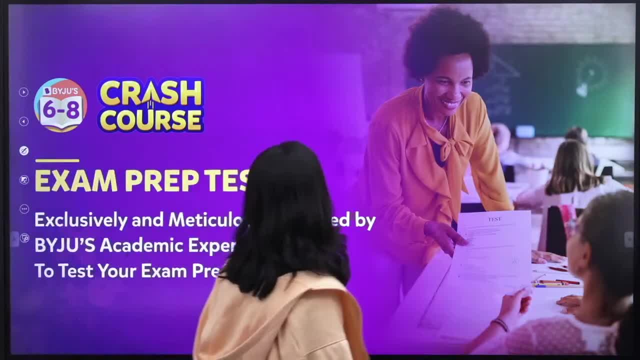 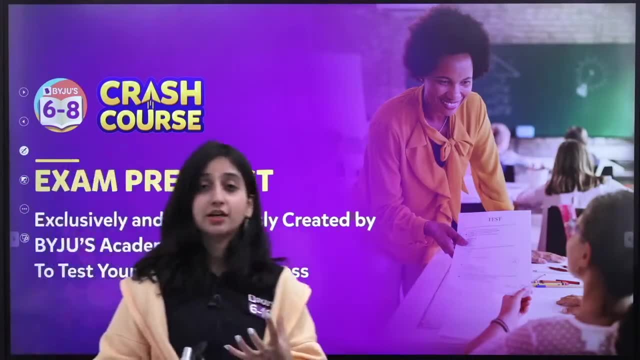 There is one more exam prep test left. You will get the link in the description box. If you are not feeling that confident, or if you want to prepare well and want to check that how well you have prepared, then this test has been prepared by the academic specialists. 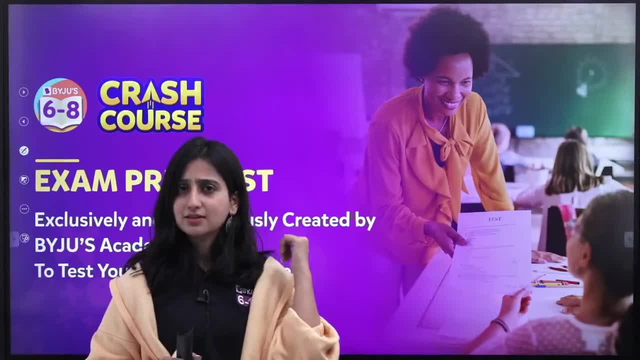 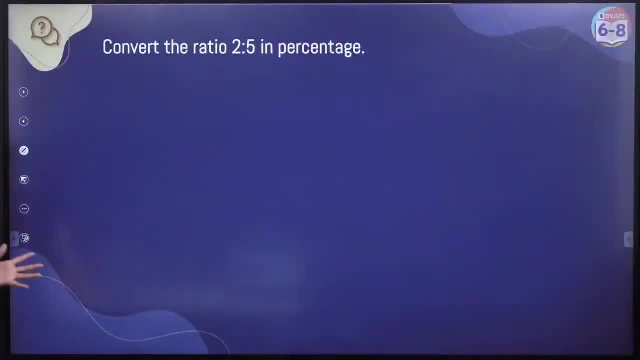 for you. Okay, So you can go. you can check this link in the description. Go and attempt this test. You will get some idea that how much more effort you have to do and how much more preparation you have to do. Now let's move on. 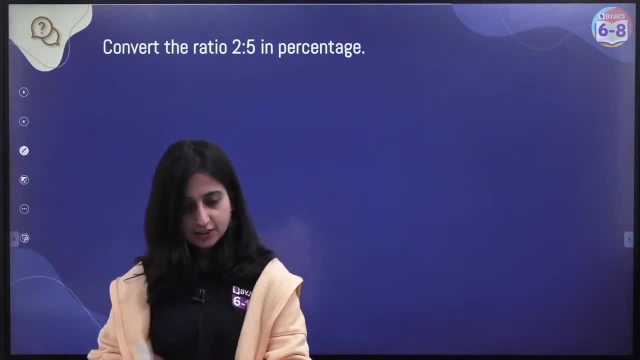 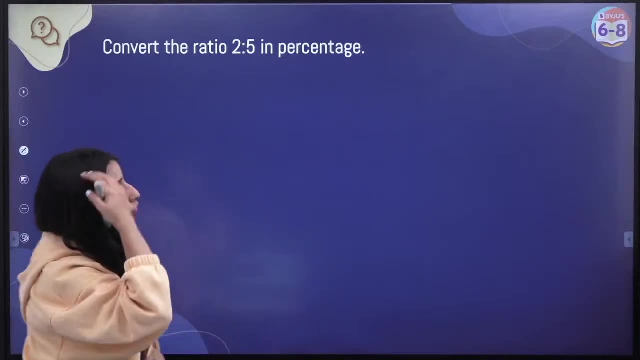 to the questions. Let's go Now. let's solve the questions quickly. Yes, son, this one will be online. Yes, Let's solve the questions now. So question number one: Convert the ratio into percentage. See, now you have to participate. 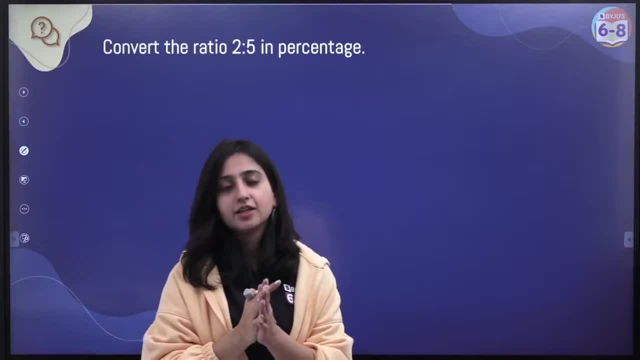 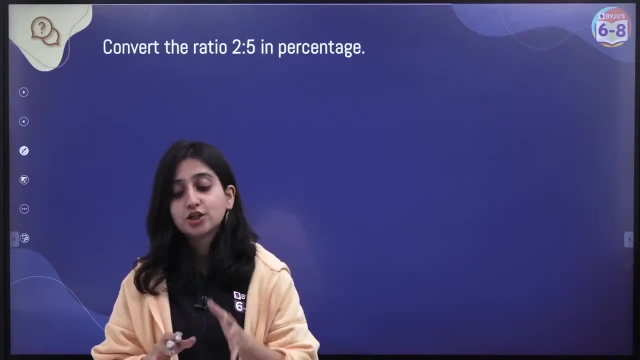 actively in the chat. Quickly keep telling me the answers in the chat. I will take your names. you give me the answers in the chat. So first question says: convert the ratio 2 is to 5 into percentage. Very good, Harshit Mastan. very good. 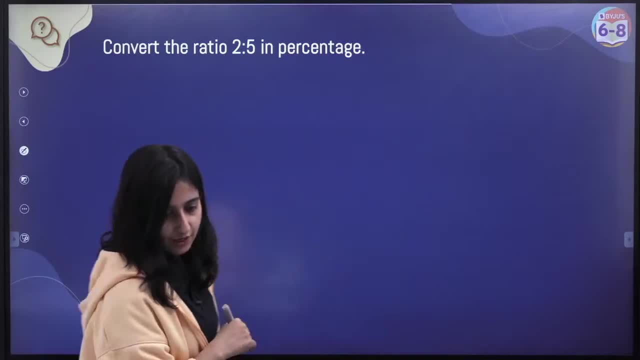 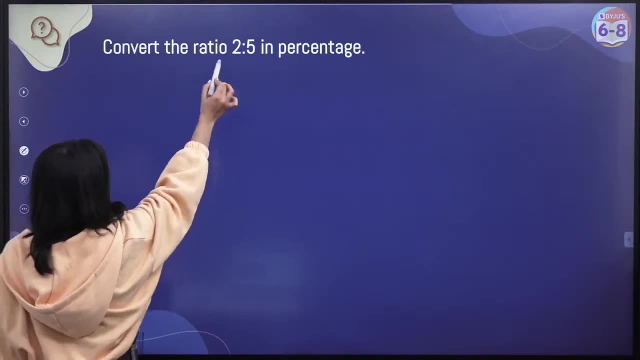 Vivek, Miss Unique, Nidhi, Venu, Sneha. very good children, Amit. wrong answer is coming. See, you have the ratio 2 is to 5.. So how will you change it into percentage? First, change the ratio into fraction. 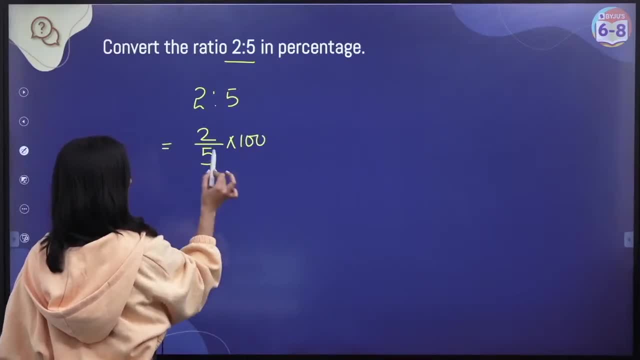 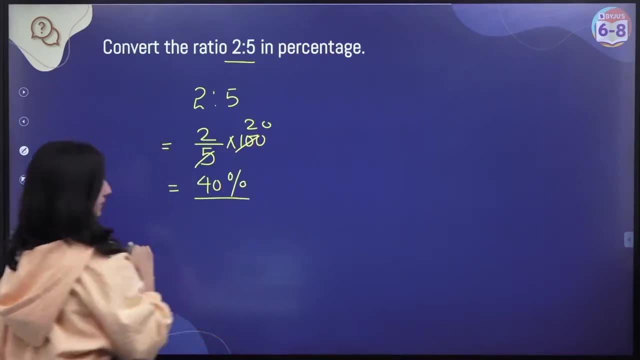 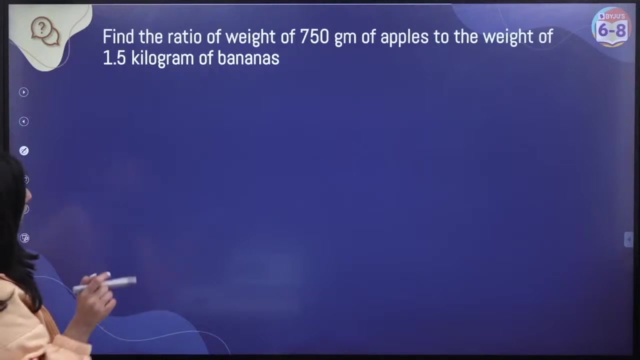 Then multiply it by 100. So you will get how much 5 into 20 is 100. So this becomes your 40%. How much did you get? 40% is the right answer. Come on next question: Find the ratio of the weight. 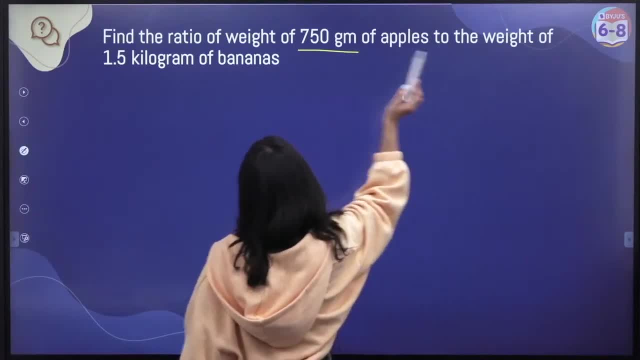 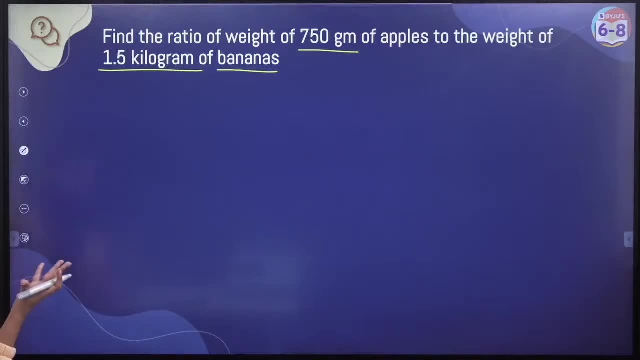 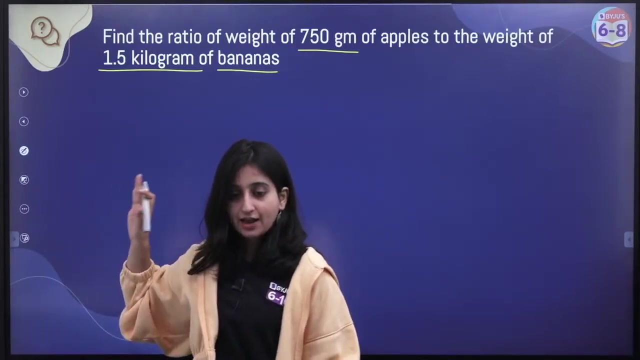 of 750 grams of apples to the weight of 1.5 kilograms of bananas. So we are comparing the weight of apples and bananas. We are taking their ratio. So tell me quickly what will be their ratio. Quickly give me the answers in the chat. 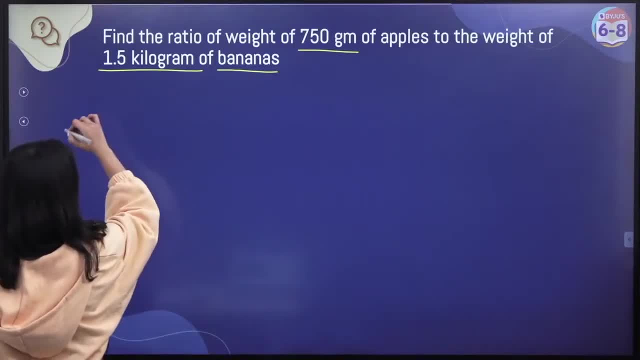 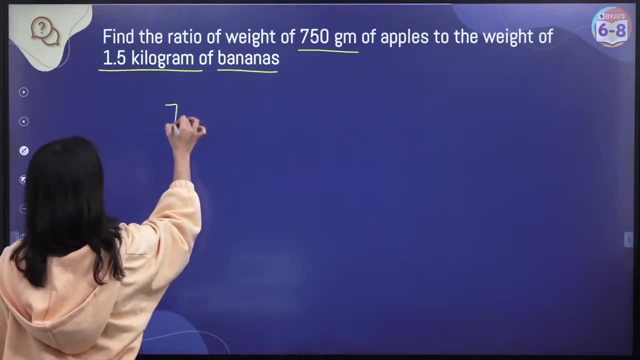 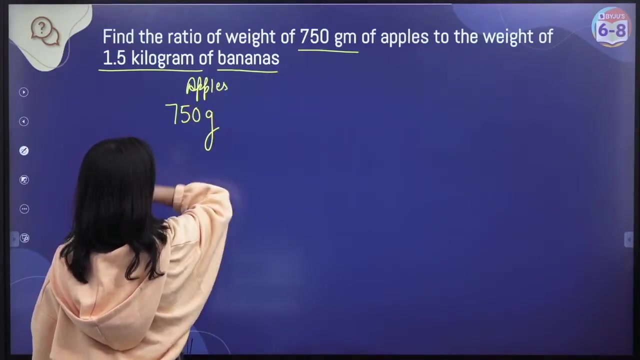 Quickly give me the answers in the chat. So weight of weight of 750 grams of apples. So how many apples do we have, 750 grams, And how many bananas do we have? The amount of apples we have is this much? Weight of 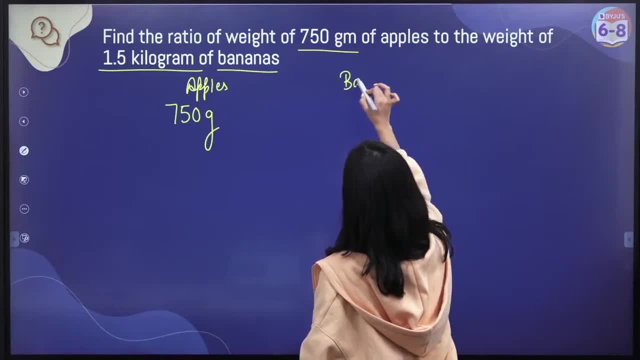 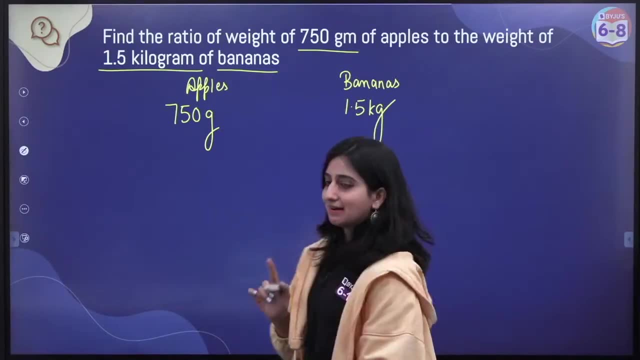 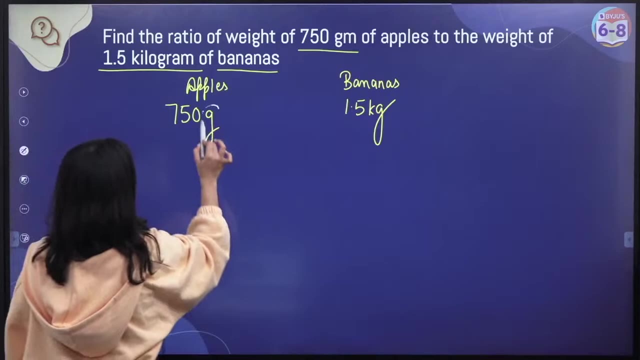 apples is 750 grams and weight of bananas is. weight of bananas is given as 1.5 kg. So tell me what is the first thing you have to do? Very easy, right, Yes? So first of all, if you notice here units- 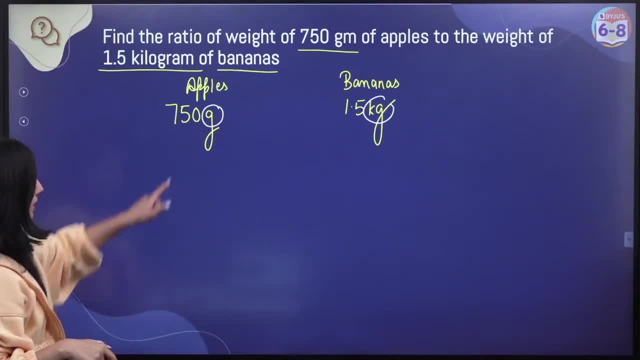 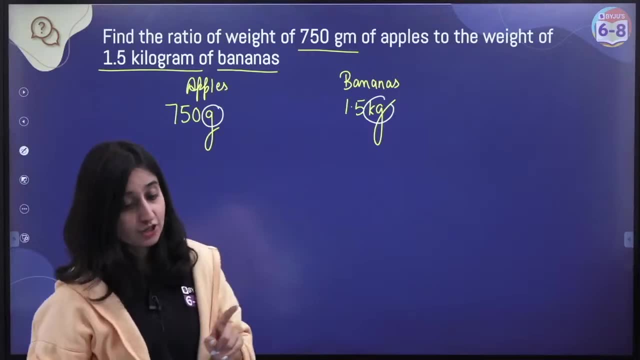 are not same. Here we have kilograms, here we have grams. Either we have converted this into kgs or grams. Whichever you find easier, go with that. Just make sure to convert the units. It is very important to do the same, So I am taking 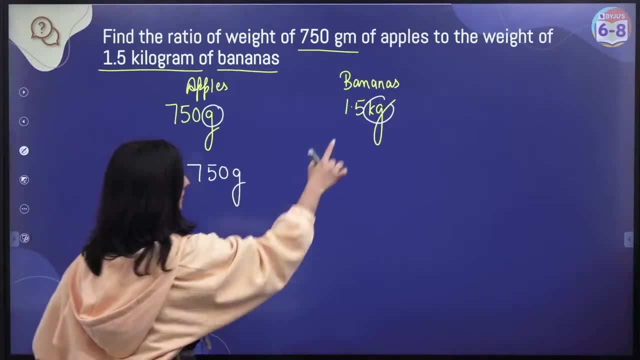 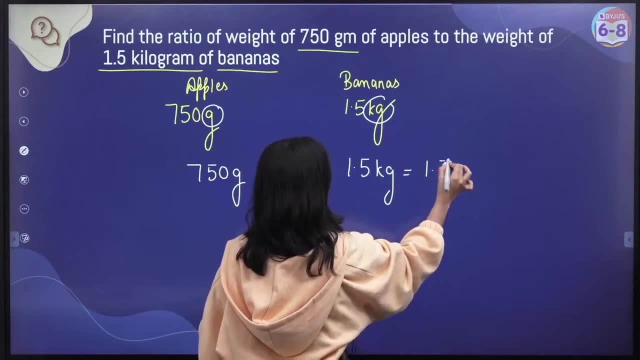 this grams as it is, I am taking this grams as it is and I am converting these bananas- 1.5 kgs- into grams. So what is 1.5 kg? equal to 1.5 into 1000 grams, Because how many grams are there in 1 kg? 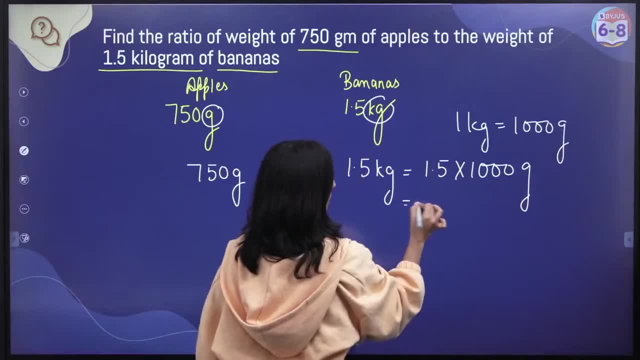 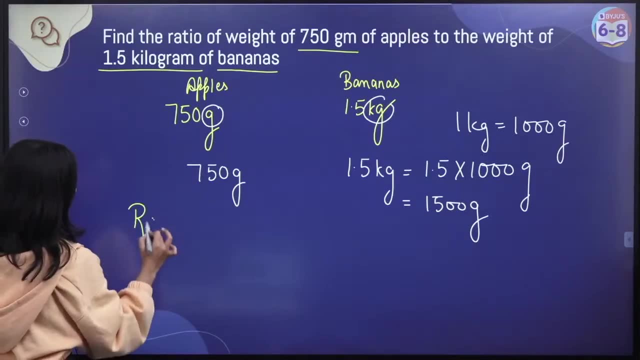 1000 grams, Right. So how much will we have? 1500 grams? Now we will take the ratio. Now we will take the ratio. So what is the ratio equal to? Ratio will be equal to 750 upon 1500.. 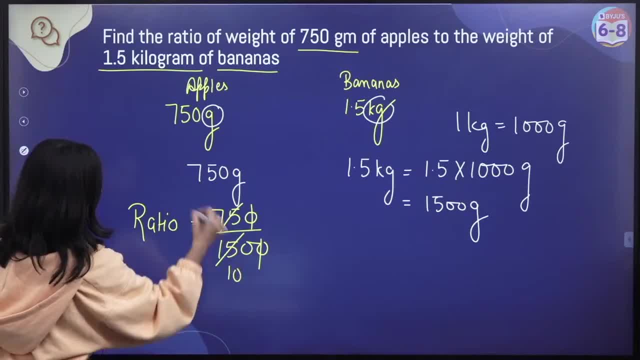 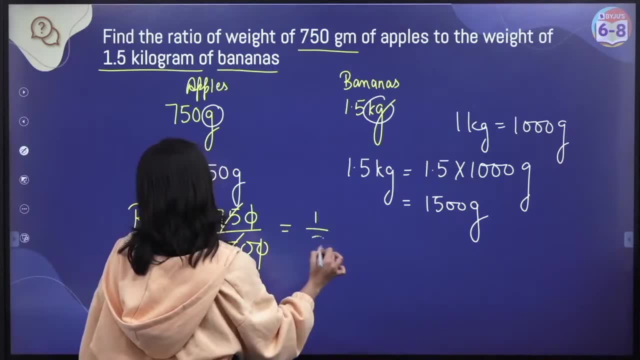 So this went on the table of 15.. You can say it like this: 15 tens, 15 fives, 5 twos, 75 twos are 150 too. So 1 by 2 is the right answer. So this is the ratio. 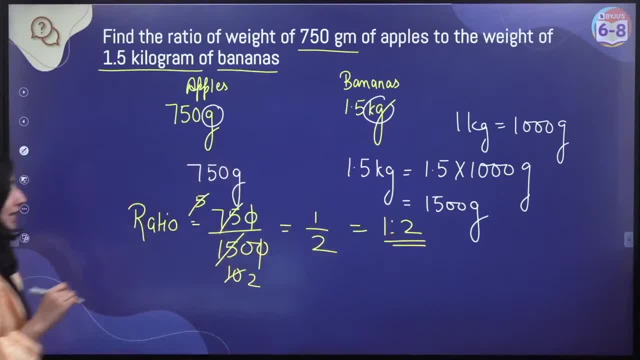 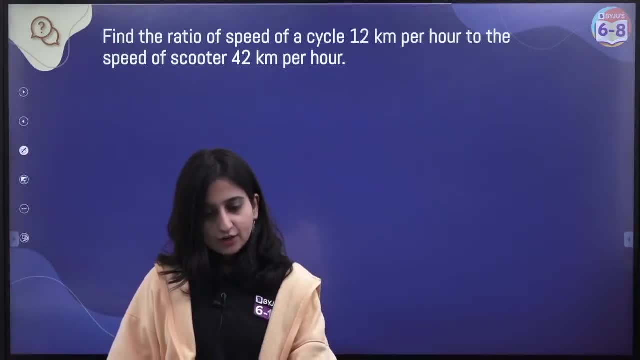 This became a fraction. I am converting it into the ratio 1 by 2.. Next question on your screens. Next question on your screens. Very good, All the children are giving the right answer. Very good, Let's move on to the next question. 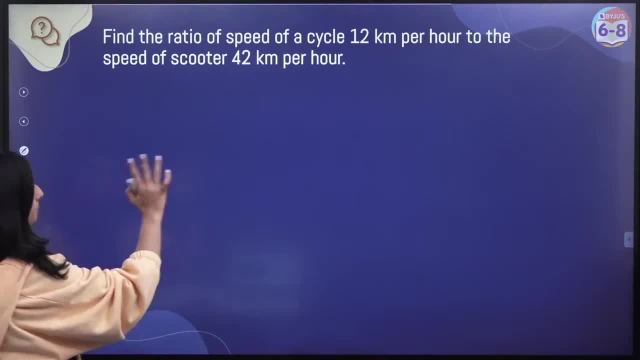 Find the ratio of the speed of a cycle- 12 km per hour- to the speed of a scooter, which is 42 km per hour. So in this question we have been given the speed of cycle and speed of scooter. speed of cycle and speed of scooter. 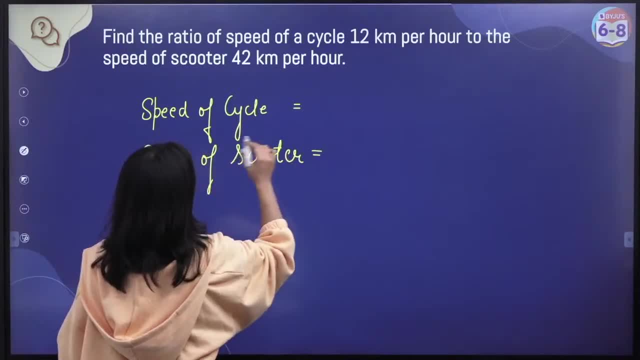 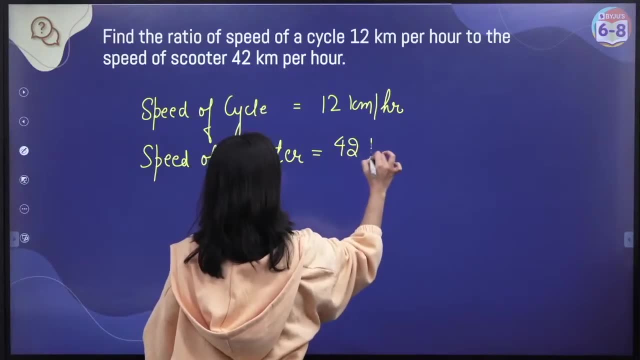 First of all check that the units of both the speeds are same. It is going at the speed of 12 km per hour, It is going at the speed of 12 km per hour And scooter is going at the speed of 42 km per hour. 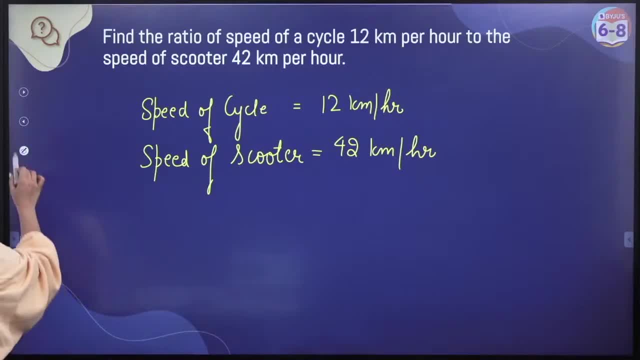 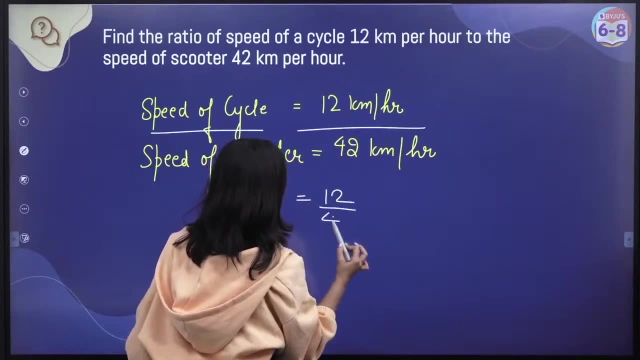 Yes, the units are same. So if you want to take the ratio here, super easy, Just divide these two. If you want to take the ratio, then we will divide these two: 12 upon 42. So how much will it be? 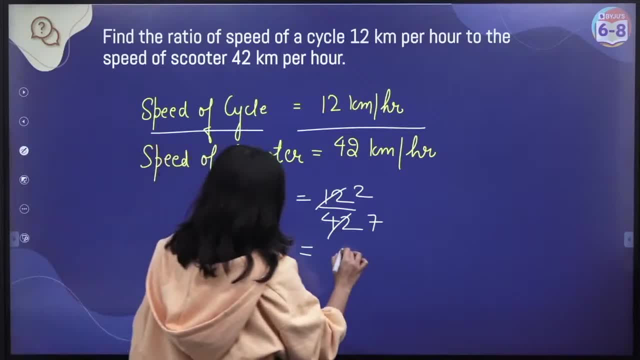 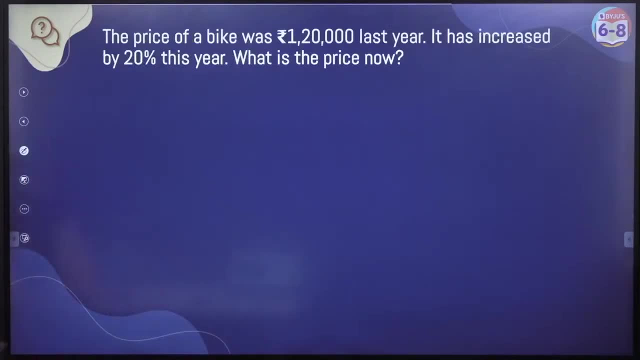 2 by 7, So the ratio will be 2 is to 7.. It went on the table of 6. Easy peasy. Next question: The price of a bike was 1,20,000 last year. It has increased. 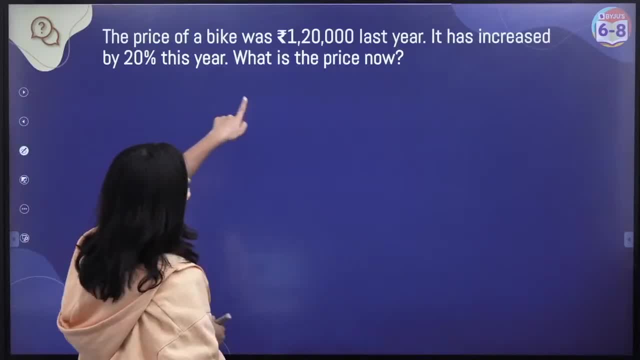 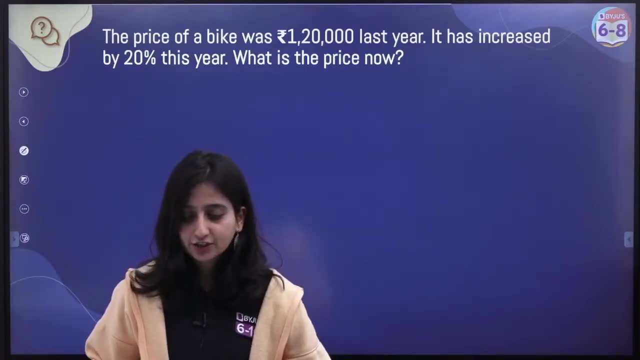 by 20% this year. What is the price now? From which concept is this question being asked? From which concept is this question being asked? Tell me quickly. Yes, The price of a bike was 1,20,000 last year. 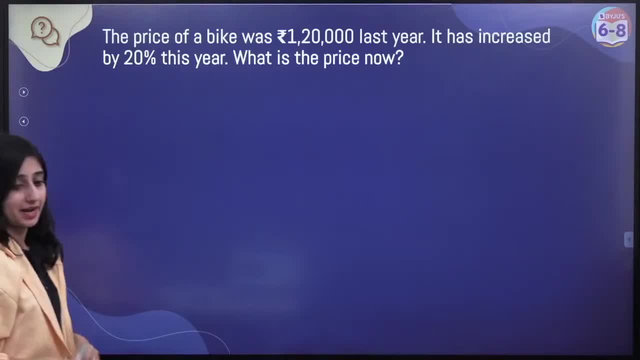 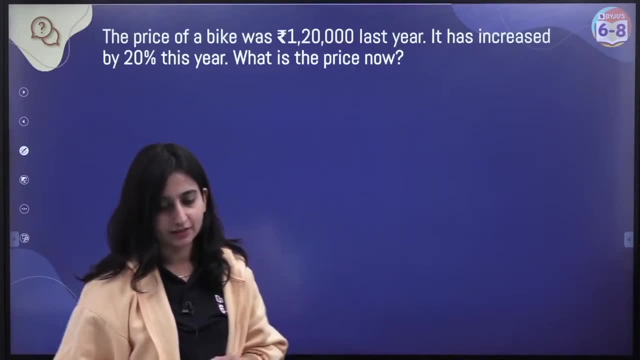 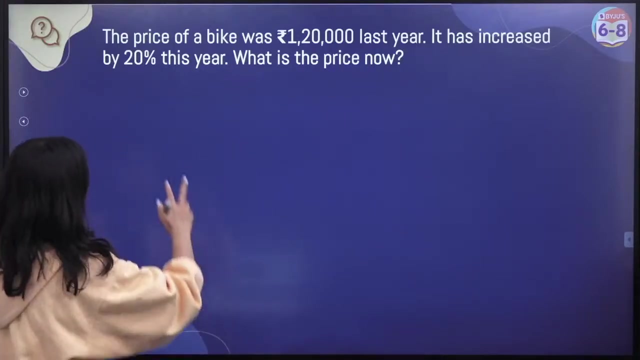 And that price has been increased by 20%. The price has been increased by 20%. What is the price now? Very good Madhyag Mishra. Very good kids. Yes, The price has been changed. The price has been increased. 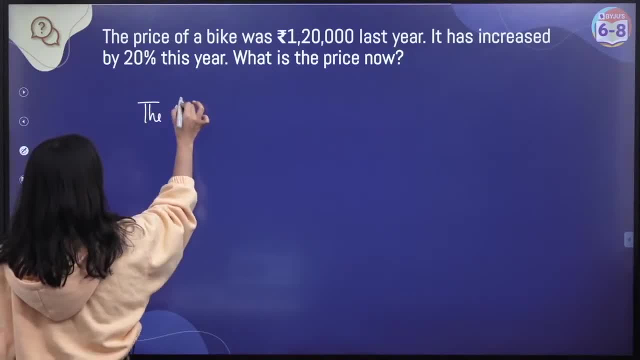 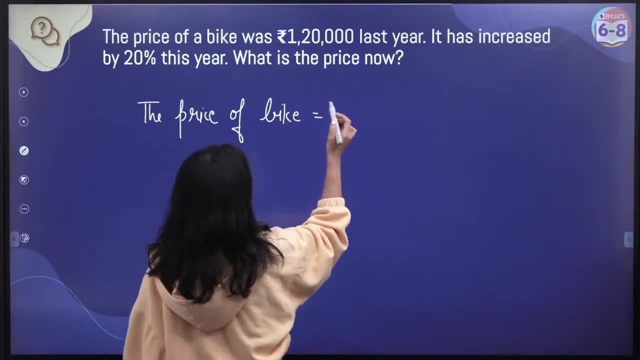 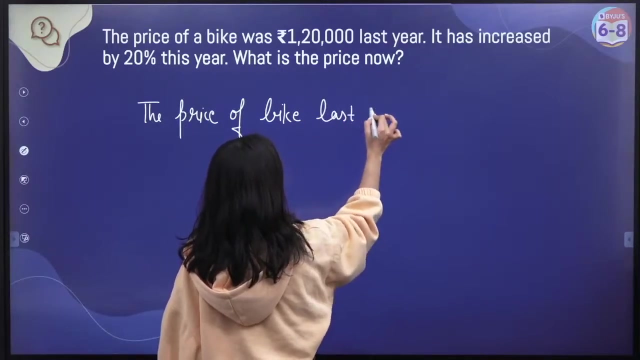 So the price of bike? So the price of bike is given as How much? Tell me last year Price of bike. last year, How much has it been given? How much was the price of bike last year? 1,20,000, 1,20,000. 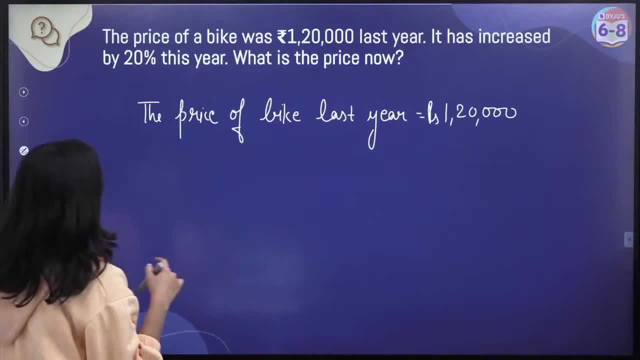 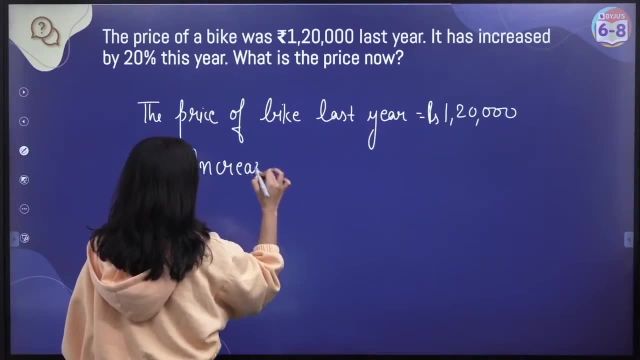 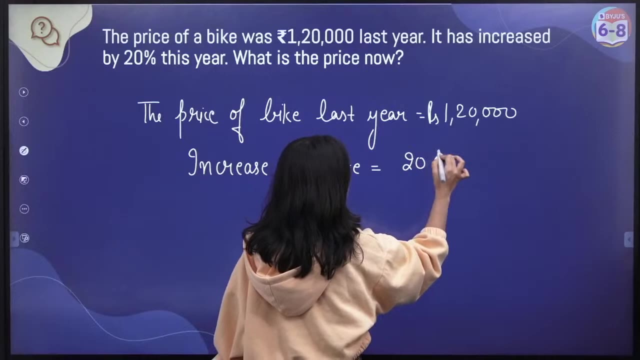 This was the price. Now, 20% increase, Right, So the price has been increased. So how much has been increased? Increase in price: If we calculate the increase in price, then someone will tell me that 20% increase has been done. 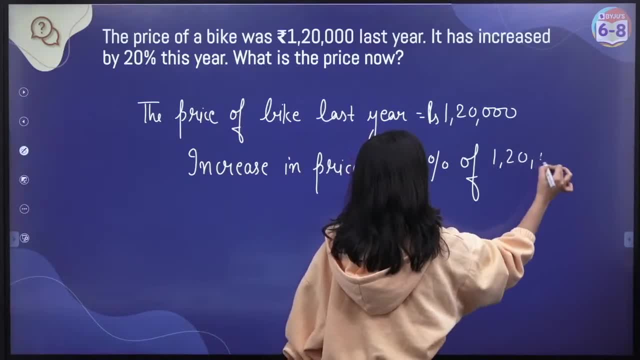 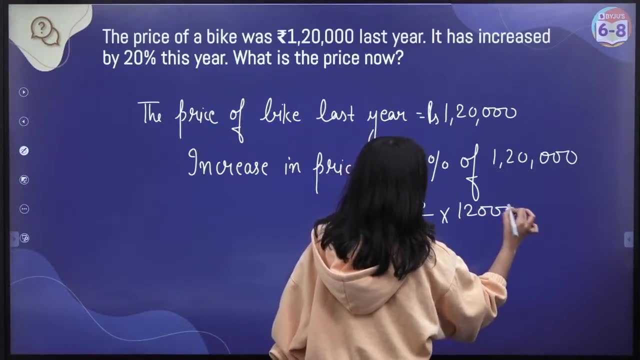 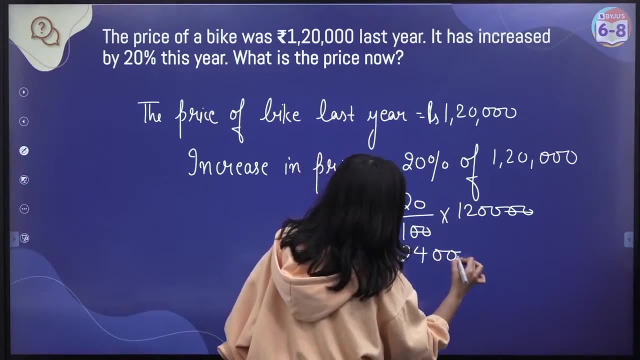 That means 20% of 1,20,000 has been increased, So this means 20%. you have to calculate this. So this will become how much? Rs 24,000, Rs 24,000, Rs 24,000. 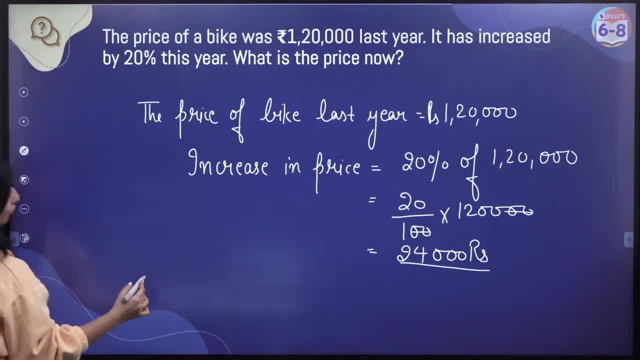 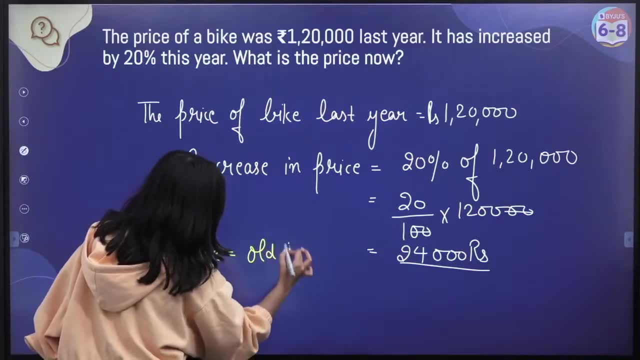 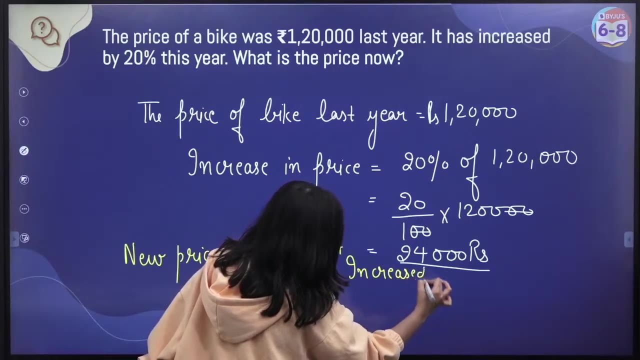 This much price has been increased. So what will be the new price? So what will be the new price? What will be the new price? It will be equal to old price plus increased price. So our price has been increased Right Plus increased price. 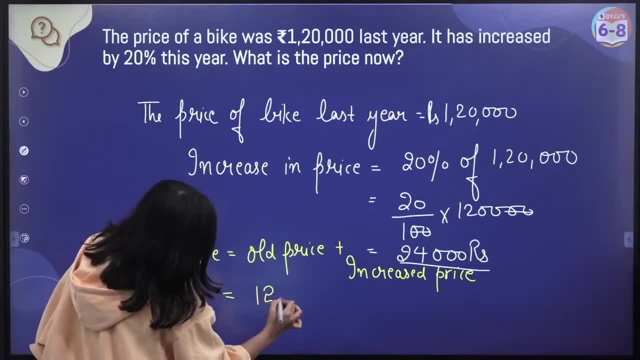 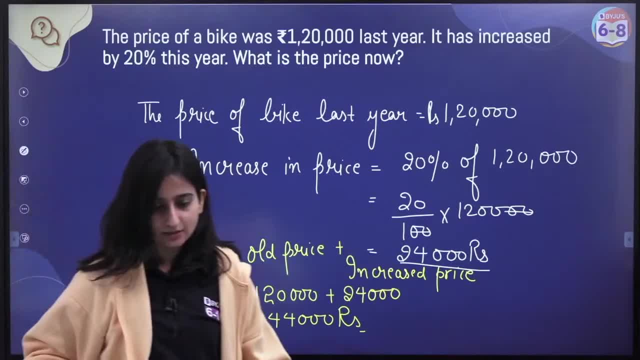 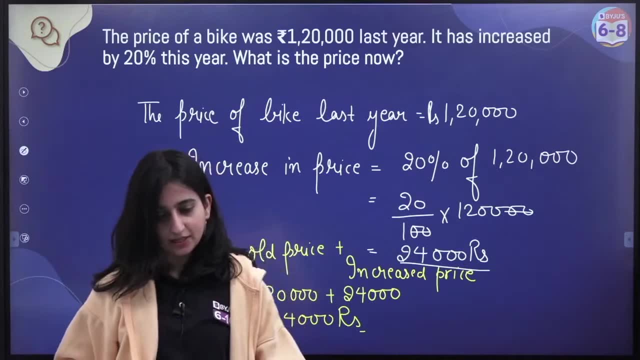 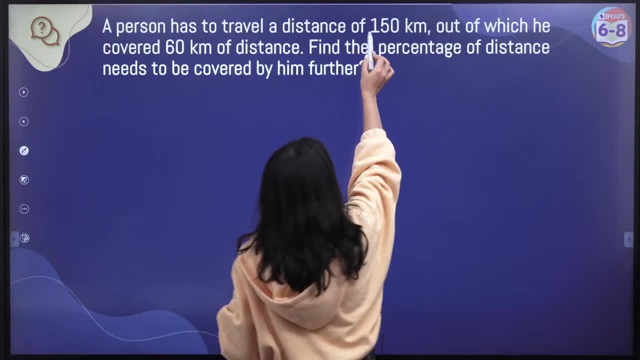 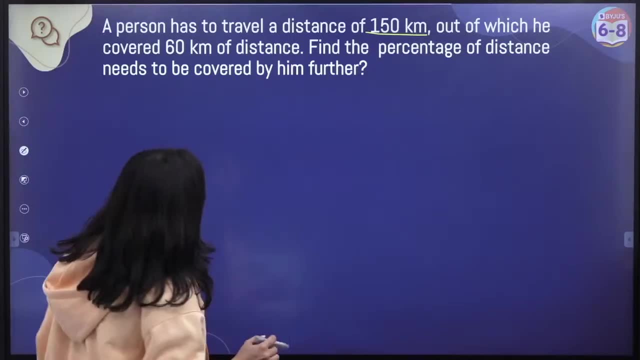 A person has to travel a distance of 150 km. A person has to travel a distance of 150 km. A person has to travel a distance of 150 km Right Now. out of which, Let's make it first: This person wants to travel a distance of. 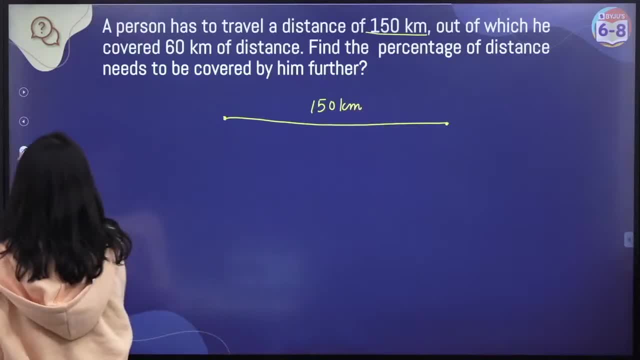 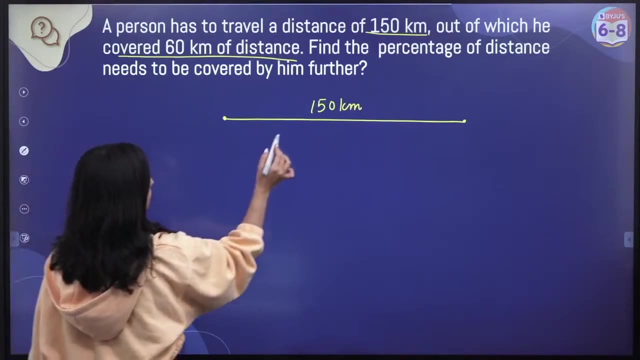 150 km. Very good, He has to travel this distance: 150 km, 150 km, Alright, Out of which he covered 60 km. 150 km, Out of which he covered 60 km. This distance has been covered. 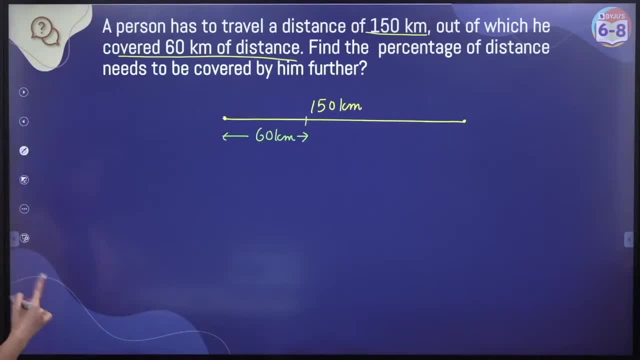 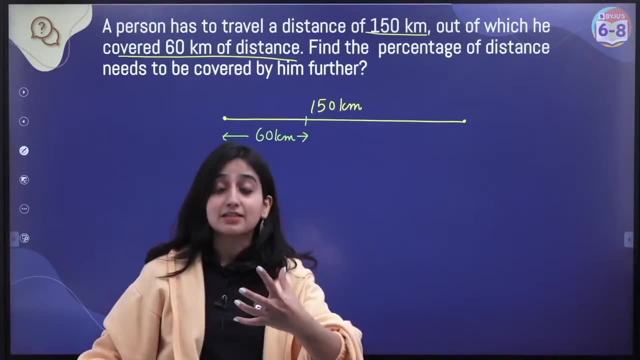 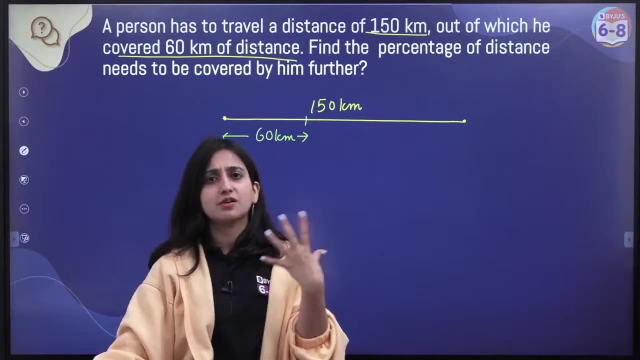 He has covered this distance Right. Find the percentage of the distance that needs to be covered by him further. How much more distance will he have to cover? Tell me in percentage: Is 30% distance left, 40%, 50%, 70%. 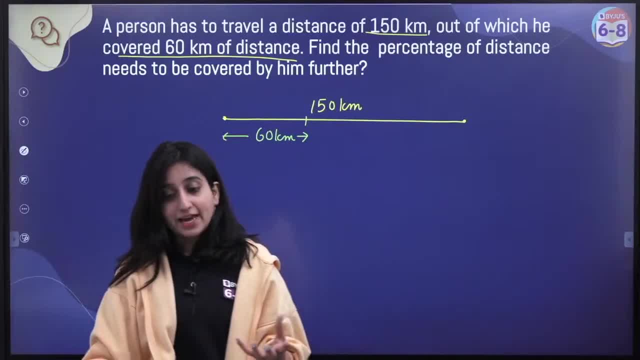 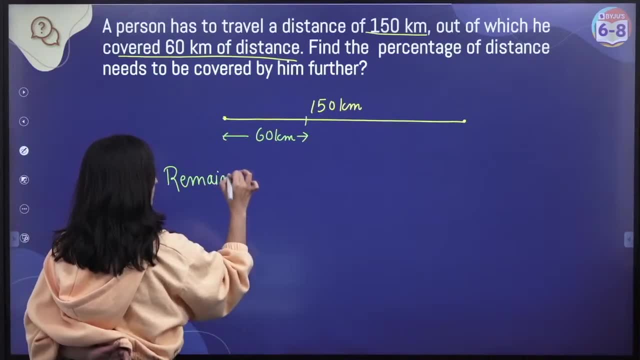 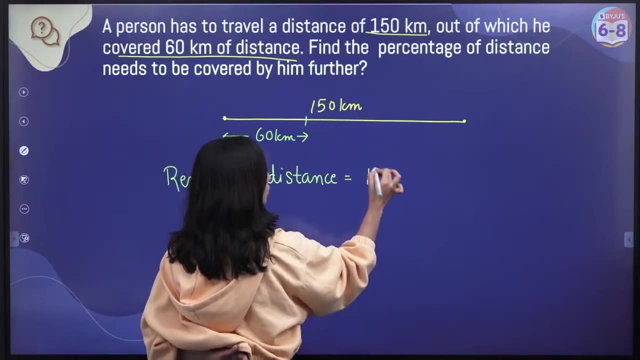 How much more distance will he have to cover? Let's find the remaining distance. Let's find the remaining distance. What will be the remaining distance? What will be the remaining distance that he has to cover? What will be the remaining distance? Remaining distance will be equal to. 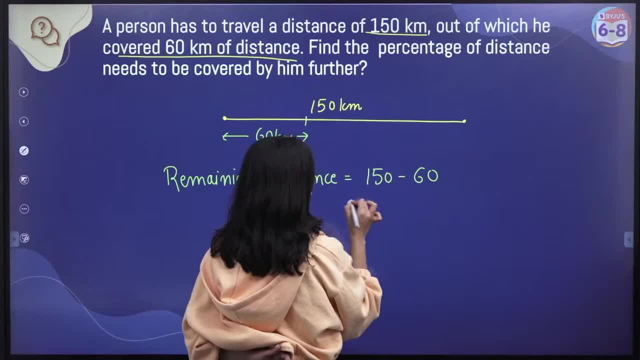 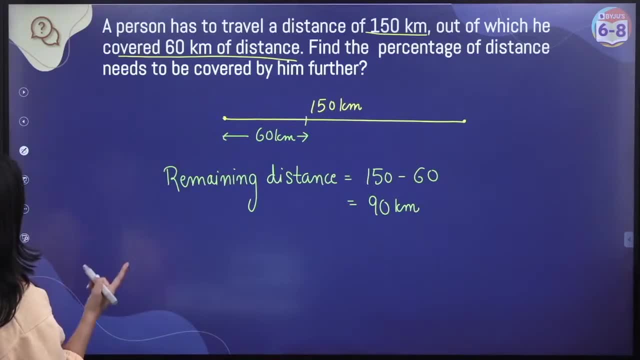 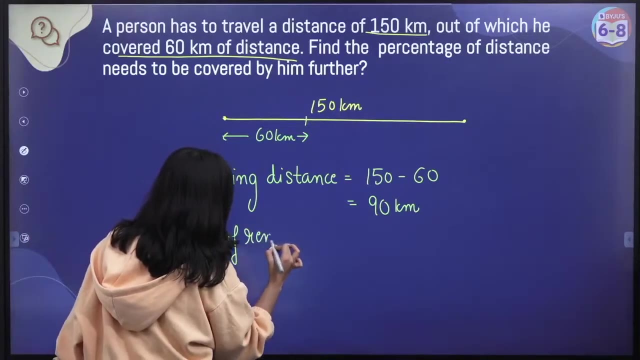 total distance minus the distance covered, that is 60 km. It is coming out to be 90 km. But you have to find the percentage of the distance. You have to find the percentage of the remaining distance. You have to find the percentage of the remaining distance. 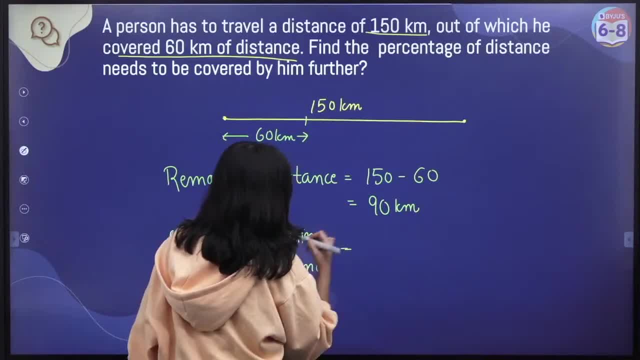 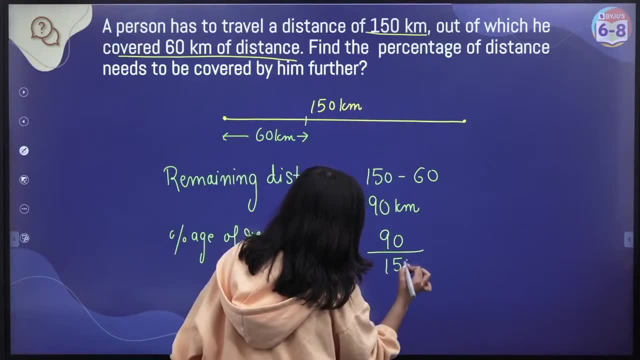 And how do we find the percentage? How will the percentage be? It will be equal to the remaining distance, that is, 90 divided by the total distance. What was the total distance? 150 multiplied by 100. So tell me, how much did it come? 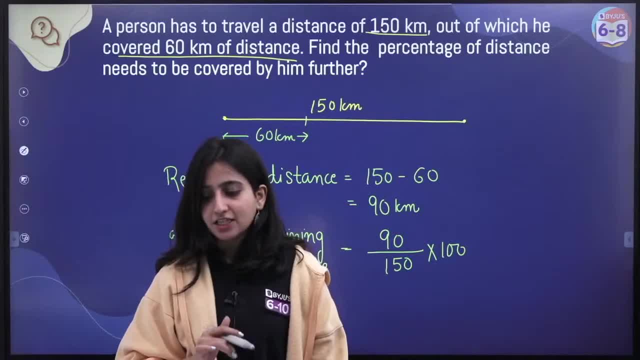 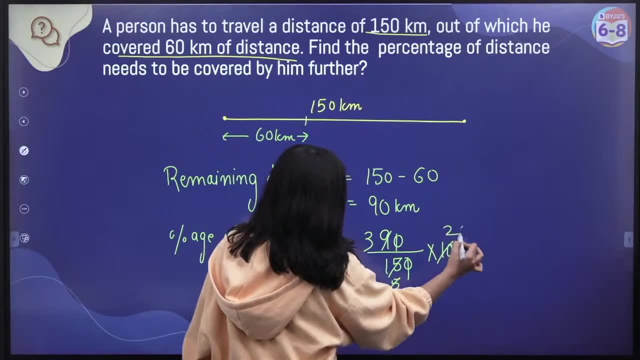 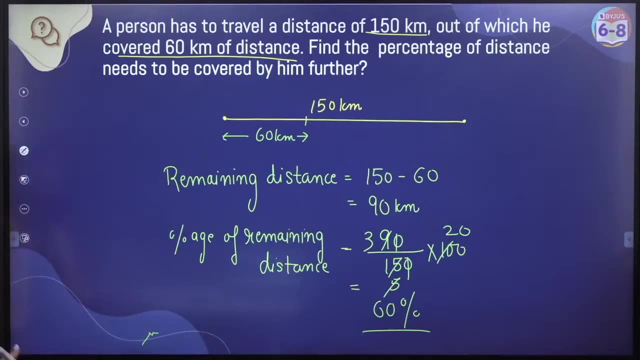 Yes, Yes, it will be in the last. So how much did it come? Can you tell me? How much is it coming? 3 to the 6th. So 60% distance is still left that he has to travel. 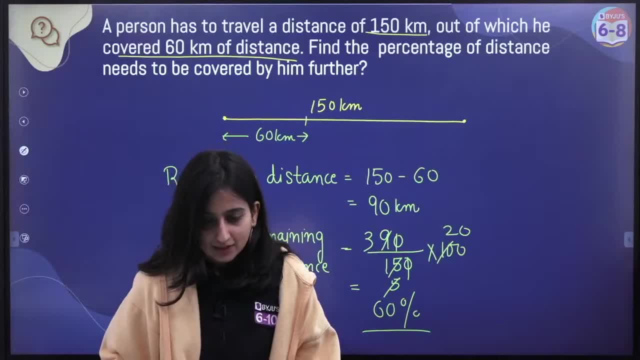 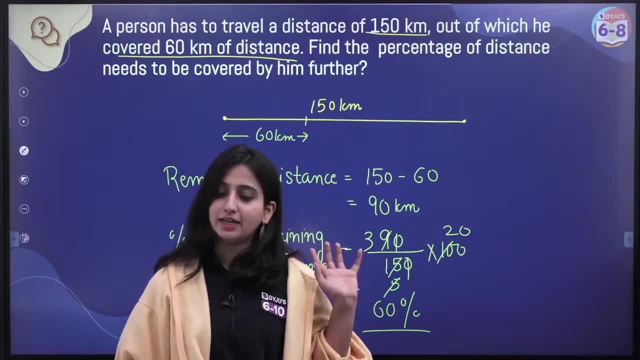 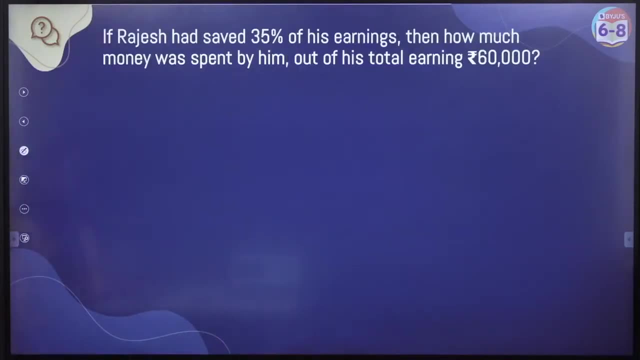 So 60% is the right answer. Clear everyone. Very good, Mubin Menti will start. Let's practice few questions, then we will have the Menti quiz. Let's move ahead. So we will start with Menti. 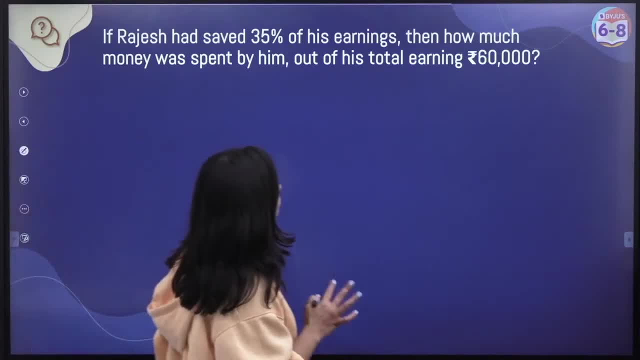 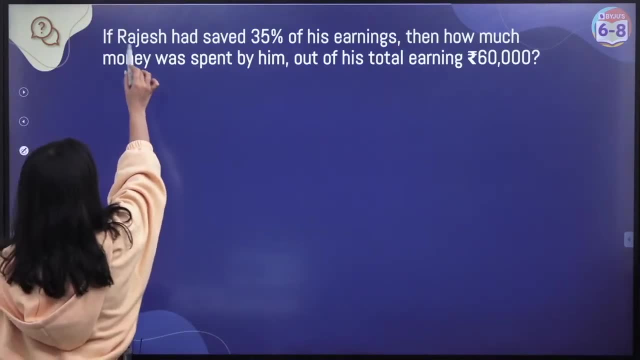 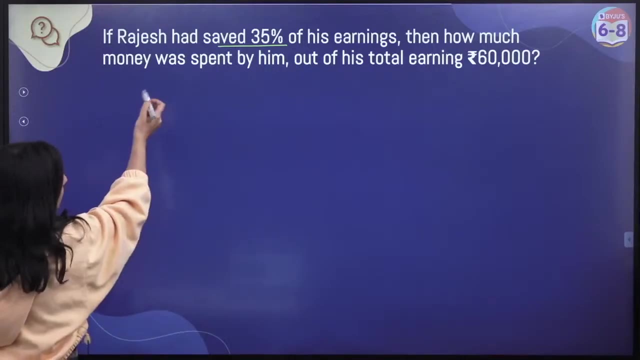 If Rajesh had saved 35% of his earnings? Listen to the question. Listen to me very carefully. Read the question carefully. If Rajesh had saved 35% of 35% of his earnings, then how much money was spent by him out of his total earnings? 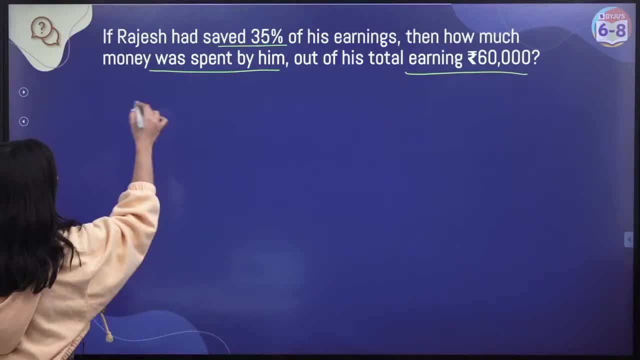 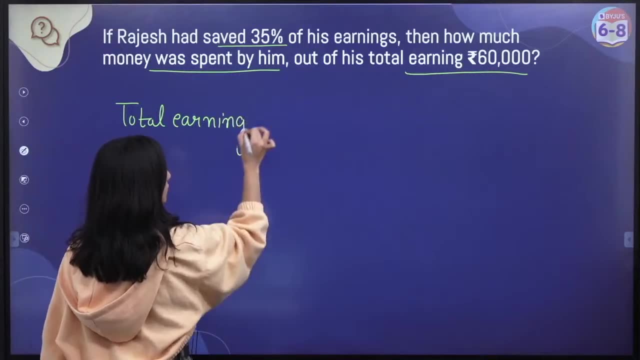 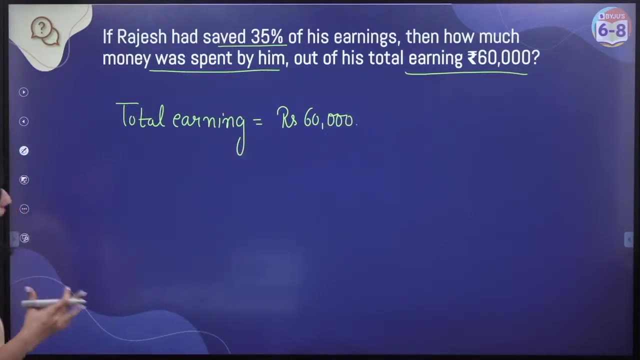 60,000?. Now let's understand this question. What is the total earning? Total earning: How much is Rajesh earning? Rajesh is earning 60,000 rupees. He is earning 60,000 rupees Now, out of. 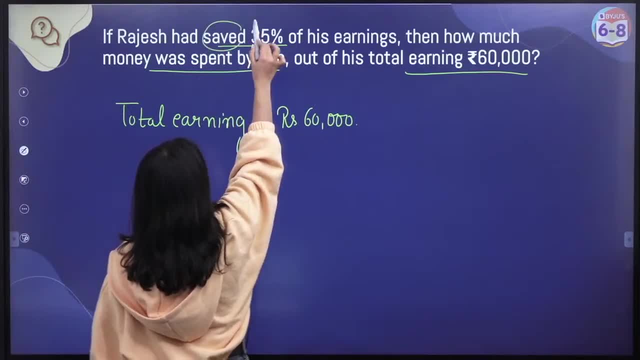 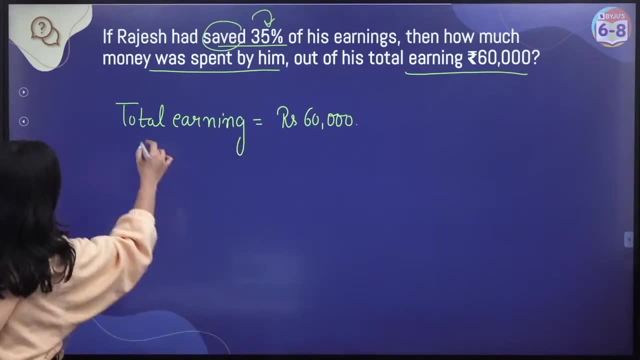 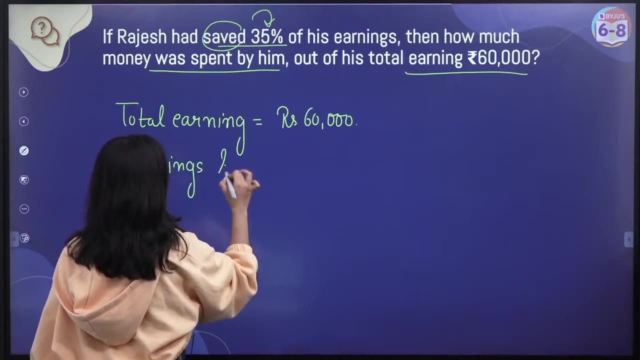 these 60,000 rupees, Rajesh is saving 35% of his earnings. He is saving 35% of his earnings. So how much will be the saving? You can write earnings saved or you can also write savings This Earnings saved. 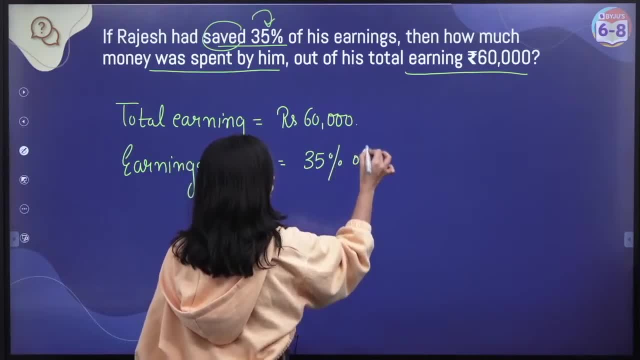 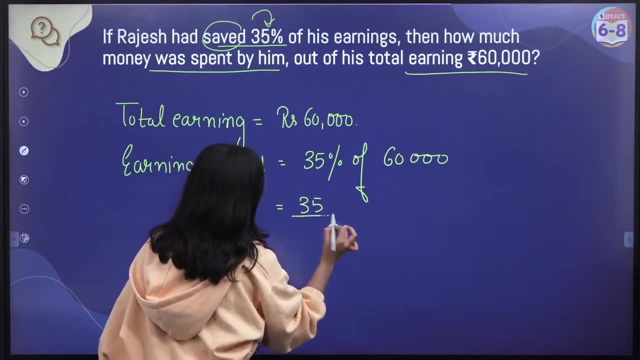 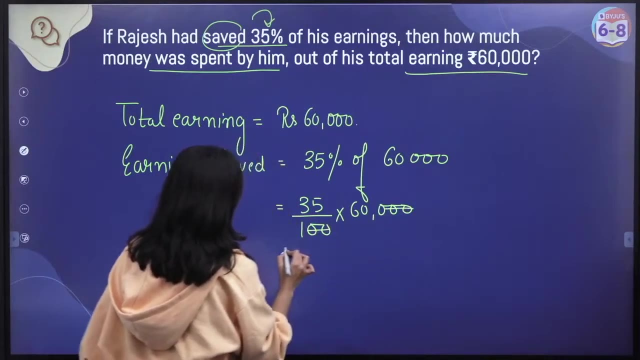 How much will be the saving 35% of the salary he is earning, that is, 35% of the 60,000.. So how much is he saving? 35% means 35 by 100 into 60,000. So how much is he saving? 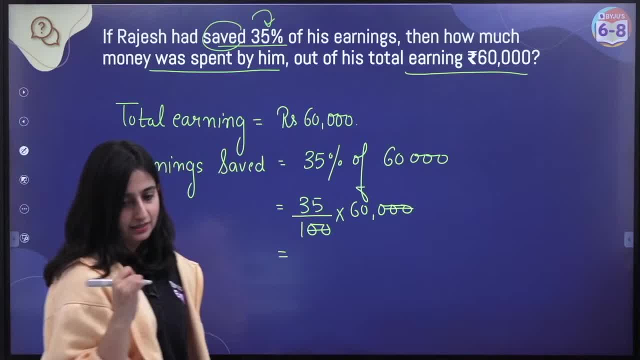 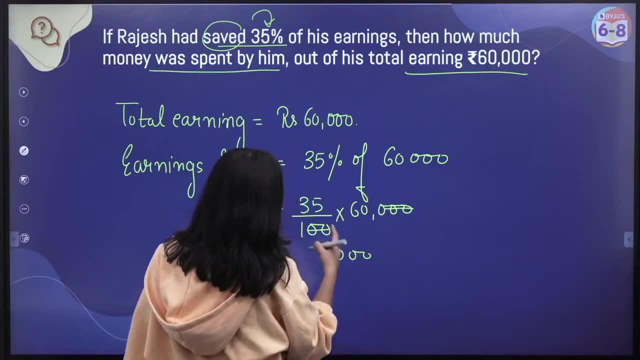 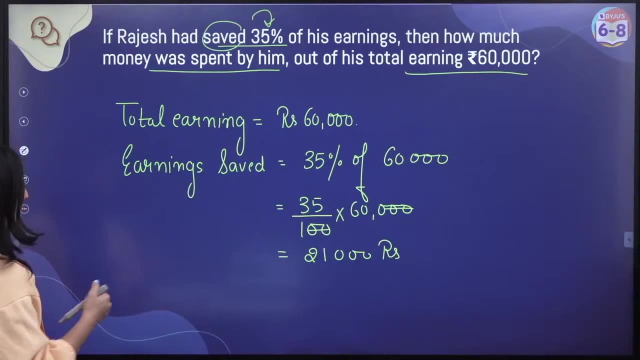 How much is he saving? Tell me quickly. How much is he saving? Yes, So he is saving 21,000.. So 21,000 he is saving. So if he is saving 25,000, these are his savings. This is how much he earns. 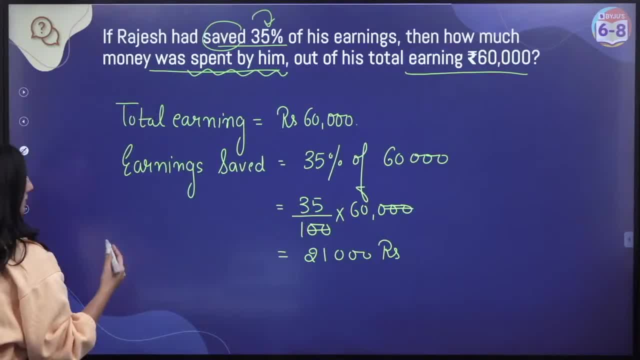 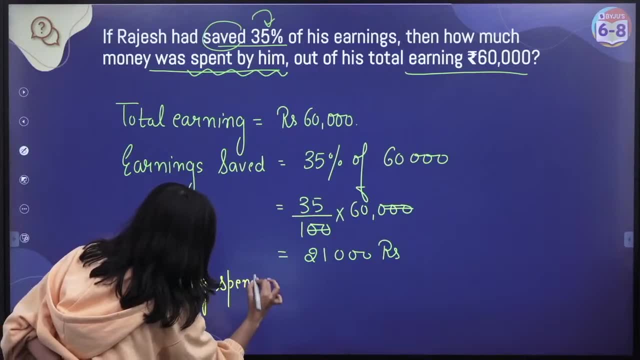 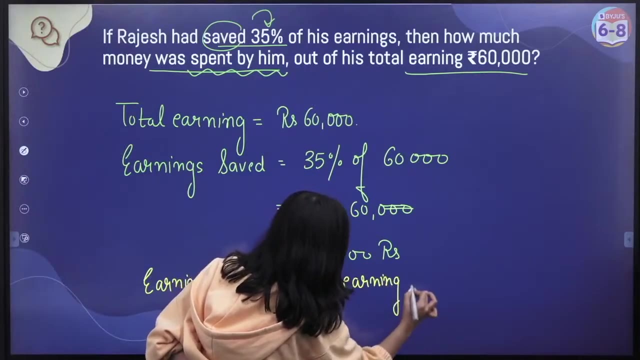 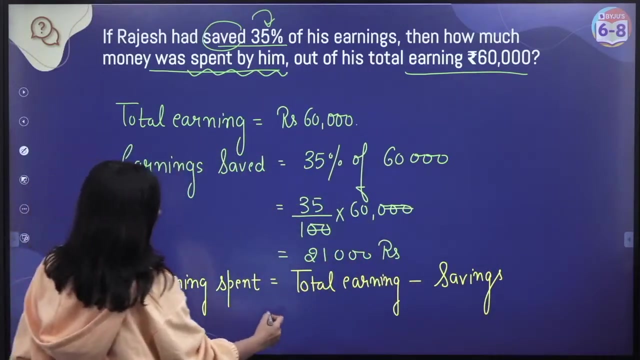 So how much is he spending? How much will be the expenditure? So earnings spent, So earnings spent will be. How much will he spend? Total earnings: total earnings. total earnings minus savings: total savings. Okay, So how much is the total earning? 60,000. 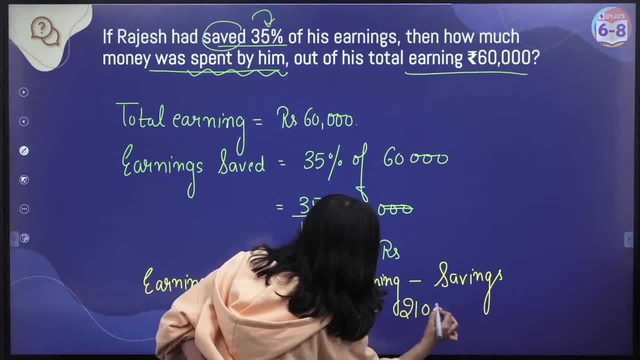 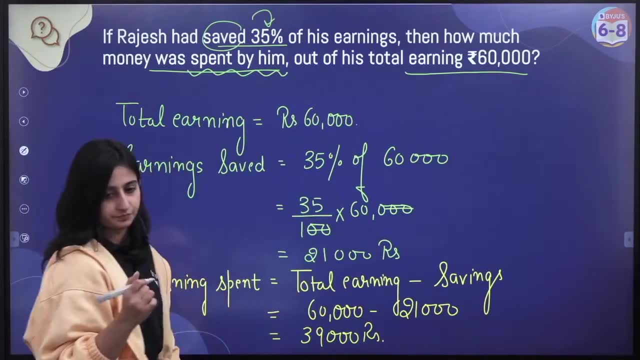 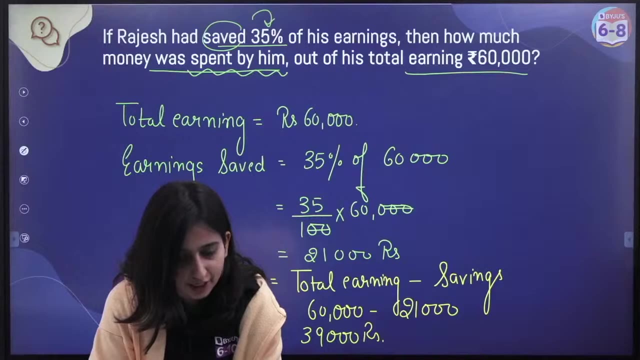 You just have to subtract the savings from this amount he is earning, So you will get 39,000 rupees. Is it clear? Very easy, Yes, Did everyone understand? Yes, Very good, Very good, Very good, Okay. 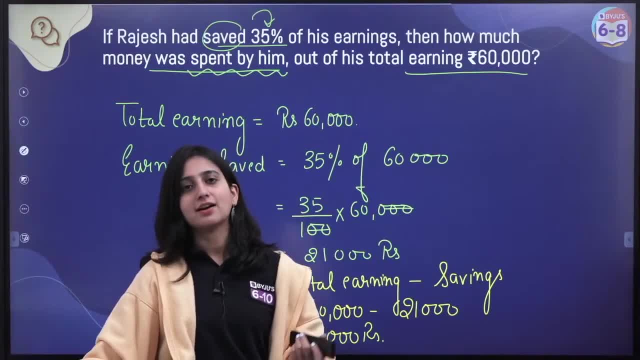 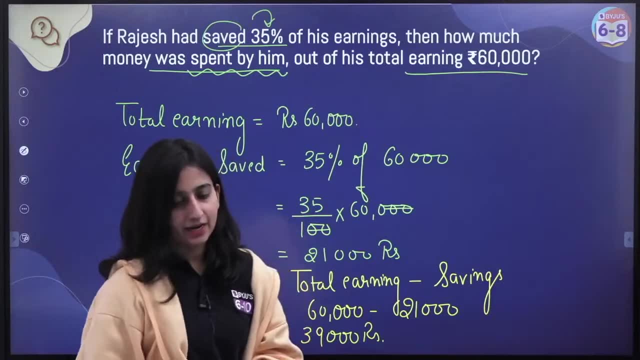 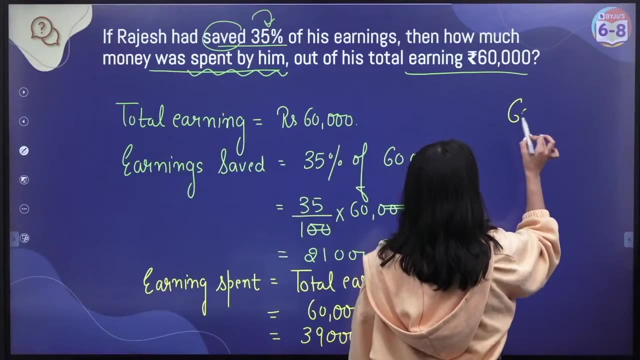 Aditi, we don't remember, so you have to check the schedule. You just have to check the schedule, Right? Yes, I will explain one more time. So in this question you are getting the salary 60,000.. You are getting 60,000 salary. 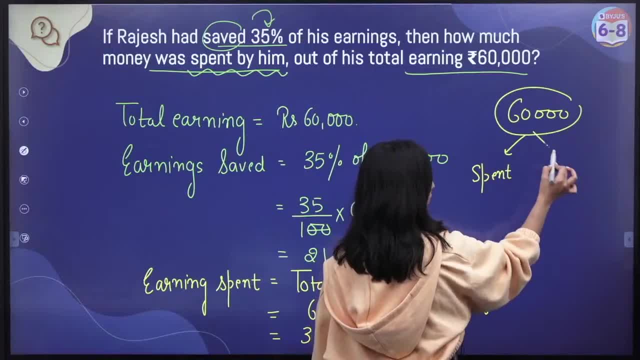 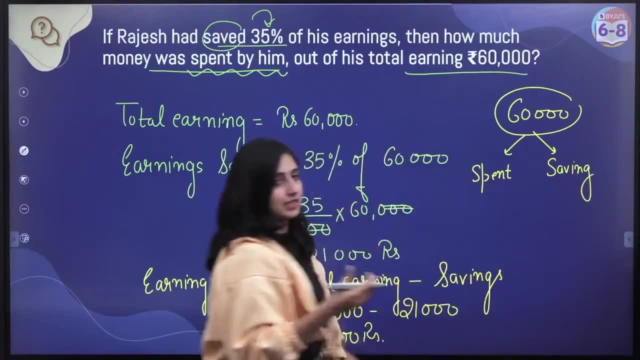 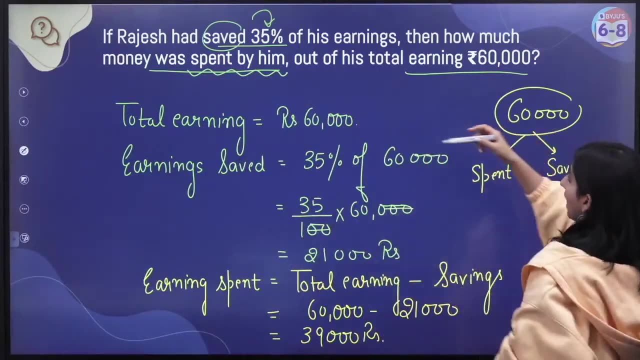 Now, in this 60,000, you must have spent something. You have some expenses, You are spending something and there must be some amount that you are saving also. You must be saving something and spending something. So in this question it is said that he is earning 60,000. 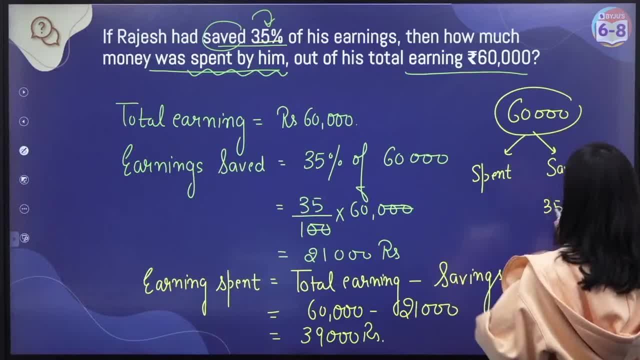 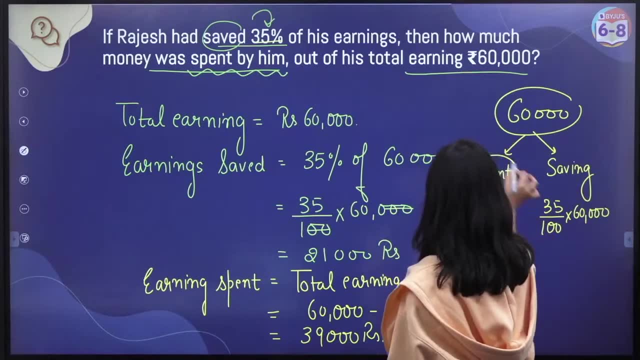 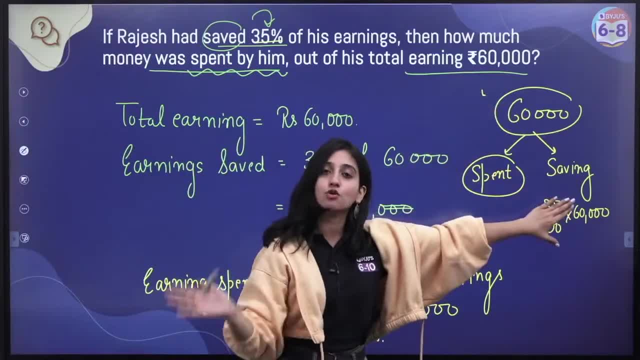 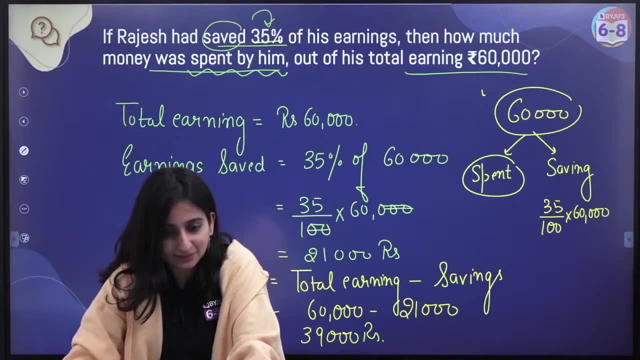 So how will we get it? If you subtract the savings from the total earnings, then you will get the expenditure of this man. then you will get the expenditure of this man, Right, Is it clear? No, children, Harshit. there is nothing like this. 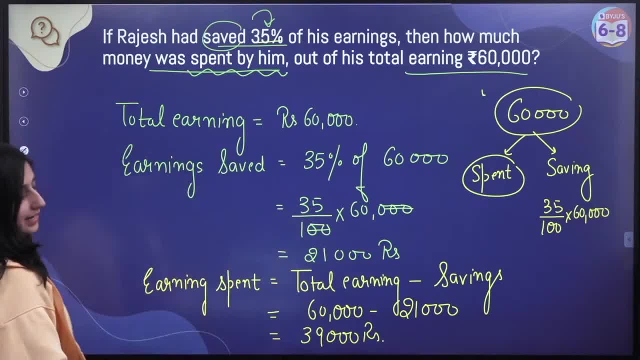 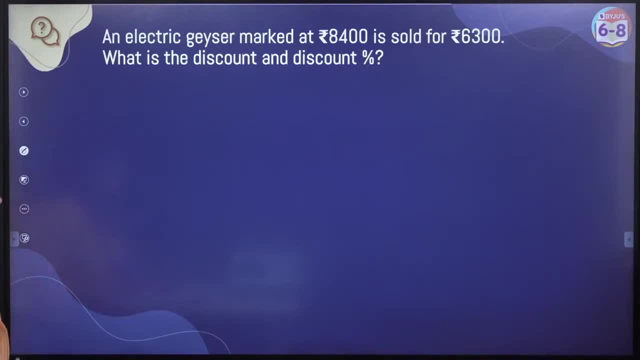 I am not ignoring anyone. Don't say like that. Let's move on to the next question. An electric geyser marked at 8400. An electric geyser marked at 8400 is sold for 6300 rupees. is sold for 6300 rupees. 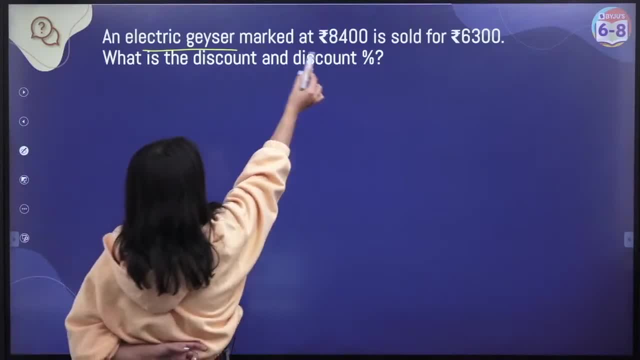 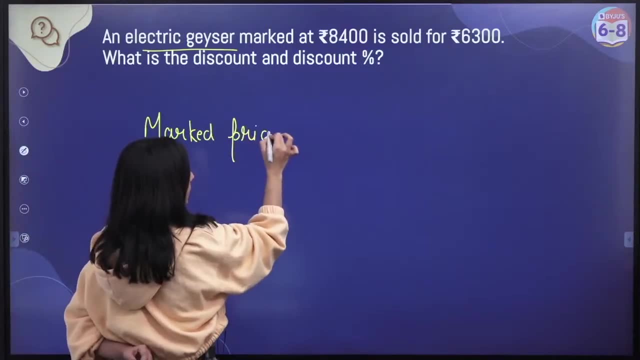 Okay, so we have an electric geyser with us. Okay, so we have an electric geyser with us. What is its marked price? So, marked price. What is the marked price? The price that is written, The marked price, of the geyser, is given as: 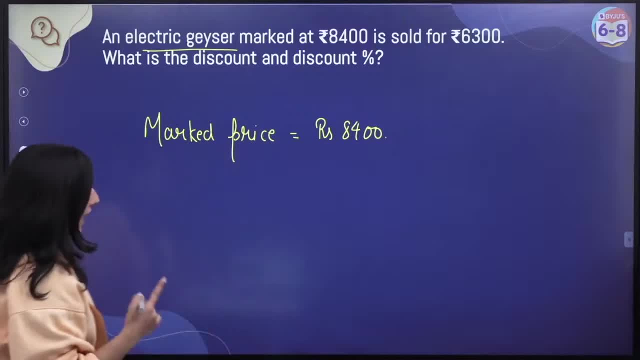 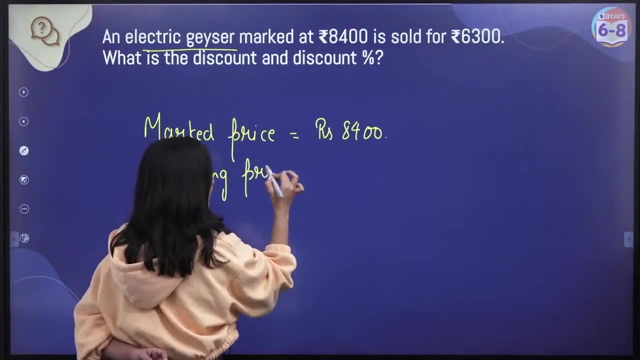 Rs 8400.. Rs 8400.. And it is sold for 6300.. Now, what is the selling price? The selling price means the amount at which it has been sold. The amount at which it has been sold, So selling price is. 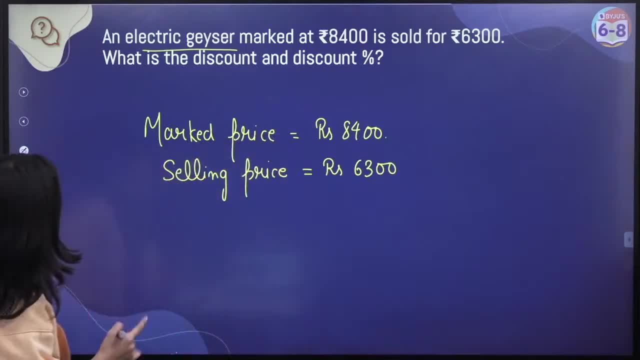 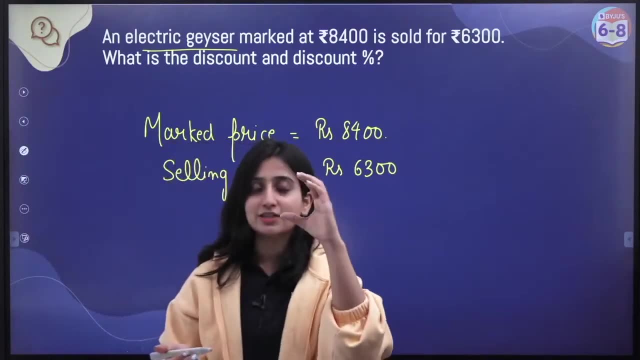 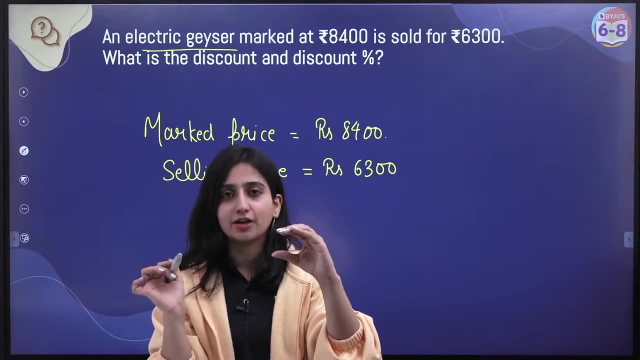 Rs 6300.. Right, What is the discount and discount percentage? Now you tell me You go for shopping. If you see the tag, then what is the original amount written on that tag, Suppose 8400.. And then what is written by cutting it down? 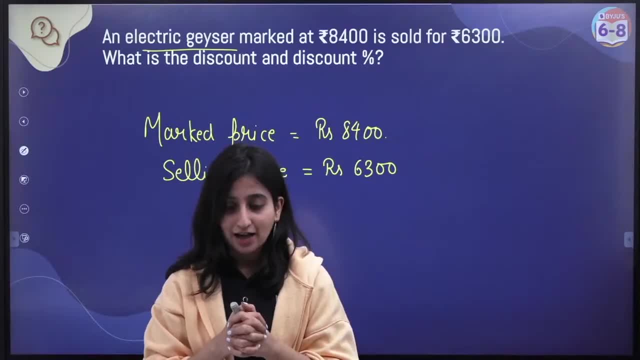 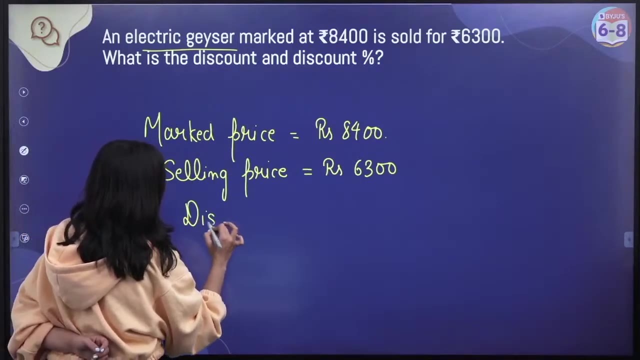 6300.. What is the discount? How much discount are you getting? Quickly tell me How much discount are you getting. Yes, Okay, Very good, Sneha. So how will we get the discount? Discount will be equal to. Discount will be equal to. 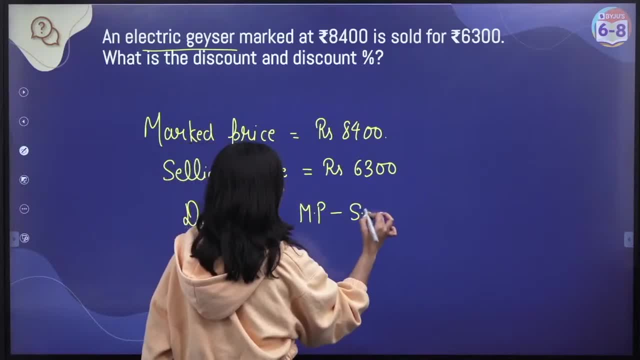 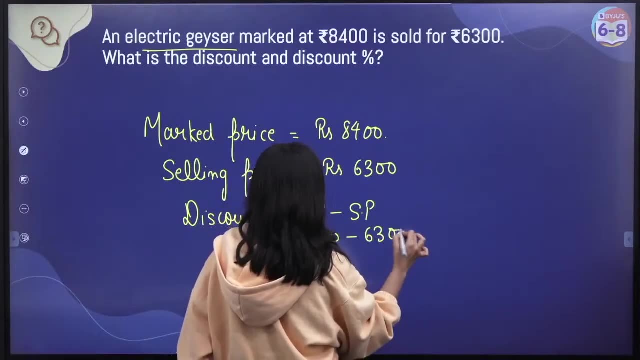 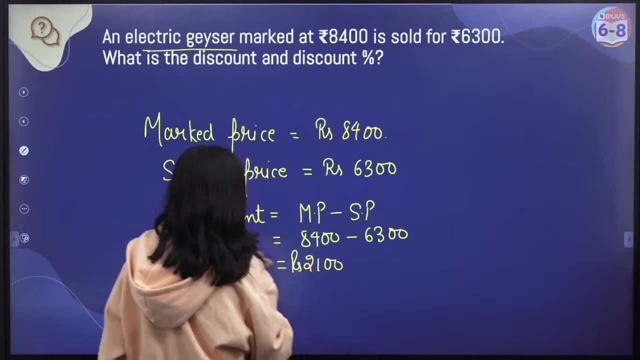 Marked price, which was our marked price minus selling price. What is the price? 8400 minus 6300, minus 6300.. How much is it coming? Tell me quickly. It is coming out to be 2100 rupees, Yes or no? 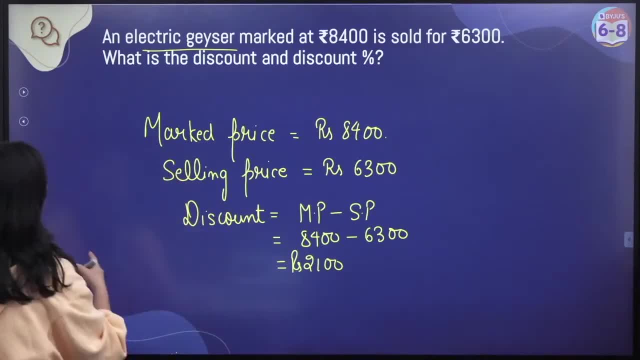 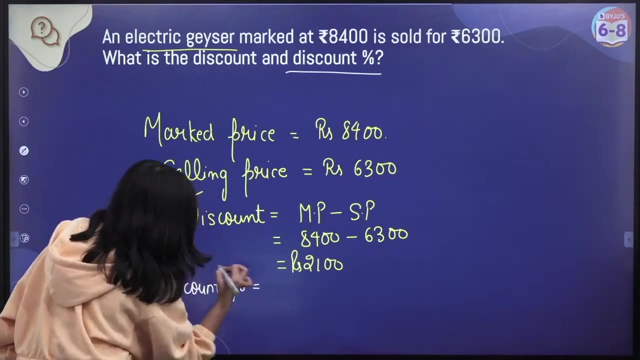 2100 rupees is coming. Yes, Okay, Now you have taken out the discount. One more thing you have to find: You also have to calculate the discount percentage. How will you calculate discount percentage? Discount percent will be equal to discount. How much discount is there Divide? 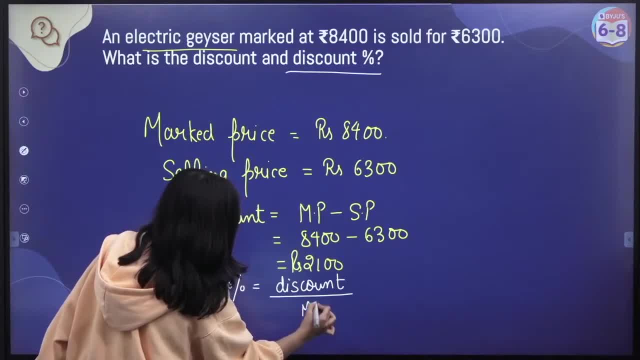 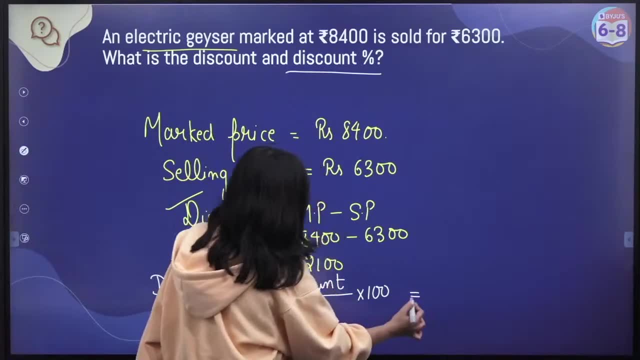 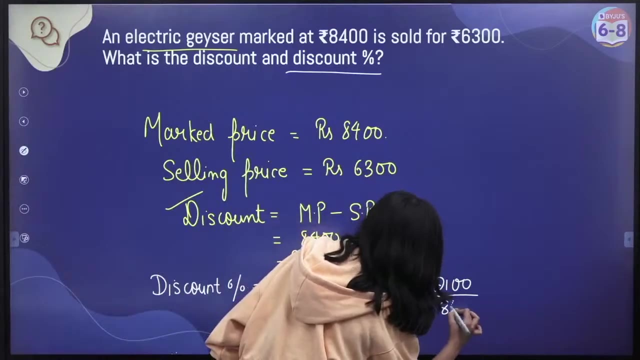 by how much was the mark price? How much was the original price Multiply by 100.. So what is coming? Who is it coming equal to? It is coming out to be 2100 divided by mark price. how much is it? 8400.. 8400 rupees. 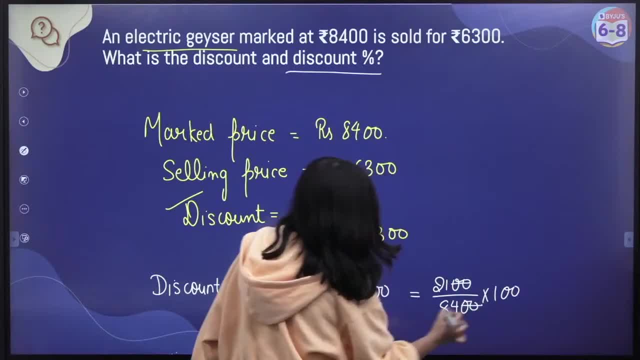 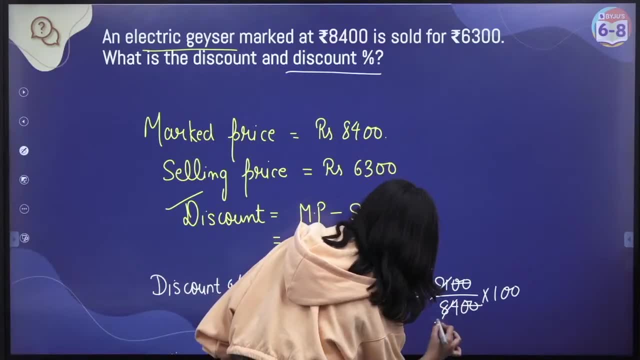 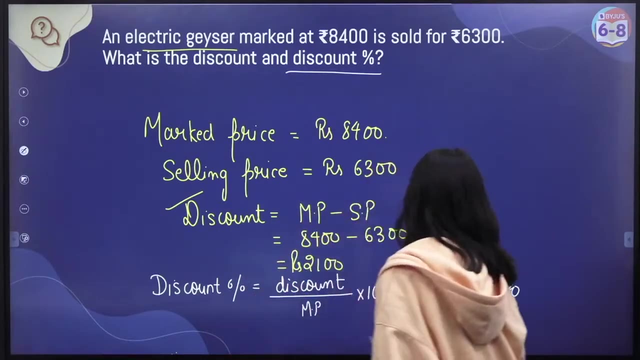 8400 multiplied by 100.. So how much is coming? Tell me the answer quickly, Quickly tell me the answer: 425.. Yes, So the answer is coming out to be 25%, Isn't it? You also got 25%. 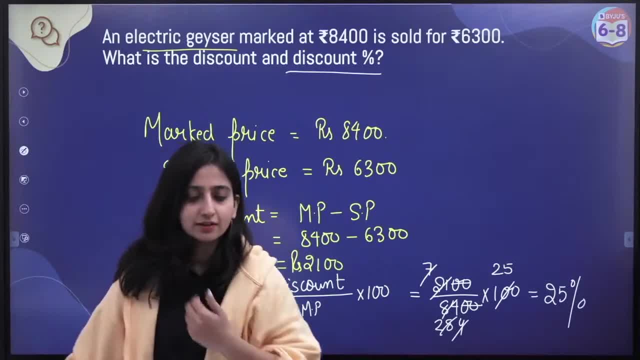 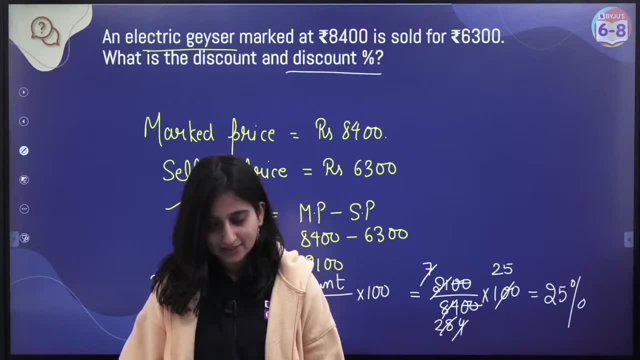 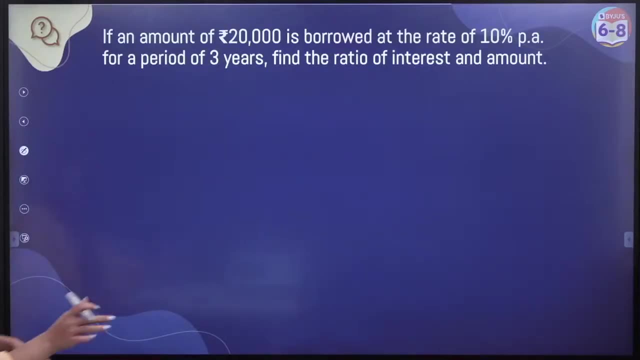 Yes, Very good. Very good, Devik, Very good, Miss Unique, Anu, Chimmy Nitin. Yes, So the right answer is 25%. Very good, Okay, Now you have a simple interest question. Now we are having here simple interest question. Come on, Let's see. 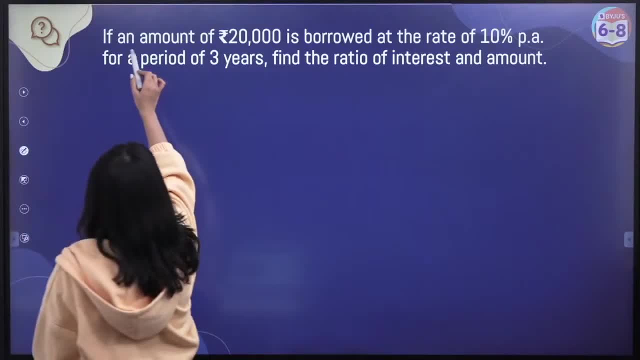 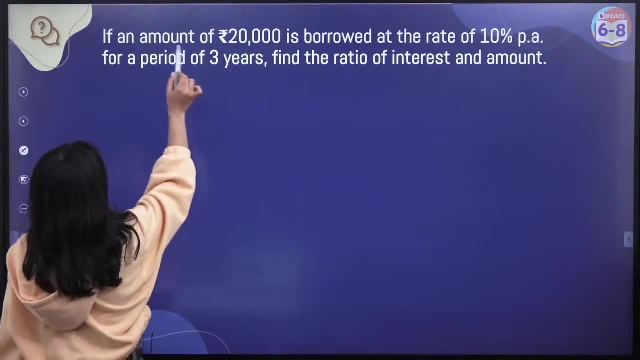 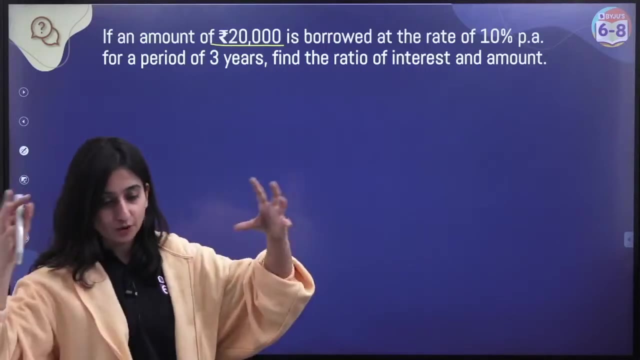 how to calculate If an amount of 20000 is borrowed. See what will some children do After reading the amount: they will feel that this is the amount, So they will calculate the amount given to us. But no, Try to read the entire sentence. Let's try to read the. 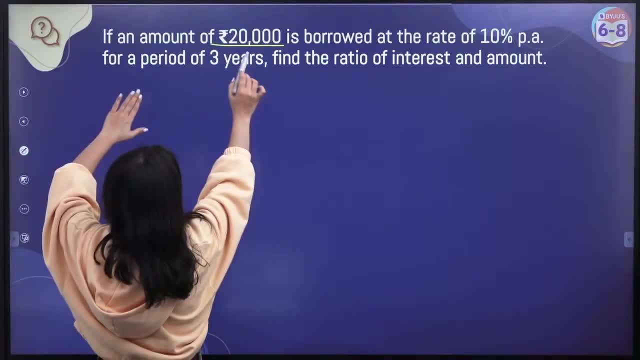 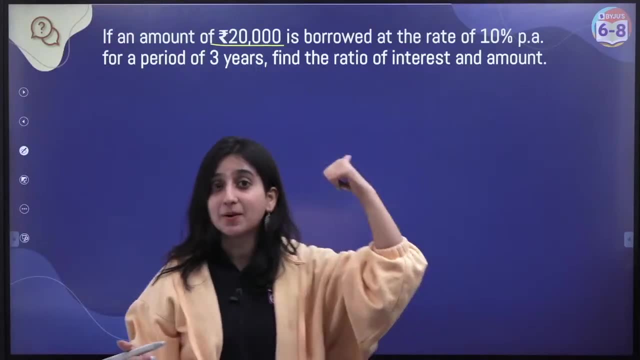 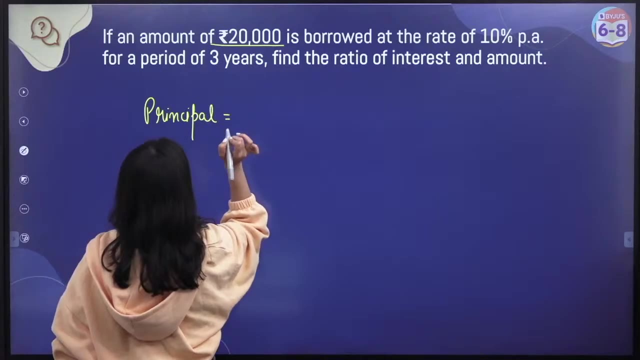 entire sentence. Good evening Purnima. Amount of 20000 is borrowed. If I am borrowing this much amount, That means this is my principal. What will become of my principal? So, according to this question, principal is given as how much. How much principal you have given you? 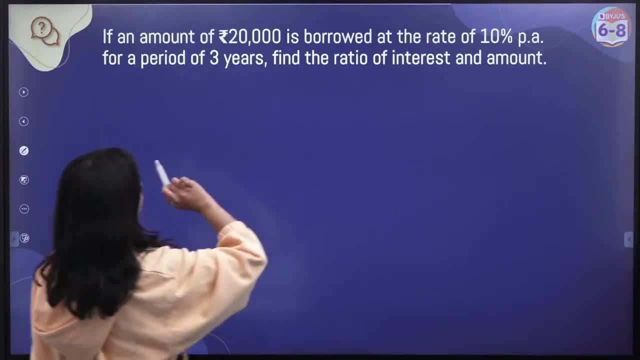 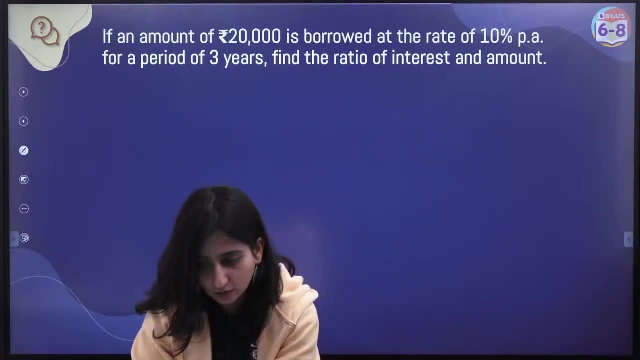 Yes, children. How much principal amount you have given? How much principal amount you have? 20,000, yes or no? so principal a chukka aapke paas 20,000. rate is given as 10%. R aapke paas 10% de rakha hai. period time period is given as 3 years. 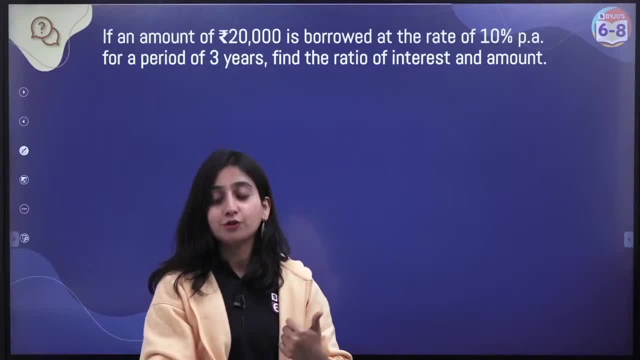 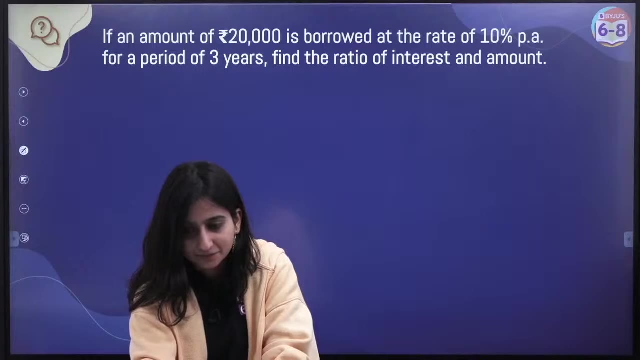 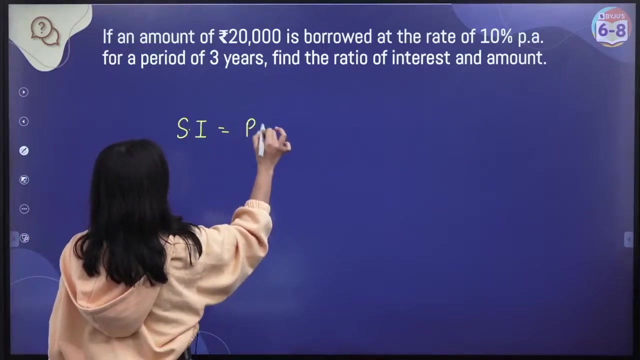 to t aapke paas 3 ho jayega and you have to find the ratio of the interest and amount. chalo aap jaldi se mujhe batao yes, kya answer aayega? iska, we know that. we know that simple interest is equal to PRT by 100. 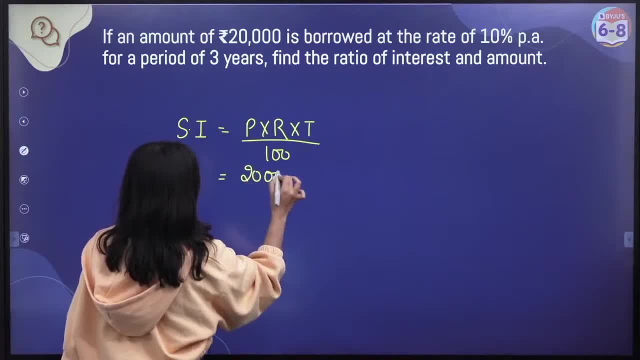 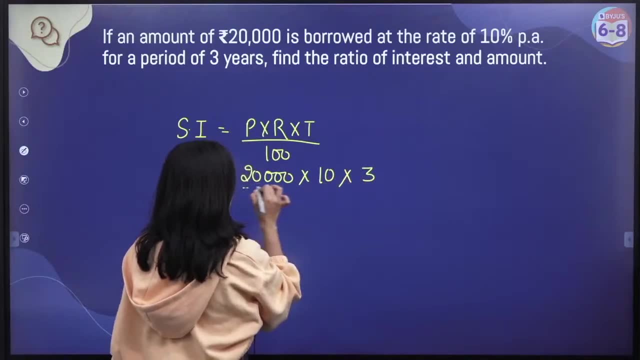 so the principal is given to us as 20,000 rate is given as 10%. time is given as 20,000 time is given as 20,000 rate is given as 10%. three years divided by 100, so simple interest: kitna ban raha aapke paas. 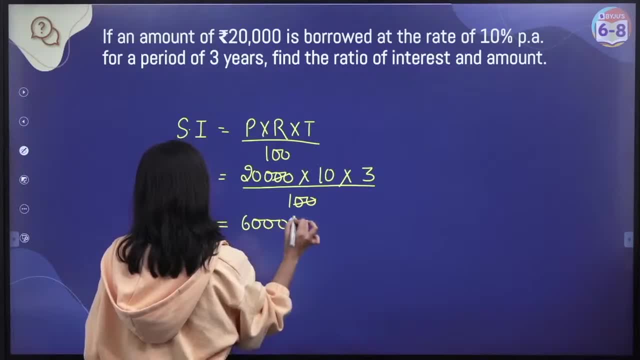 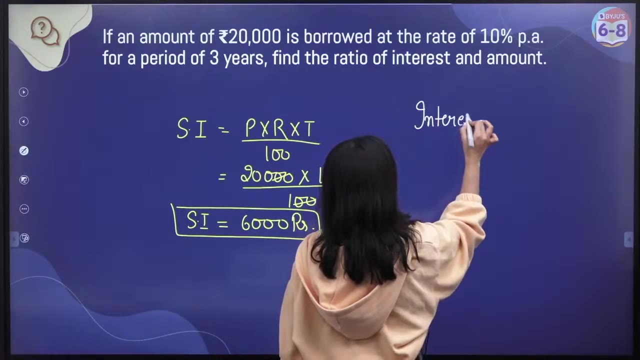 simple interest: ban raha hamara 6,000 rupees. yes, ye, hamara ban chukka hai. simple interest, right? this is my simple interest. aapko nikalna kya hai? find the ratio of the interest and amount? aapko nikalna kya hai? you have to find the ratio of the interest and amount. 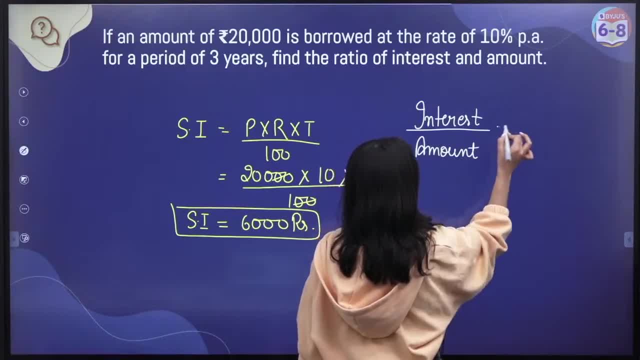 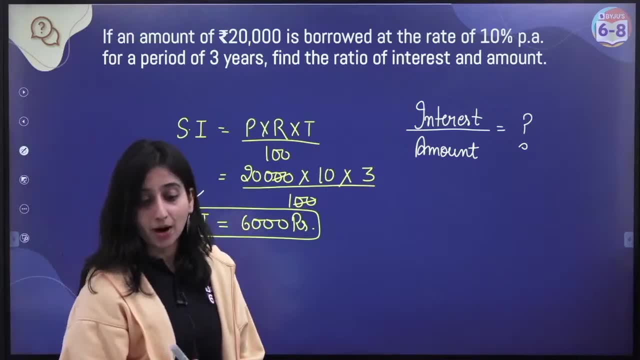 aapko interest or amount ka ratio nikalna hai, matlab aapko ye wali value nikalni hai, so iske liye interest aa chukka hai hamare paas now. the second thing that we have to calculate here is amount. 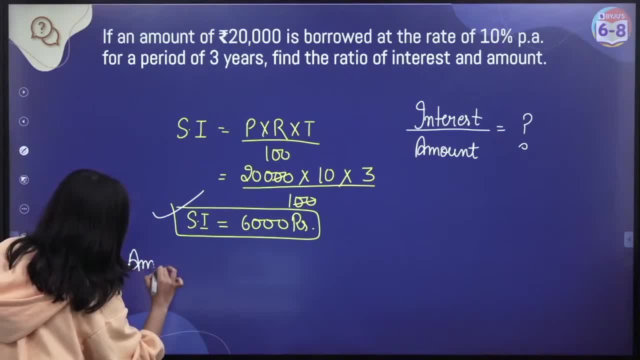 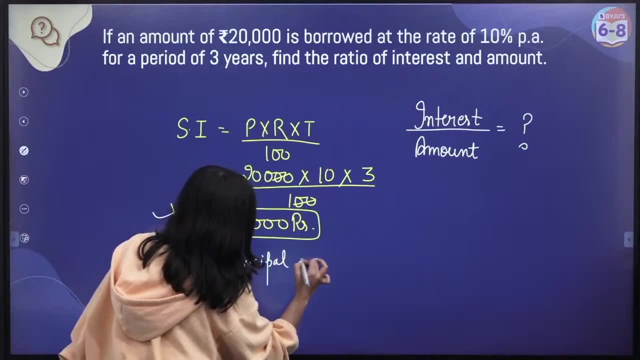 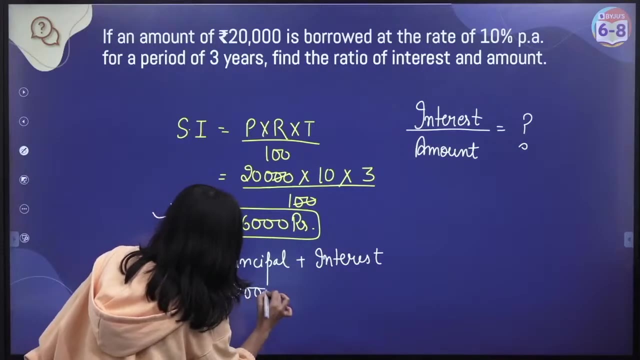 to amount kiske barabar hota hai amount aapko kya sikhaaya tha. amount hota hai principal plus interest. amount hota hai principal plus interest. ok to, jab aap in dono ko add kar doge, that is 20,000 plus 6,000. 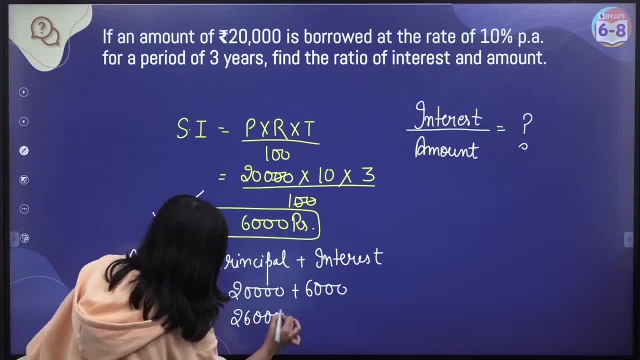 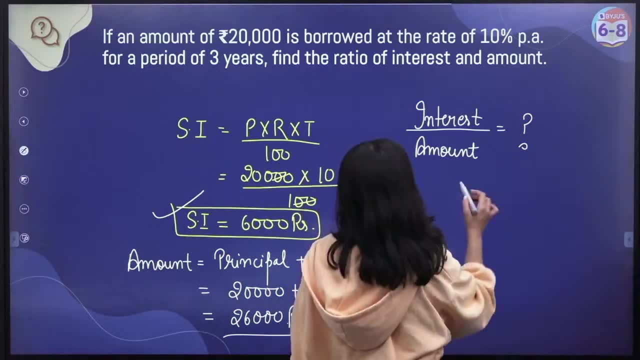 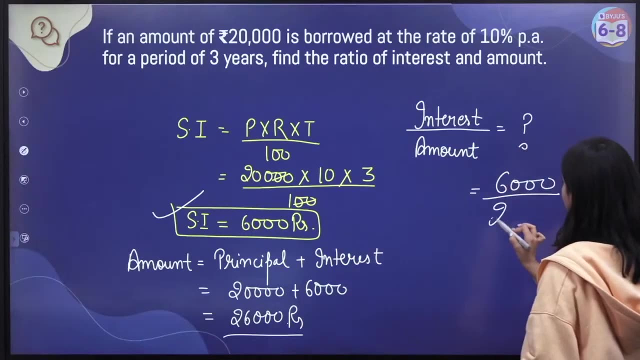 you will get 26,000. yes, to ye aapka amount ban gaya to ratio kiske barabar ho jayega ratio will be equal to interest, interest, which is 6,000, and amount that is 26,000 to aapke paas. kya ban gaya. 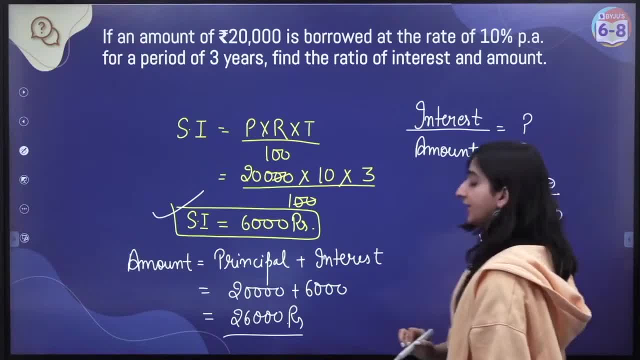 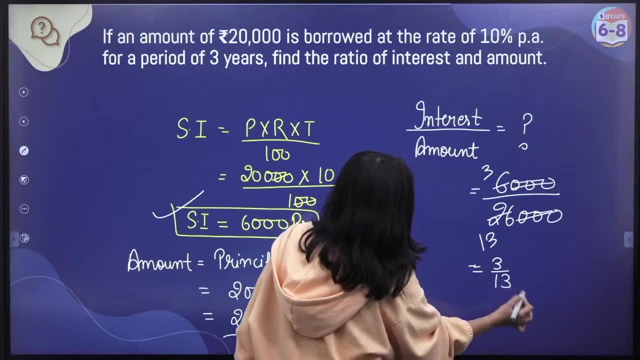 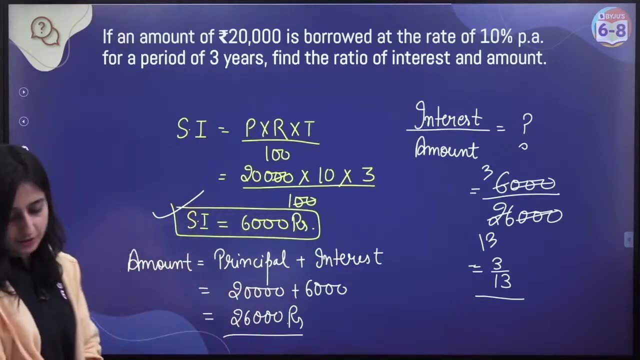 3 is to 13. ratio aa gaya sabka. 3 is to 13, so ratio is coming out to be 3 is to 13. is it clear? yes, menti bhi hoga. bache menti. we will start at 6 pm. 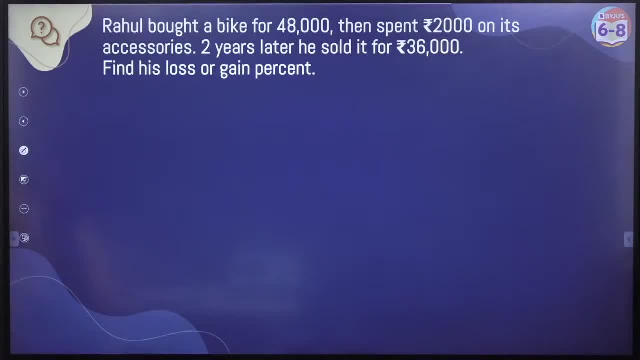 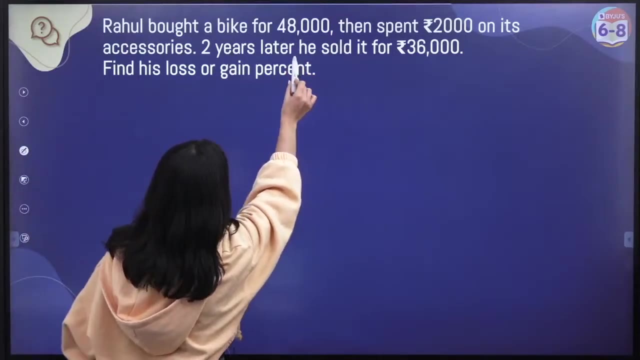 chalo. next question: dekhte hai, Rahul bought a bike for 48,000 rupees and then spent 2,000 on its accessories. acha Rahul ne bike kharida for this much amount? bike ka cost kitna hai 48,000. 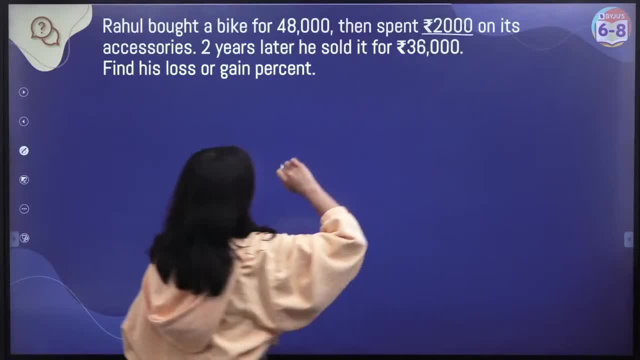 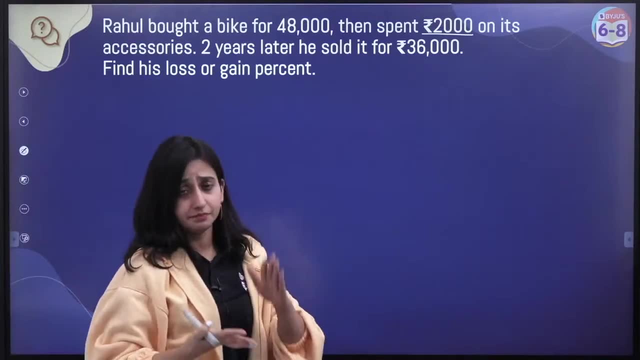 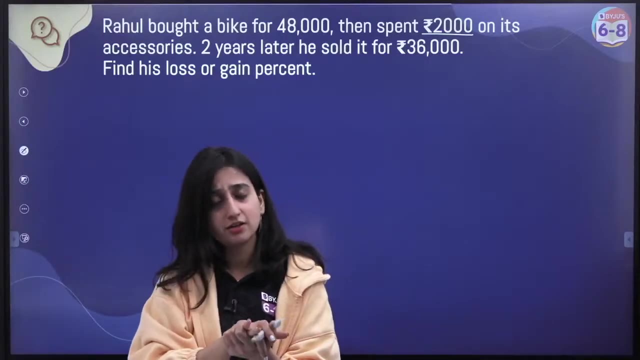 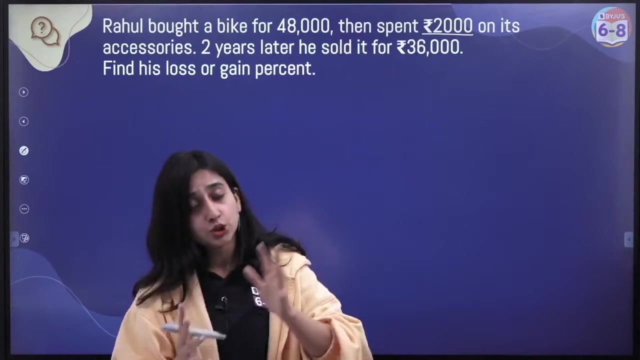 aur usne accessories me kitna spend kar diya 2,000 kiske barabar hota hai 48,000 rs thousand. he put more accessories on it. So how much total bike did he get? Now you tell me you have gone to buy a bike. a bike of 48,000 came and you put accessories on it to decorate it, or you put additional accessories on it, so he got 2,000 more. So actually how much bike did he get? He got a bike of 50,000, right, How much did he pay him? 50,000 to get that bike? right Now, 2 years later? now those 2 years later he wants to sell the bike. Now he sold it for 36,000 rupees. Now you have to tell me: did he gain or did he lose? Yes, did he gain or did he lose? Come on, tell me quickly. Tell me quickly. yes, did he gain or did he lose? Come on, let's check now Here. if we take out the cost price, if we look at the cost price, then how much will the cost price be? 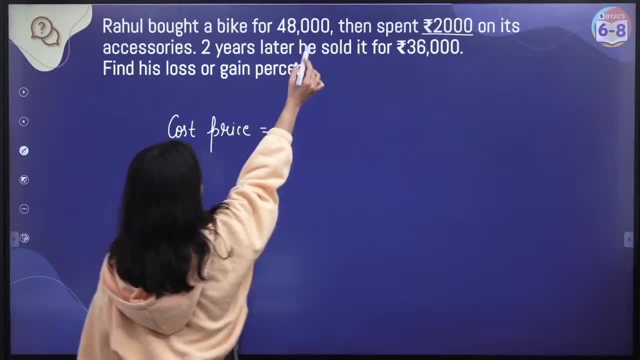 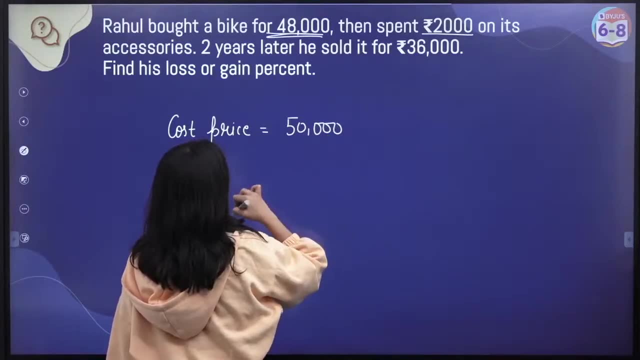 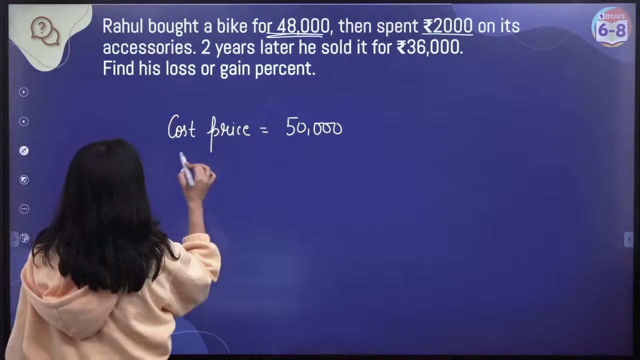 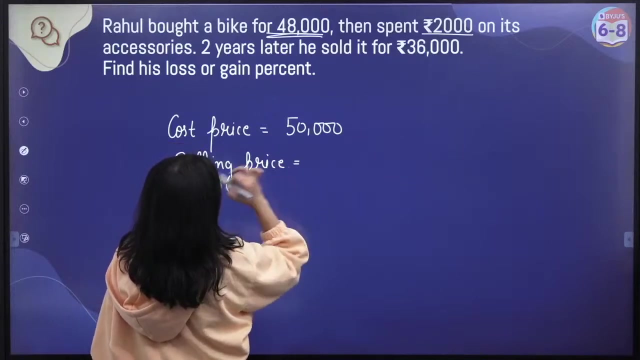 The cost price will come to us 48,000, as much as he bought the bike plus the accessory amount. So the cost price here is 50,000 rupees. How I told you, 48,000 plus 2,000.. Right Now selling price: how much is he selling the bike? How much is the selling price with us Selling price in this statement problem is 36,000.. He is selling in 36,000.. 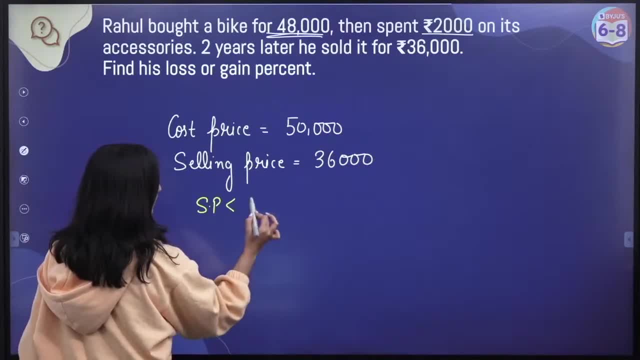 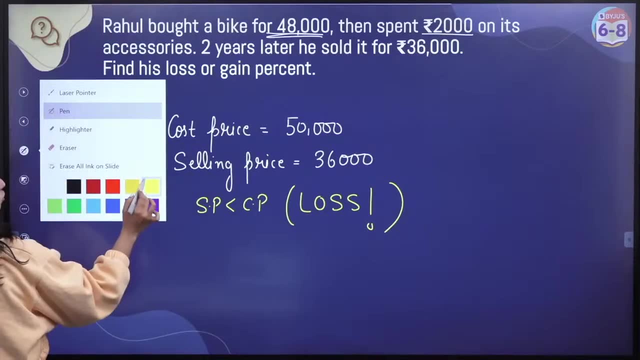 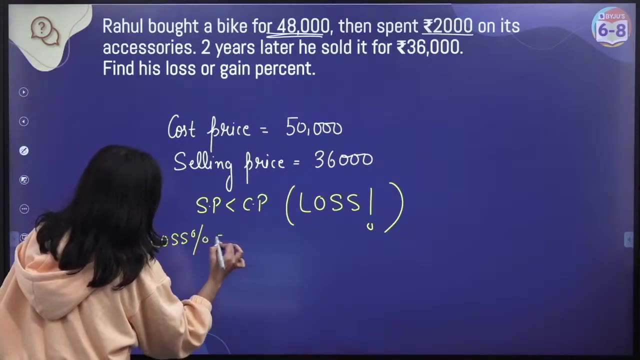 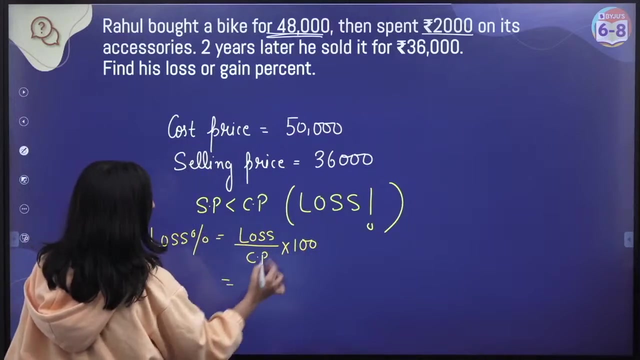 Selling price. we have reduced Selling price is less than cost price. That means we are having loss. We have lost here. Okay, So come on. now we have to find the loss percentage. Let's find the loss percentage. Now, loss percentage, what is it equal to? It is equal to loss upon cost price into 100. Right, How much loss? How will loss come? Selling cost price minus selling price. So cost price is less than cost price. 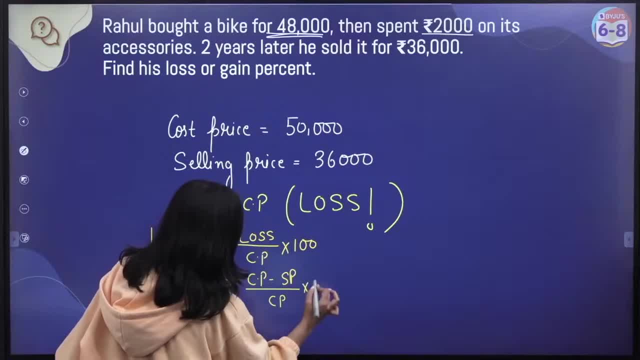 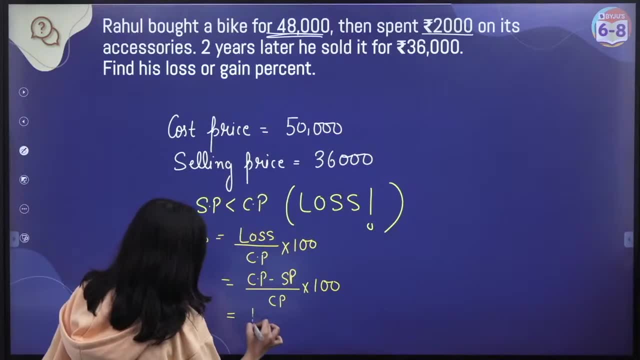 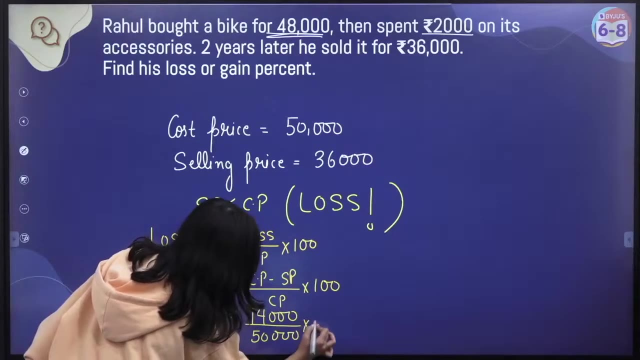 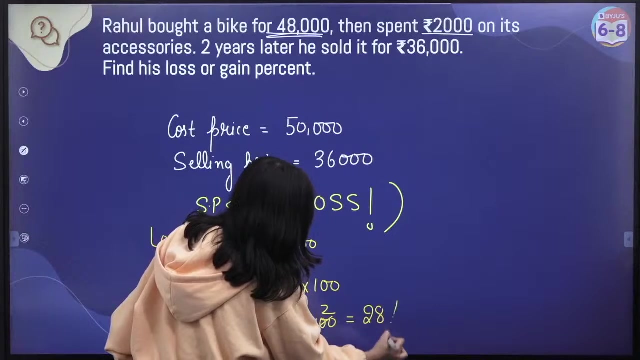 Selling price minus selling price, divided by cost price, into 100.. Come on, calculate Cost price minus selling price. How much is it coming? Tell me 14,000.. So it became 14,000 divided by cost price. How much was it? 50,000 multiplied by 100.. So what came? What answer did you make? Answer is coming out to be 28%. That means he had a loss of 28%. 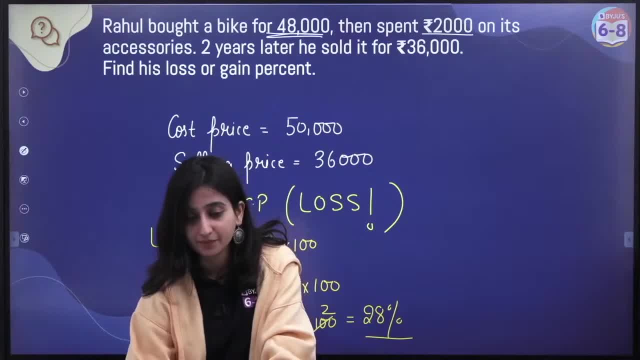 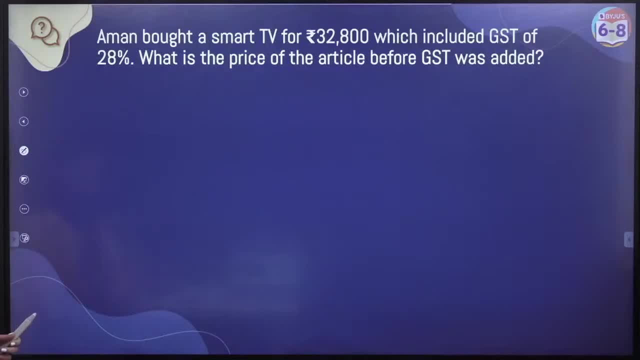 He had a loss of 28% here. kids, Okay, Is it clear? Yes, Come on. very good Now, moving on to the next question: Very good question, Come on, let's see how many kids do this. I am giving you few seconds to understand, interpret the question and try to solve it yourself. Okay, Come on, let's see Here. the question says: Aman bought a smart TV for 32,000. 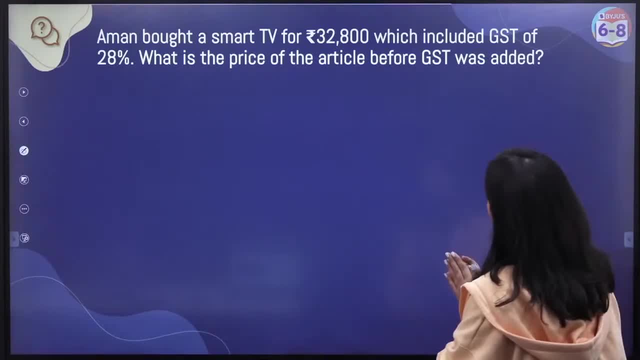 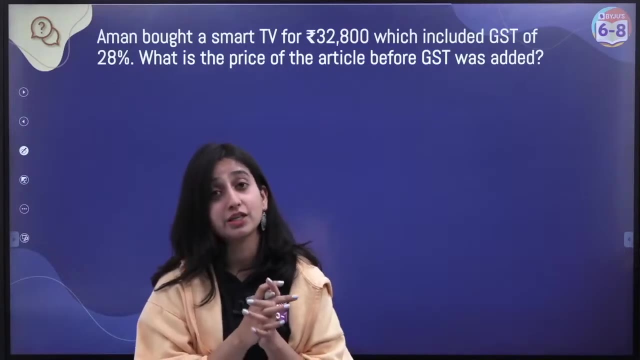 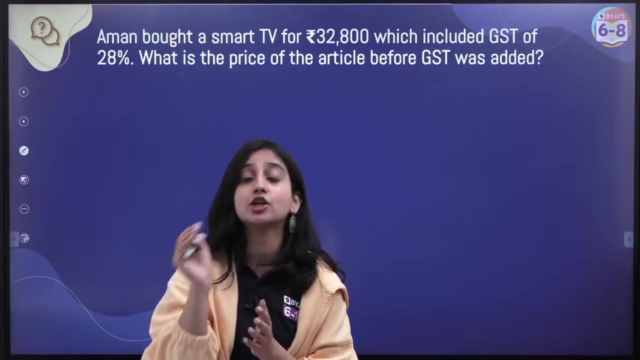 He bought a smart TV for 32,800 rupees, which included GST of 28%. What is the price of the article before GST was added? Now look, Aman went to buy a TV. He bought a TV for 32,800. And in this amount, GST means tax is included. This is inclusive of GST. Okay, You have to tell that without GST. Aman bought a smart TV for 32,800. 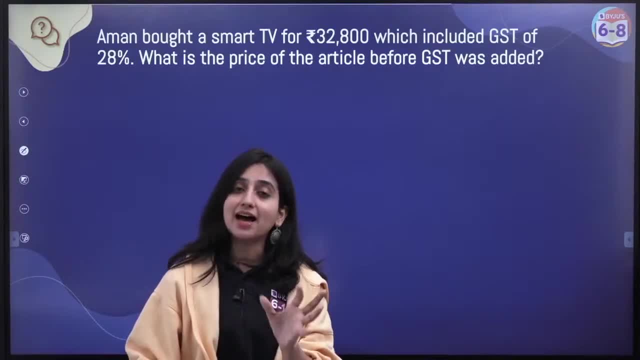 If I don't add GST, then what will be the price of this TV? What will be the price of this TV without adding the GST? Yes, How will we do this question? Any ideas You can give me in the chat? Yes, 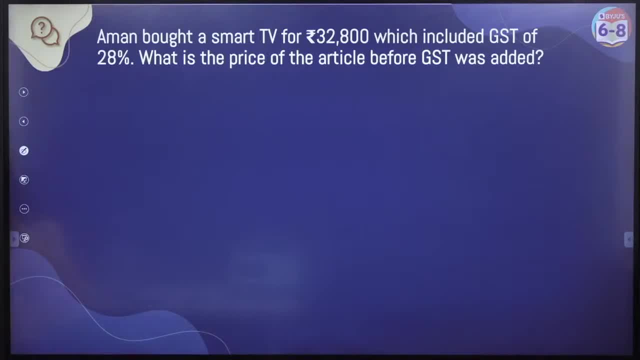 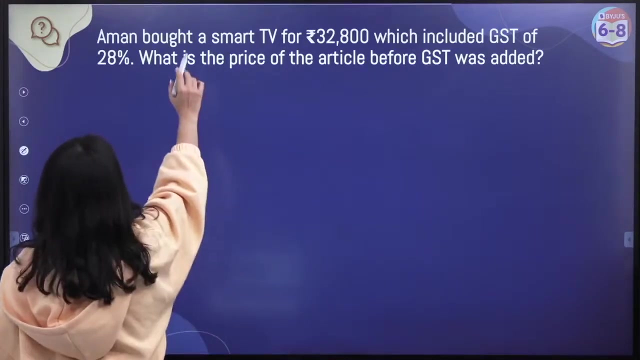 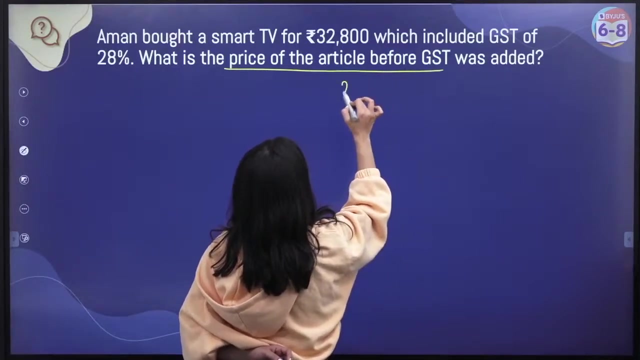 Can you give me the idea in the chat? Okay, Yes, So let's try to understand the problem. Let's try to understand the problem here. Come on, let's assume the price of the article before GST is X rupees. Let's assume What did I do? Let's assume 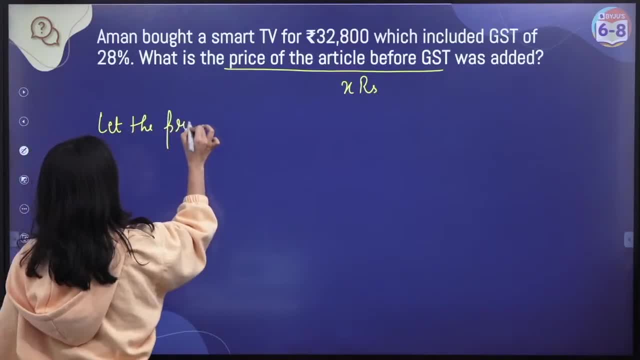 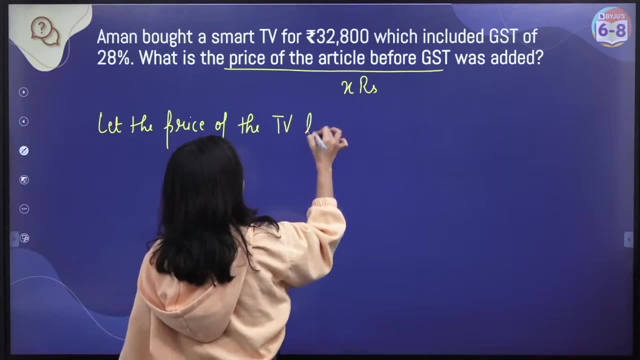 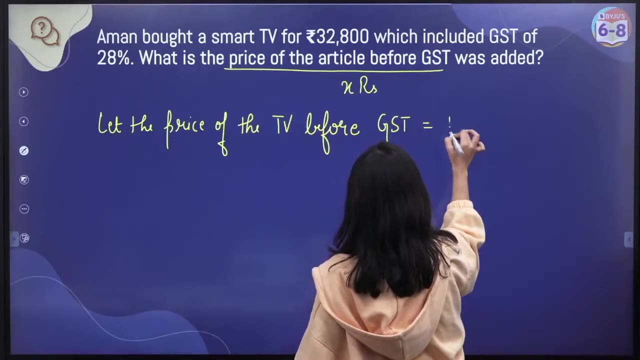 Let the price. Let the price of the article, Let the price of the TV. You can say before: Before GST was added. Or I have written like this: Before GST be rupees X. Let's assume that this is actually a TV without tax Added. Okay, 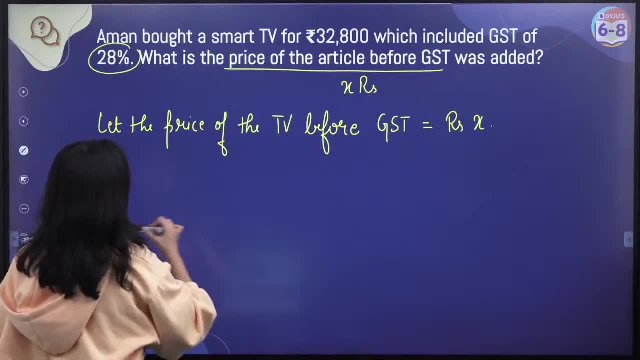 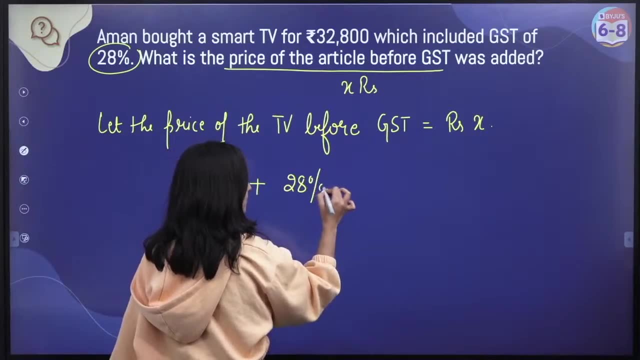 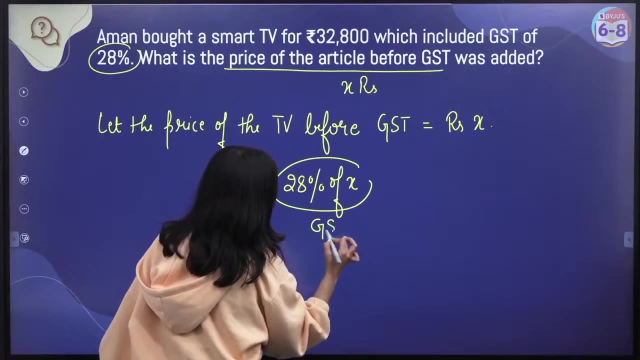 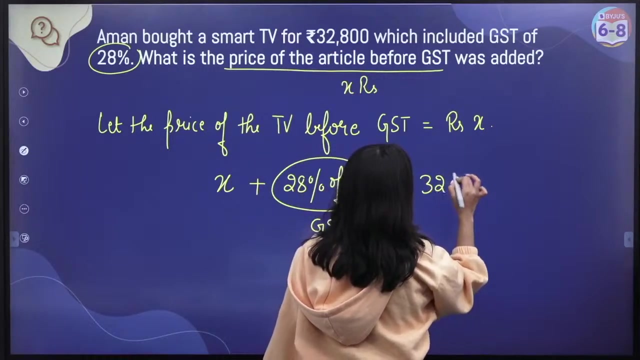 Now, how much tax are we applying on it? 28%, So the amount of TV is X rupees. On top of that, I have added 28% of tax. I have added tax. This is my GST. This is my GST. Okay, So how much total amount is being made by me which I have paid to the shopkeeper? That is, 32,800 rupees. 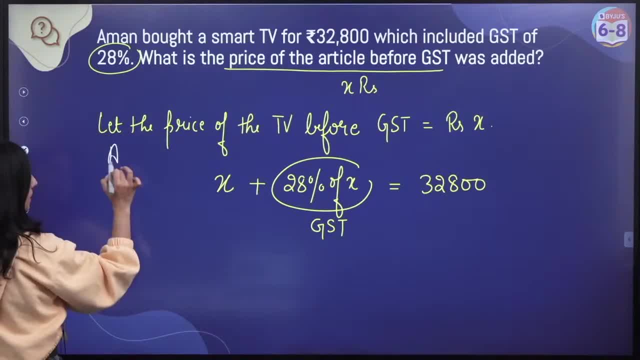 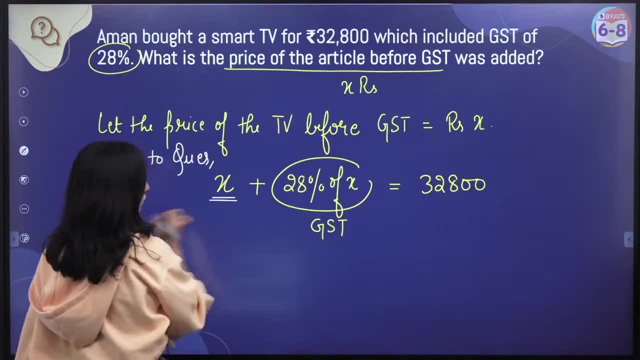 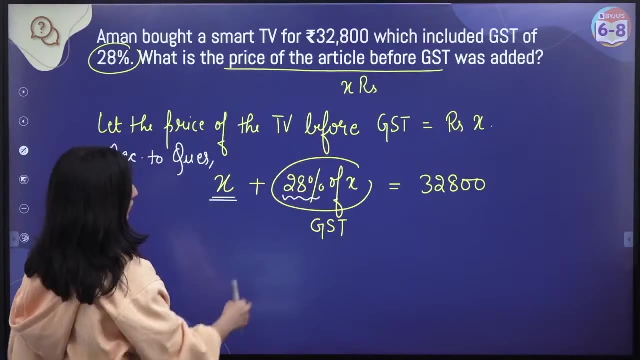 So did you understand the statement? What did I do So you can write here, According to the question, what has been given to you? Suppose this is the original cost of the TV. Okay, 28% tax is 28% tax. we are paying on this amount. So, 28% of this X we are paying as the tax. And how much total amount is being made? 32,800. 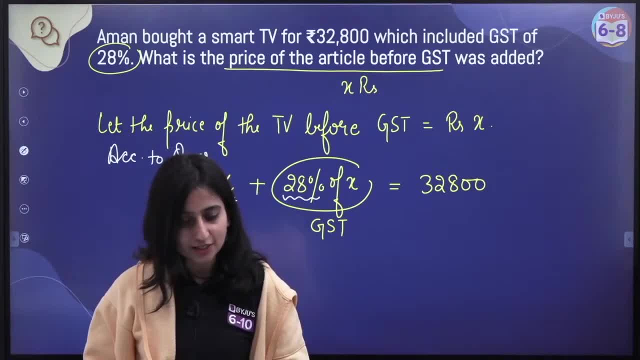 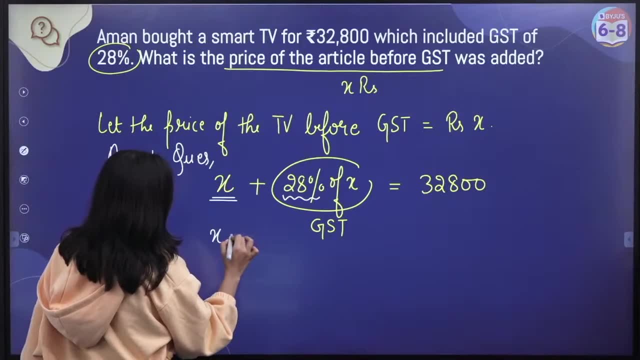 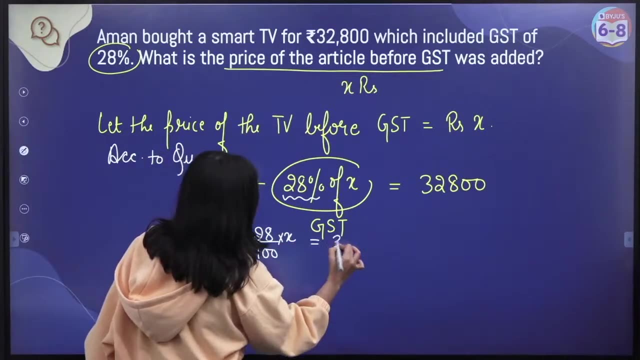 Did you understand this statement? Did you understand this statement? So here you have to calculate what is the value of this X. Let's go So this will be X plus 28% of X means 28 by 100 into X equals to 3.. 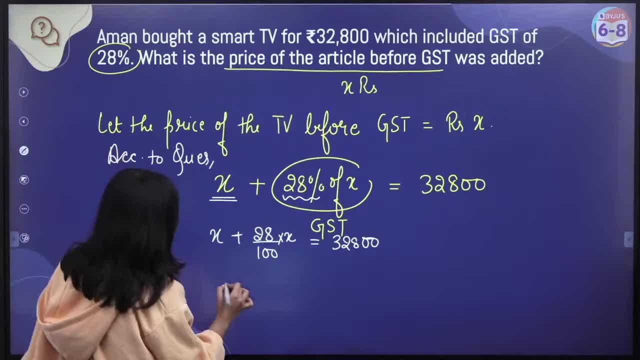 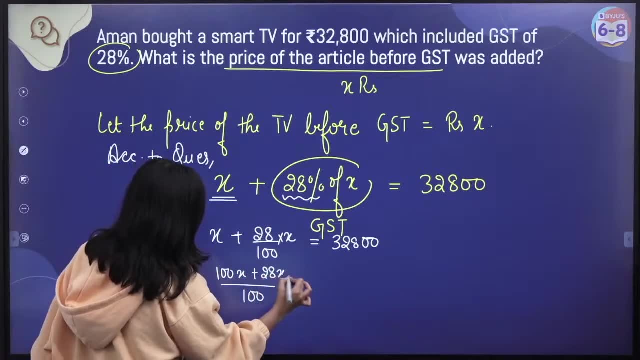 3, 2, 8, double 0.. Let's take this as LCM. When we took LCM here, 100 has come. It will be 100X plus 28X equals to 3, 2, 8, double 0. 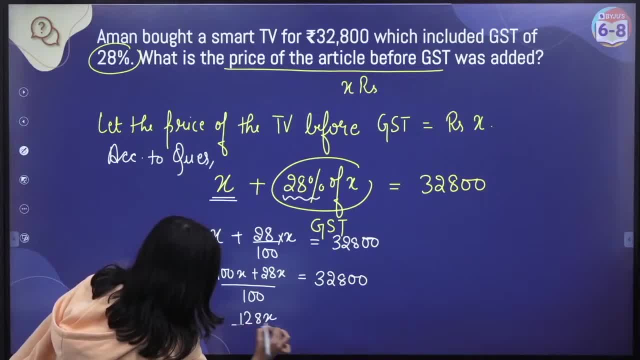 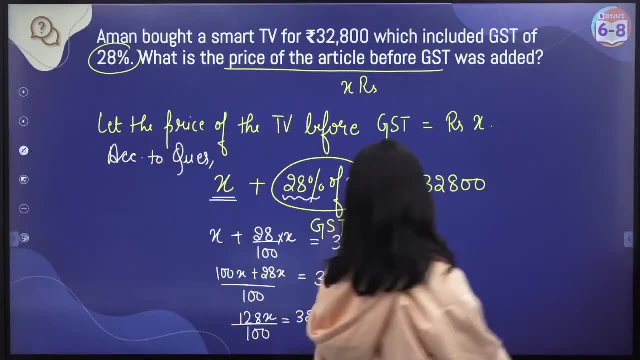 So this becomes 128X. 128X divided by 100 equals to 3,, 2,, 8, double 0. So from here we can calculate the value of X. So the value of X is coming out to be: 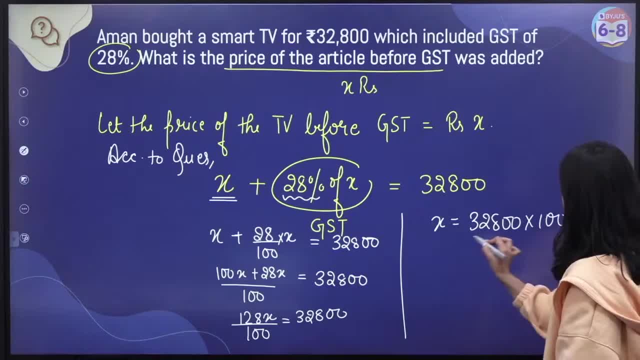 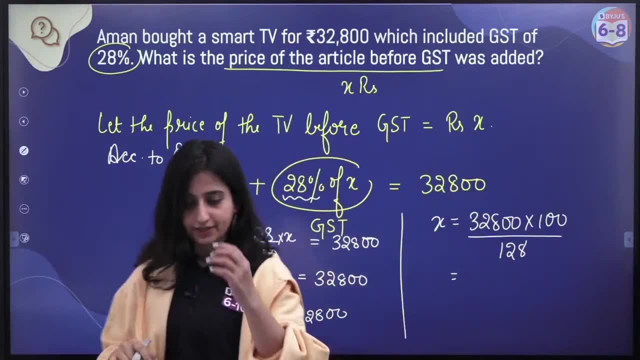 3,, 2,, 8, double 0 into 100, divide by 128.. Chalo, batao x ka value. kya aa raha hai? Yes, everyone, Quickly tell me what is the value of x coming here? 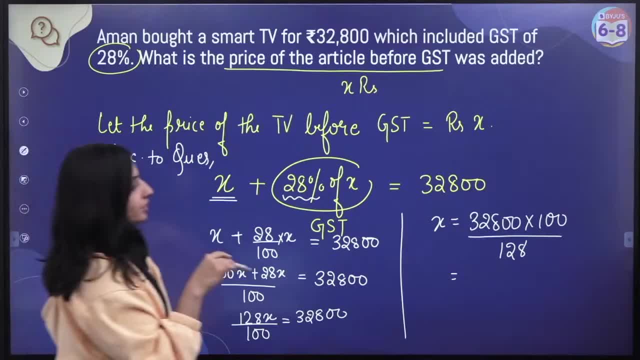 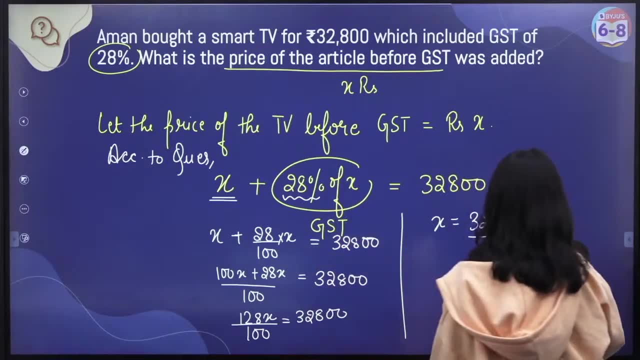 Jaldi se cancellation karo Solve this problem? Yes, quickly. 8 pe cancel kar do isko Ye ban gaya. 8 ones are 8,, 8 sixes are 48.. 8 fours are ye ban gaya 4100. 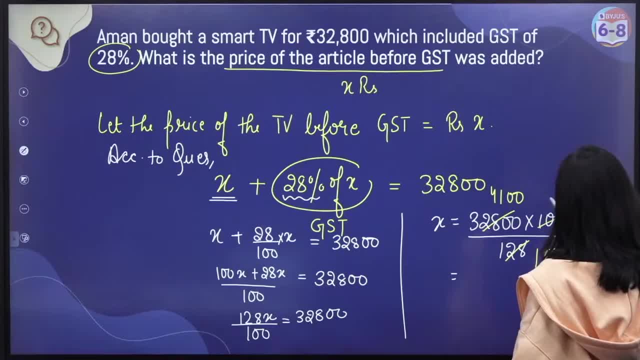 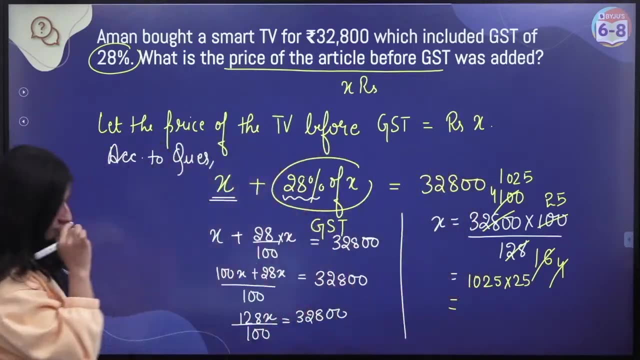 Isko bhi cancel kar dete hai. Ye ban gaya 25.. Aur ye ban chuka hai 1025.. To 1025 multiply by 25.. Batao kya aa raha hai: 1025 multiply by 25.. 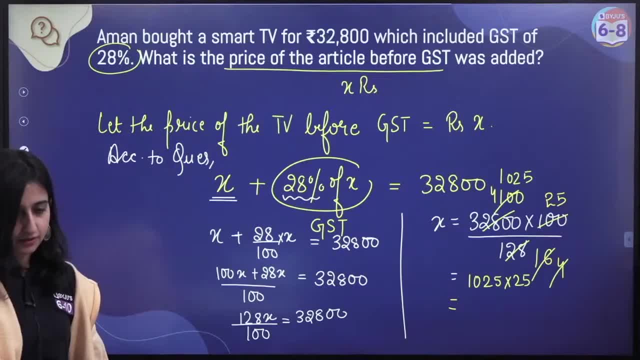 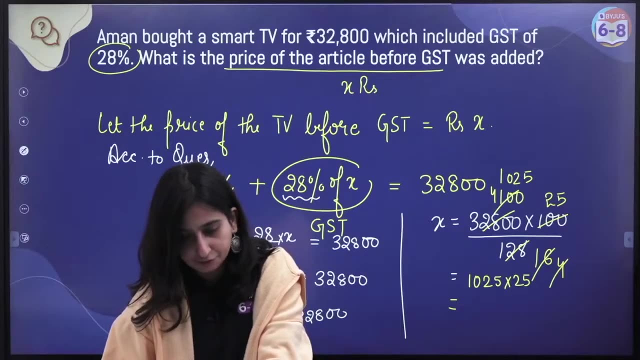 What is it coming Beech mein? kuch bachcho ke galat answer aa raha hai. beta. Please check your answers once. Some of you are giving me the wrong answers. So 1025 multiply by 25. 23,600: kaise ban raha hai, bachcha Payal? 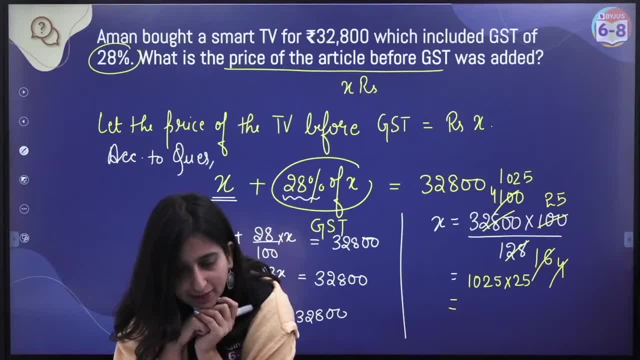 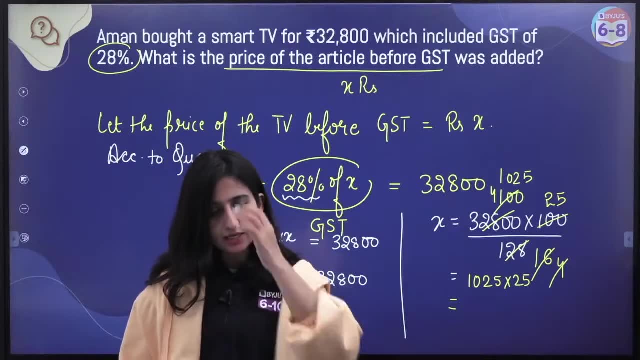 Please check your calculation. It will be 25,625.. That is correct. Very good, Rudransh, Money nahi sahi, answer nahi aa raha hai. Please check your answers. Ma'am clear nahi hua. fourth step pe: 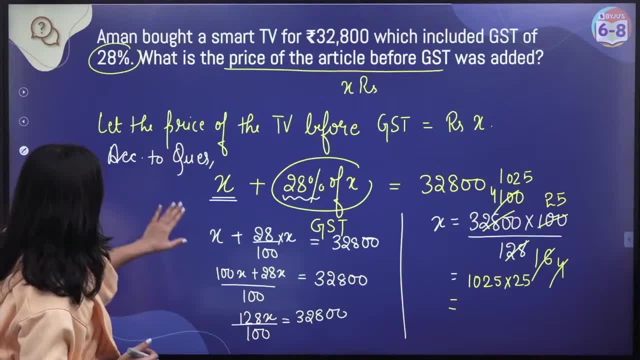 Fourth step: Kahan se beta. fourth step: 1,, 2,, 3,, 4.. Yahaan pe bachche Vaishnavi. Sorry, one shika Which step is not clear? Step number likh rahi hu main. 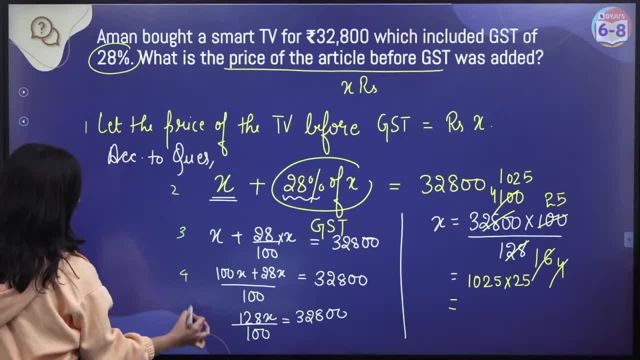 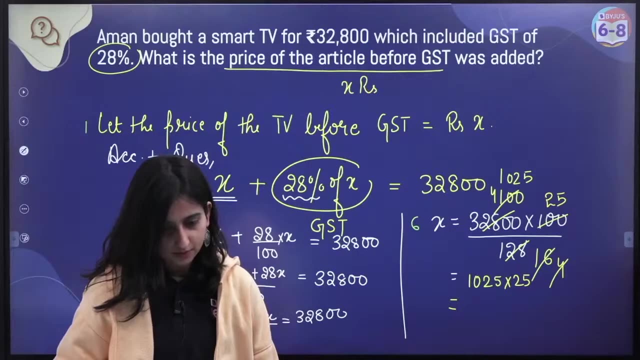 1,, 2,, 3,, 4,, 5. Tell me which step is not clear? 6. 6. Which step is not clear? Which step is not clear? Menti quiz beta Is question ke baad. 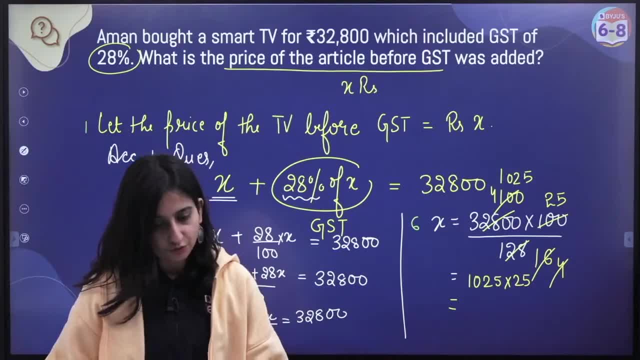 We are starting the menti quiz. 6 baji hum menti start karengi. Fourth step is not clear. Acha fourth vada step Ye nahi clear hua. Acha yahaan pe kya kiya beta. 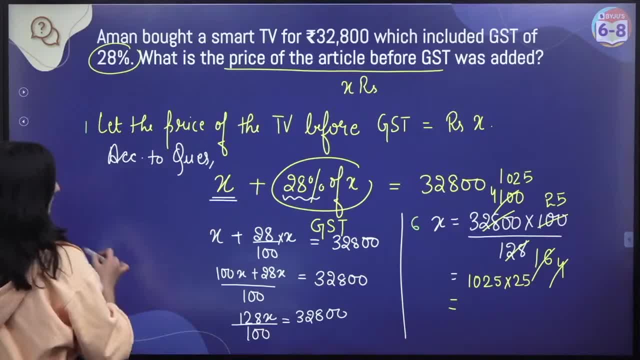 LCM liya hai. LCM lena aata hai, aapko LCM lena sikhaha hai Hai na LCM kaise lete hai. Humne yahaan pe LCM liya hai Dekho. 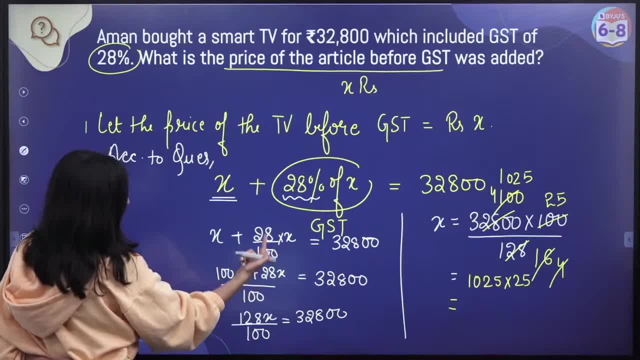 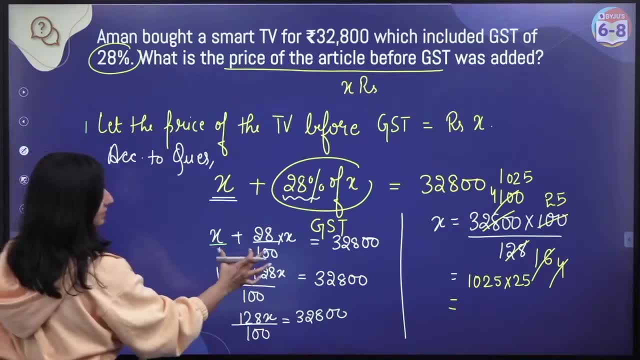 Jab aapke bachcha pass here in denominator. see here, 100 is there Here. what we have in denominator is 1.. So 100 and 1, what will be the LCM of LCM? What is the LCM of 100 and 1? Obviously 100.. Okay, So I am writing. 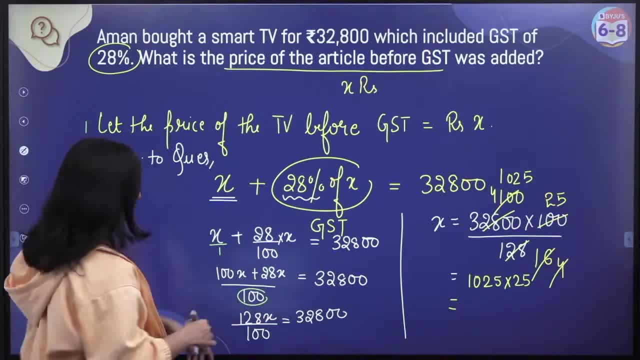 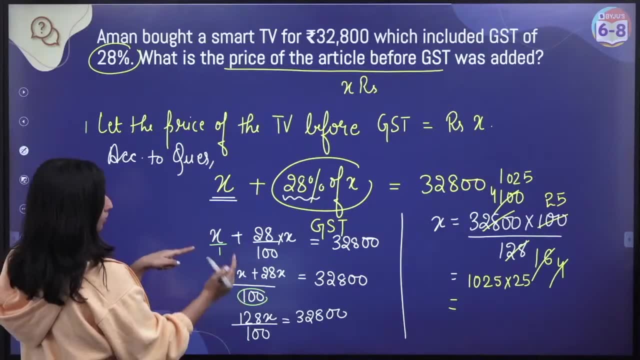 100 here. Here, 100 is written After that. what do you do? What do you do You cross. multiply these two, See 1,. 100 is 100 and 100 into x is 100x. This is how we take LCM, Right When you write. 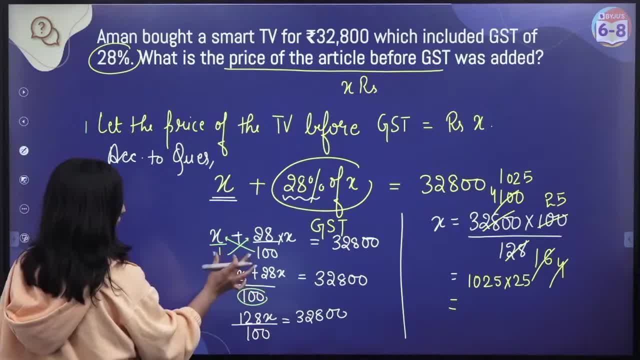 these two by multiplying. here. then you can cross multiply like this, only when you are, when you are writing here, the multiplication of this 100 into 1, here 100 has come. Basically, what is the LCM of 100 and 1? It is 100.. So here, in this case, you can cross multiply if 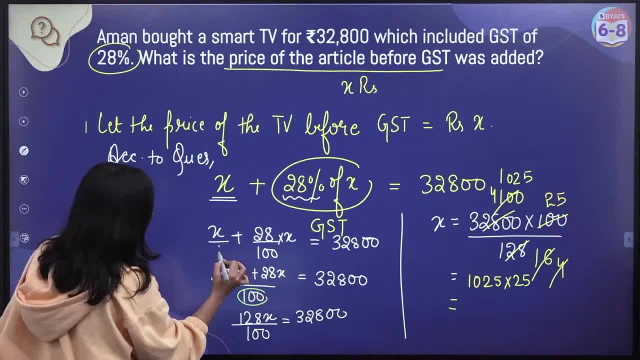 you are getting confused. Otherwise, in the right way, you can cross, multiply. So here: what is the LCM of 100 and 1?? You see how much of the denominator is multiplied and 100 is coming. So 1, 100 is 100, and then 100 into x is 100x. Okay, Similarly, now talk. 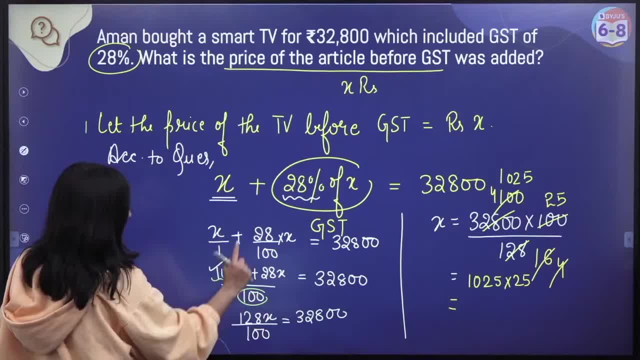 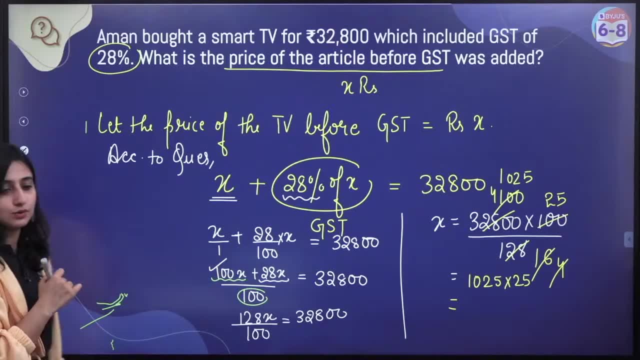 about this term: 100, 1 is 100, and 1 into 28x will be equal to 28x. That is why I have written 28x here. This is how you take LCM Right. This is how we take LCM Right Now. 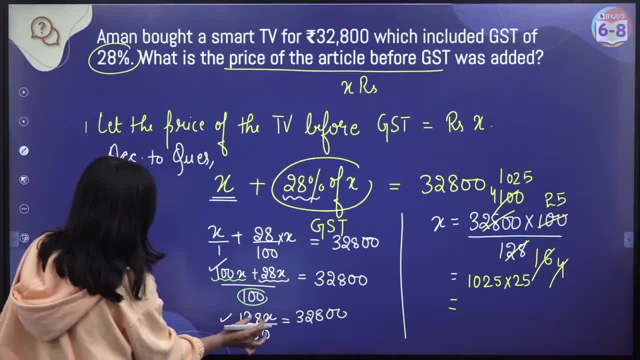 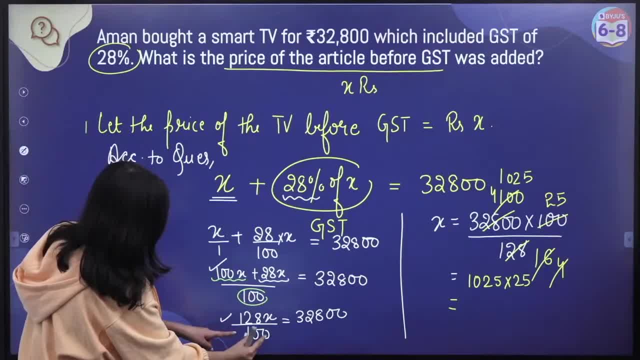 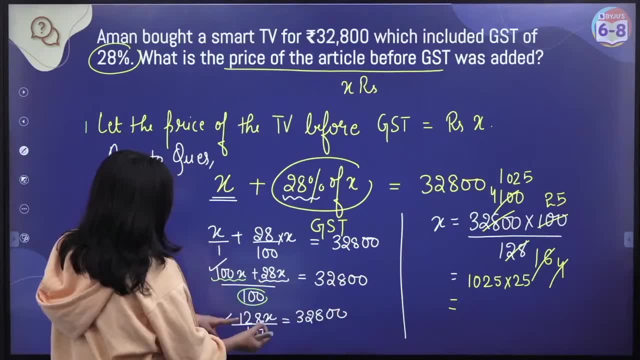 128x divided by 100 into this. After that, what we did, We took 100 there. 100 is getting divided here. If I take it to the right hand side, it will get multiplied Right, And this 128 is getting multiplied with this x. When I will take it to the right hand side, it 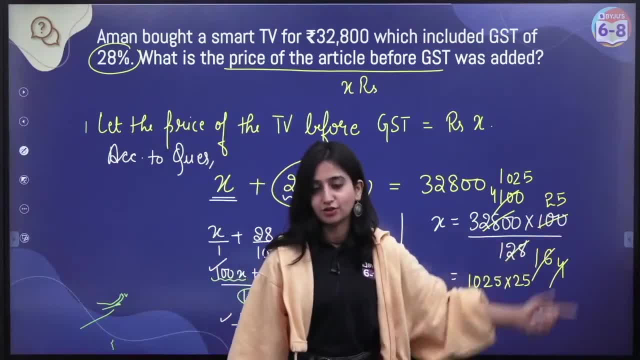 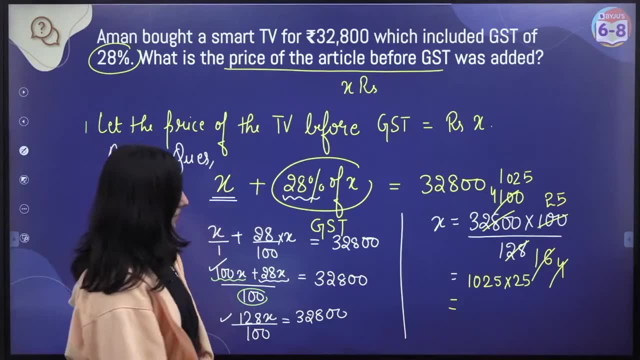 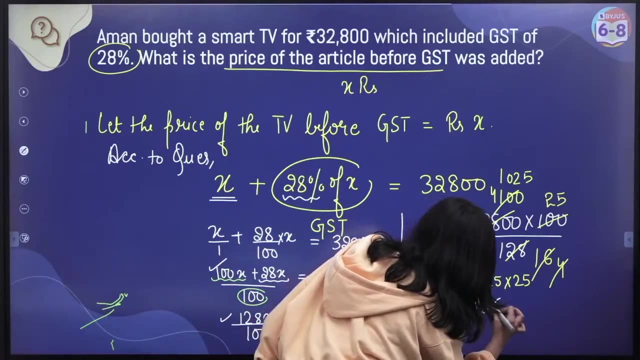 will get divided Right. So that's why we wrote 28 below We multiplied 100.. Okay, Did everyone understand? Yes, So the answer is coming out to be is 25625. yes, 25,625 is the right answer. so this is the original price of. 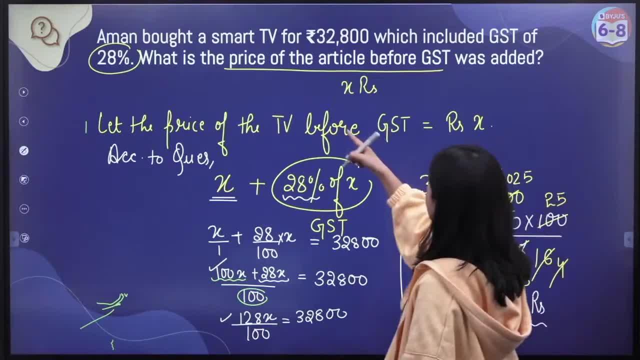 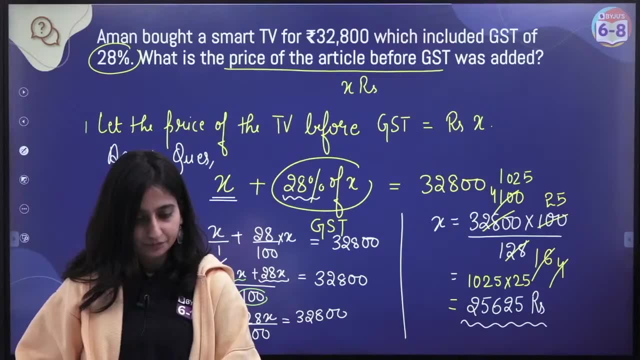 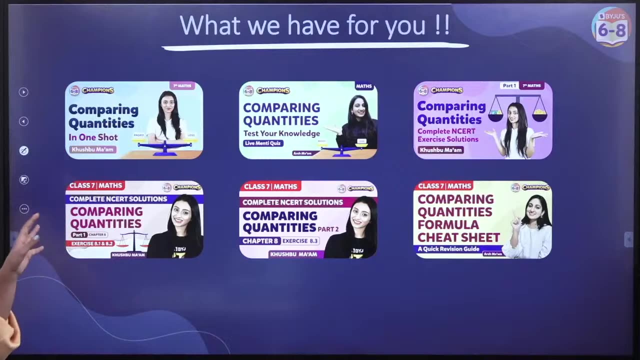 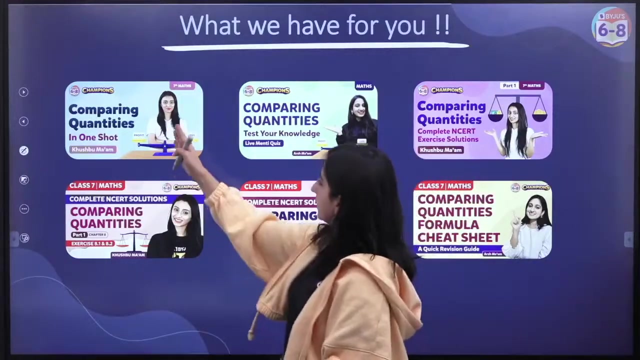 the TV. This is the original price of the TV After applying GST on it. you have to pay this much. Let's move on to the mentee quiz Before this. if you face any kind of problem in this chapter, then you can refer to all these videos. We have taken so many sessions on the comparing quantities. 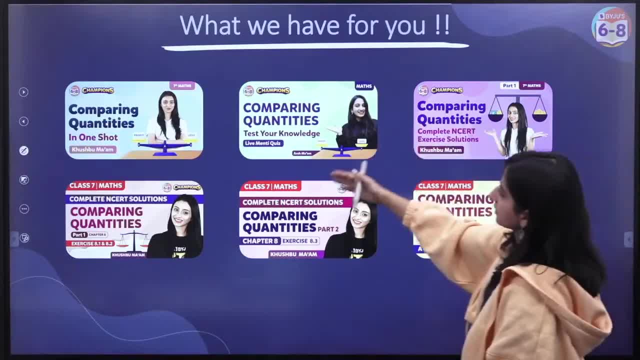 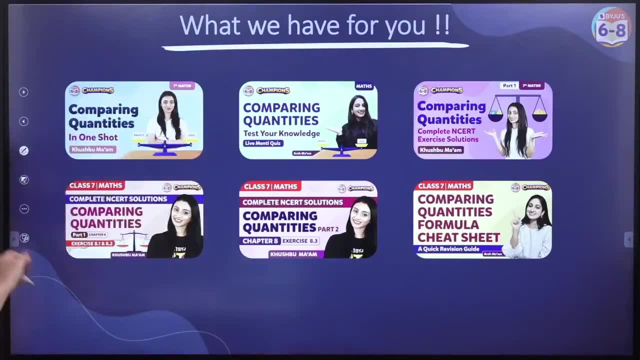 I have done a cheat sheet. we have taken so many sessions in khushboo. I have also done live mentee quiz with you guys, So we are going to give you a story in this chapter sessions already so you can go and watch these sessions if you face any type of difficulty still. 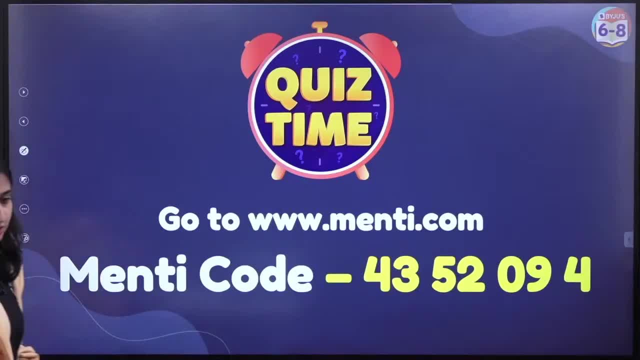 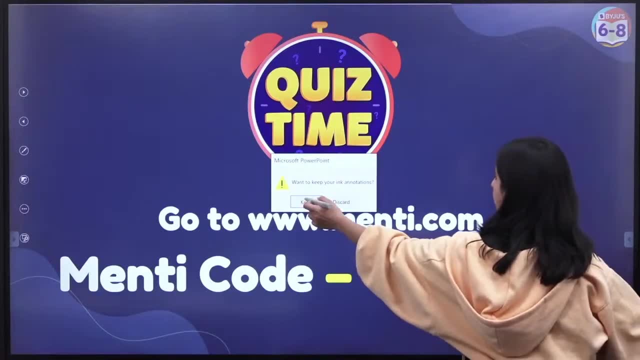 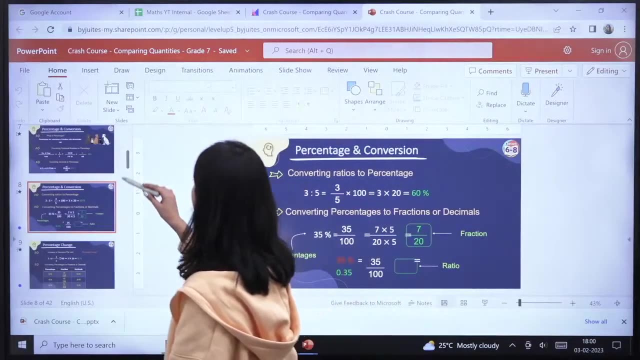 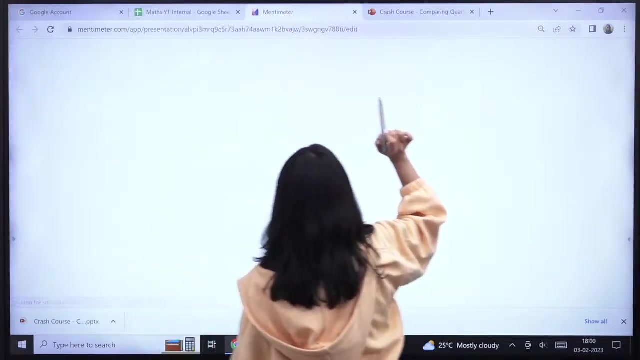 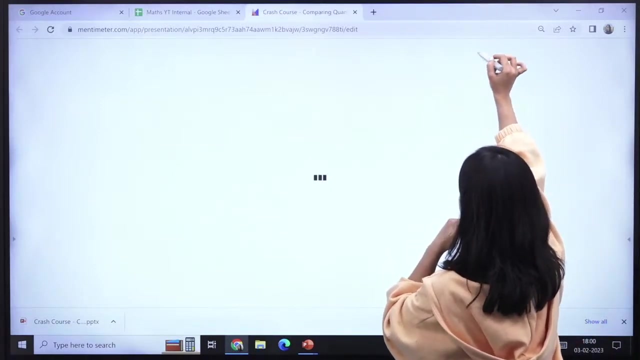 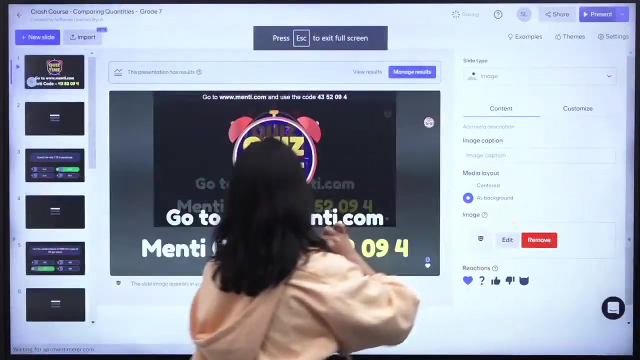 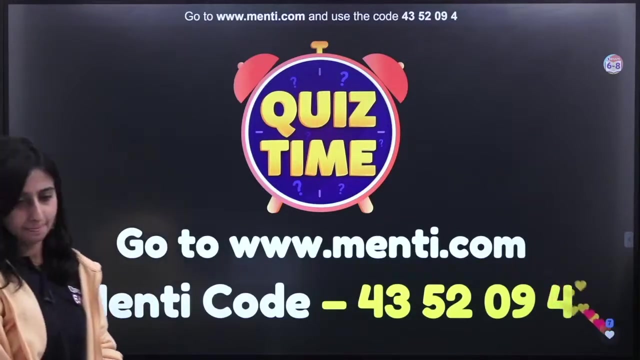 and now let's move to the mentee quiz. let's move to the mentee quiz now. all right, so okay. so just let's just wait for a second. it's loading, yeah, let's start. okay, now go to wwwmenteecom and enter the question. 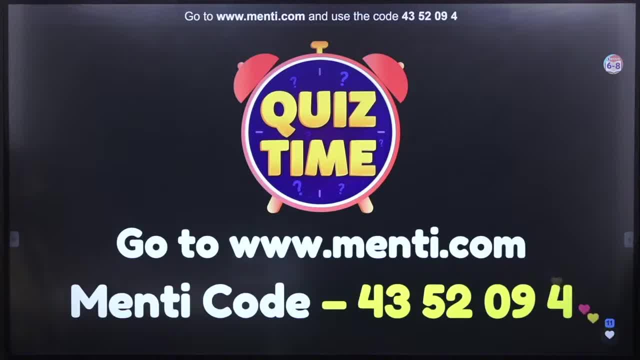 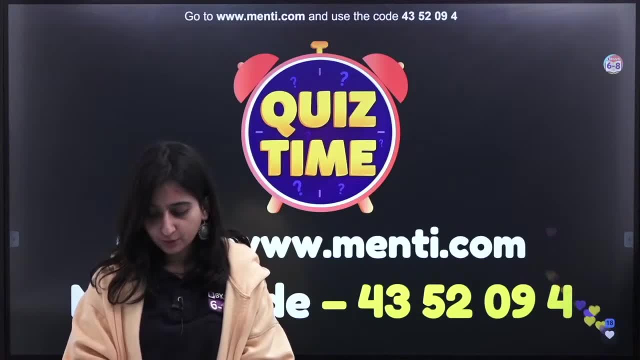 enter the code 4352094 and join the quiz quickly. yes, chaldi se. go to wwwmenteecom bacha and join the quiz. yes, chimmy has joined. very good, kimaya. i've joined vani. very good, nitish. quickly join the quiz. rudraan shimmy is giving your answer. 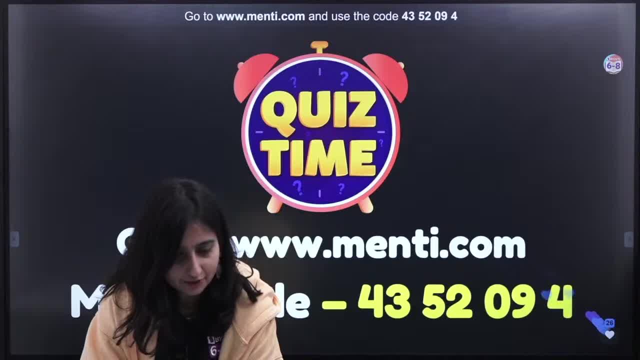 daivik. very good, nutan has joined shabash satyam. okay, satyam, i will give you time. don't worry, chaldi, se aap log quiz, join karlo. your quiz code is 4352094. quickly join the mentee quiz bache. 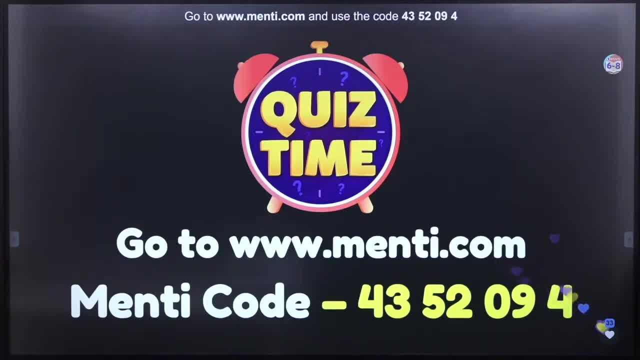 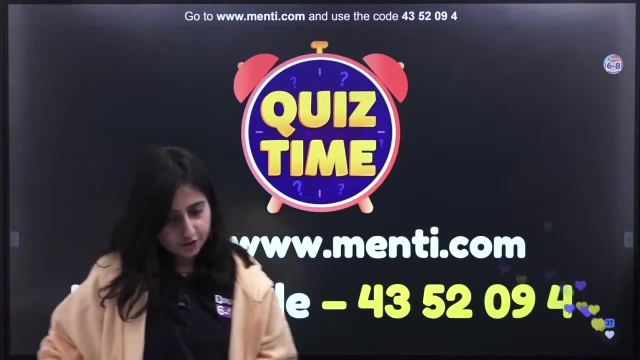 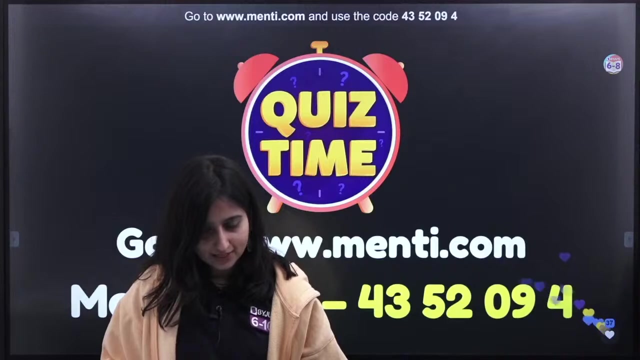 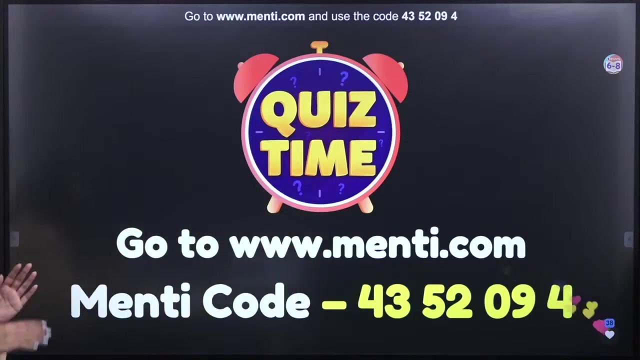 yes, and bananas have fit. yo asli muktad kiya hai. very good, itesh mubeen. sankit hi nitesh priyane. very good, join the quiz and then we will start. so let me move to the next page so that you can write your. 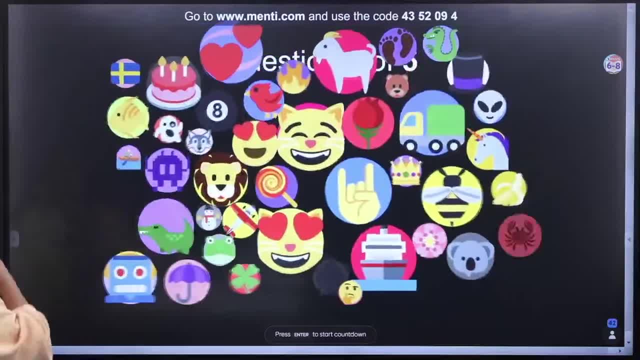 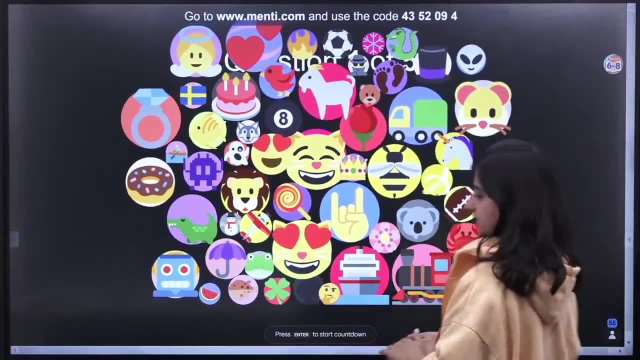 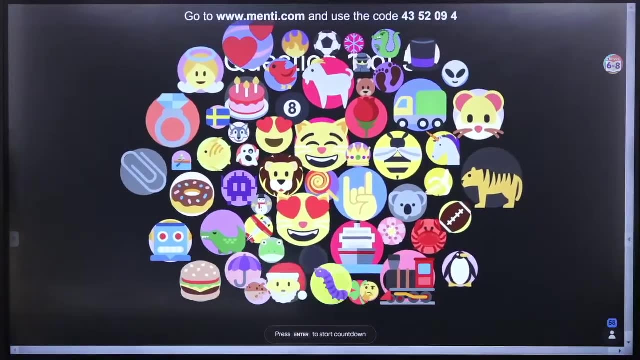 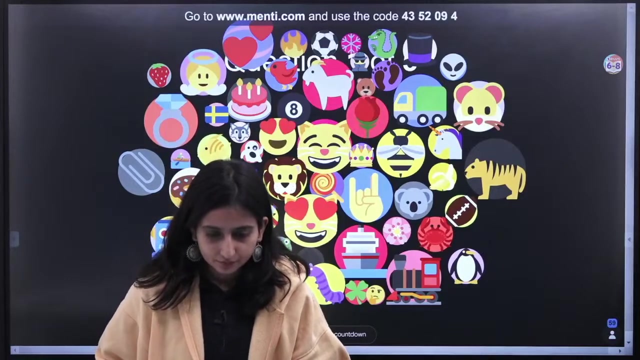 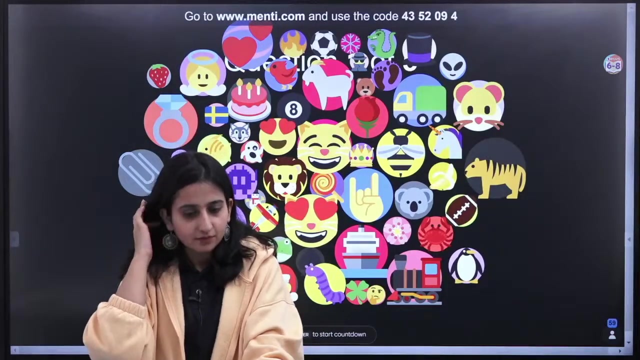 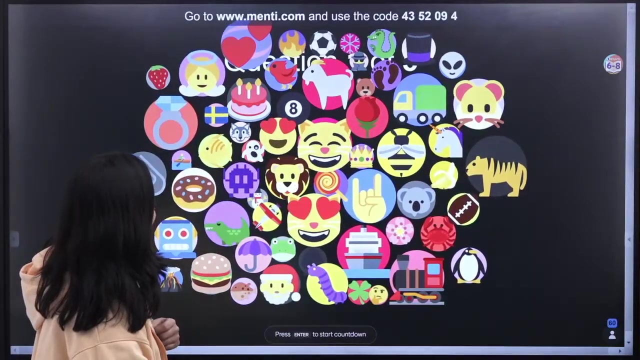 names. write your names quickly. so 54 students have joined the quiz. yes, everyone. and also quickly hit the like button. quickly hit the like button also, let's go. so now. fish is aditya. okay, where is the fish? when you speak like this, then I stop seeing. 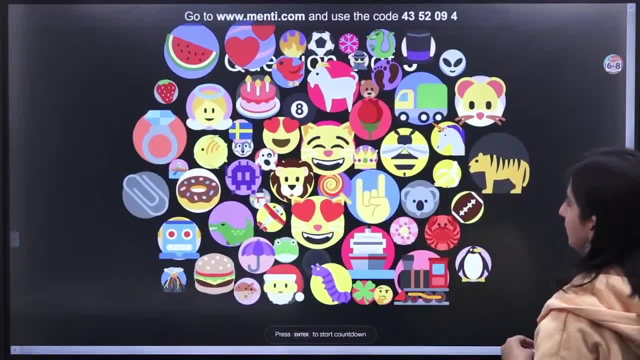 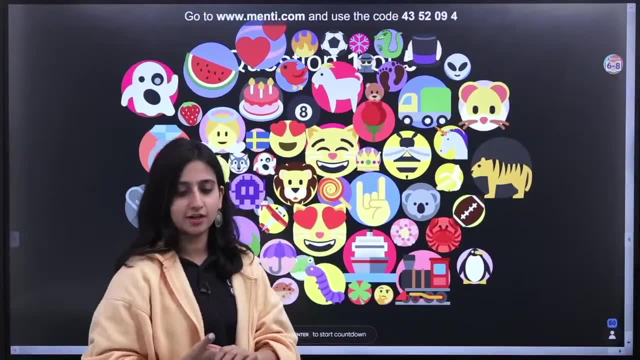 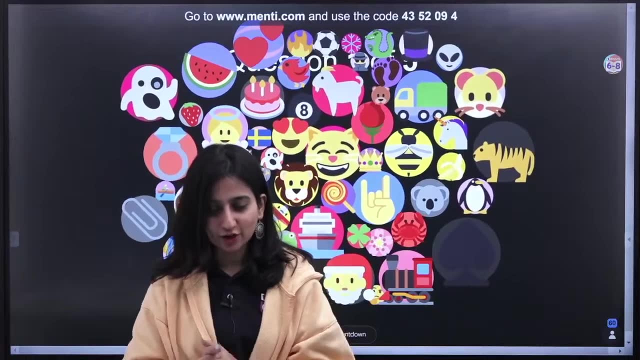 ok, I can't see the fish. no, no, no, I see the fish. I see you, aditya. then we have ghost with us. who is burger? mamta is a wolf. okay, yes, fayaz, join the quiz quickly. nidhi is unicorn, then vanshika is. 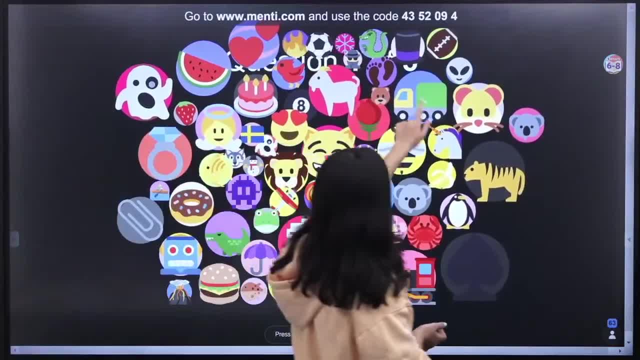 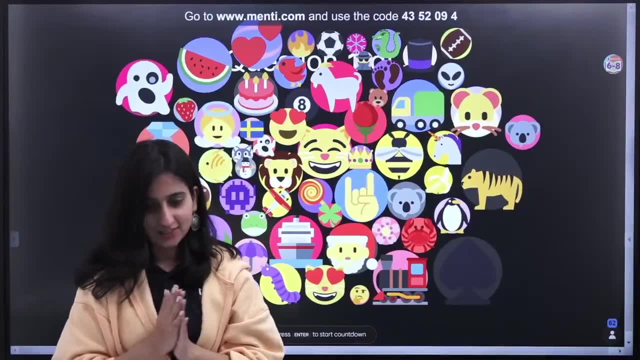 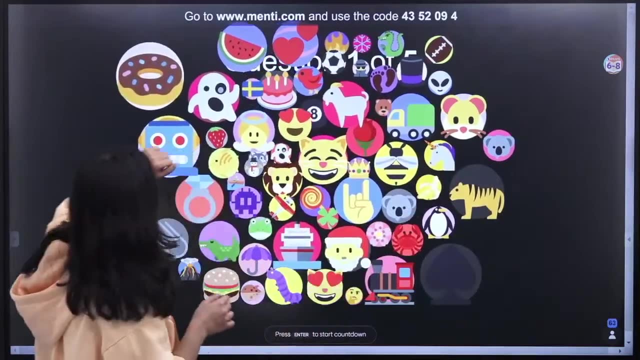 teddy. where is teddy? here it is, and I got unicorn too. I got teddy too. very good, come on. come on. yes, I can see the rose. okay, yes, I have seen. I have spotted the roads here, rings, no man. okay, so many of you have joined the quiz. well done, chalo to start cutting. Hey with the very first question. 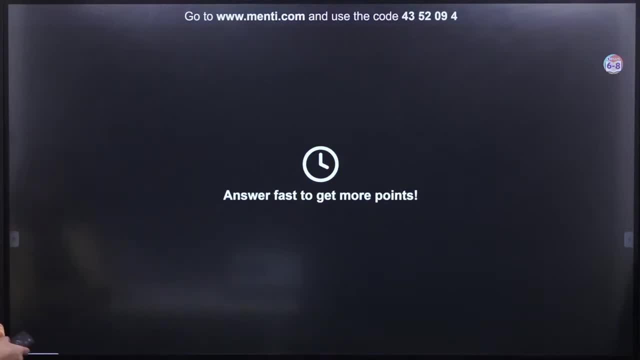 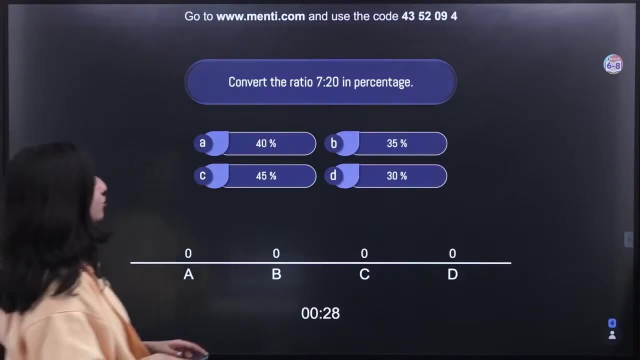 okay, so first question comes on your screen. look at the first question: convert the ratio seven is to twenty and percentage. you have to can do the conversion. convert this ratio. you have to convert the ratio 7 is 20 in percentage. you have to do the conversion. you have to convert the ratio 7 is 20 in. percentage. you have to come do the conversion, convert the ratio. 7 is 20, not very available, but when you you do the conversion, convert this ratio 7 is 20 in percentage. so this is the conversion. this is the position you hadplay. you have to guess will be like ת् Bamberto longuu, I get 17,ト்кв. 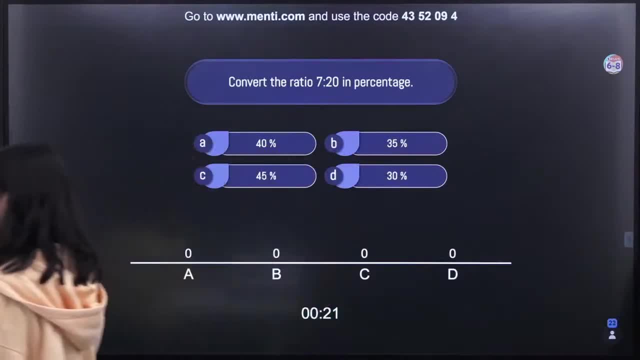 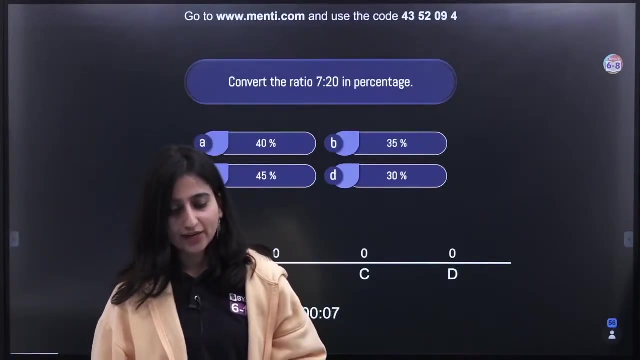 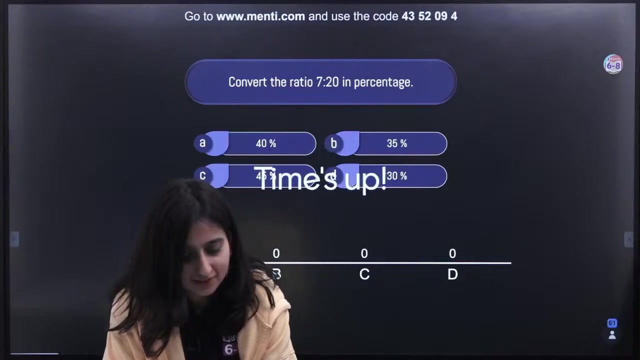 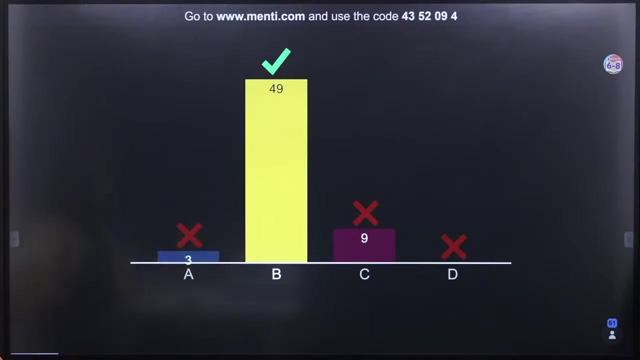 conversion. convert this ratio into percentage. yes, everyone. okay, last 10 seconds are left. bacha, last 10 seconds are left and it'll quickly join the quiz. okay, so we have. okay. so 49 students have given the right answer. very good, so 7 by 20. 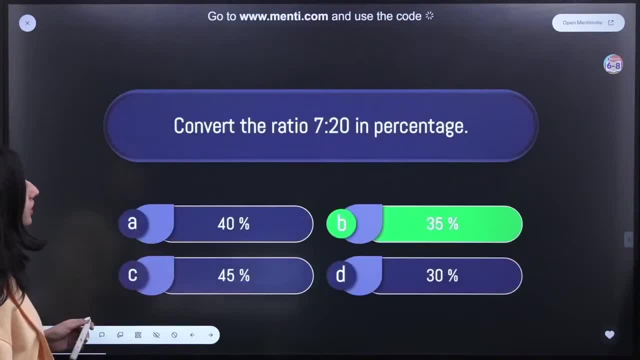 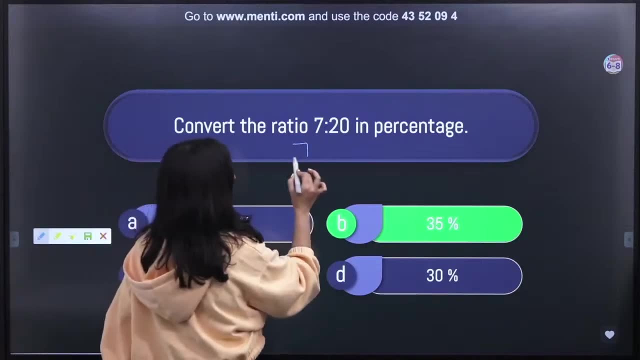 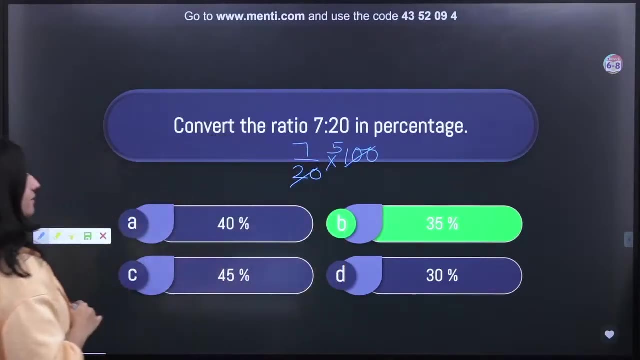 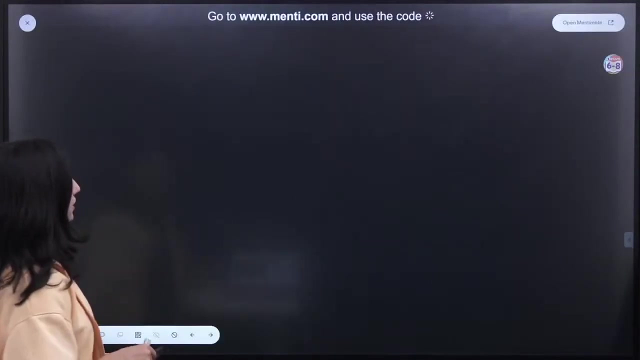 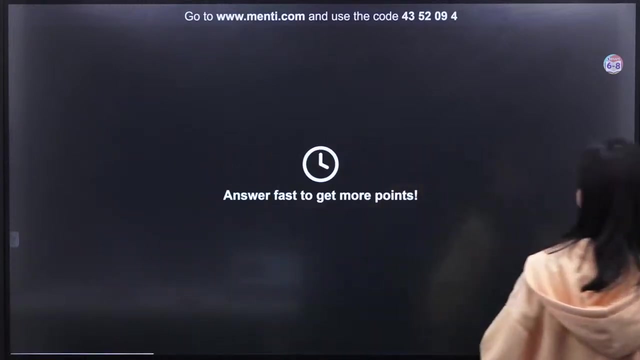 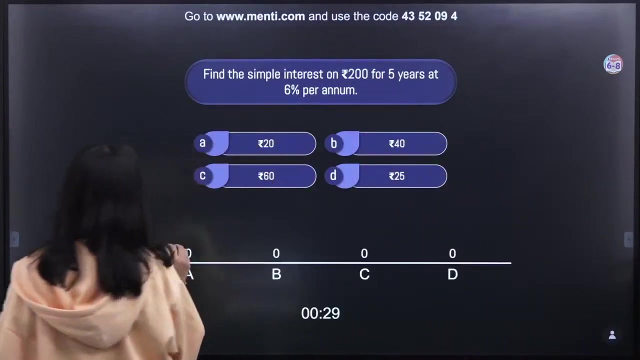 we know how to convert a ratio into percentage. 7 by 20 into 100, right, 35, 35 is the right answer. yes, let's move on to the next question. so question number two, coming right up on your screen. okay, find the simple interest on 200 rupees for five years at six percent per annum. 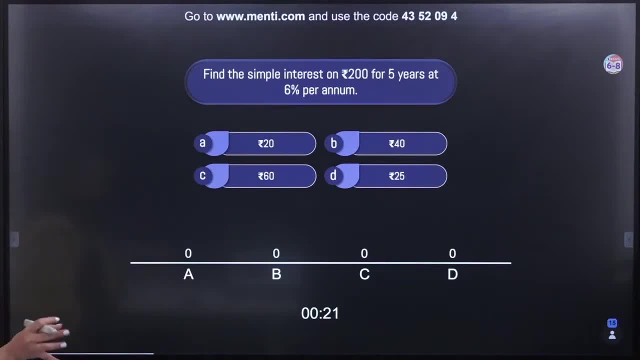 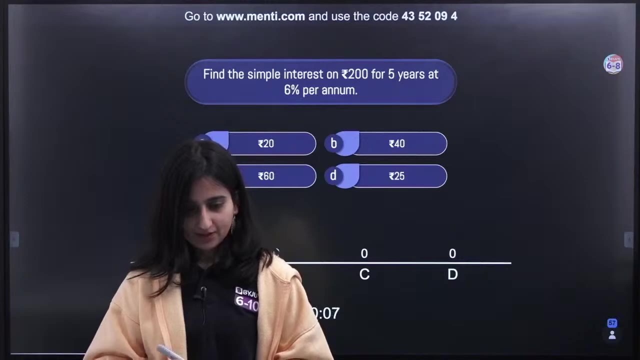 so okay, find the simple interest on 200 rupees for five years at six percent per annum. so time b hai apke pass rate bhi de rakha hai. you have to calculate the simple interest, just direct formula based question. yes, everybody. what is the answer? 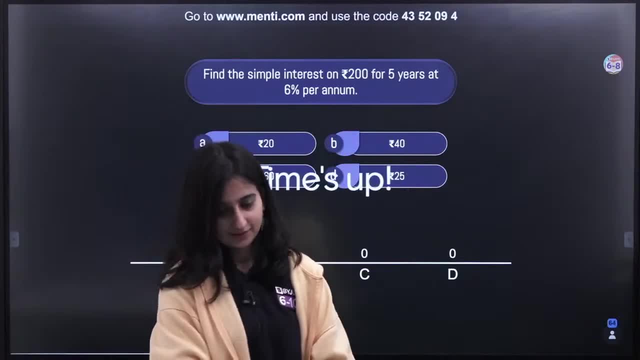 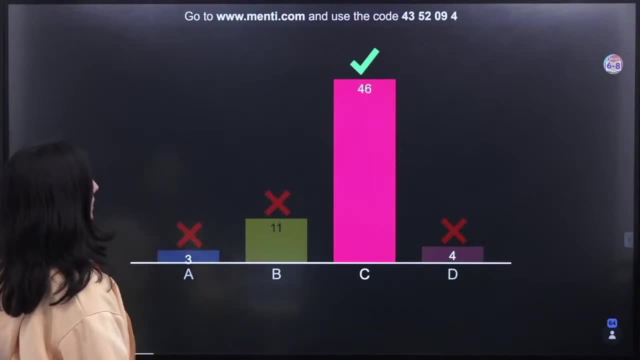 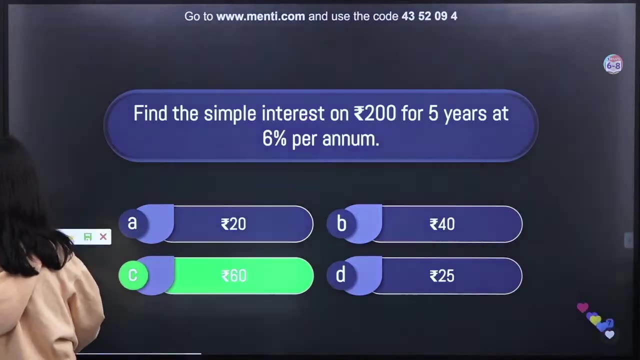 okay, time is up, all right. so 46 students have given the right answer. very good, bacha, PRT by 100 lagna tha aur kuch bhi nahi karna tha. iss question me hai na. so aapke paas principal amount kitna de rakha hai. 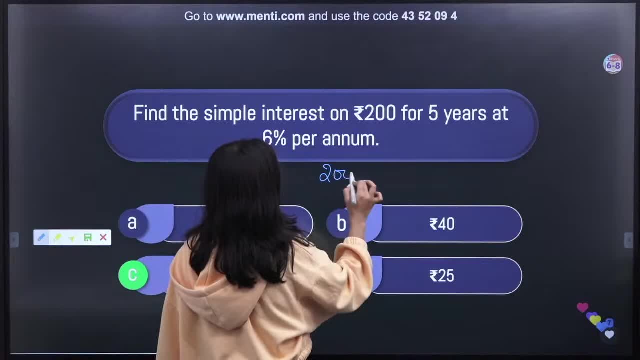 principal amount is given as 200 into R rate. kitna hai 6% time, kitna hai 5 years PRT by 100 to aapke paas kitna ban jayega ye: 6 x 5 is the 30, 2 is the 60. 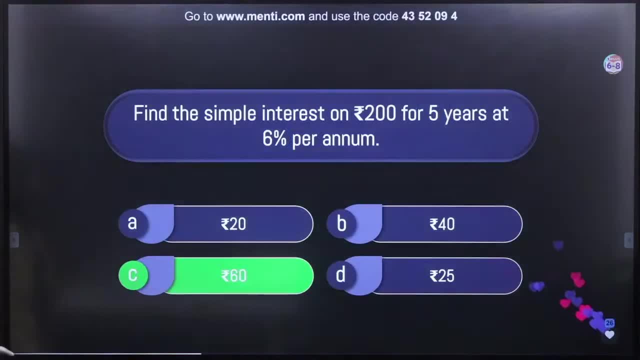 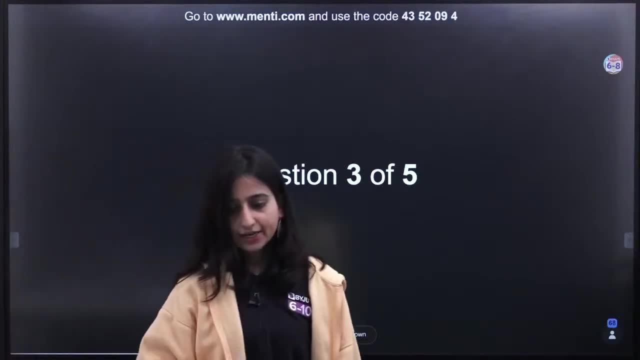 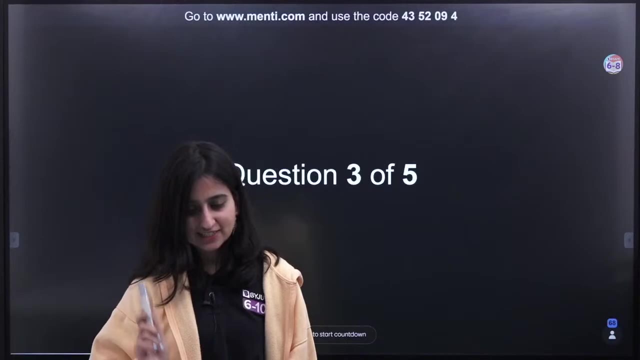 to 60 rupees is the right answer. chalo next question on your screens: hi Antara ab khush hi Aradia. yes, Simranjeet, 60 is the right answer. bacha, koi baat nahi, devik. next question: dhyan se click karna. 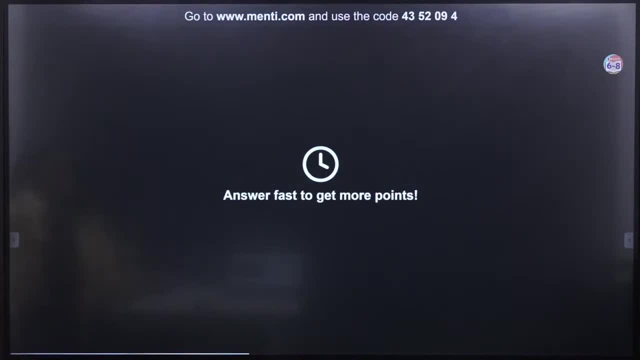 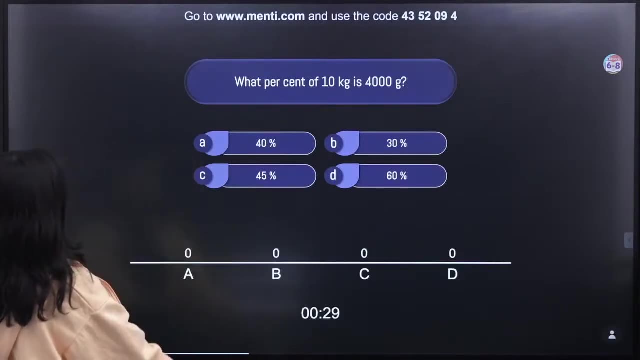 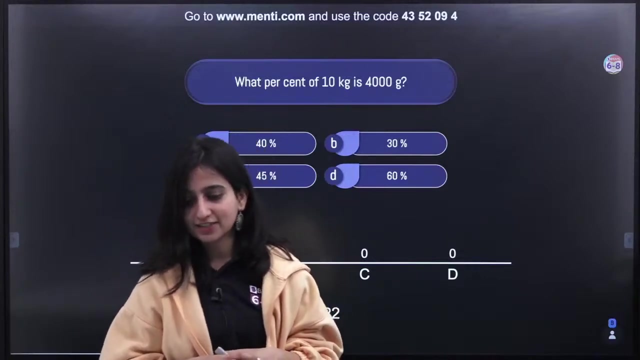 question number 3 on your screens: what percent of 10 kg is 4000 grams? I remember maine ye question aapko one shot me bhi karaya tha, jab humne comparing quantities revised kiya tha. maine tab bhi aapko. 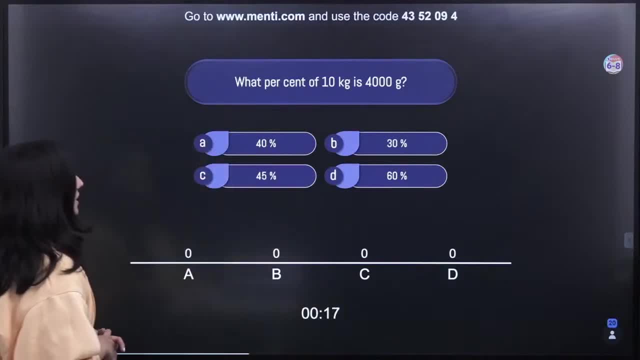 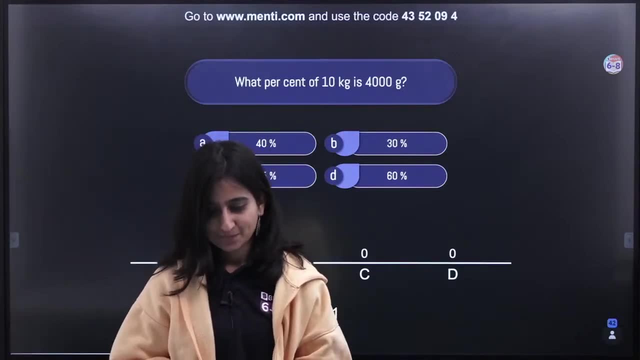 aisa sa question karaya tha. let's see how many of you can get it right. what percent of 10 kg is 4000 grams? Pooja has done, Sneha has done. ok, dekhne wali baat. ye hai ki kitne bache. 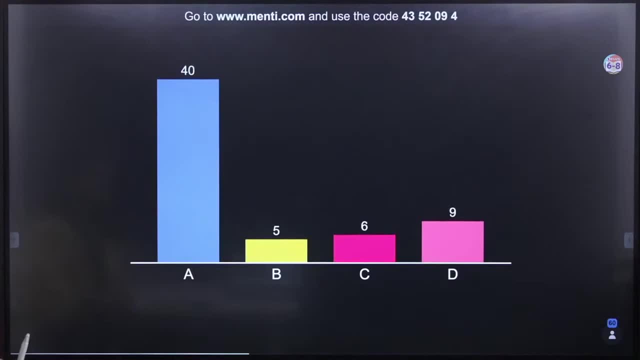 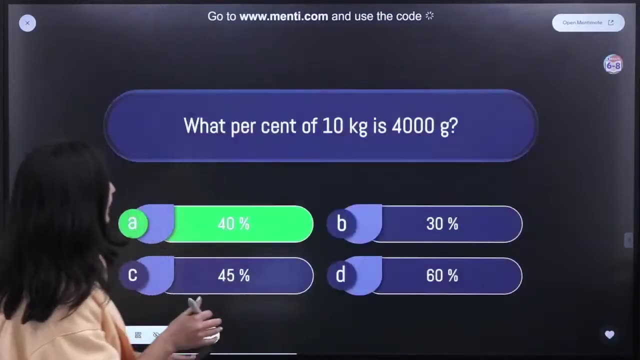 iska answer sahi dete. kyunki silly mistake ho sakte hai, agar aapne conversion nahi kiya. very good, maximum students ne sahi answer diya hai: shabash, shabash, chalo. toh is question ko kaise karna tha? 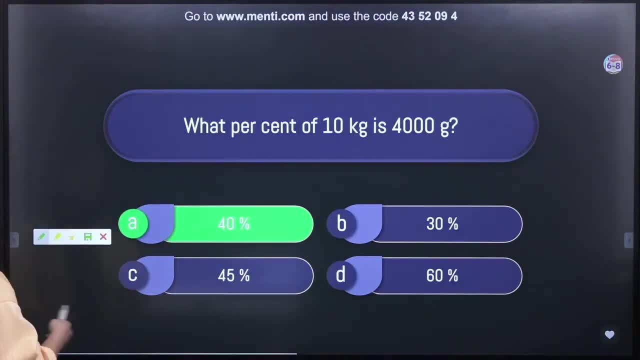 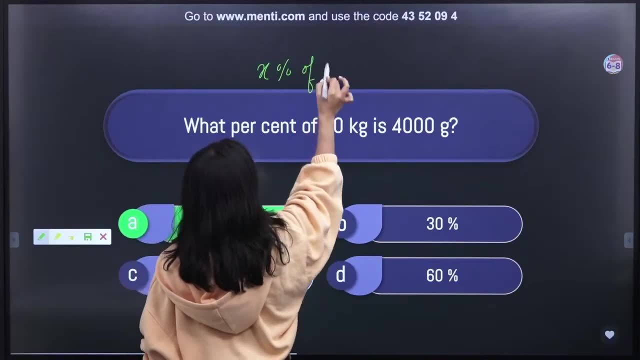 dekho jinka galat hua hai. wo kaha pe mistake hui hai. let's find the mistake. what percent of 10 kg matlab? I don't know what percent. let's say that x percent of 10 kgs is how much? 4000 grams? 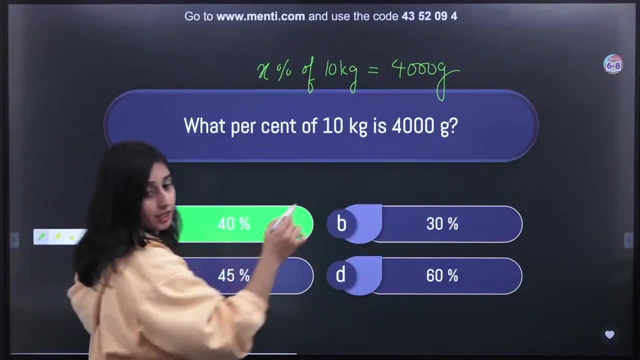 now sabse badi baat, yaha pe aapko kya notice karne thi units same nahi hai. yaha pa yaha pe kg hai, aur yaha pe grams hai. toh yata aap grams ko kgs me change kar do. 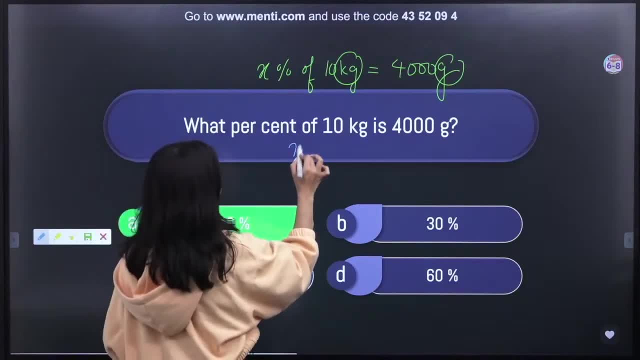 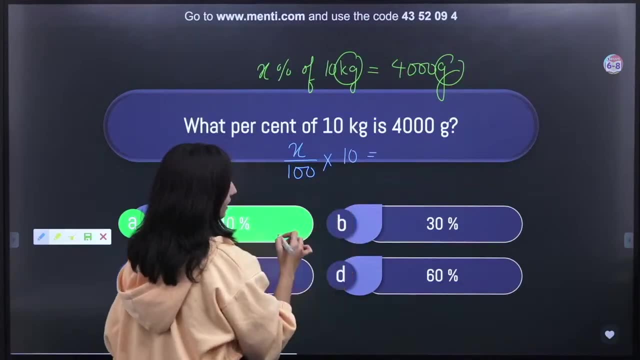 yaa kgs ko grams me change kar do, toh hum kya karenge. x percent ko likh diya, x by 100 off ko kar denge into 10 ko 10 kgs ko mai kgs hi rakh rahi hu. 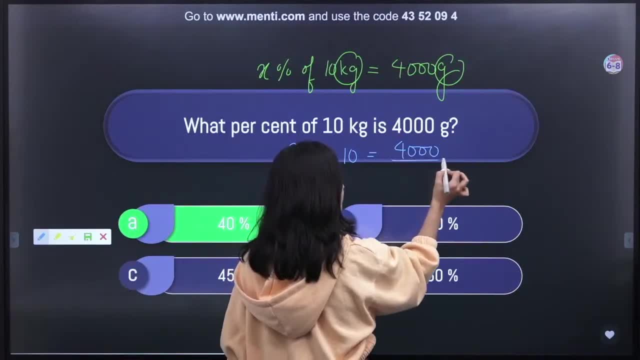 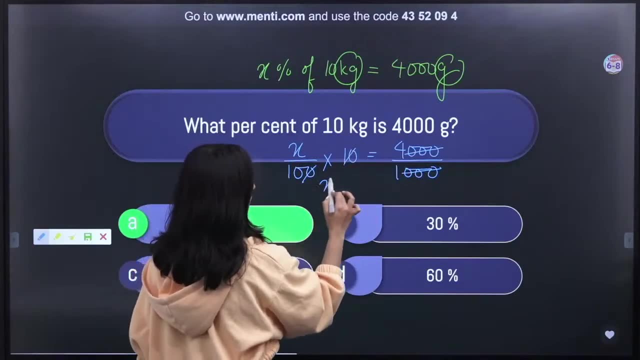 aur yaha pe, mai grams ko kyunki 4000 grams hai, usko kgs me convert karenge, toh divide by 1000 ho jayega. toh, yaha pe, kya ban gaya aapke paas. x is coming out. 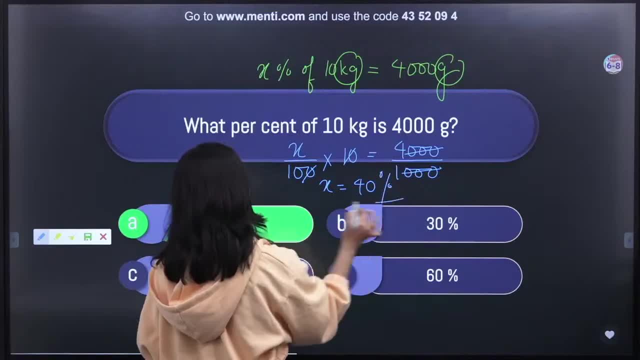 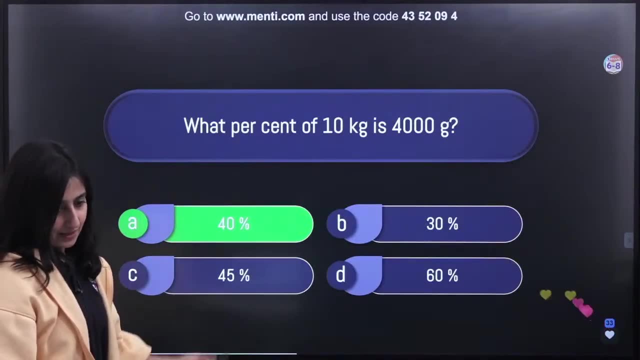 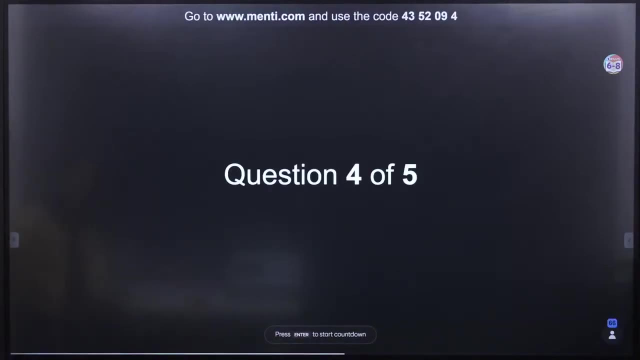 to be 40 toh. kyunki x percent tha toh 40 percent is the right answer, chike chalye. now moving on to the question number 4, last second question of the day, everybody chalye. so here comes your question number 4. 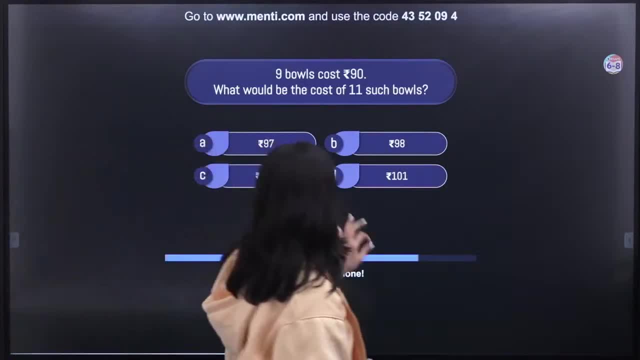 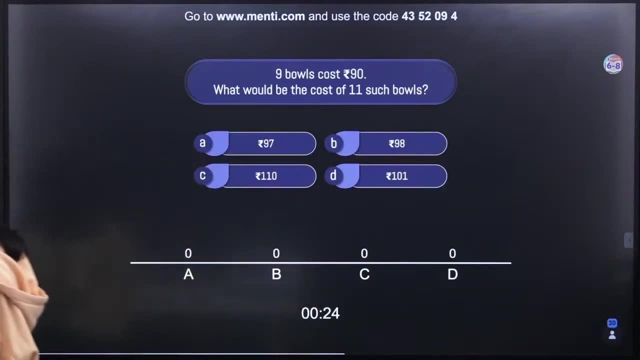 9 bowls cost 90 rupees. what would be the cost of 11 such bowls? 9 bowls ka cost aapko de rakha hai aapko extra cost aise 11 bowls ka cost nikalna hai, toh aapko pata hai. 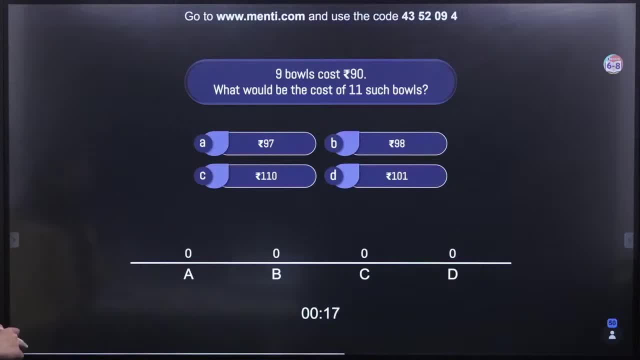 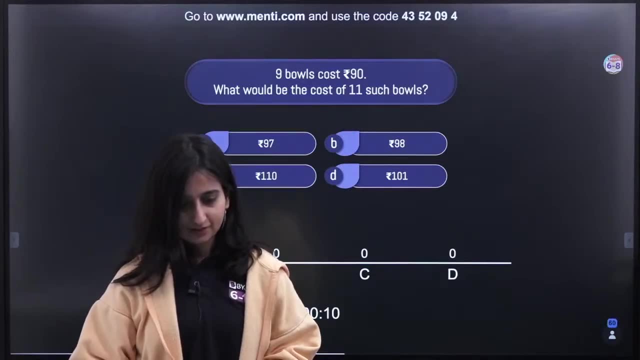 ki aise questions me ham kya use karte hai? we can use unitary method, right? yes, yes, mubeen misclick kar diya vani ne chalo, koi baat nahi. so your time is up. ok, i can see so many of you. 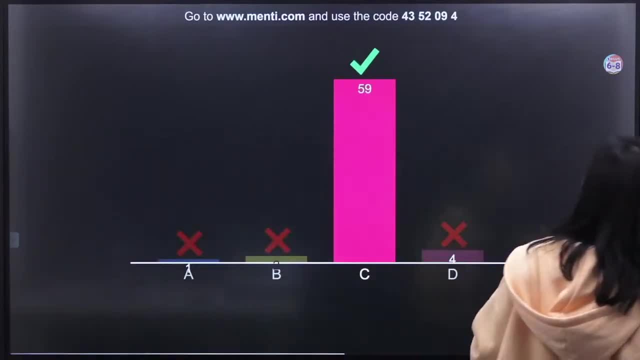 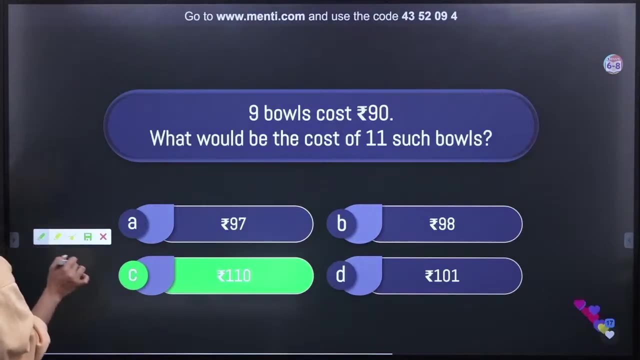 have given the right answer. very good guys. guys, toh isko kaise karna tha. is question ko chalo unitary method lagate hai. toh unitary method kya bolta hai? this method says: 9 bowls cost 90 rupees. 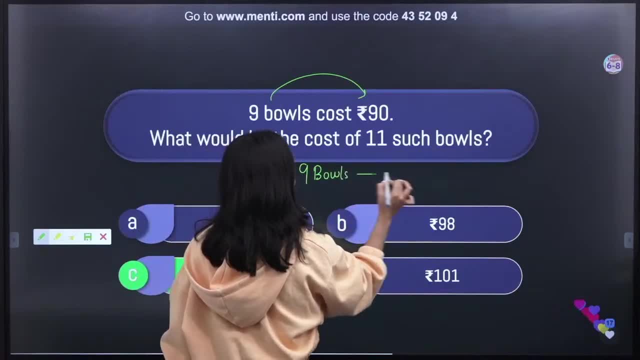 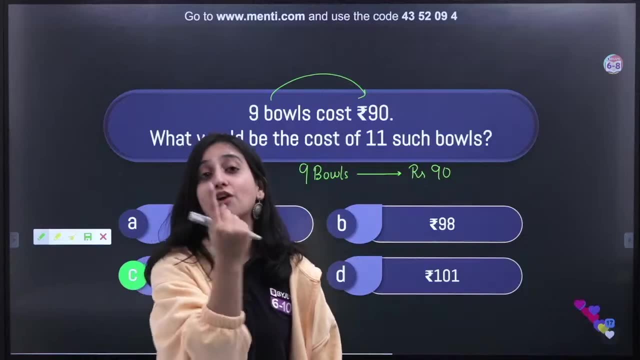 toh 9 bowls ka cost kitna hai. cost hai rupees 90 achay can i calculate the cost of 1 bowl? if 9 bowls are for 90 rupees, toh 1 bowl ka cost kitna hoga. so 1 bowl. 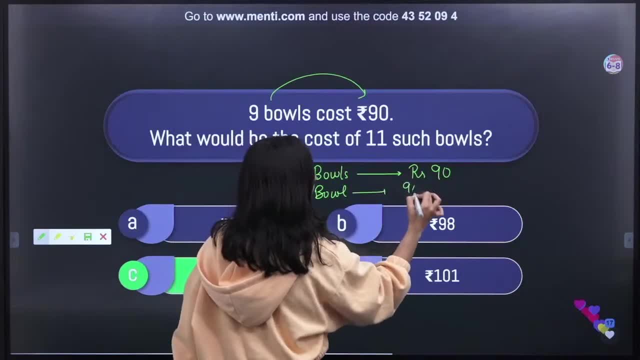 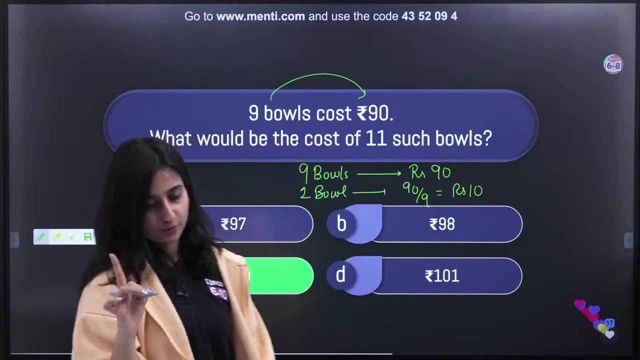 ka cost ho jayega. hamare paas kitna 90 divide by 9, that is rupees 10. toh 10 rupees ka 1 bowl hai hai na 1 bowl kitna hai 10 rupees ka hai. ok, now what would be? 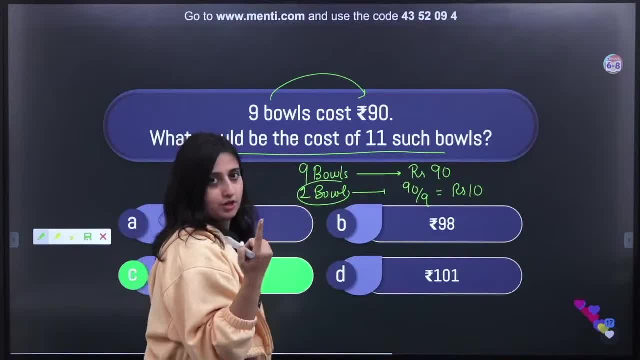 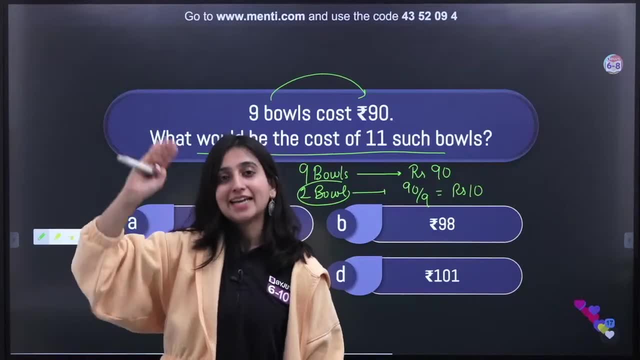 the cost of 11 such bowls. now i know the cost of 1 bowl, toh 11 bowls ka cost kitna hoga. if 1 bowl is for 10 rupees, toh 11 bowls will be of how much? 10 into 11, that is. 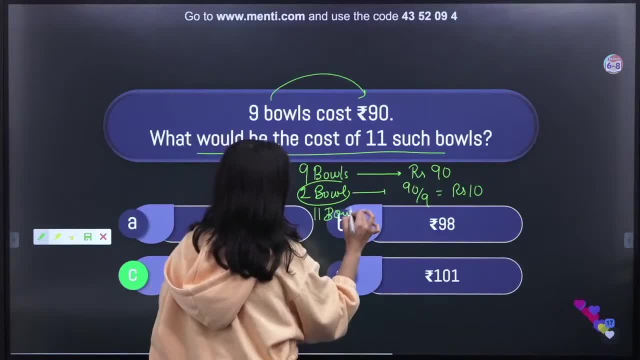 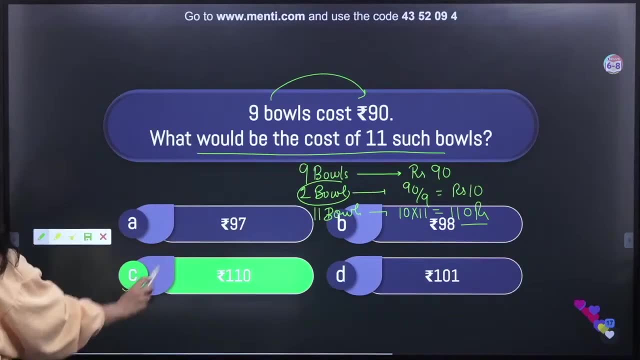 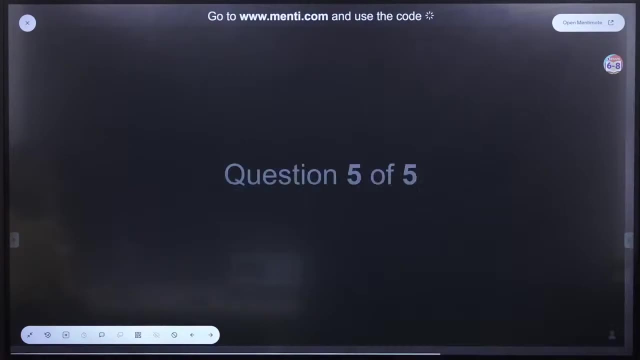 110 rupees. toh, agar 11 bowls ka ab amane cost nikal na hai, that will be equal to 10 into 11. that is 110 rupees. so c is the right answer here. ok, now last question of the day. let's move to. 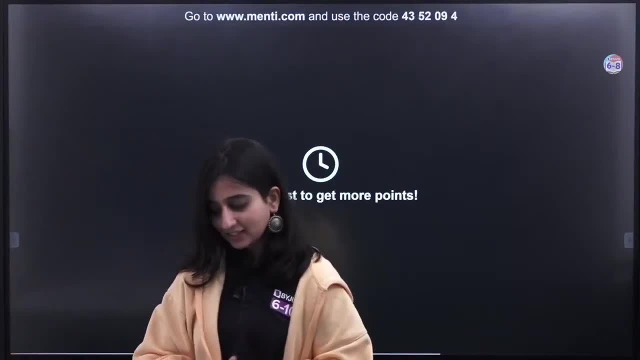 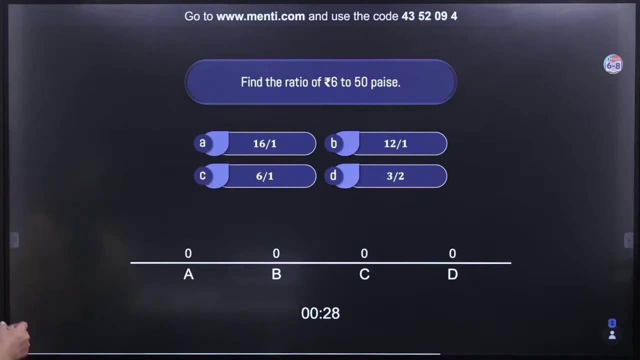 the last question of the day everyone. yes, done in 3 seconds. very good, sneha chalo. so last question: kya bolta hai find the ratio of rupees 6 to 50? paiste aapko ratio nikalni hai? please dhyan se. 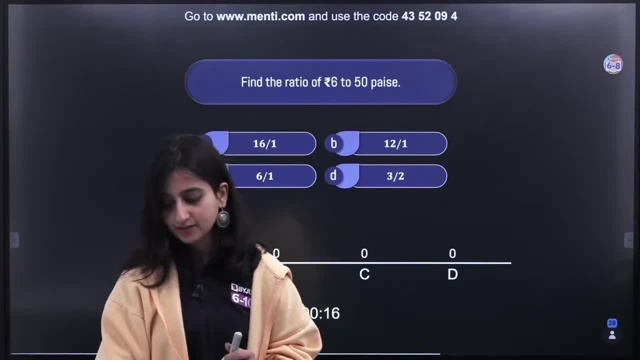 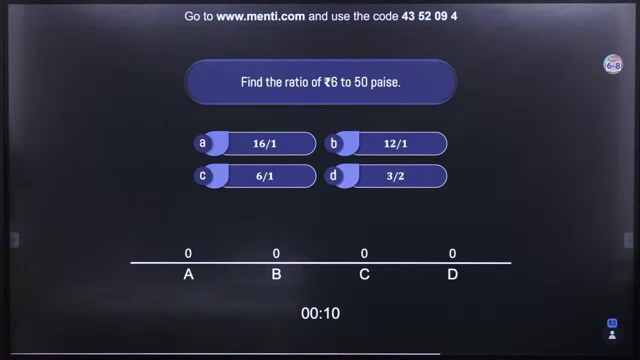 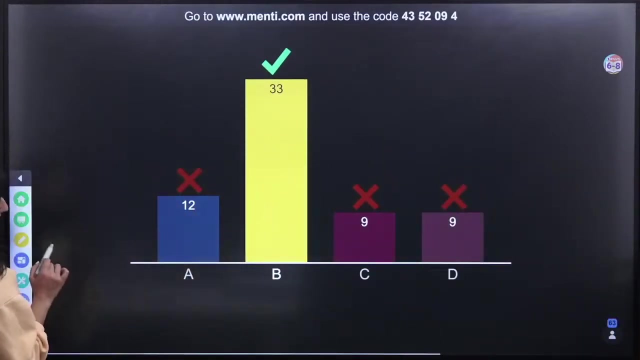 karna. try not to misclick in this question. question is very easy. question is very easy. last 5 seconds: 5, 4, 3, 2 and 1. very good, so 33 students have given the right answer. mai dekh rahe hoon ki. 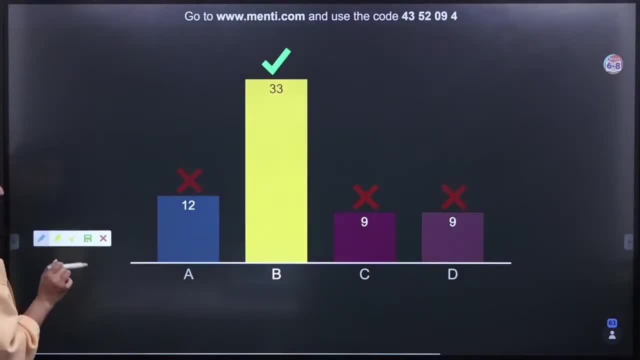 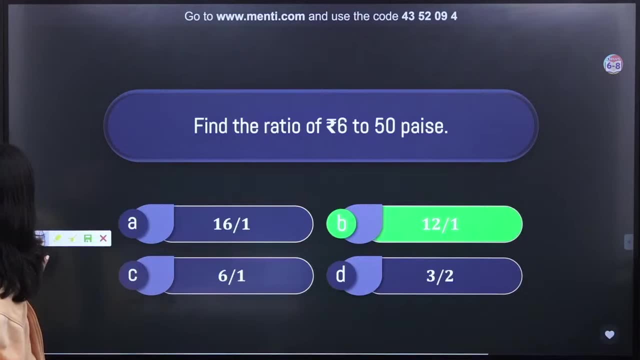 galti bhi iss question mein kaafi bachcho ne kar di hai. kya ho gaya iss question mein kaise karna tha wait. so yeh tha hamara question to iss question ko kaise solve karna tha, dekhte hain. 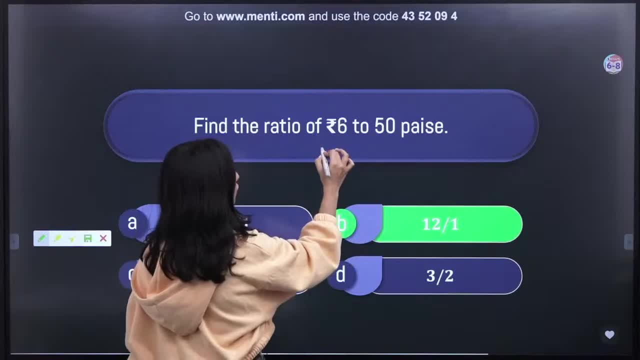 find the ratio ratio. lena tha 6 rupees. dekho 1 rupee mein kitne paise hota hai. 1 rupee mein kitne paise hota hai. 100 paise hota hai, ki nahi hota hai. 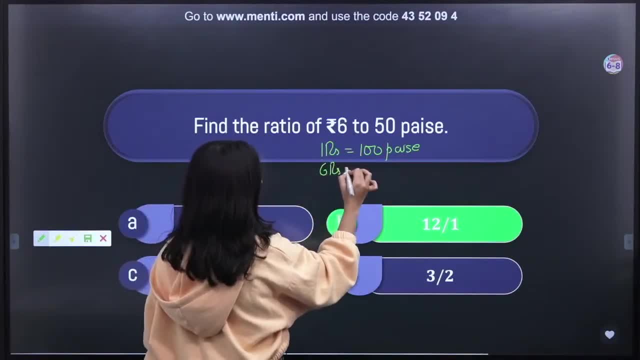 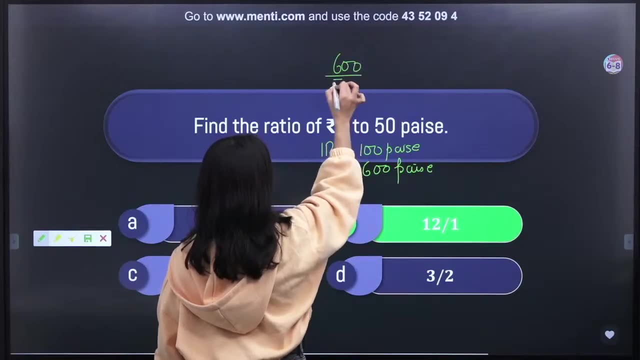 yes or no to 6 rupees mein kitne paise ho jayenge. batao 600 paise honge ki nahi honge. yes or no to bas aapko kya karna tha. 600 divide by kya karna tha. 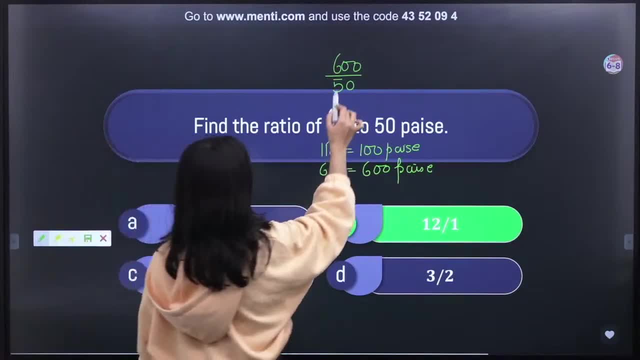 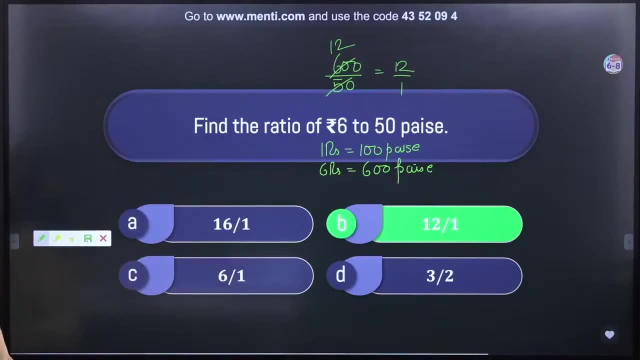 50 karna tha. to yeh kya ban gaya aapke paas, aapke paas 12 ban gaya to ratio aajayega aapka 12 is to 1 to ratio. aajayega 12 is to 1. 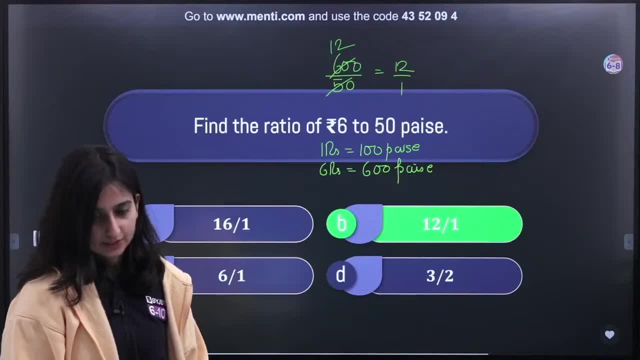 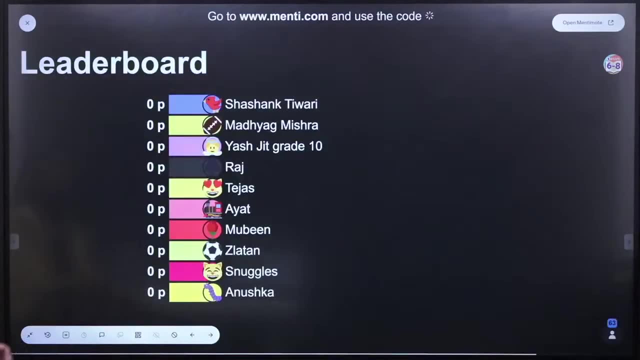 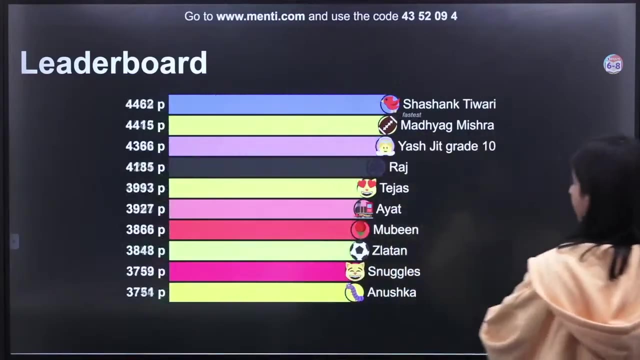 that is B option, chike chalye. so now it's time for the leader board. ok, so we have shashank, madhyag, yashjeet, raj tejas, ayat mubeen, zlatan, snuggles and anushka. these are the. 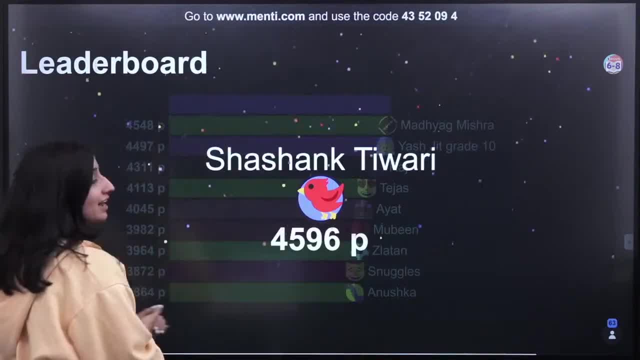 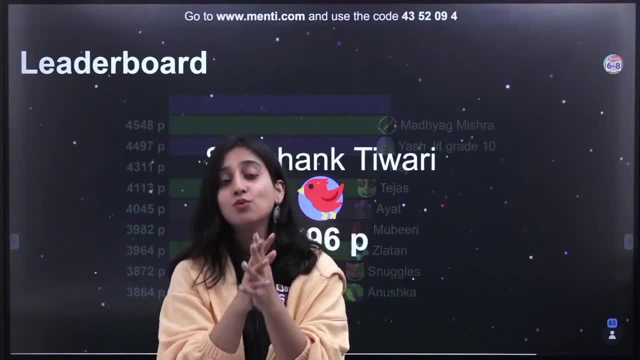 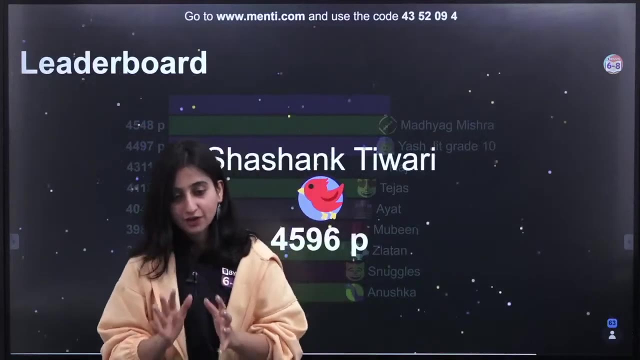 top 10 students in the leaderboard and shashank tiwari has won the quiz. very good, shashank, and very good to each and every one of you who have participated in the quiz. well done to all of you, very nice participation and kaafi acha. 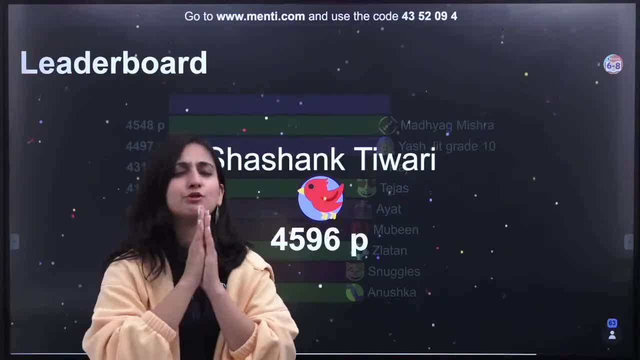 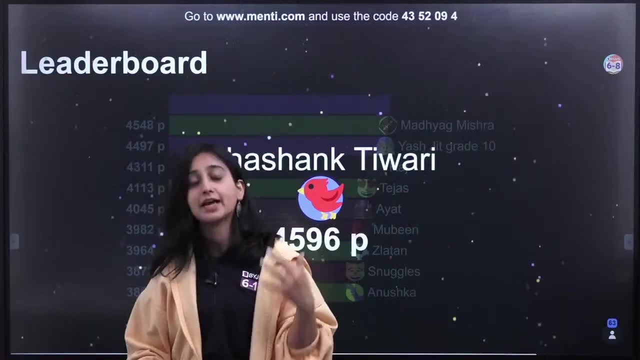 aapne perform bhi kiya hai. so i hope, aapko yeh chapter samajhme aaya hai. itna mushkil chapter nahi hai, agar aap isko dhyan se samjho, agar fir bhi thode bohat. 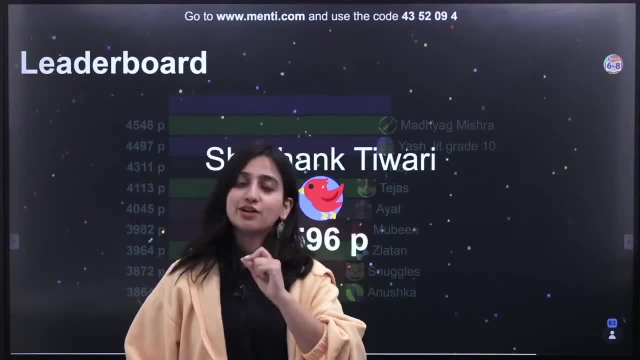 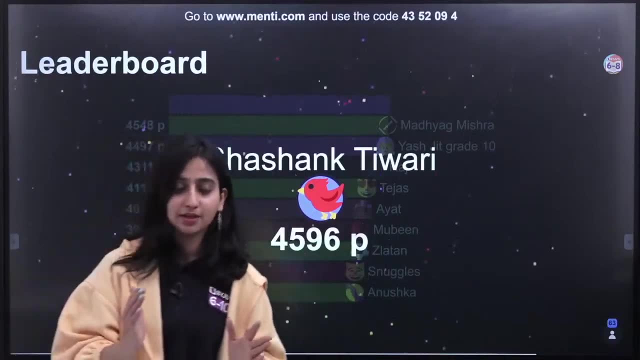 detail me ekdam padhne ke liye. make sure ki aap one short session zaroor dekhe. yeh crash course tha to isme, hamne sare concepts revise kiye, questions bhi solve kiye aur mentee bhi kiya. 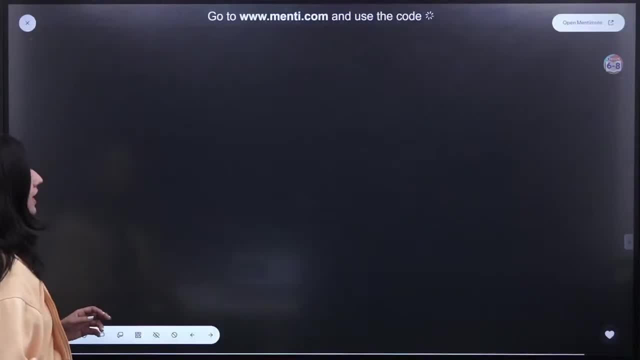 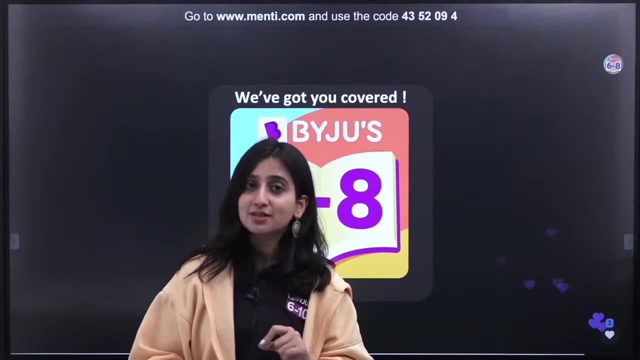 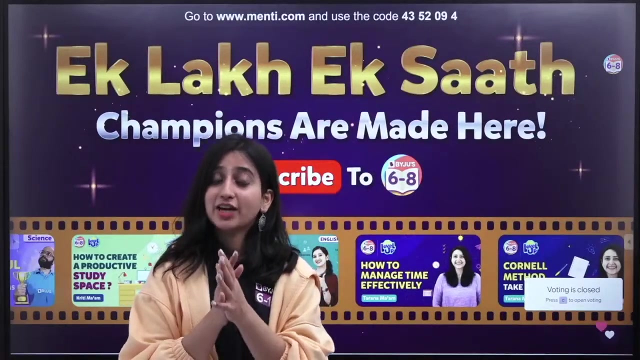 theek hai. so thank you so much for coming here. live with me this evening. right, and you know that advises we have got you covered. so make sure. if you haven't subscribed to the channel, yet, so make sure you subscribe, and do hit the like button and share the videos.